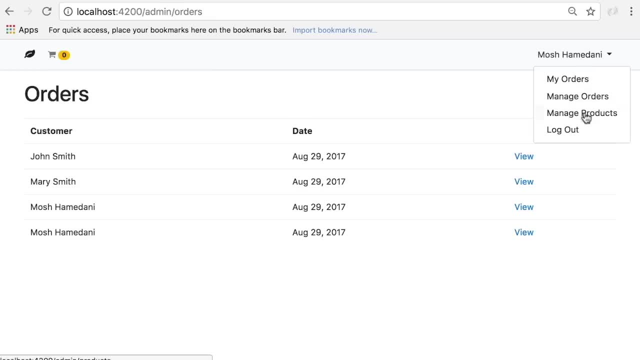 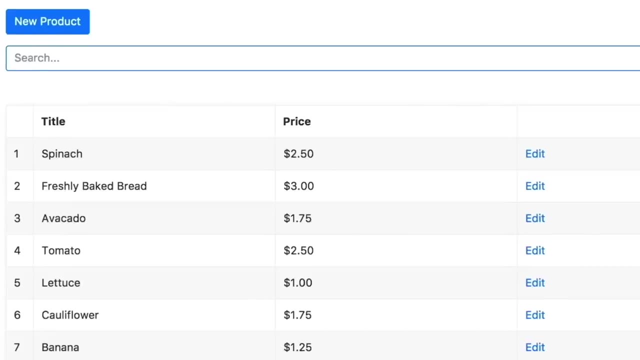 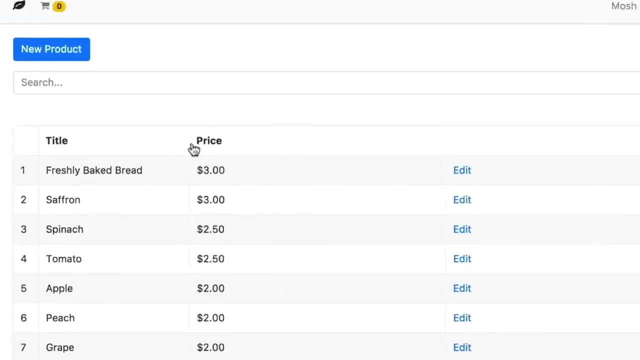 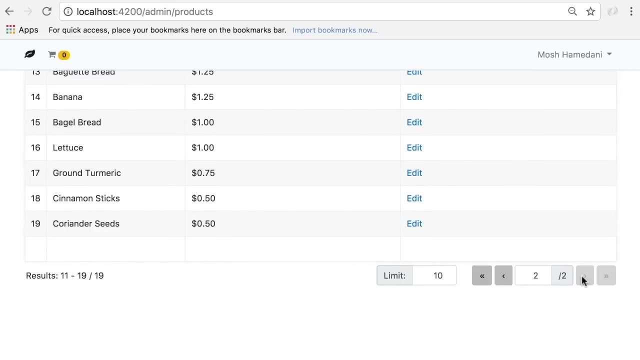 and authorization. As an admin, I can also manage the products. So here we have all the CRUD operations. We can quickly search for a product, You can sort the data, You can resize the columns or navigate to a different page. These are the patterns that you see in a lot of real world applications And in this course. 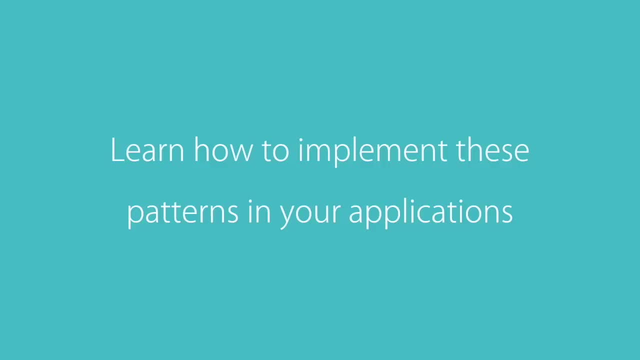 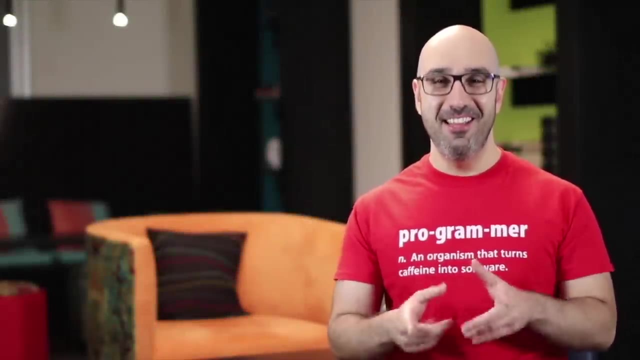 you're going to learn how to implement these patterns in your applications. So are you excited to learn Angular and build this application? Then let's jump in and get started. So you can clearly see right now that the product is here and some of the data, like 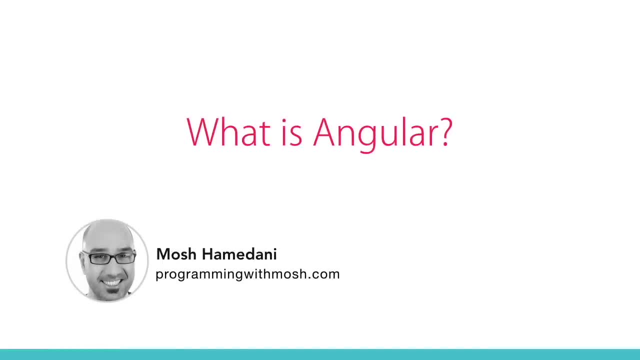 the inventory is here And when you click around you can see it. the website is here. So if we click on this email- and this is the address I'm at- we can see that there's some. So in case you're an absolute beginner with Angular, let me quickly explain in two minutes. 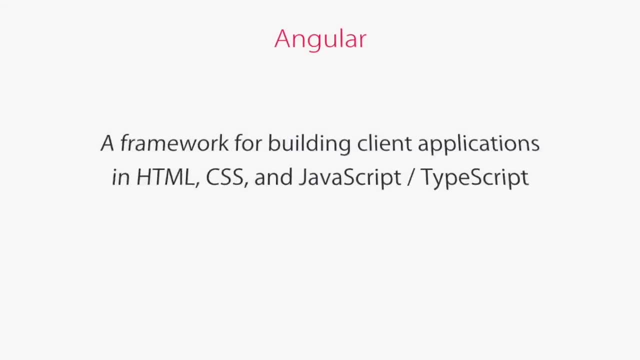 what Angular is and why you should learn it. Angular is a framework for building client applications in HTML, CSS and either JavaScript or a language like TypeScript that compiles to JavaScript. A TypeScript is more common in the Angular community because Angular itself has been 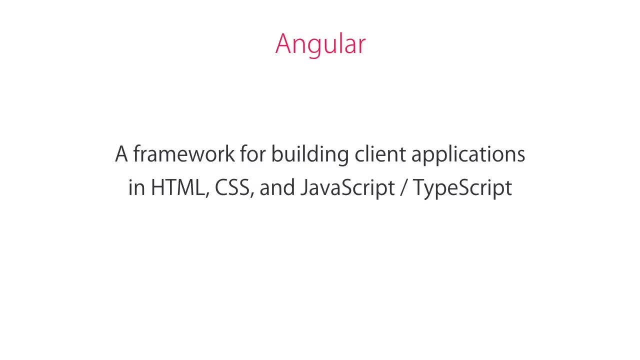 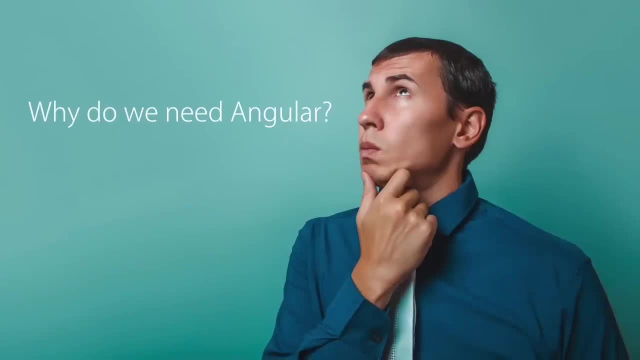 written with TypeScript. If you have never worked with TypeScript before, don't worry at all. It's very easy and you're going to get familiar with it in this course. Now, one question that a lot of beginners have is: why do we need Angular? 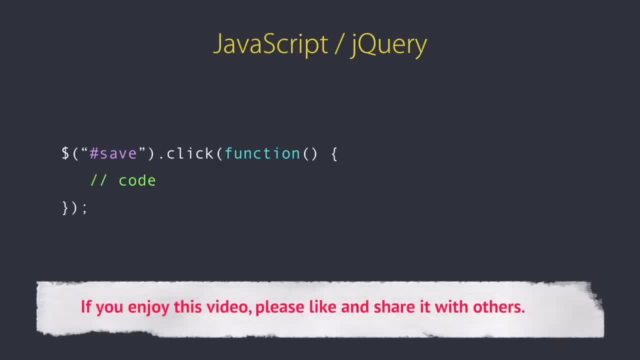 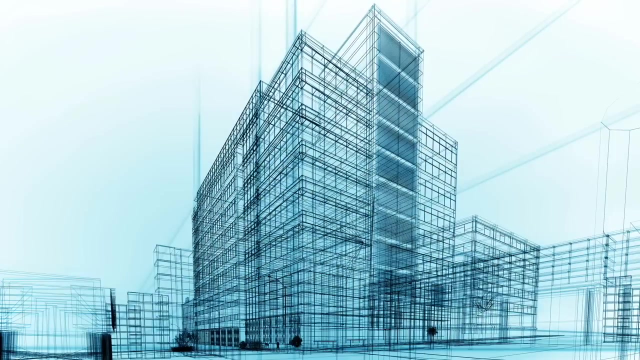 Can we not use plain old JavaScript or jQuery? We certainly can, and that's how a lot of web applications out there are built. But as our applications get more complex, vanilla JavaScript or jQuery code becomes hard to maintain. We need a way to properly structure our application. 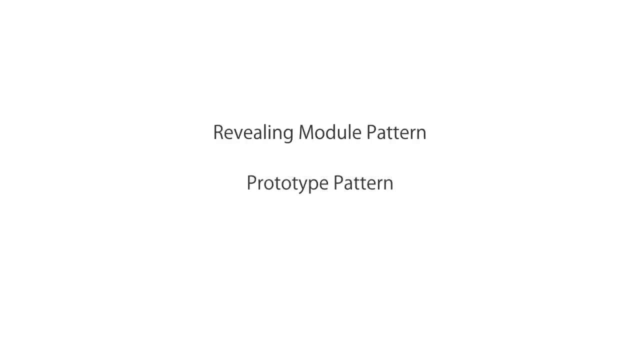 Sure, there are JavaScript patterns out there that help us with the structure, But these patterns are hard to understand for a lot of beginners to JavaScript. Plus, a lot of applications built with vanilla, JavaScript or jQuery are hard to test, And that's why, over the past few years, various frameworks have been built and evolved to 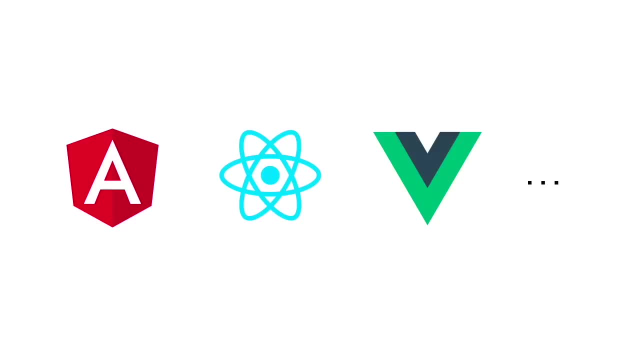 make web application development easier. Angular is an example of such frameworks. It gives our applications a clean and loosely coupled structure that is easy to understand and easy to maintain. It also brings in a lot of utility code that we can reuse in various applications, especially. 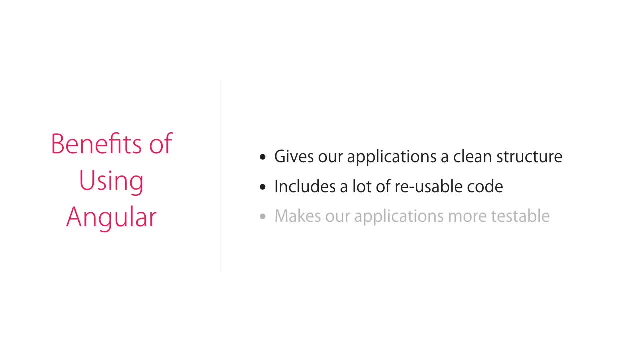 when dealing with the user's navigation and the browser history. Plus, applications built with Angular are more testable, so we can easily write automated tests to test various parts of our application, as I will show you later in the course. So to answer this question, no, you don't need a framework like Angular to build client. 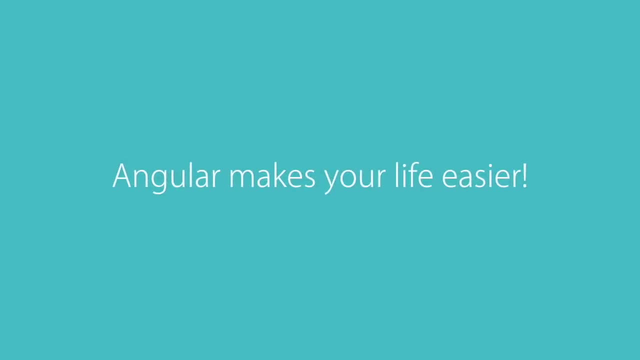 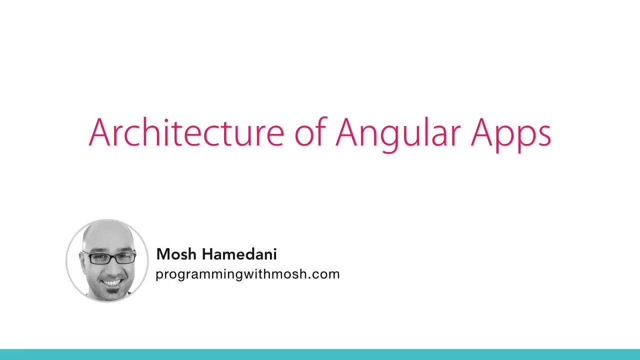 applications, but using Angular makes your life a lot easier. Alright, now that you know what Angular is, let's take a look at the architecture of Angular applications. A lot of modern applications have at least two parts: a front end and a back end. 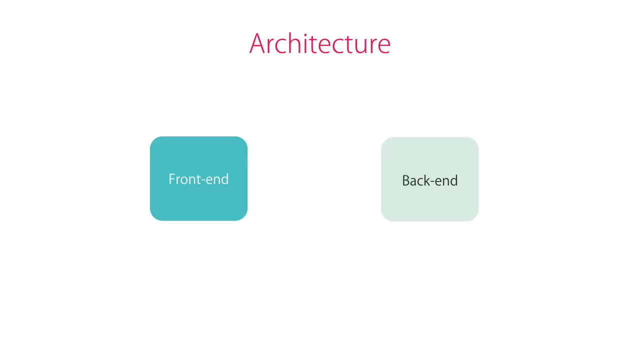 The front end, also called the client, is the part that runs in a web browser and this is what the user sees and interacts with. So it essentially includes the user interface or UI of an application. We use HTML, CSS and C++. 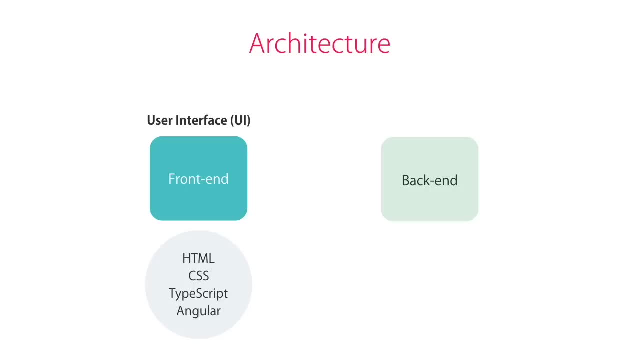 We also use JavaScript. We also use JavaScript, TypeScript and Angular to build the front end. The back end sits on a web server or multiple web servers in the cloud and is responsible for storing the data and doing any kind of processing. Our front end, or the client app, talks to the back end to get or save the data. 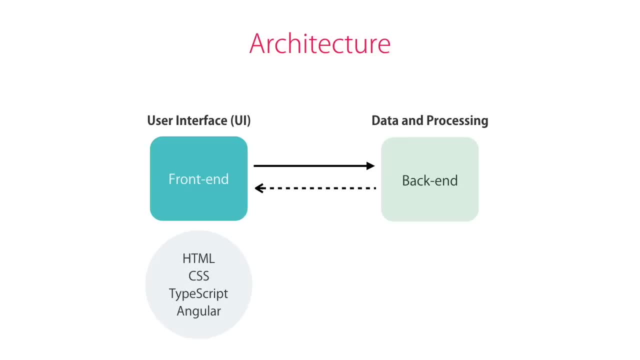 One of the questions that a lot of beginners ask me is: Mosh, how do I save my data in Angular? Well, you don't. In most cases, you don't save the data on the client Because you don't have to do that. 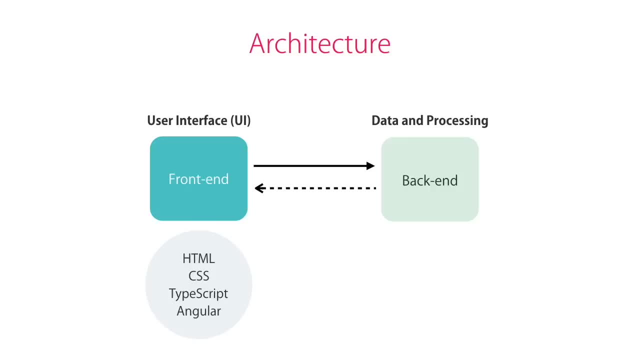 it can easily disappear as the user clears the browser data or moves to a different computer. that's why, if you store the data on the server, so here- we often have one or more databases, as well as a bunch of HTTP services or API's to make this data available to the clients. in case you don't know, API stands for: 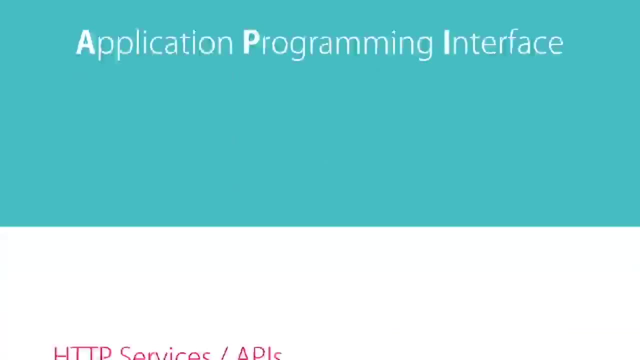 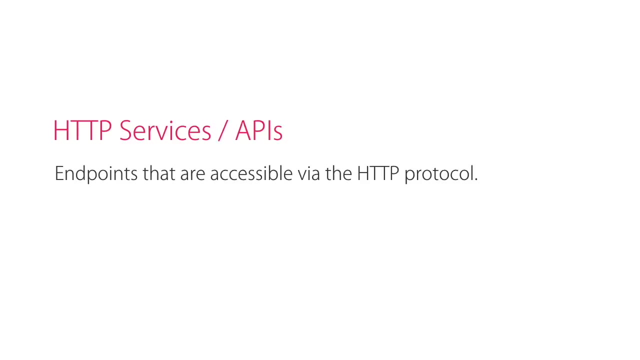 application programming interface. now, if you put this fancy name aside, these HTTP services or API's are essentially endpoints that are accessible via the HTTP protocol, so we can call them using simple HTTP requests to get or to save the data. if that's too much technical jargon here, let me give you a metaphor. 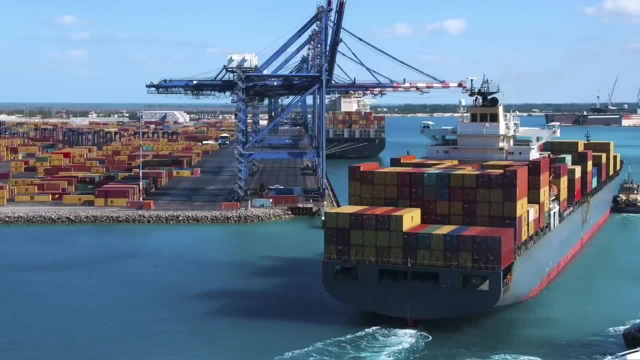 think of a port where ships load or unload. these are points to get loads in and out of a town right now. imagine these ports are HTTP endpoints. ships are HTTP requests and loads our data. so just like we can send a ship to a port to get some load and bring to us, a client app sends an HTTP request to an endpoint. 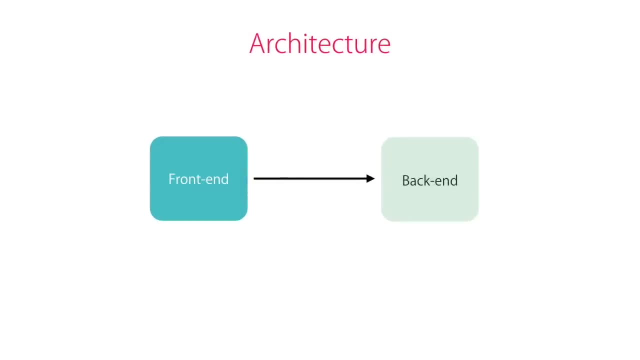 to get some data. so this is how the big picture works. our web applications have a front-end and a back-end. on the back end we have one or more databases and API's that make the data available to the clients for a large application around a complex domain. 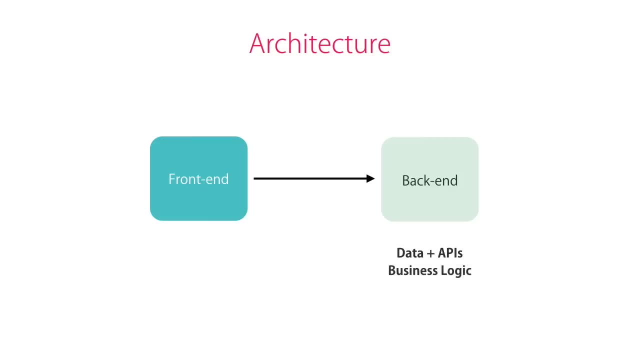 this is where we implement the business logic of the application, like calculating the tax and shipping cost based on various parameters. the front-end, or the client, on the other hand, is all about the presentation. so here we have our HTML templates as well as the presentation logic of our application. this logic is all about displaying data and responding. 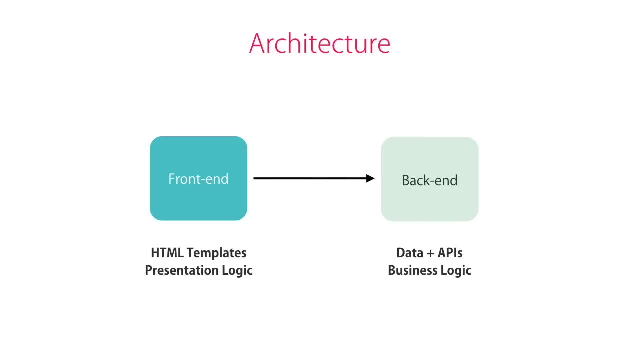 to user actions, like what should happen when the user clicks on a button that or navigates away from a page. these are examples of the presentation logic, or the logic that is all about the presentation aspect of an application. now, in terms of the implementation, building the back-end requires familiarity with other languages and frameworks, and that's completely outside the 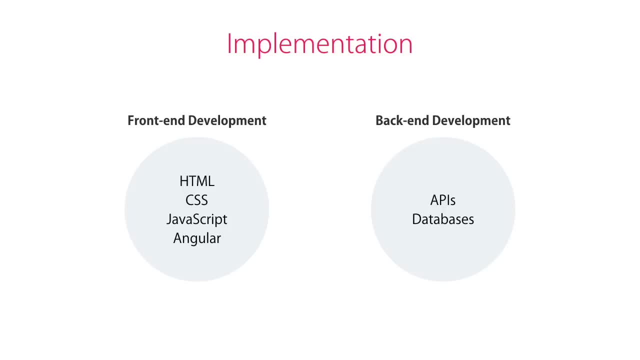 scope of building client apps with angular. so, as an angular or a front-end developer, you don't have to worry about this. this is the job of a back-end developer or a full-time stack developer who knows both the front-end and the back-end. so, for the purpose of this course, 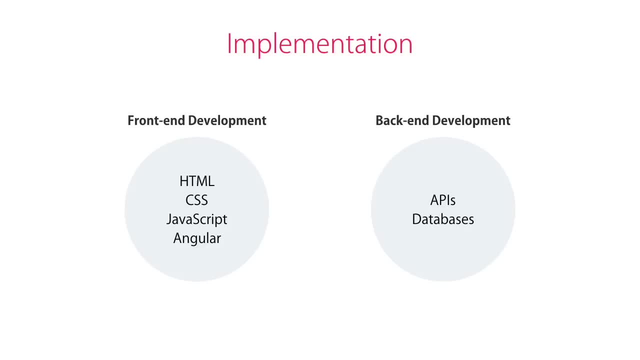 we're going to focus on the front-end, and if you want to learn about the back-end development, you can always pick up a course later down the road. but for now, let's just focus on one thing and do it well. all right. in this lecture, I'm going to show you how to set up your development environment. 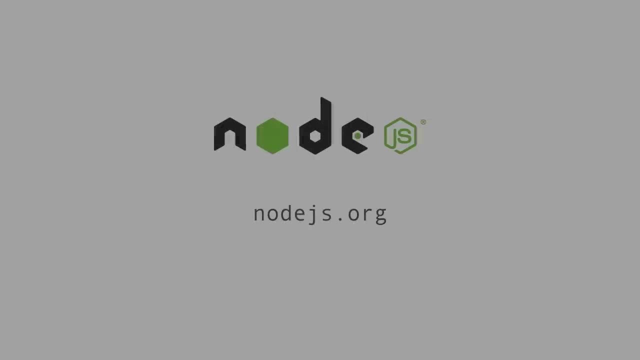 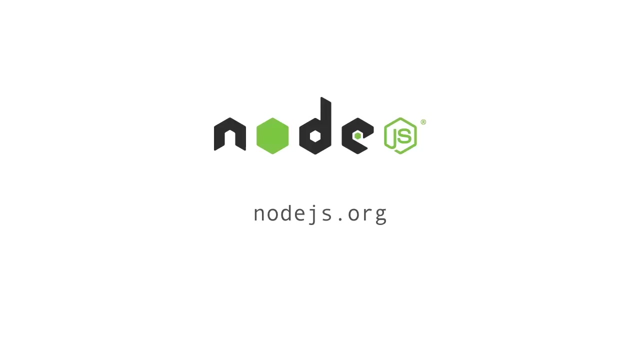 and create your first angular project, so the first thing you need to install is the latest version of node. in case you have never worked with node before, it's basically a runtime environment for executing javascript code outside the browser. in this course, we're not going to work with node, but 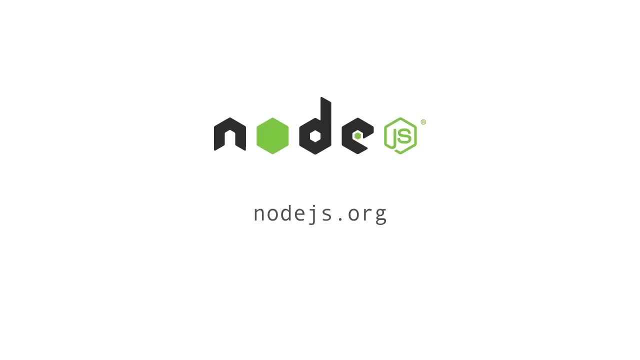 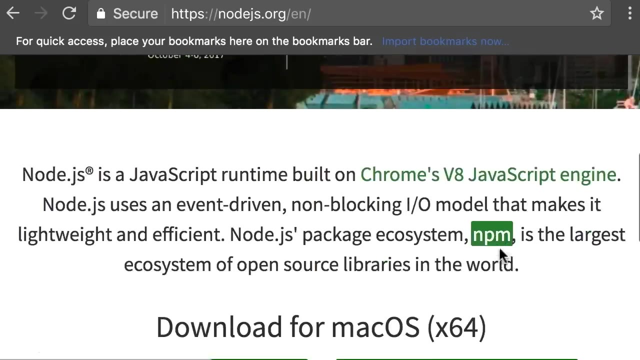 node provides some tools that we need to build angular projects. so if you haven't installed node, head over to nodejs org. on this page you can see the latest version of node for your operating system. so here the latest stable version is six point eleven and the latest version of node is 6.11. 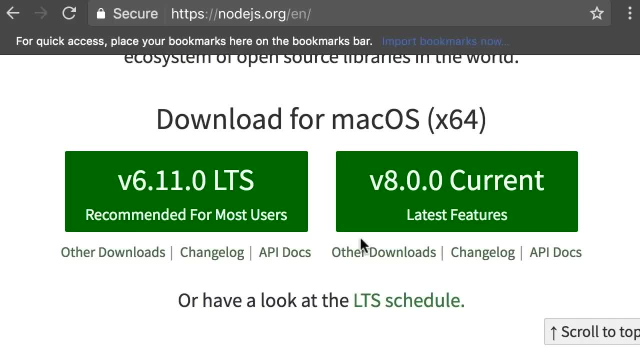 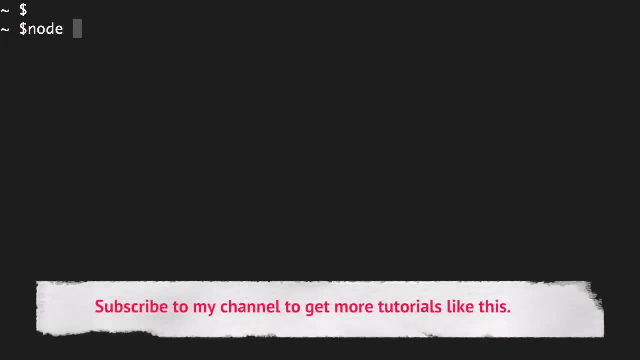 latest version is version 8.. Now this latest version has more features, but it's not quite stable yet. So go ahead and install the latest stable version. When you do that, open up the terminal on Mac or command prompt on Windows and type node dash, dash version. 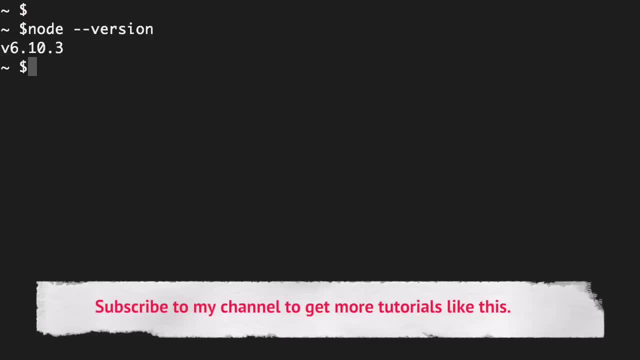 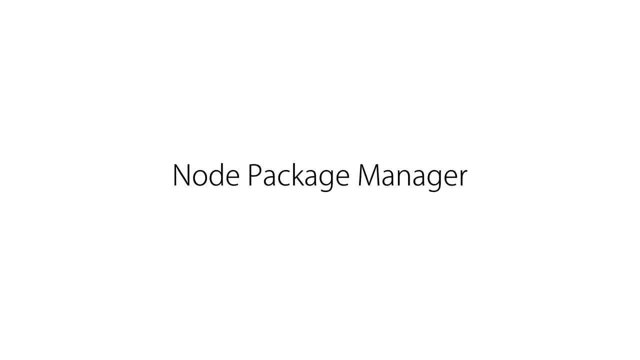 So you can see, on my machine I'm running node version 6.10.. The minimum version required for building Angular applications is version 6.9.. Once you have node, then we're going to use a tool called node package manager or NPM. 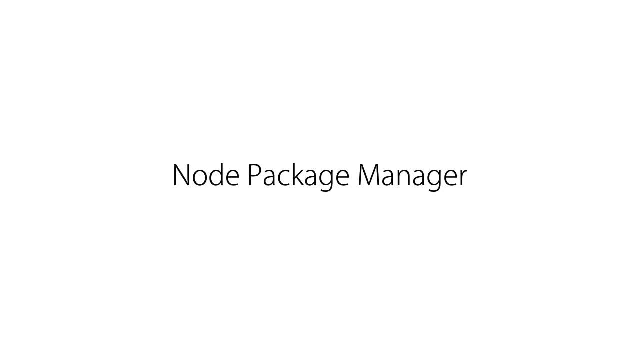 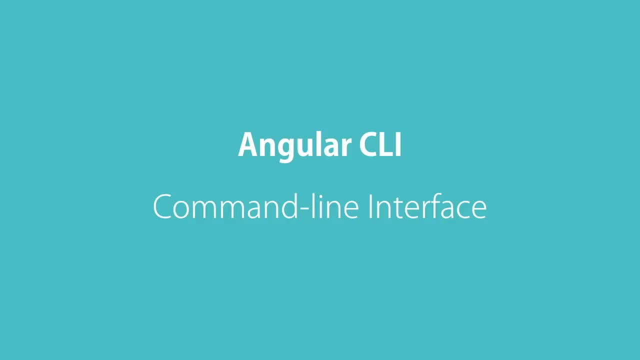 to install third party libraries. One of those libraries we're going to install in this lecture is Angular CLI, which stands for command line interface. So it's a command line tool that we use to create a new Angular project or generate some boilerplate code, as well as create deployable packages. 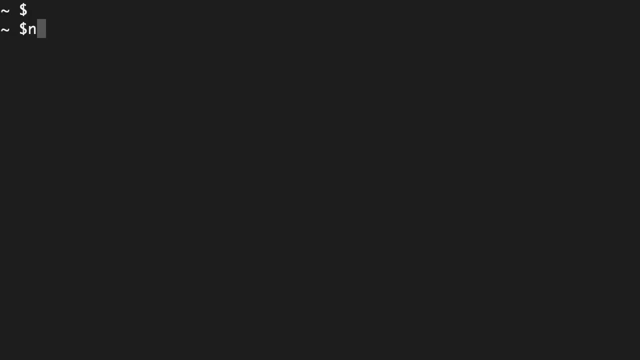 So once again in the terminal we run NPM, install dash G, which stands for global, and finally the name of the package which is at Angular slash, CLI. If you don't put dash G here, Angular CLI will be installed only in the current folder. 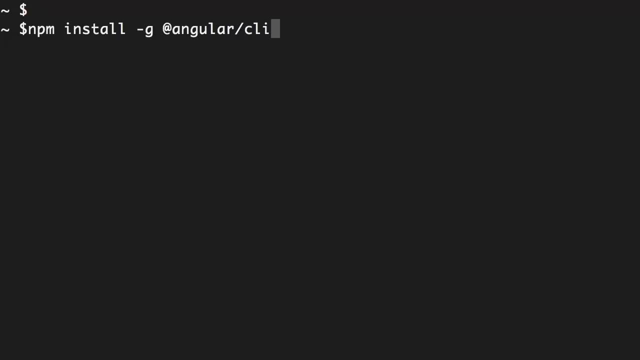 and it's not going to be accessible anywhere else. Now, if you're on Mac, you need to put sudo at the beginning of this command to execute it as an administrator, Alright. next we need to enter our password, and now this process is going to take a little while. 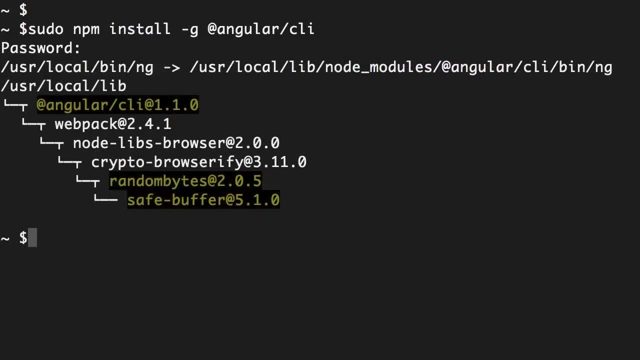 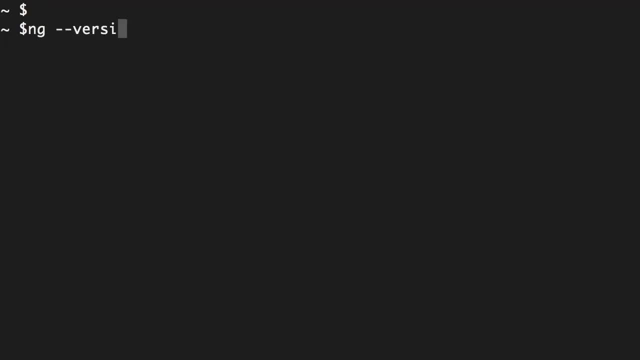 Alright, beautiful. we installed Angular CLI. now, to ensure that the installation was successful, we can type ng dash dash version so you can see I'm running Angular CLI version 1.1.0 and below that you can see the version of node on. 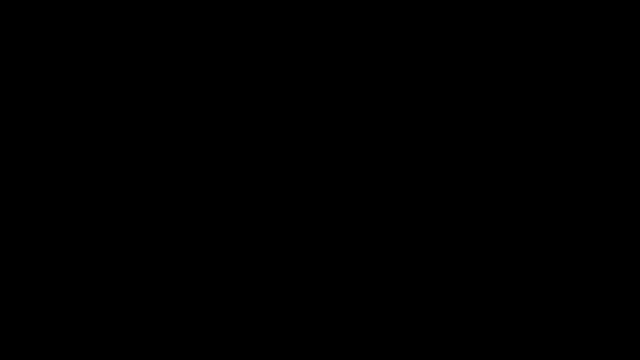 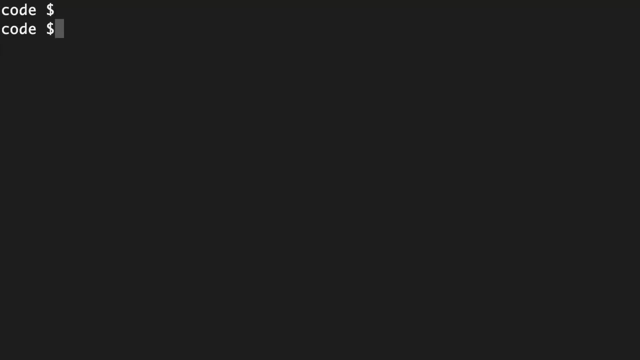 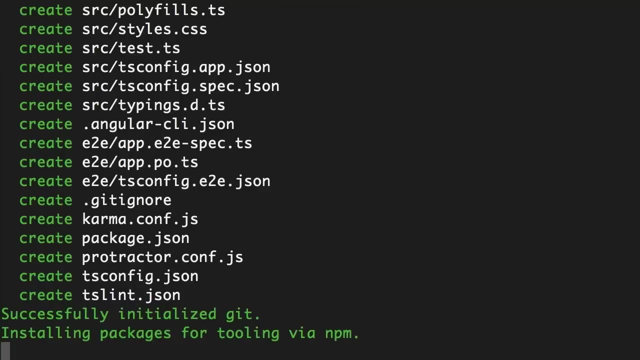 my machine Once again, it's 6.9. 10. So with Angular CLI in place now we can create a new Angular project. So we type ng new and let's call this project hello dash world. So this generates a bunch of files and folders and then it's going to use. 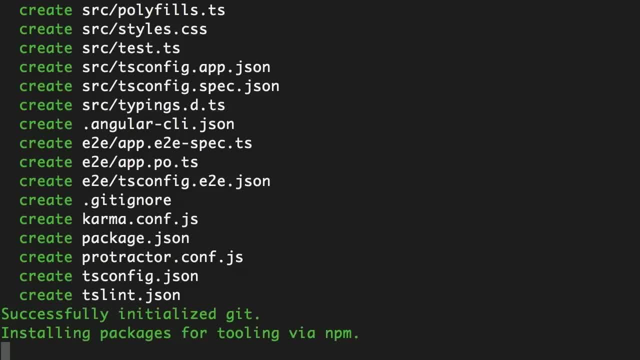 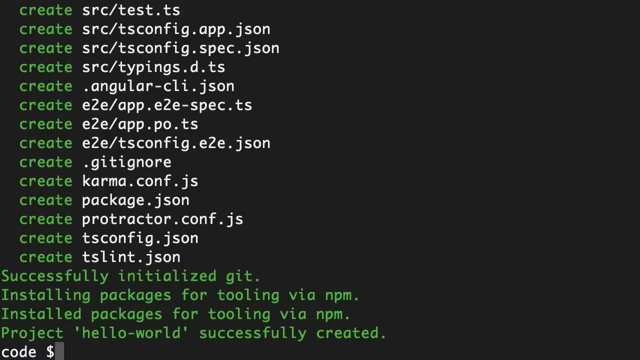 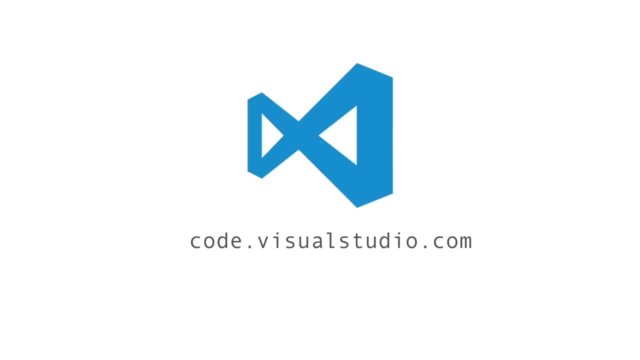 NPM to download the third-party libraries. Alright, our project is successfully created. Now to start coding, we need a code editor. the editor I'm going to use in this course is Visual Studio code or VS code. it's a beautiful, cross-platform, lightweight editor and you can download. 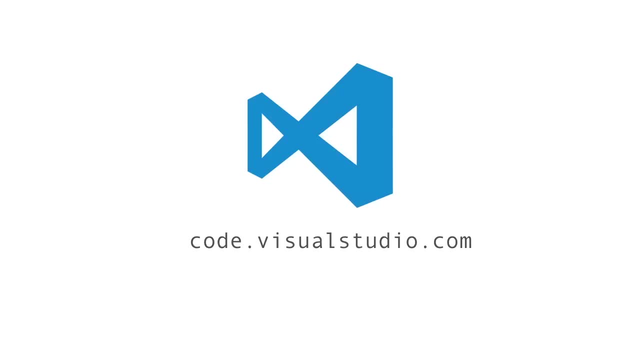 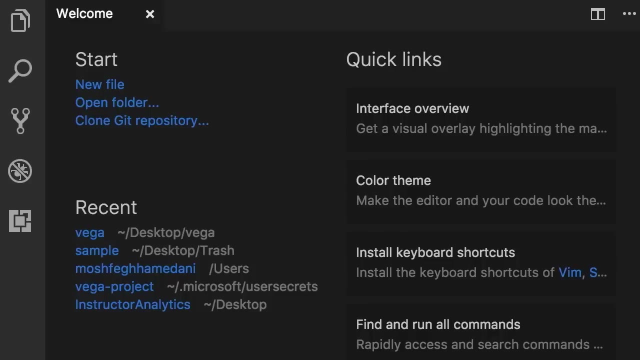 at codevisuallstudiocom. If you don't like this editor, feel free to use any editors that you prefer. you can use Sublime, you can use AddAMP or any other editors. Now, if you're going to use VS code, it's difficult to get them together. 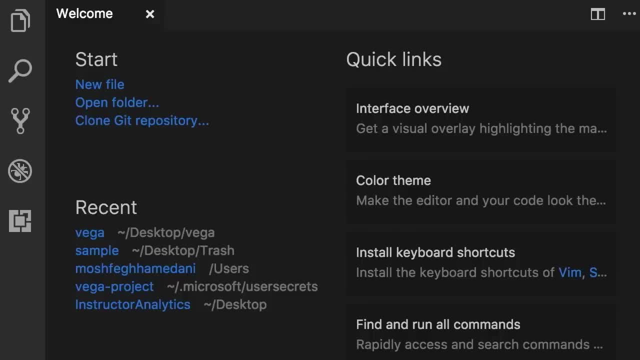 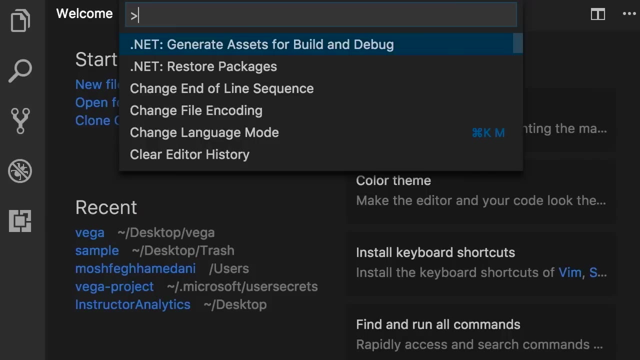 use vs code. i want you to add it to the path so you can easily open it from the terminal. so here, if you're using mac, press shift, command and p, or if you're using windows, press shift, control and p, this opens up the command palette. now here type code. 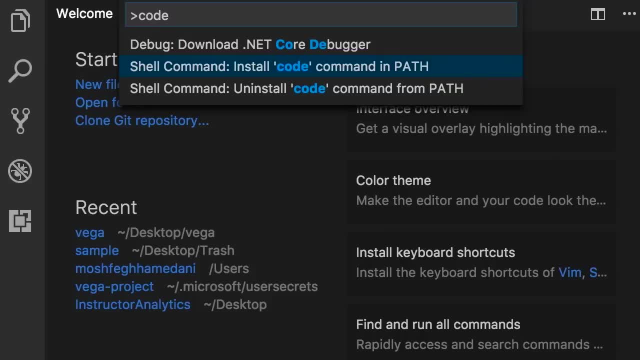 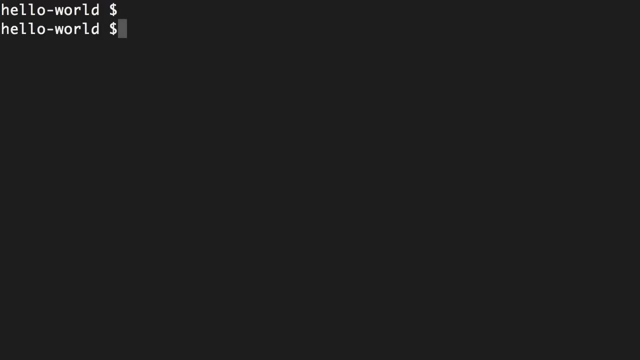 look at this command here. install code command in path. with this we can go to the terminal in the folder where we created a new project, hello world. simply type code period. so this opens up vs code pointing to the current folder. now, in the next lecture, we're going to look at this structure. you're going to learn. 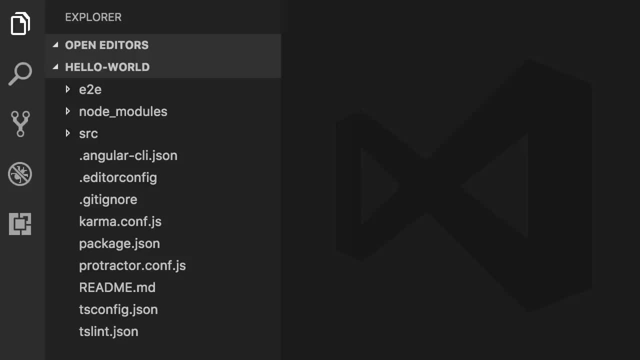 what files and folders we have here. but before we get there, let's make sure that this application works. so back in the terminal. once again, we use angular cli to load our application and we're going to load our application. and we're going to load our application. 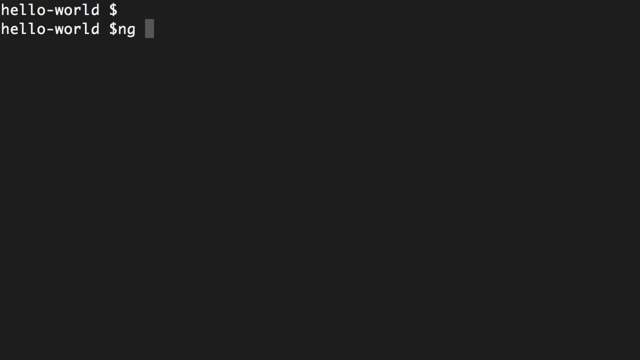 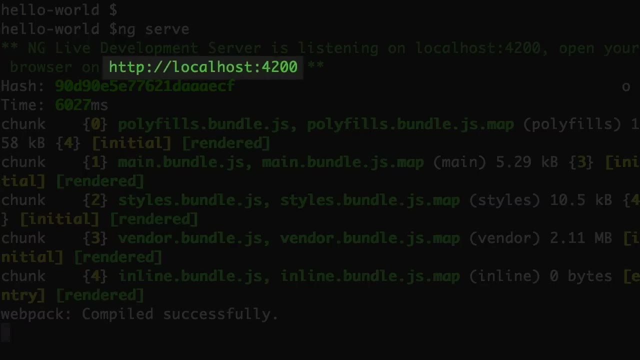 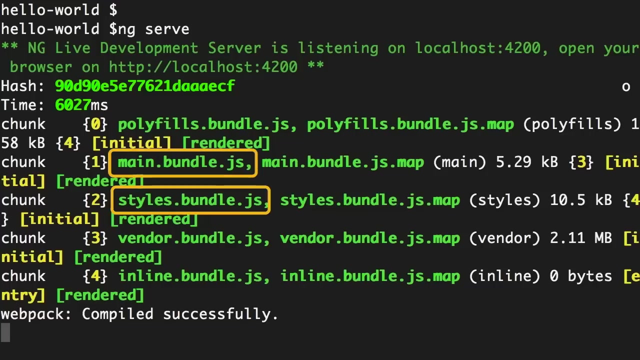 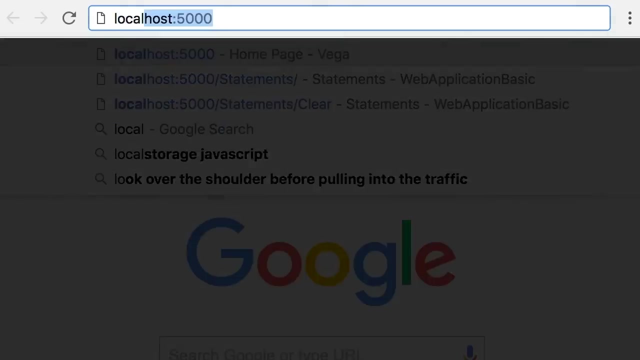 in a web server so we type ng space serve. so now we have a live development server listening on localhost port 4200, and angular cli also compiled our application. it generated bundles for javascript and css files so we can open up chrome and head over to localhost port 4200. beautiful, this is our 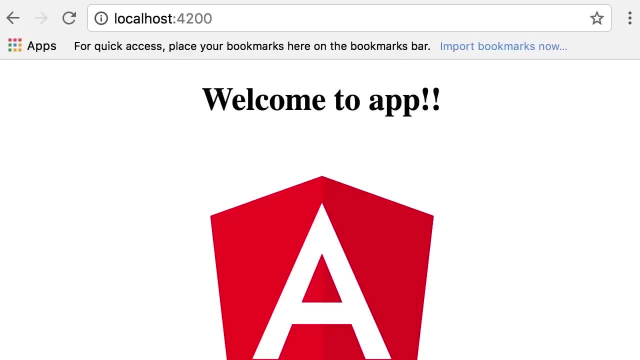 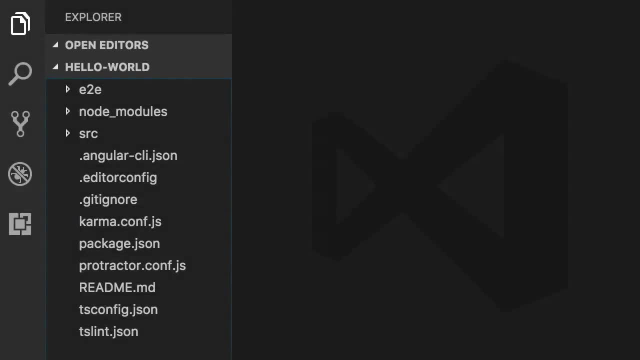 first angular app. next we're going to look at the structure of our new angular project. all right, now let's see what files and folders we have in this new project. so the first folder we have here is e2e, which stands for end-to-end, and this is where we write. 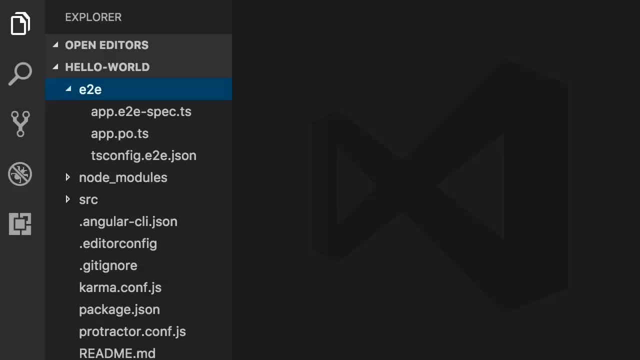 end-to-end tests for our application. if you have not worked with end-to-end tests, these are basically automated tests that simulate a real user so we can write code to launch our browser, email orkun and willy and like to see all the stuff that's happening on our system. so that's. 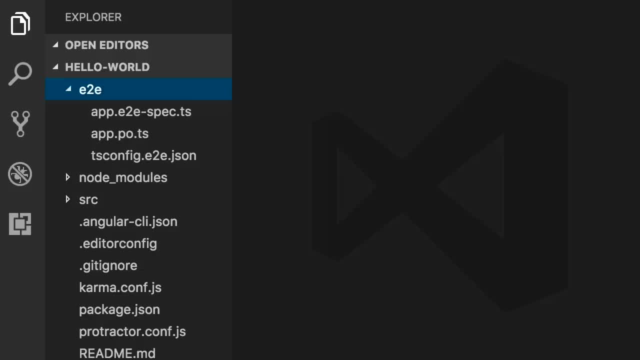 navigate to the home page of our application, click a few links here and there, fill out a form, click a button and then assert that there is something on the page. This is an example of an end-to-end test. Now, that's. 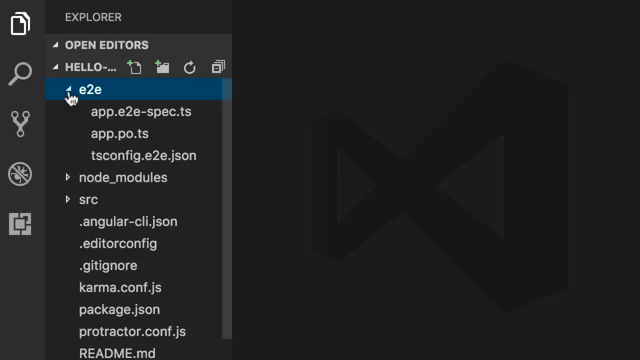 beyond the scope of this course, so we don't have to worry about it yet. Below that we have node modules, and this is where we store all the third-party libraries that our application may depend upon. Now, this folder is purely for development, so when we 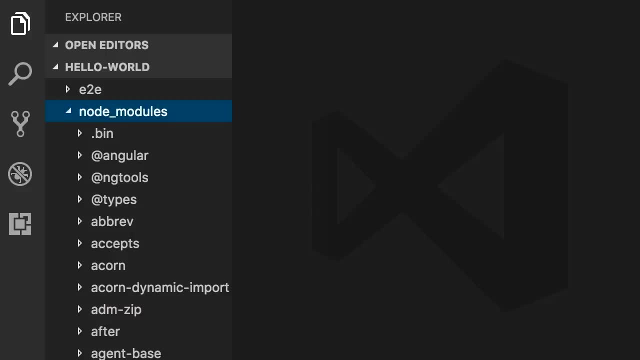 compile our application. parts of these third-party libraries are put in a bundle and deployed with our application. So we're not going to deploy this node modules folder to a server. You're going to see this later in the course Below that we have. 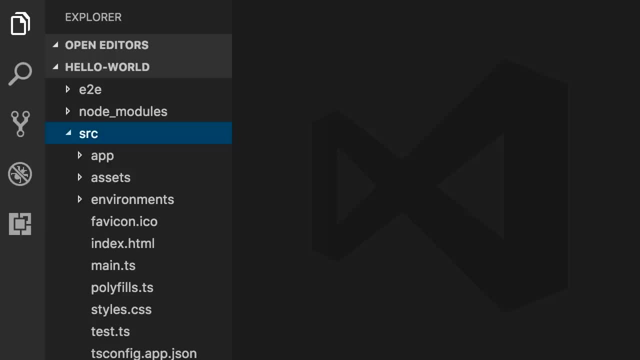 the source folder, and this is where we have the actual source code of our application. So we have this app folder here and inside this folder we have a module and a component. So every application has at least one module and one component. You're going to get familiar with these components and modules very soon. 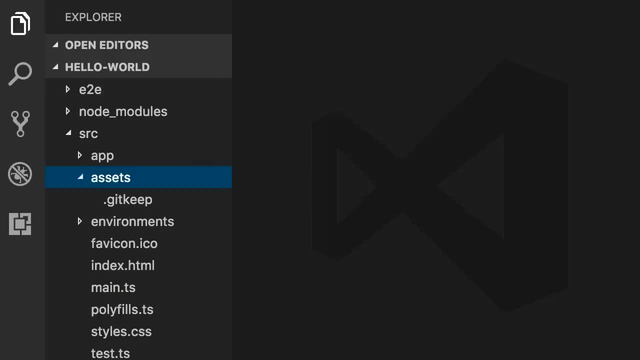 Below that, we have this assets folder where we store the static assets of our application. So if we have any image files, any text files, any icons, all of these go here. Below that, we have this environments folder and this is where we store configuration settings for different environments. 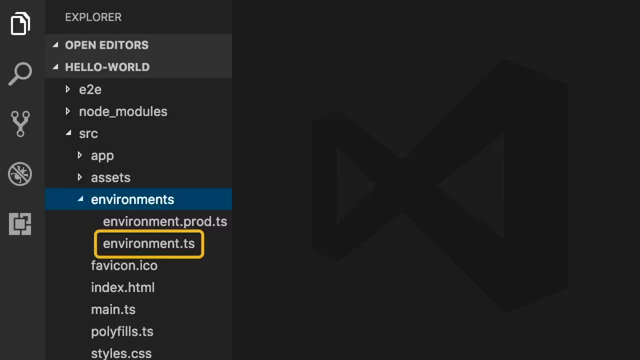 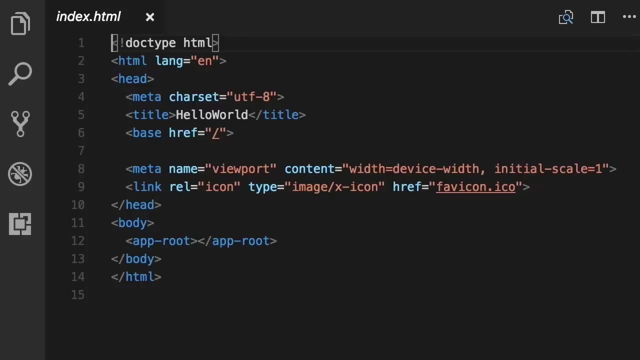 So we have one file for the production environment and the other for the development environment. Now the other files we have in the source folder are favorite icon, which is the icon displayed in the browser. We have indexhtml, which is a very simple HTML. 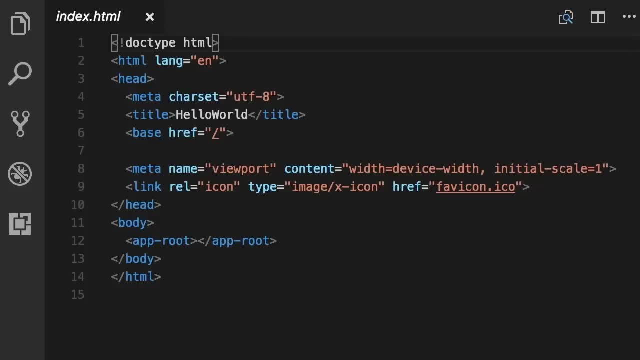 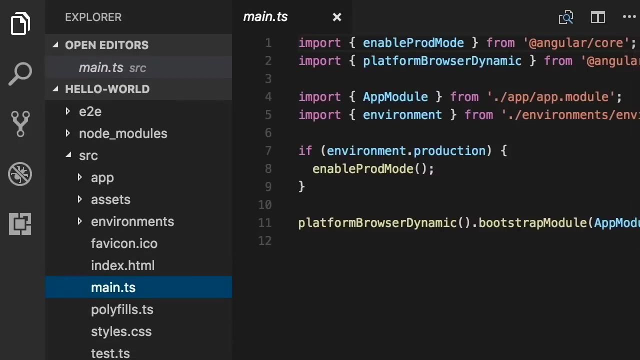 file that contains our Angular application. So note that here we don't have any references to a script or a style sheet. These references will be dynamically inserted into this page, as I will show you later in the course Below that we have this main file, which is a TypeScript file, and 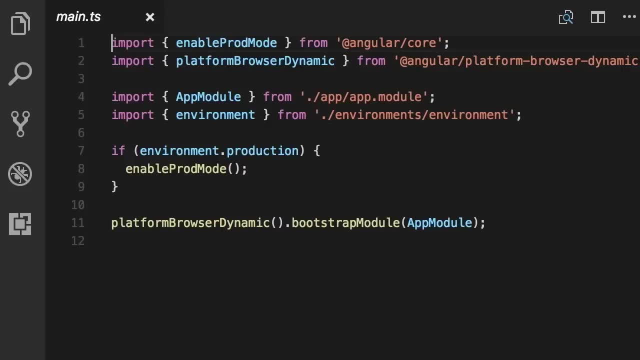 this is basically the starting point of our application. So in a lot of programming languages we have this concept of the main method, which is the starting point of a program. We have the same concept in our Angular applications. So all we're doing here is bootstrapping the 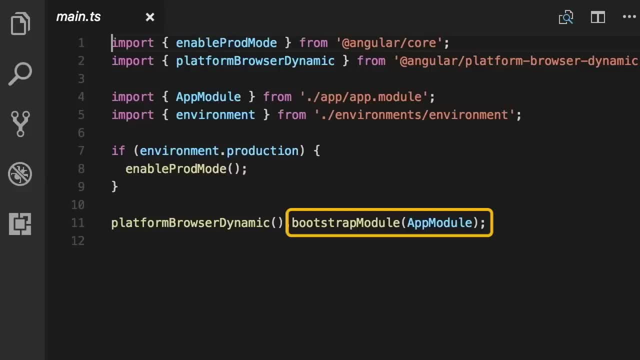 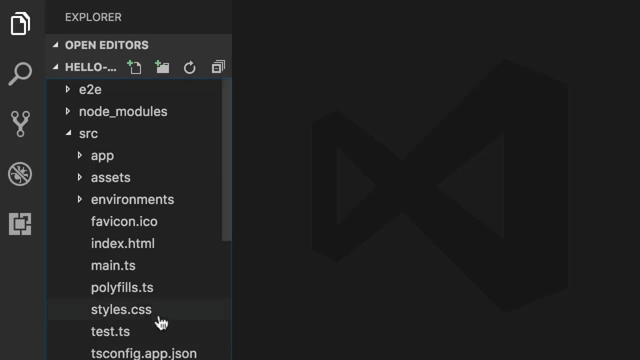 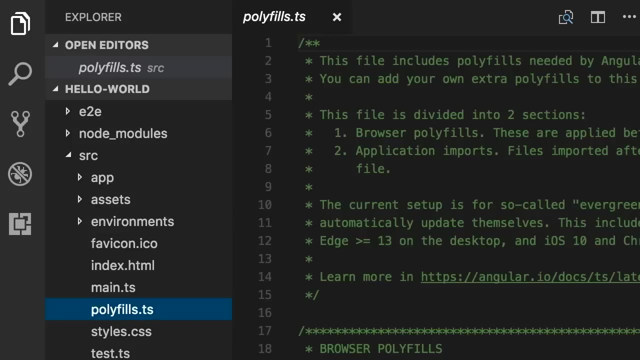 main module of our application, which is, in this case, app module. So Angular loads this module and everything else starts from there. We have this polyfills file, which basically imports some scripts that are required for running Angular, because the Angular framework uses features of JavaScript that are not available in the current 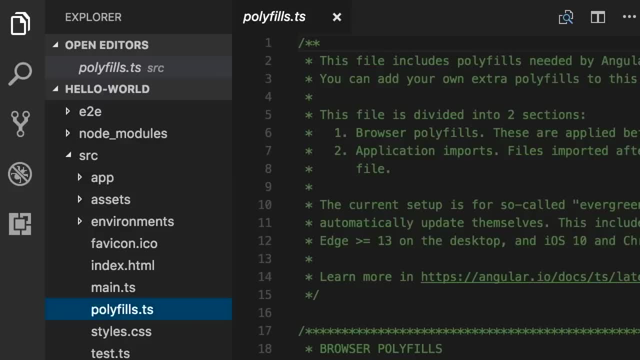 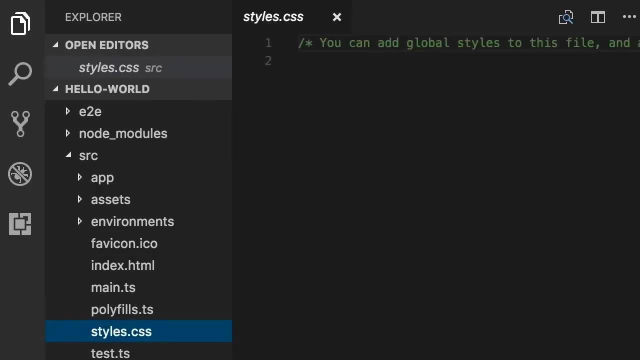 version of JavaScript supported by most browsers out there. So these polyfills fill the gap between the features of JavaScript that Angular needs and the features supported by the current browsers. Below that, we have stylescss, and this is where we add the features of JavaScript that we need. 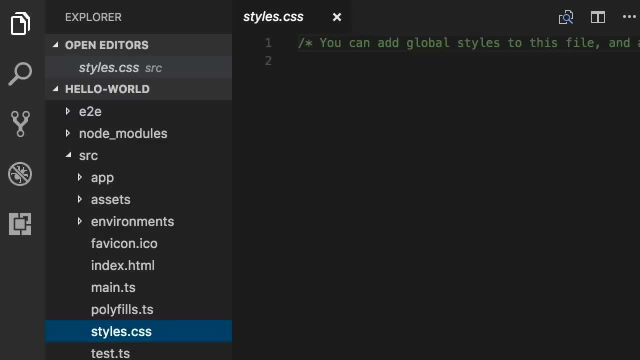 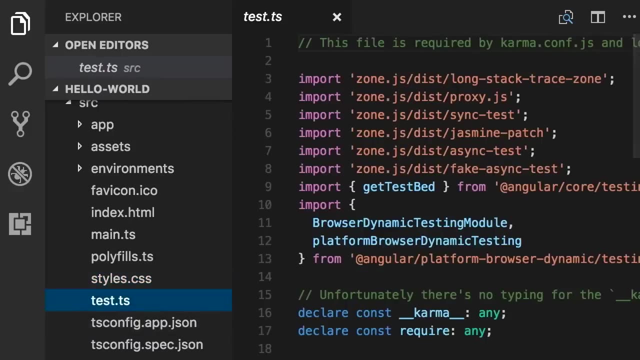 We add the global styles for our application And also each page or each component can have its own styles. as you will see later in the course Below that, we have testts, which is basically used for setting up our testing environment. Again, for now we don't have 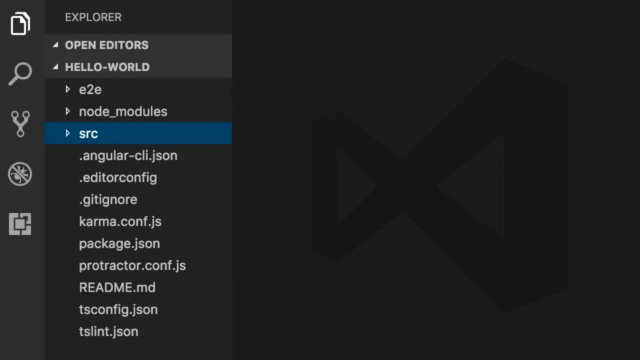 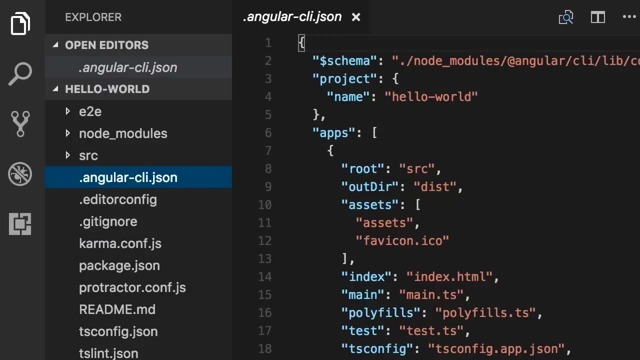 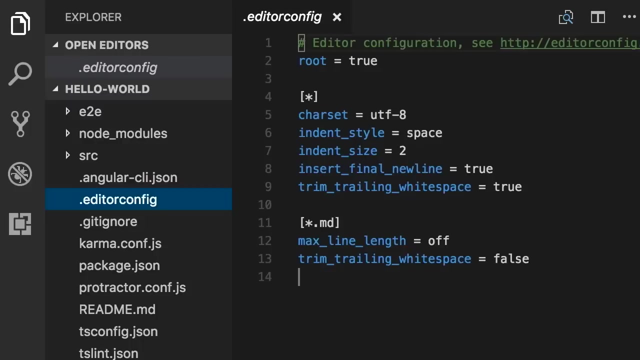 to worry about this. Outside the source folder we have a configuration file for Angular CLI. It's pretty standard configuration. You don't have to worry about this for the most part. Below that we have editor config. So if you're working in a team environment, you want to make sure. 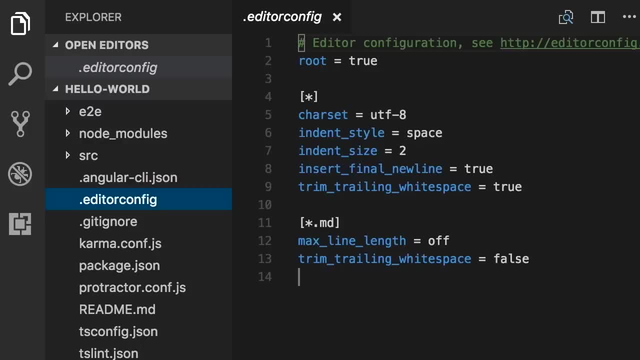 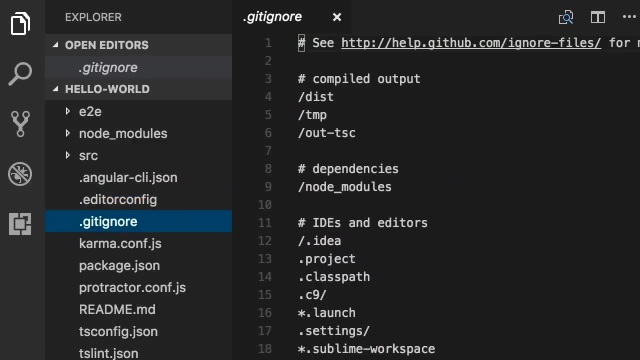 that all developers in the team use the same settings in their editors, So this is where you store your settings. We have this git ignore file, which is basically for excluding certain files and folders from your git repository. If you have not worked with git, don't worry, It's not something that you need to know in order to. 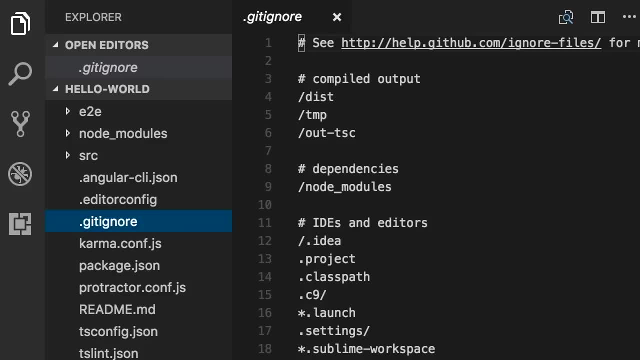 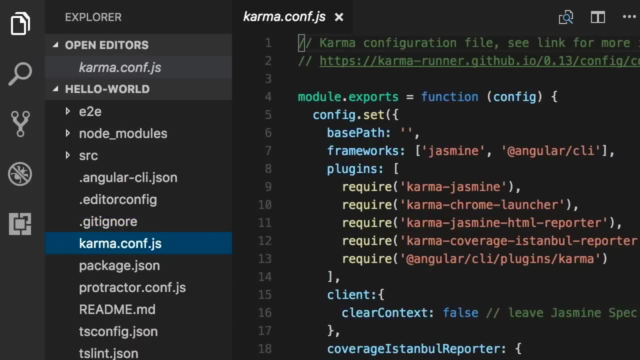 build applications with Angular. It's basically a tool for managing and versioning your source code. Now, below that, we have karmaconfigjs, which is a configuration file for karma, which is a test runner for JavaScript code. Again, we're not going to worry. 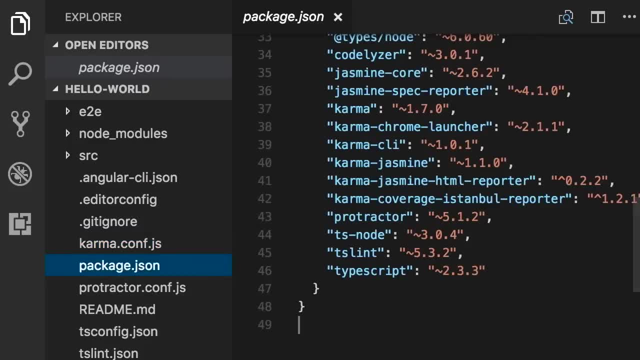 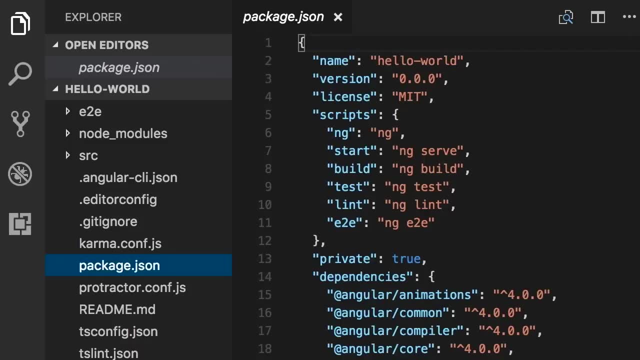 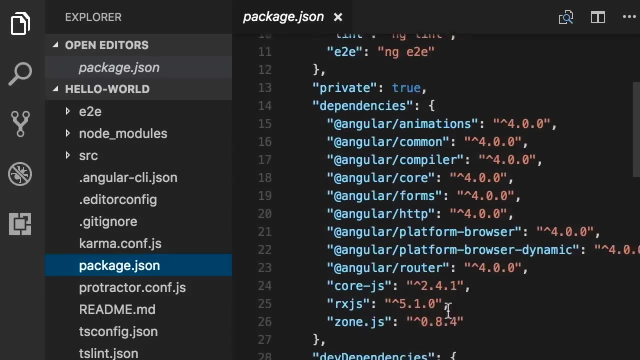 about running tests at this stage. Now, below that we have an important file, packagejson. Now, this is a standard file that every Node project has. Apart from a bunch of basic settings here, like the name and version of your application, we have this setting here. 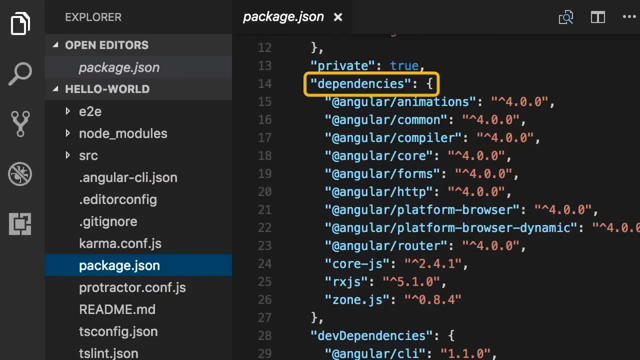 dependencies, which determines the libraries that your application is dependent upon. So here you can see, we have nine references to Angular libraries. All these libraries start with at Angular and after that we have the name of the library. So the first library here is for animations. 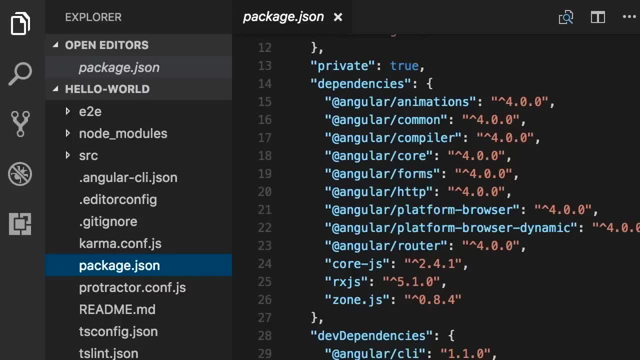 If you're not going to use animations in your application, you can delete this here. So in the future, as we use third-party libraries, you will see them listed here under the dependencies. Now, below that, we also have another setting or another key called. 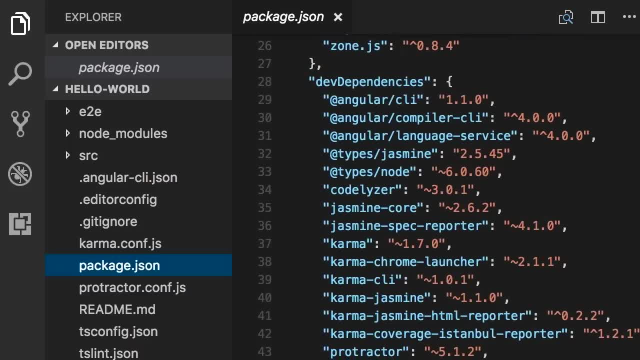 dev dependencies, And these are the libraries that we need in order to develop this application, So we don't need these to run our application on a production server. These are purely for a developer machine. So here we have a reference to Angular CLI, which you're already familiar with. 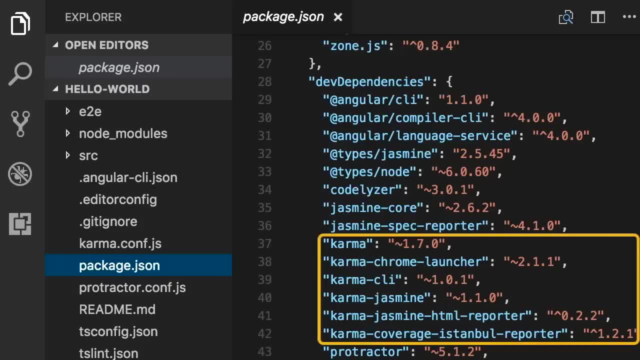 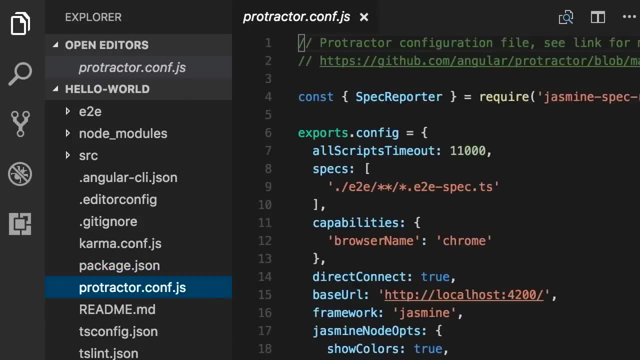 We also have a few other references to karma, which is again a test runner for JavaScript code. Below this packagejson we have protractorconfigjs, which is basically a tool for running end-to-end tests for Angular. Again, we're not going to worry about it. The end of the file here. 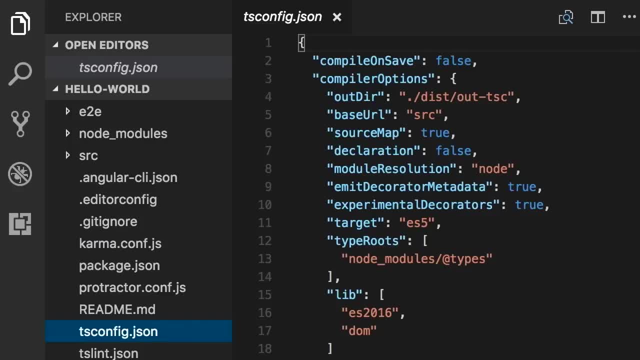 is tsconfig, which has a bunch of settings for your TypeScript compiler. So your TypeScript compiler looks at these settings and, based on these settings, is going to compile your TypeScript code into JavaScript that browsers can understand. Again, for the most part, any of these here. just be aware that if in the future in a complex project, 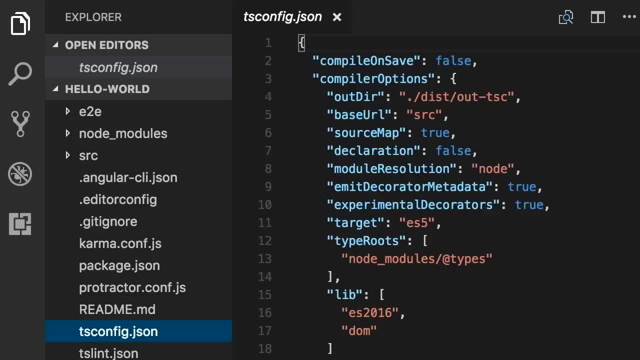 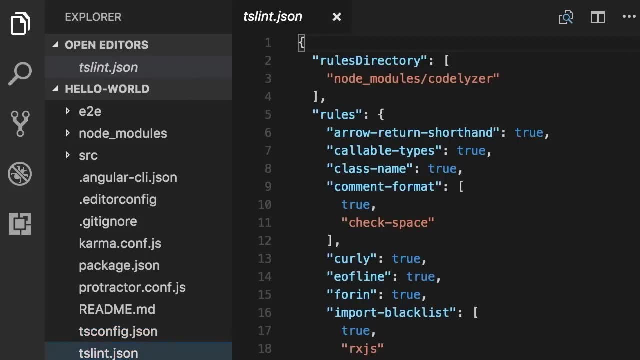 you need to change your TypeScript compiler settings. this is where you need to apply your changes. And finally, we have tslintjson, which includes a number of settings for tslint. In case you don't know, tslint is a static analysis tool for TypeScript code, So it checks your TypeScript. 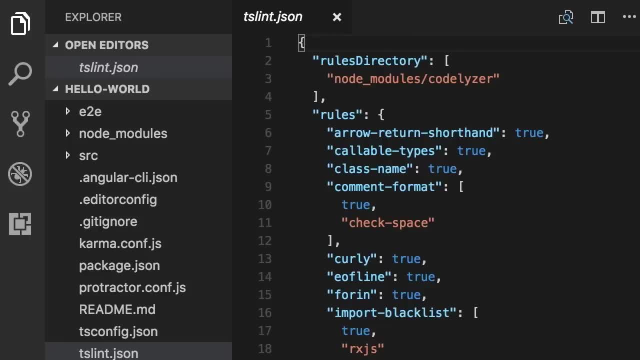 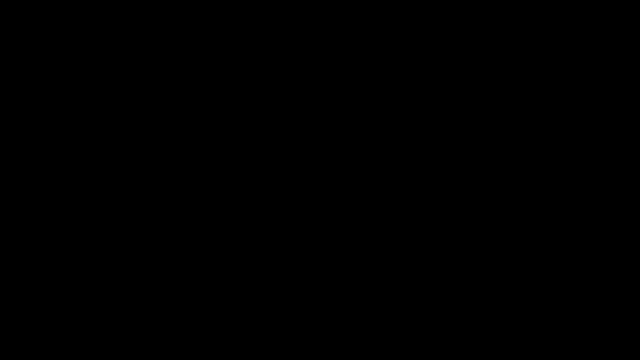 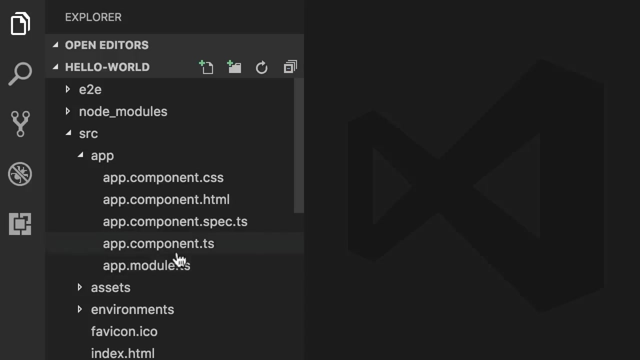 So let's get started. So let's get started. structure of an Angular project. Alright, now let's make a tiny change to this application. So, in the app folder, open up appcomponentts. Now, if you have never worked with TypeScript before, 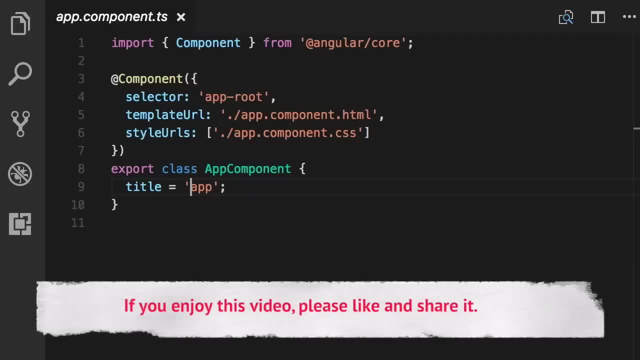 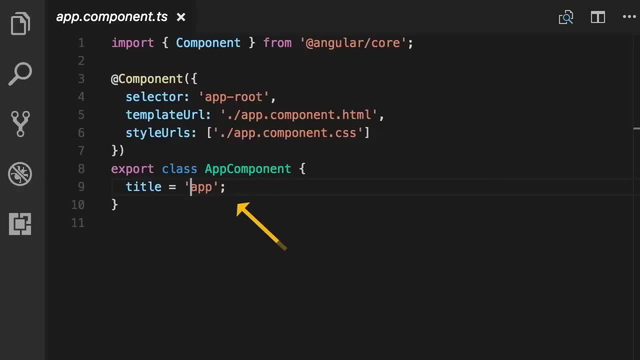 don't worry about this code. as we go through the course, I'm going to break this up for you, so you will know exactly what is happening here. So all I want you to do here is to change this string from app to Angular app. Now save the file. 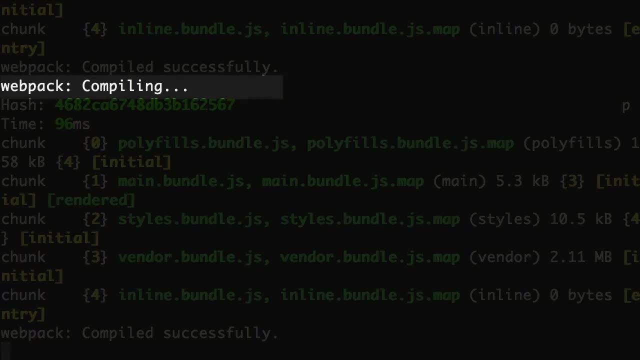 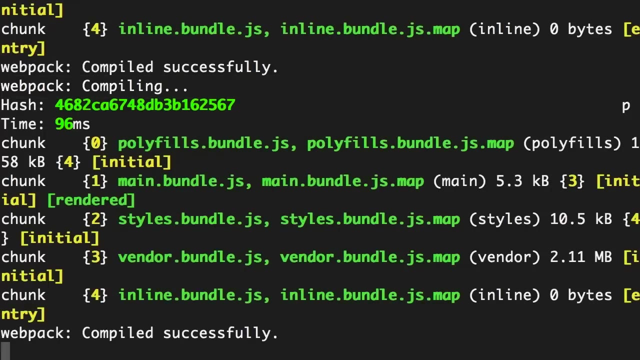 back in the terminal. look at this message: webpack compiling. So Angular CLI uses a tool called webpack, which is a build automation tool. It gets all our scripts and stylesheets, combines them, puts them in a bundle and then minifies that bundle. And this is for optimization. 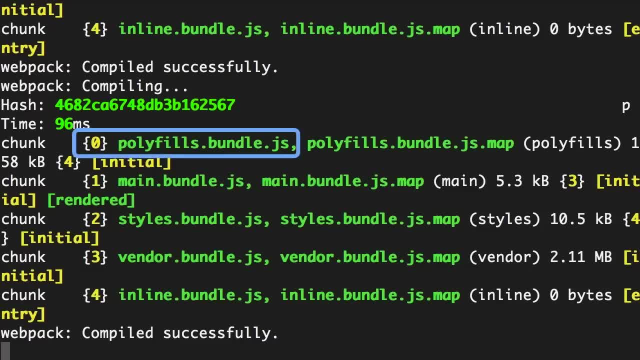 So here you can see, we have a few bundles like polyfills, which includes all the scripts to fill the gap between the version of JavaScript that Angular needs and the version of JavaScript supported by most browsers out there. We have main bundle, which is all the source code of our application. 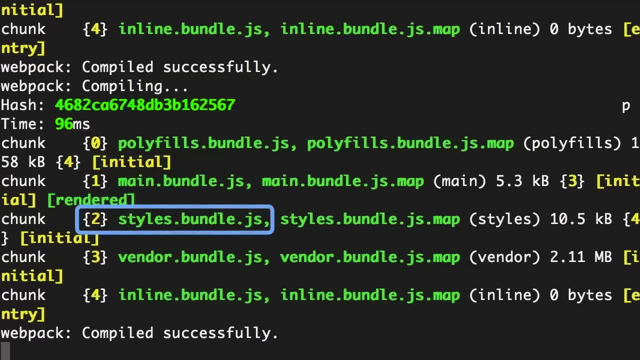 We have styles bundle, which includes all our stylesheets, And note that here stylesheets are actually stored in a JavaScript bundle. You're going to see that in a second. We also have this vendor bundle, which includes all the third party libraries. Now at the. 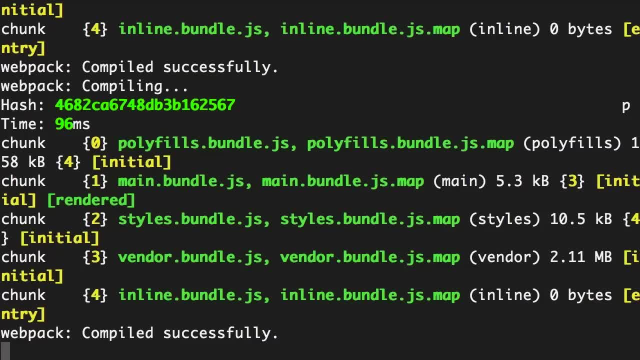 time of recording this video actually Angular. CLI does not allow you to customize the name of these bundles or add additional bundles, But there is a discussion going on on GitHub. Chances are this may change in the future. Now, that aside, what I want you to note here is that whenever you change one of your files, 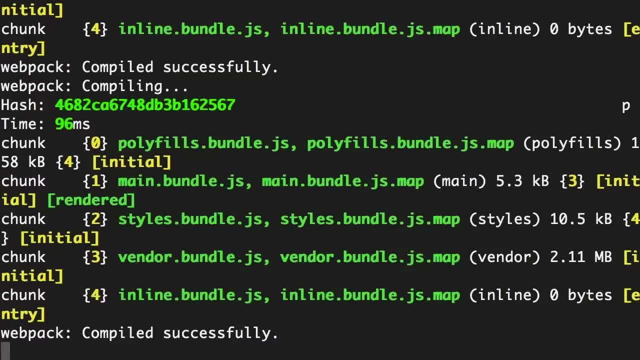 whether that file being a stylesheet, a TypeScript file or an HTML file, webpack automatically recompiles your application and refreshes your bundles. So now, here at the bottom, you can see webpack compiled successfully. Now, if you go back to the browser, 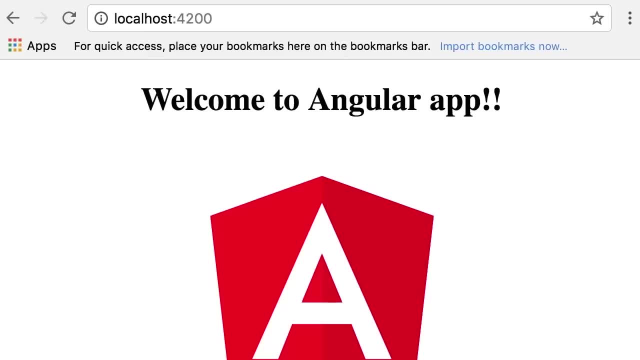 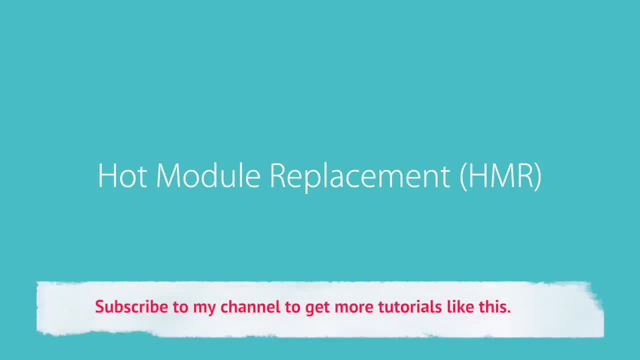 look without me even refreshing this page. now we have the new title: Welcome to Angular app. So this is a feature of webpack, called hot module replacement or hot module reloading. So whenever one of the source files is modified, webpack automatically refreshes your browser. 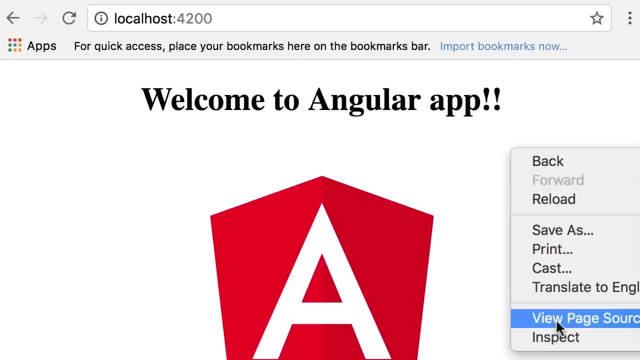 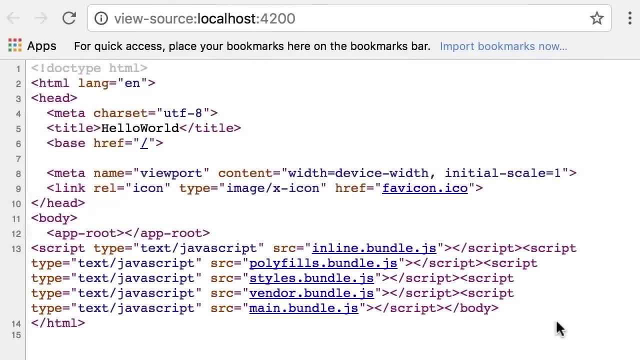 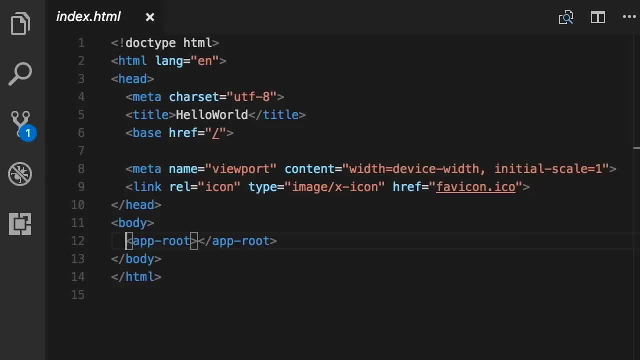 Now let's right click on this page and go to view page source. On the bottom of this page, look at these script tags. So all the bundles that webpack generated. it also injected them into our indexhtml. So just to refresh your memory, here in indexhtml, look, we don't have any. 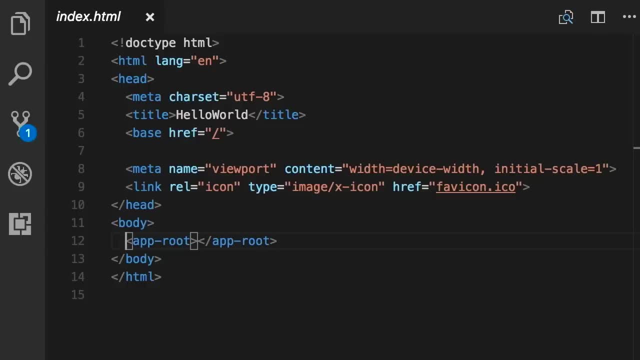 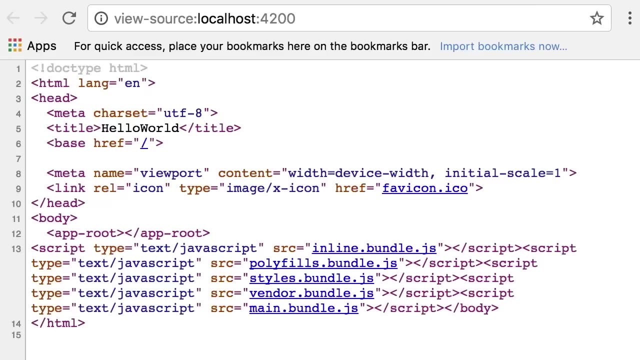 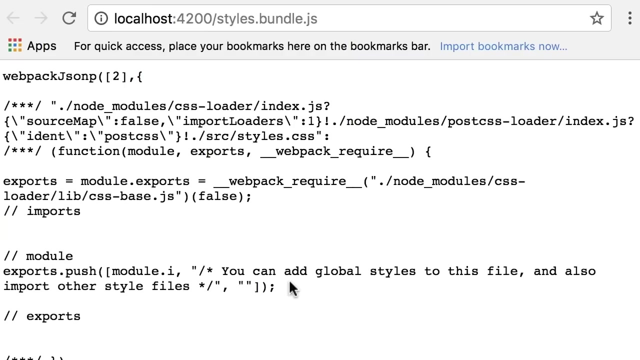 references to your stylesheet or a script file. So this is something that happens at runtime, So webpack automatically injects these scripts into our indexhtml. Now let's take a look at this stylesbundleshtml JS. so basically, what we have here is some JavaScript. 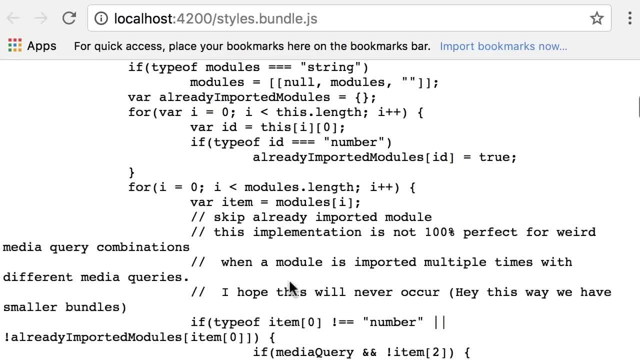 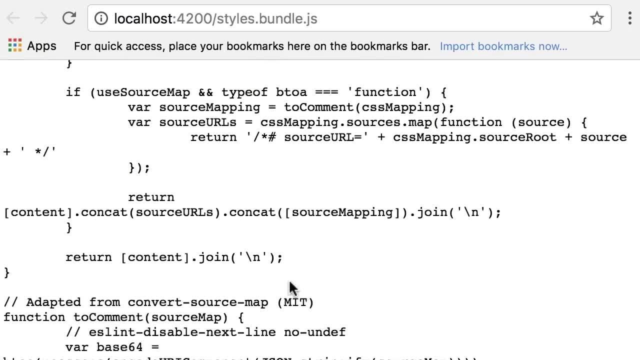 and in the middle of this JavaScript code, you can find the styles used in your application. Now, how this works is a little bit complicated, So don't worry about it for now. What I want you to know is that all your stylesheds are. 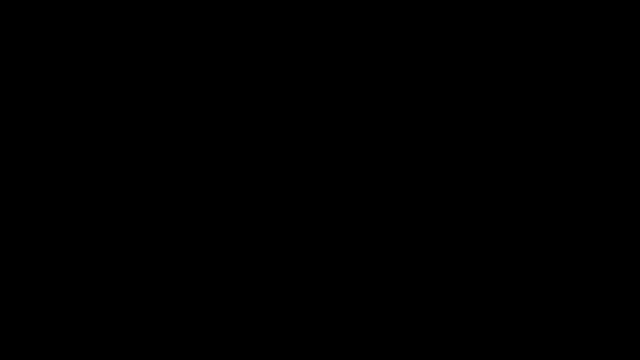 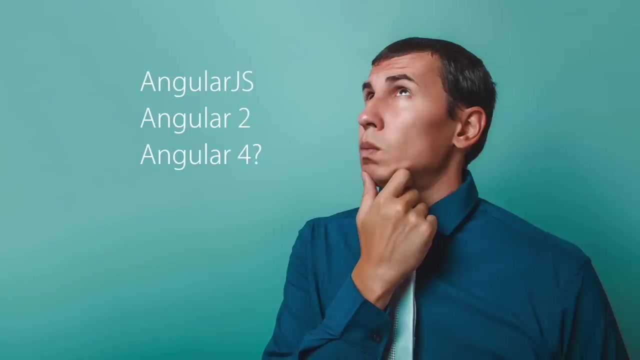 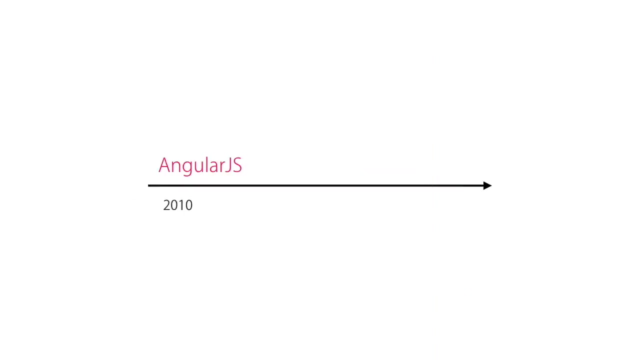 compiled into JavaScript bundle. One question that often comes up is: what's the difference between Angular JS, Angular two and Angular Four, And how did we jump from Angular 2 to Angular 4?? Well, AngularJS was introduced in 2010 as a JavaScript framework. 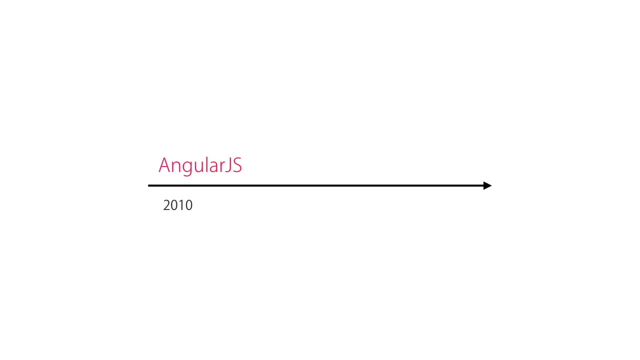 for building client applications. Soon it gained popularity and Angular team started adding new features to the core. But the framework was not designed with the needs of today's applications in mind. Plus, it was overly complex, So Angular team decided to rewrite the original framework using TypeScript and 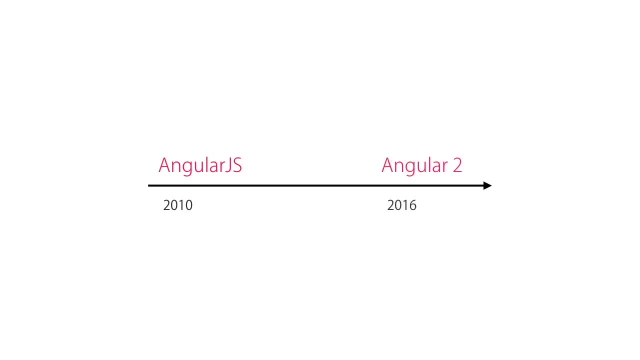 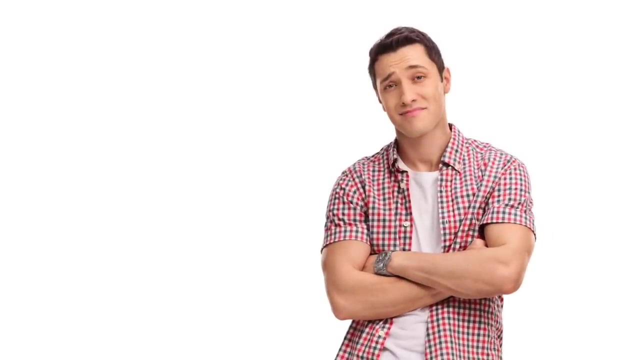 as a result, Angular 2 came out in mid-2016.. This new version is entirely different from Angular 1, to the extent that you can think of it as a completely different framework. Now, this made a lot of developers unhappy, because they had a lot of applications. 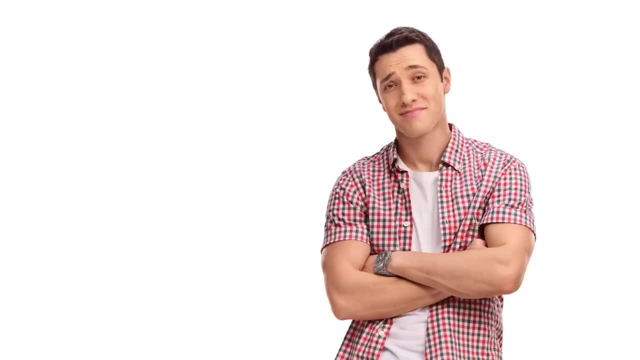 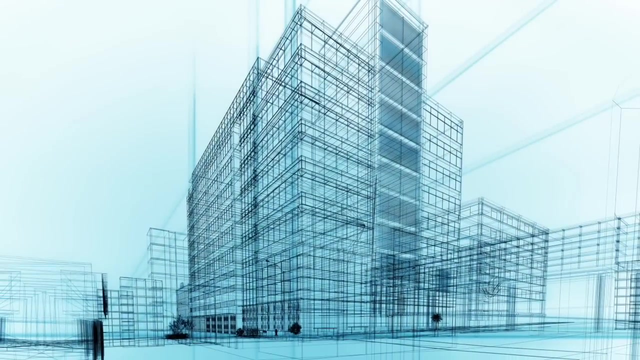 built with Angular 1, with each application over a few thousand lines of code that had to be rewritten. But overall I personally like the direction that the Angular team took and how they rebuilt Angular. This is a much better framework. it's a lot cleaner and it's a lot easier to understand. and to work with. Now, after a few minor upgrades to Angular 2, something strange happened. We were up to Angular 2.3 and then, all of a sudden, Angular 4 came out. So a lot of developers, including myself, wondered what happened to Angular 3.. 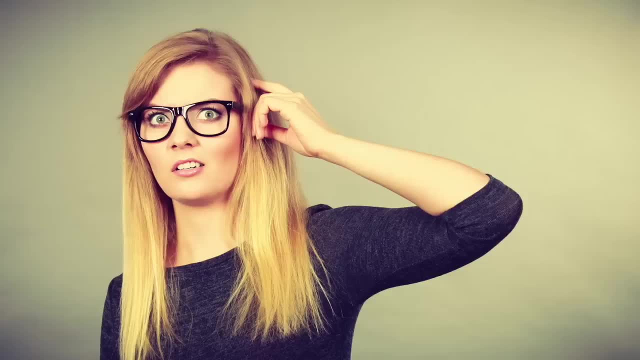 We thought we missed something really big here. but unlike Angular 2, Angular 4 was not a new framework. It worked with a lot of breaking changes. In fact, it wasn't even a major upgrade. So let me explain what happened. 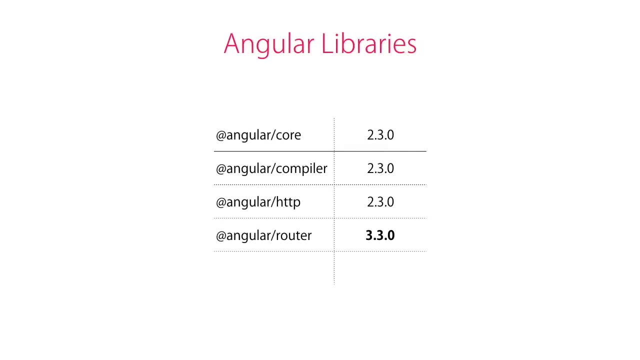 Angular consists of a few different libraries that are distributed as separate node packages via NPM, For example. we have the core library that we use in every application, We have Angular compiler, We have Angular HTTP for calling HTTP services, We have Angular router for adding navigation to applications and a few other libraries. 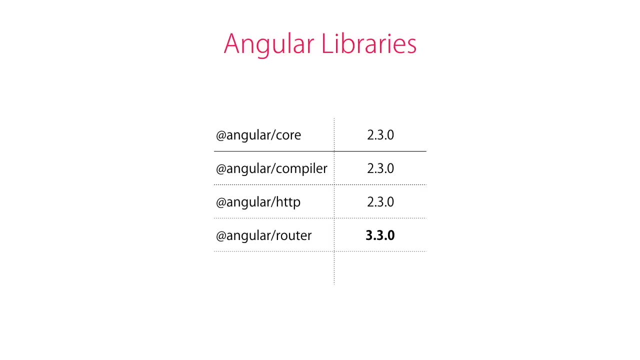 Now all these libraries were versioned the same, except the router library. So in order to align these versions and avoid confusion in the future, Angular team decided to go straight to Angular version 4.. So in a sense, Angular 4 is not a major upgrade to Angular 2, and you can think of it as Angular. 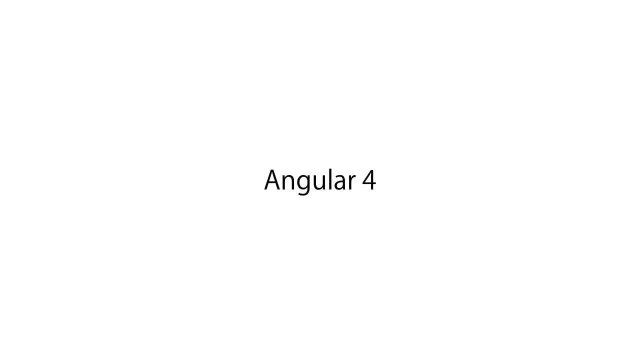 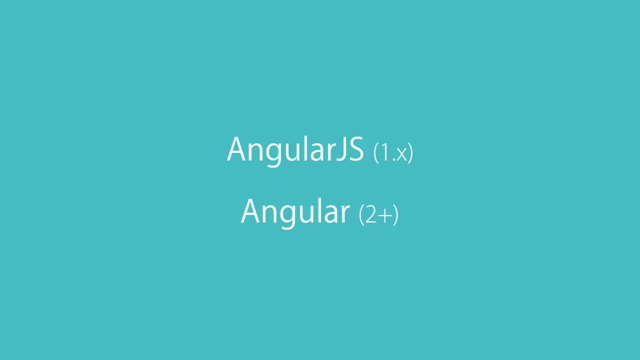 2.4, as simple as that. Now, after all this confusion in the community about Angular versions, the team decided to drop the version suffix And simply call the framework Angular. So now we have two kinds of Angular. We have AngularJS, which is the first generation of Angular written in JavaScript, and it's 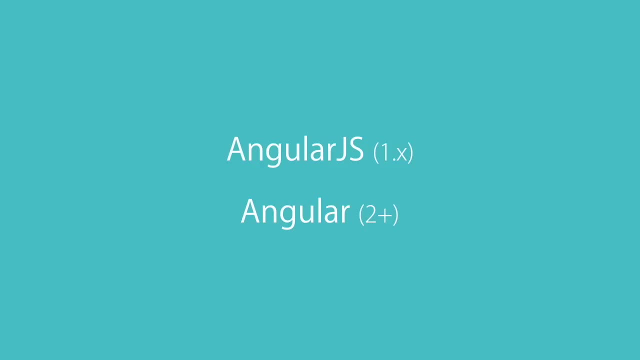 going to die sooner or later, And we also have Angular, which refers to Angular 2 or later. In our discussions, in our articles and whenever we want to talk about Angular 2 or later, we should really use the word Angular like I'm an Angular developer instead of I'm an. 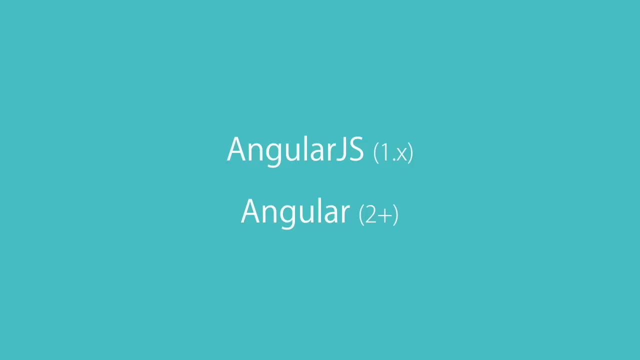 Angular 2 developer Or I'm an Angular 4 developer. See, it's really weird. We should use versions only when we need to talk about a specific release, For example, when we want to upgrade Angular 4 to Angular 5.. 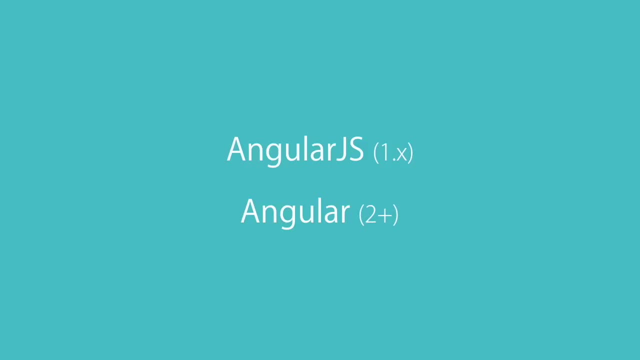 Then everybody knows what is the scope of this upgrade and what are the potential breaking changes that can impact an application. So this is all about Angular version history. All right, now let me quickly give you an overview of how I have structured Angular. 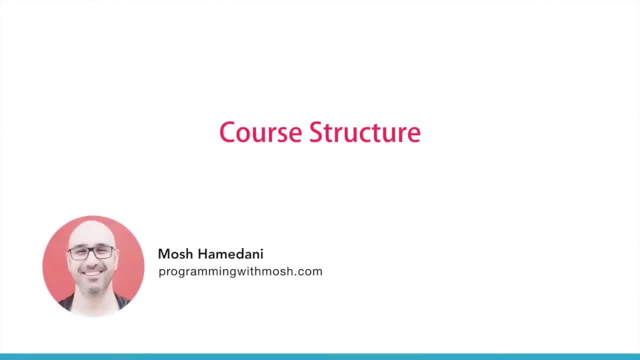 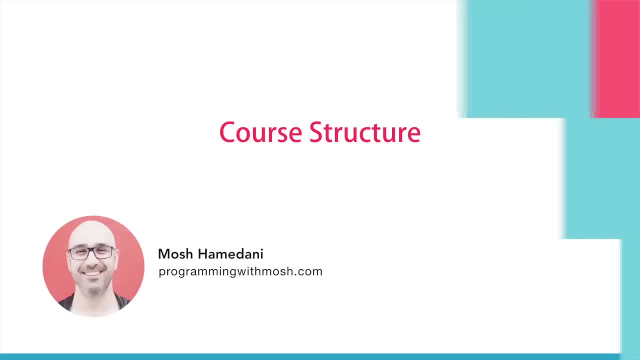 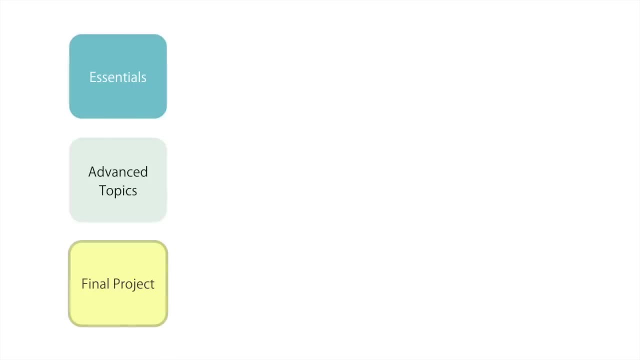 Let me give you an overview of how I have structured Angular And how you can get the most out of it in the shortest possible time. So in this course we have three parts: essentials, advanced topics and the final project. So in this course we have three parts: essentials, advanced topics and the final project. 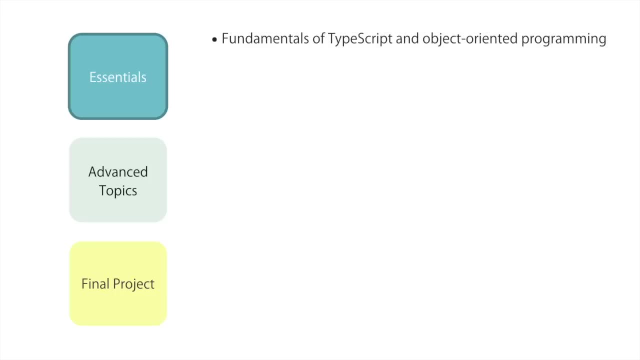 We're going to start the essential part with an introduction to TypeScript and object oriented programming. This will prepare you to build Angular applications. So then we'll look at Angular fundamentals: displaying data and handling events, components, objectives, template-driven forms, reactive forms, consuming HTTP services, routing and. 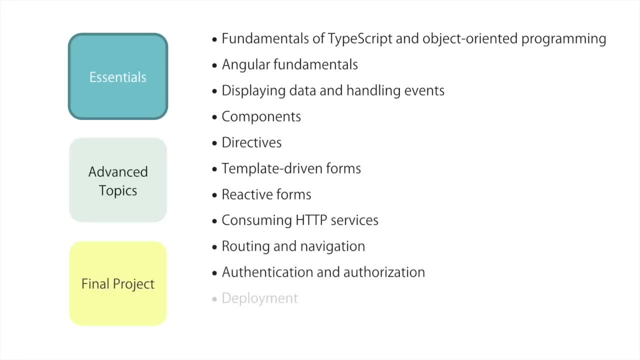 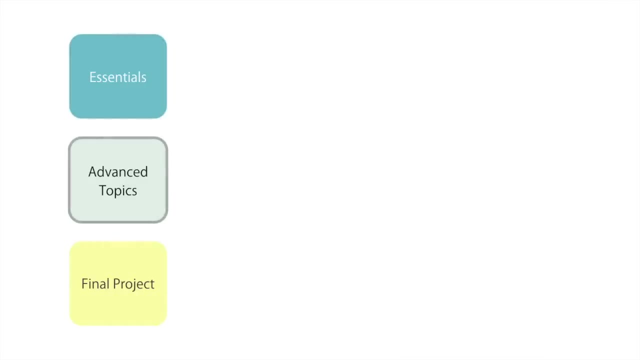 navigation, authentication and authorization, deployment and building real-time applications with Firebase. So these are the essentials that you will use frequently in real-world applications. Then we get into the territory of the advanced topics, And by advanced I don't mean complicated, I mean anything that is beyond the basics. 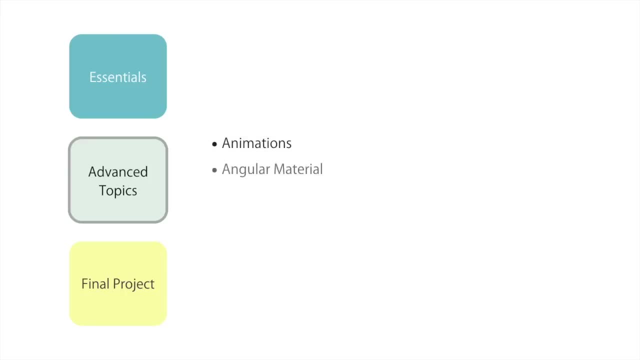 So in this part of the course I will cover animations, Angular material, Redux architecture, unit testing and integration testing, And over the last part we'll build that e-commerce application that I showed you at the beginning of the course. This part also includes a few sections, and in each section we'll build one module of. 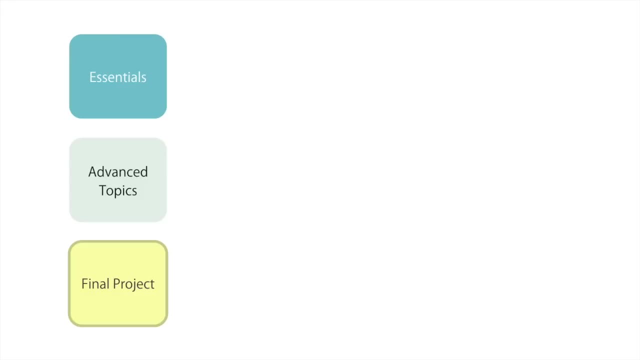 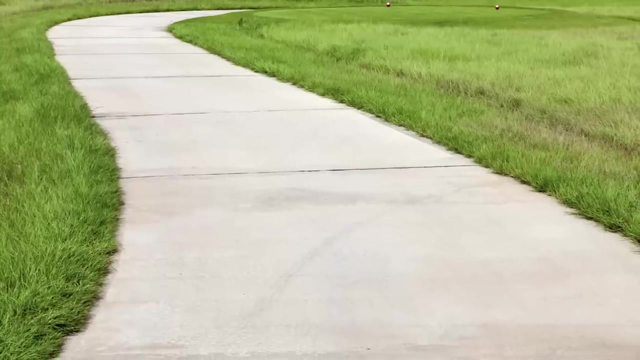 functionality in this application. So here we have sections like product management, shopping cart checkout and so on. Now I understand that you might be busy and not have enough time to watch the entire course, and that's perfectly fine, So I'm going to give you a shortcut, a shortcut that allows you to get the most out of the 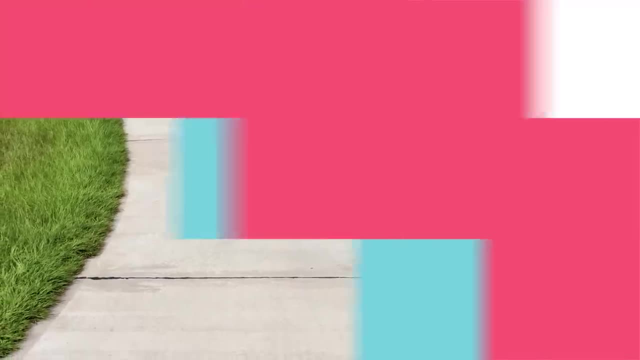 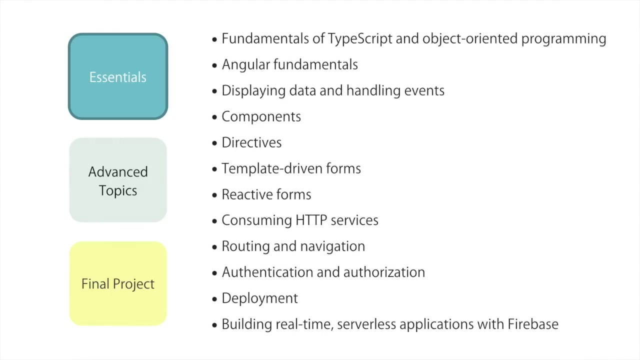 course within the shortest possible time. Start with the essentials. Watch all these sections in sequence, But feel free to skip the section called reactive forms, because we're not going to use the materials in this section In our final project. Also, you can skip consuming HTTP services, as well as authentication and authorization. 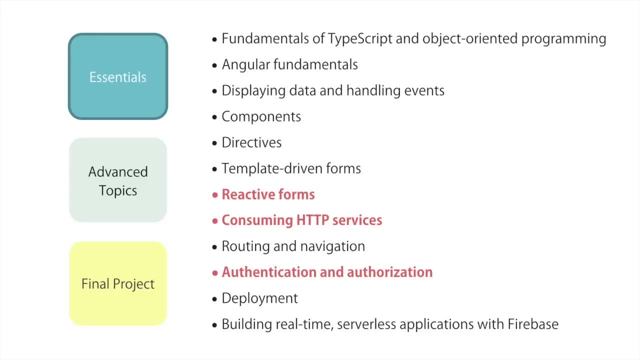 You need to watch these sections if you want to build a backend for your application using frameworks such as ASPNET, Express, Django and so on. But this e-commerce application we'll build in this course doesn't have a custom built backend. We use Firebase as the backend. 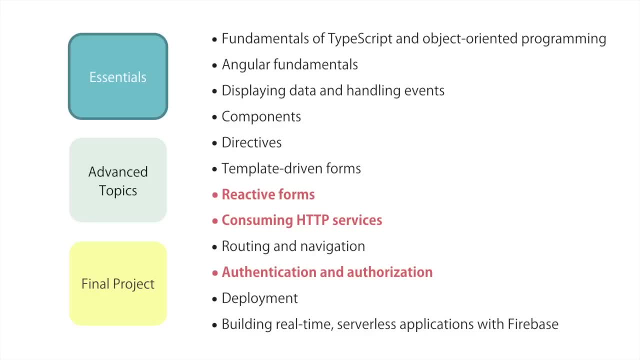 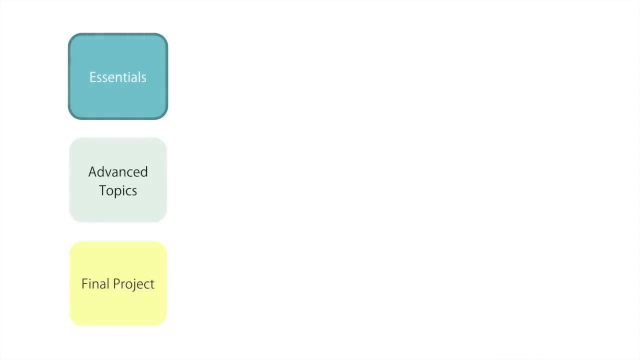 So things are a little bit different here. If this sounds confusing to you, Don't worry, I will clarify it in the section about Firebase. So here's my suggestion to you: Watch these sections in the essential parts in sequence and then move to the final project. 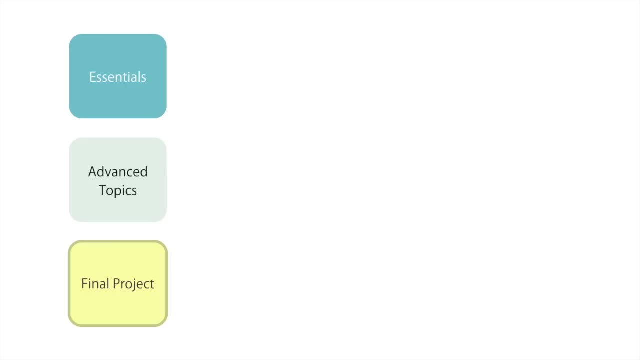 part. I want you to build this application, because that's where you will see all these moving parts coming together. Plus, those sections include tons and tons of tips and techniques that I've shared with you, And these are the things I have learned over the past 17 years of working in the industry. 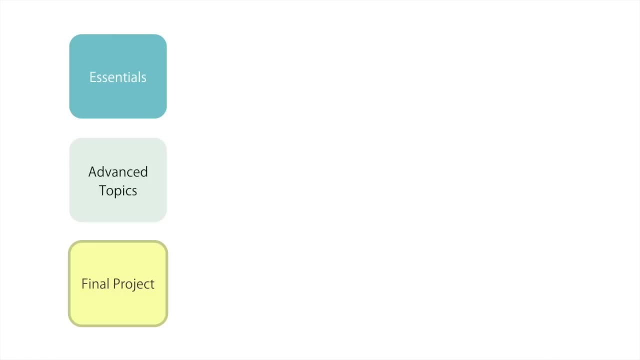 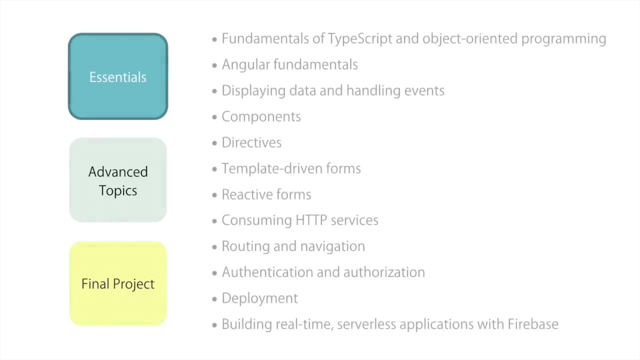 As a professional software developer. they really change your thinking about programming and software engineering. I worked really hard for these sections and I want you to watch them Once you finish the project. then you will have a good understanding of the big picture. Then you can come back and learn about the other sections in the course in isolation. 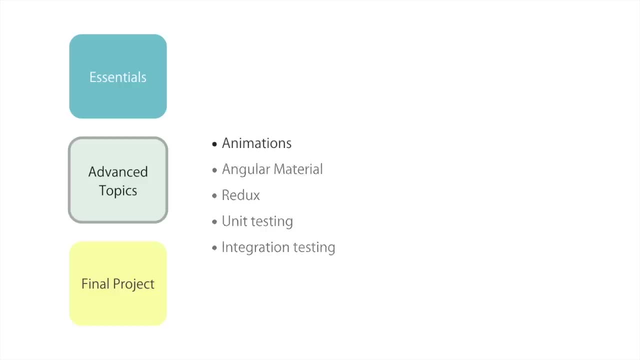 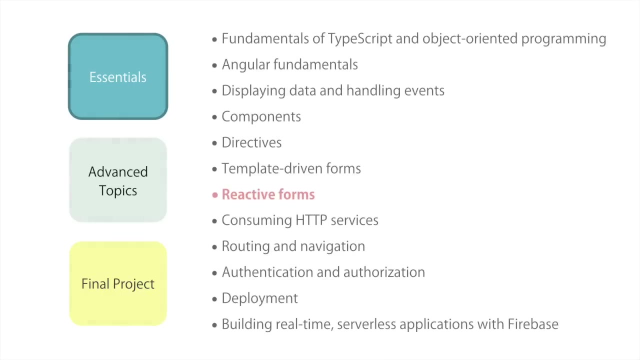 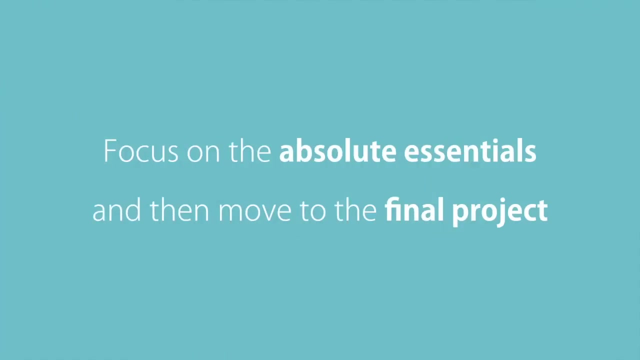 depending on your needs. For example, if you want to learn how to add animations to your applications, you can simply go watch the animation section. Or if you want to learn about reactive forms, you can just go back to that section. So focus on the absolute essentials and then move to the final project. 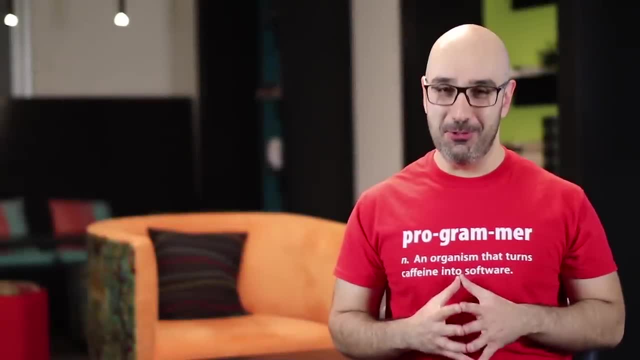 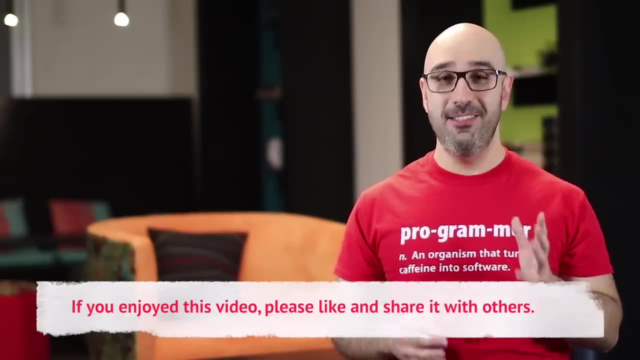 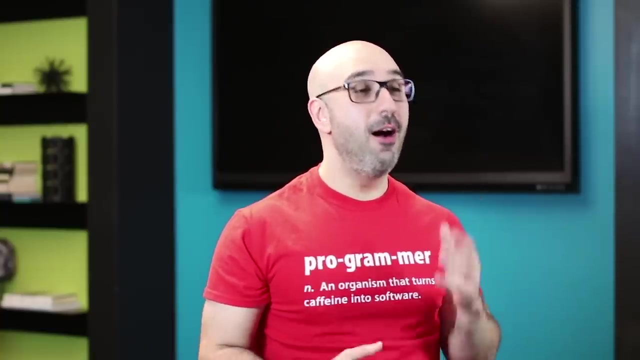 Hi, thank you for watching my Angular tutorial. If you enjoyed this video, please like it and share it with others. Also, you can subscribe to my channel for free new videos every week. This video is part of my complete Angular course, with almost 30 hours of high quality. 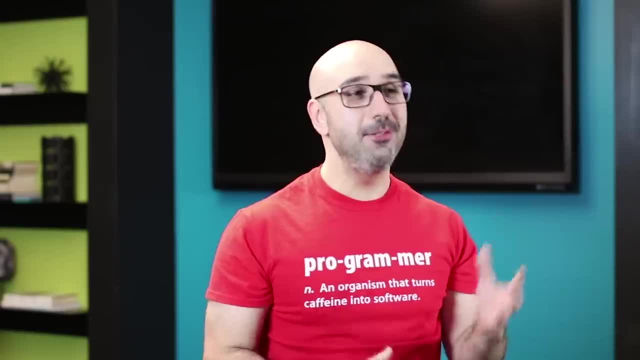 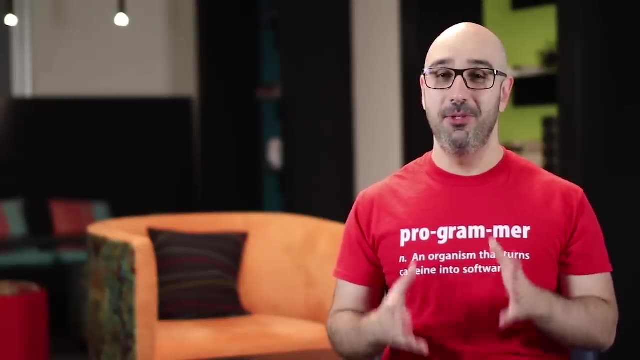 content Where you will learn everything about Angular, from the basic to the advanced topics, all in one course, So you don't have to jump from one tutorial to another. In case you're interested, you can get this course with a big discount using the link. 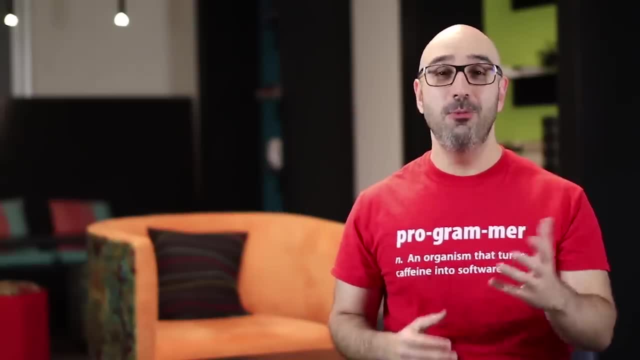 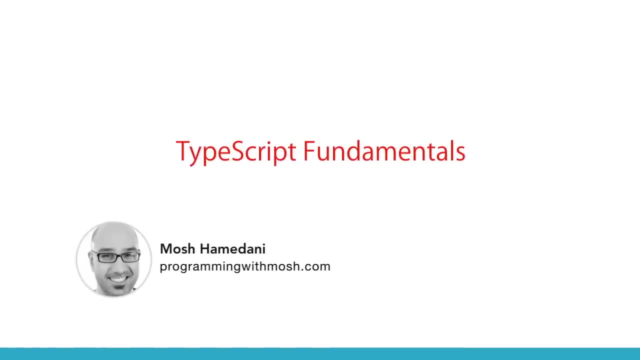 in the video description, And if not, that's perfectly fine. Continue watching as the next section is coming up. In order to build applications with Angular, you need to be comfortable with TypeScript. So in this section I'm going to introduce you to the fun part. 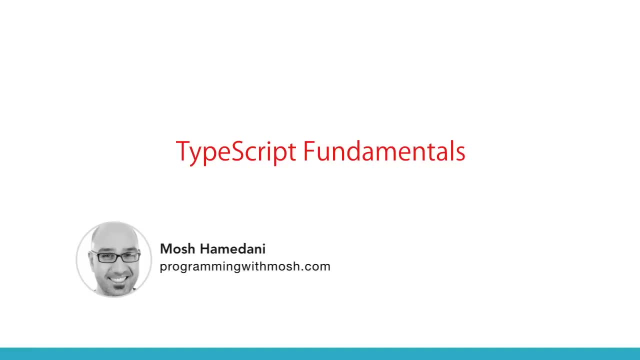 In this section. I'm going to introduce you to the fun part In this section. I'm going to introduce you to the fun part In this section. I'm going to introduce you to the fundamentals of TypeScript and object-oriented programming principles. 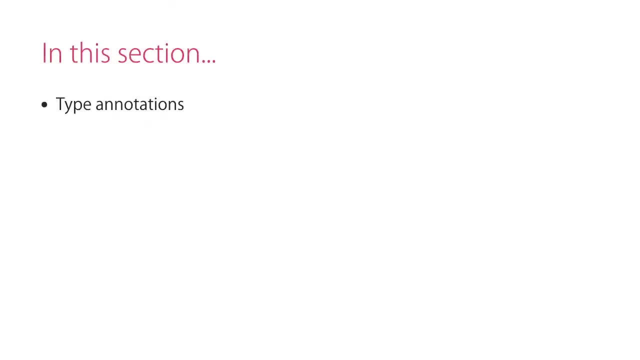 So by the end of this section you will have a good understanding of type anotations, arrow functions, interfaces, classes, constructors, access, modifiers, properties and modules, If you're familiar with this concepts and know how to implement them in TypeScript. 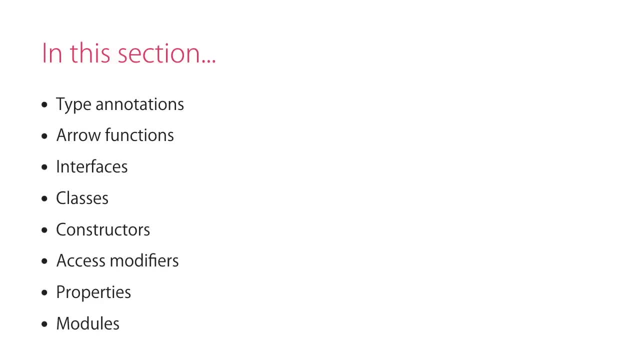 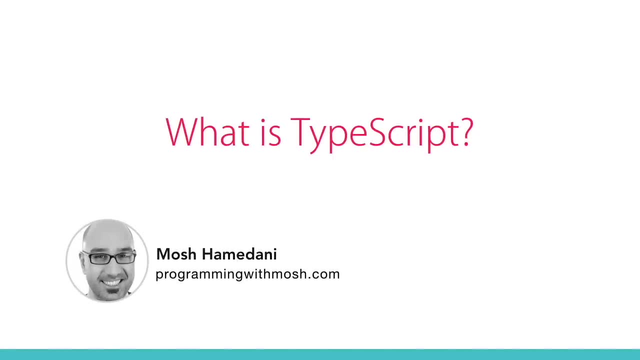 feel free to skip the section and move on to Angular. Otherwise, you really need to watch every lecture in this section. Otherwise, you really need to watch every lecture in this section. let's get started. So what is TypeScript? TypeScript is not an entirely new language. 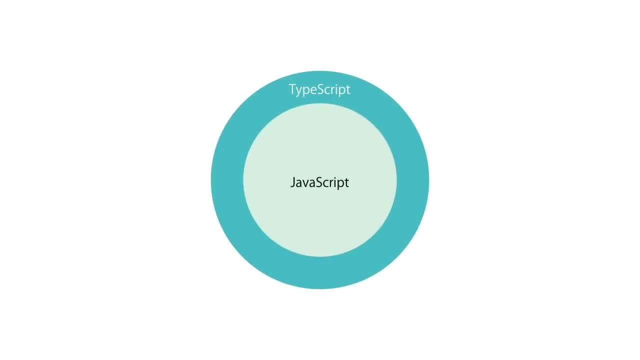 It's a superset of JavaScript, So that means any valid JavaScript code is also valid TypeScript code, But TypeScript has additional features that do not exist in the current version of JavaScript supported by most browsers out there. For example, in TypeScript we have this concept of strong or 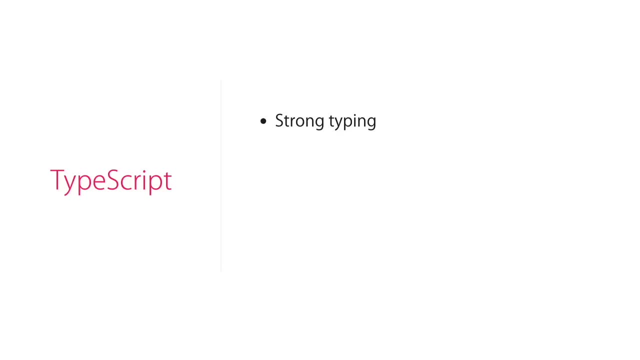 static typing. If you have worked with languages like C, sharp and Java, you know that in these languages, when we define a variable, we need to specify the type of that variable. Now in TypeScript, typing is optional, so we don't have to use this feature. But using this feature makes 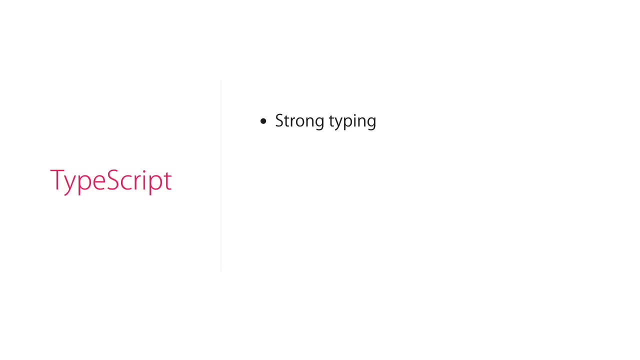 our applications more predictable, And it also makes it easier to debug them when something goes wrong. TypeScript also brings quite a few object oriented features that we have missed in JavaScript for a long time. We have the concept of class, we have the concept of type and we have the concept. 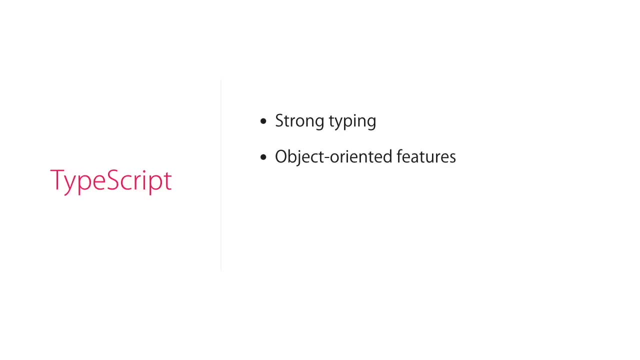 of classes, interfaces, constructors, access modifiers like public and private fields, properties, generics and so on. You're going to learn about this in this section Now. another benefit of using TypeScript is that with TypeScript, we can catch errors at compile. 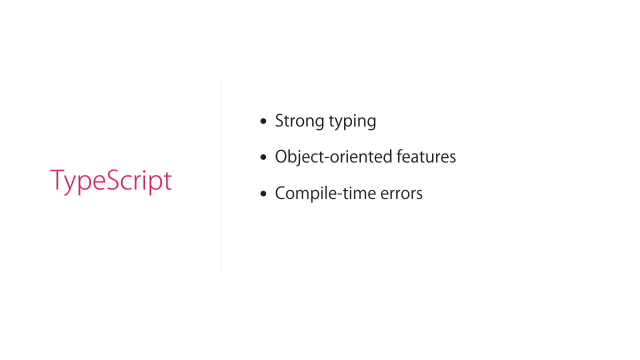 time instead of at runtime. Well, of course, not all kinds of errors, but a lot of errors. So there is a compilation step involved And when we compile our TypeScript code, we can catch these errors and fix them before deploying our application. 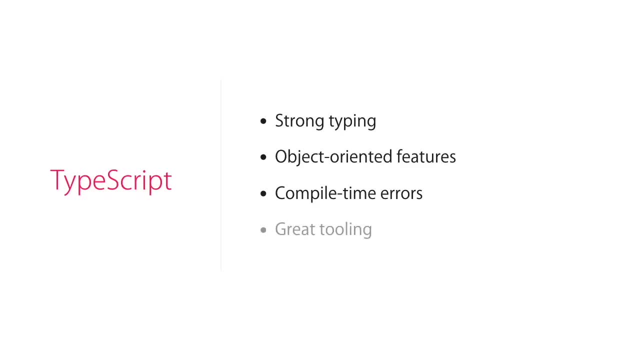 And finally, another benefit of using TypeScript is that we get access to some great tools out there. One thing that I personally love about TypeScript is the intelligence that we get in our code editors. Again, you're going to see that in this section. So TypeScript is a beautiful. 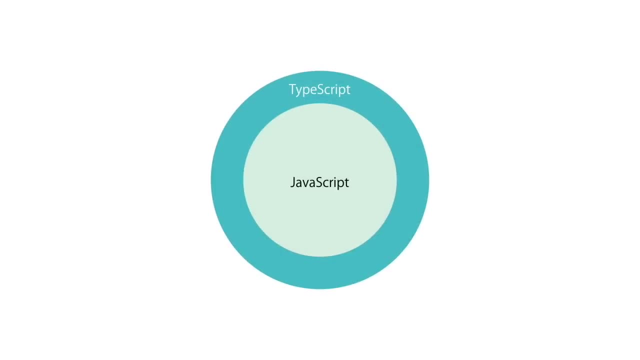 language and it's basically a superset of JavaScript. So any valid JavaScript code is also valid TypeScript code. Now the browsers out there, they don't understand TypeScript And it's very unlikely that they're going to support it in the future. 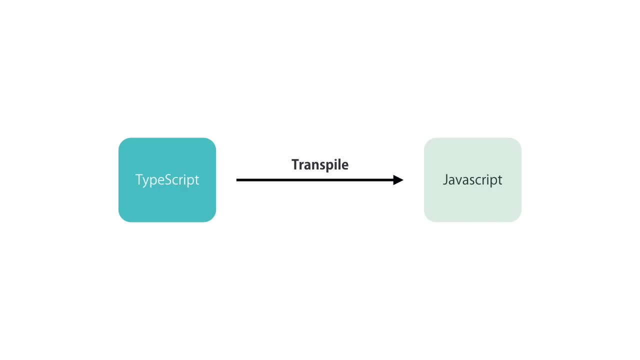 So we need to compile, or, more accurately, transpile our TypeScript code into JavaScript. So this is part of building our application. Whenever we build our application, TypeScript compiler kicks in and it transpiles our TypeScript code into JavaScript code that browsers can understand. Now, that's enough introduction. Next I'm going to show you. 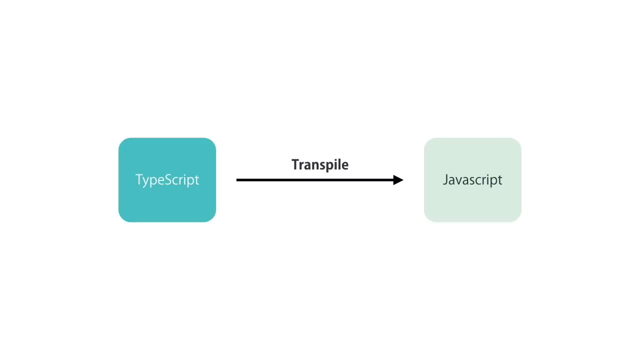 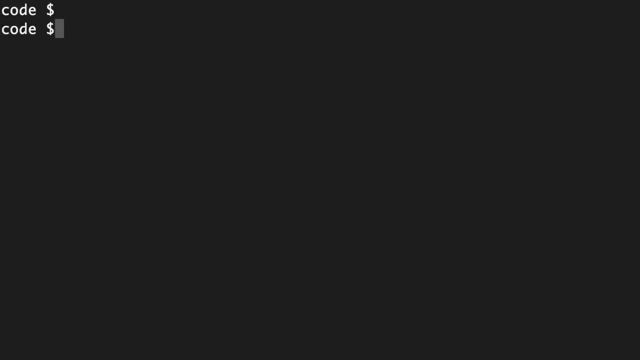 how to install TypeScript and write your first TypeScript program. In this lecture, I'm going to show you how to install TypeScript and write your first TypeScript program. In this lecture, I'm going to show you how to install TypeScript and write your first TypeScript program. So here we're in the terminal. we're not going to work with Angular in this. 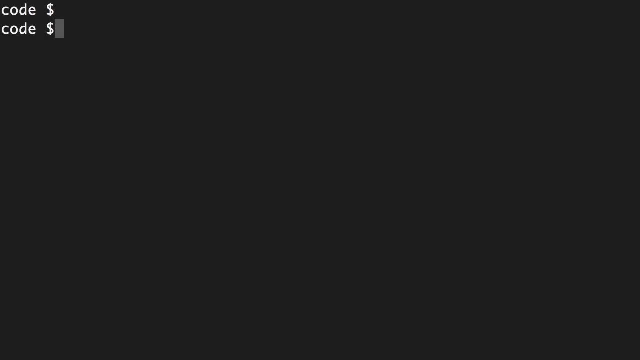 section we're going to purely focus on TypeScript. So first we need to install TypeScript globally on type script. So first we need to install TypeScript globally on our machine. So npm, install dash g, which stands for Global type script, And of course, if you're on mag you need to put 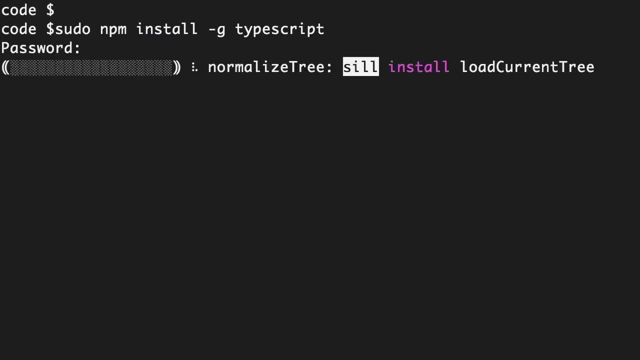 sudo at the front. All right, Beautiful, So I've got global. All right, Beautiful, So I've got global. installed, the latest version of typescript, which is currently version 2.3.4. now we can type tsc, which stands for typescript compiler. dash, dash version. again, you can see that i'm running. 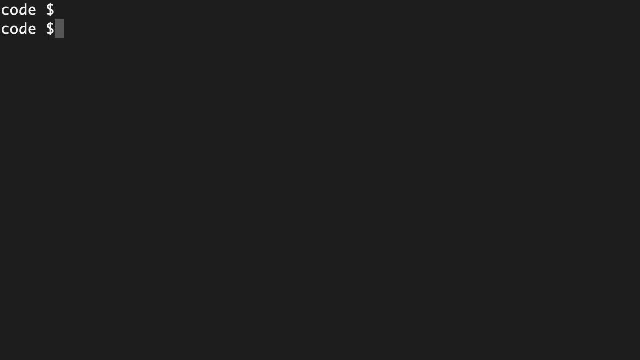 typescript 2.3.4. all right, now i'm going to create a new folder for this section, so let's call this ts: hello, let's go to this folder now. here i'm going to create a new file and open it with vs code, so code maints. so now i'm going to write some plain javascript code and i want to show you. 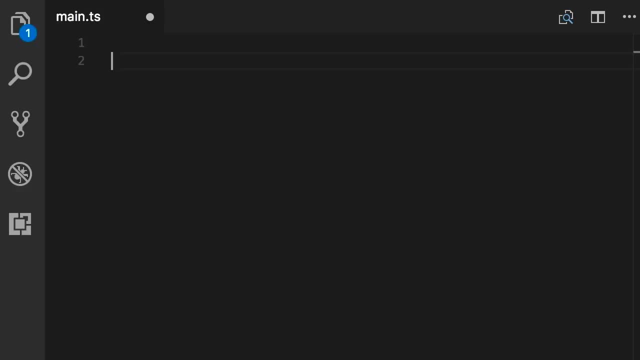 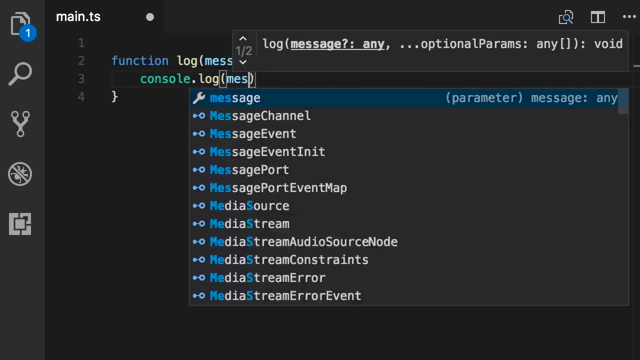 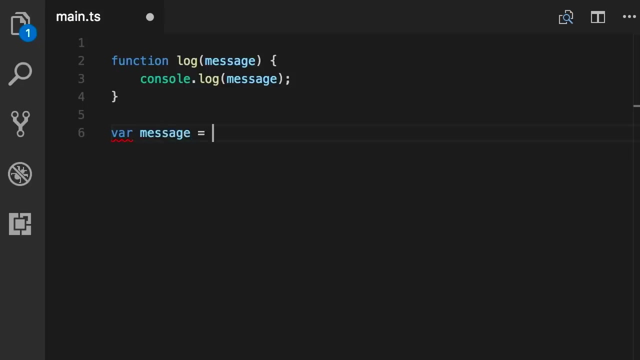 that all this javascript code is also valid typescript code. so first i'm going to define a function- let's call this log- that takes a message, and here we simply log that message on the console like this. then i'm going to declare a global variable- let's call this message: 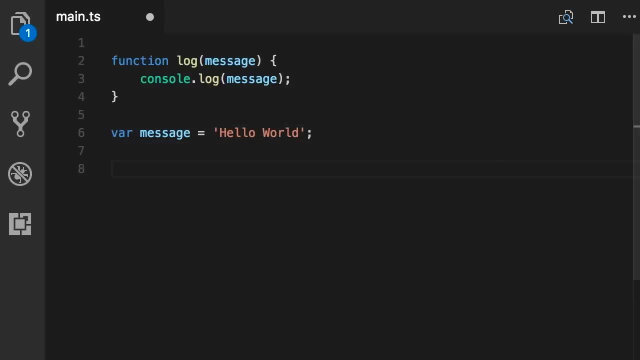 and set it to this string hello world and finally call our log function message. so this is just plain javascript code. right now save back in the terminal. we need to transpile this typescript file into javascript. so tsc or typescript compiler, maints now. if you look at: 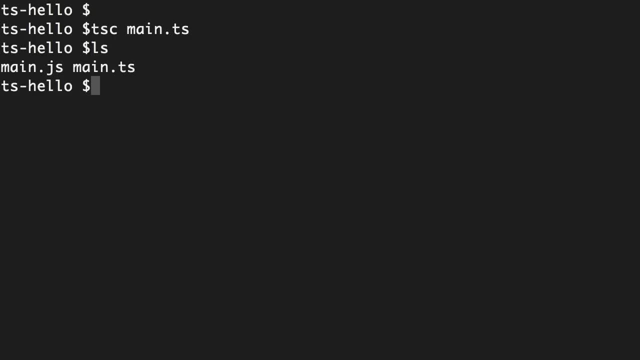 this folder. look, we have mainjs and maints. now this transpilation or compilation step, when you are building an angular app, happens under the hood, so you don't have to manually call the typescript compiler. in fact, when you run your application using ng serve angular, cli calls typescript. 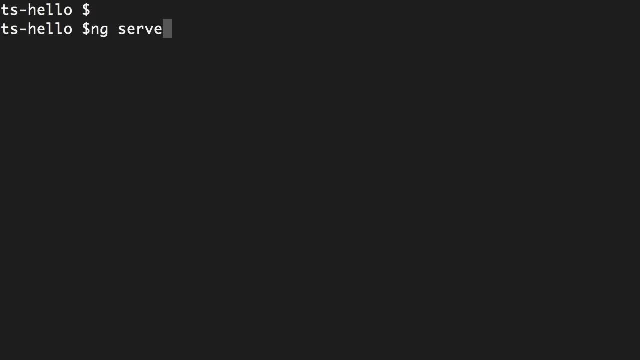 compiler under the hood to transpile all our typescript code. all right, now let's open our mainjs file. so code js. So it's exactly the same code that we wrote, but now it's in a javascript file. So all javascript code is also valid typescript code. Now back in the terminal. 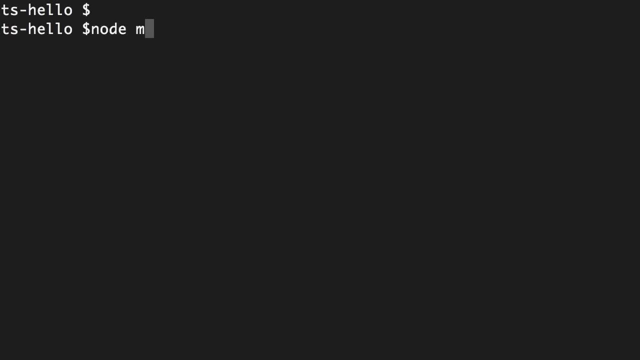 I can execute this code using node. So node main js, And we got the hello world message on the console. So from the next lecture we're going to look at specific features of typescript that we don't currently have in javascript. Alright, let's explore typescript. 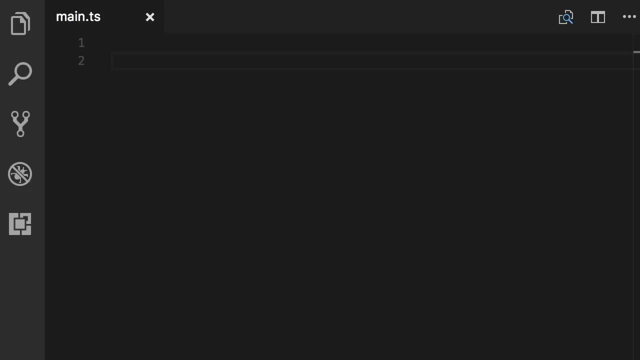 by looking at variable declarations. So in typescript there are two ways to declare a variable. We can use the var keyword which you have seen in javascript. like var number, we set it to 1.. Or we can use the let keyword, So let. 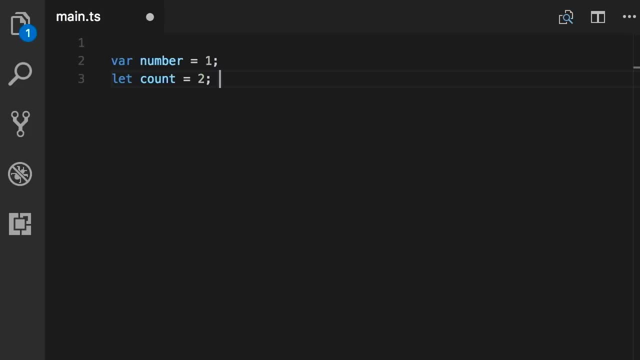 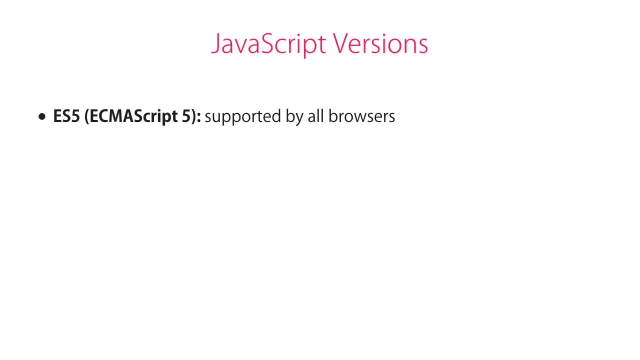 count to be 2.. Now, before I explain the difference, I need to clarify that the let keyword is also being added to the javascript. So javascript has a few different versions. We have ES5 or ECMAScript 5, which is the version of javascript supported by pretty much. 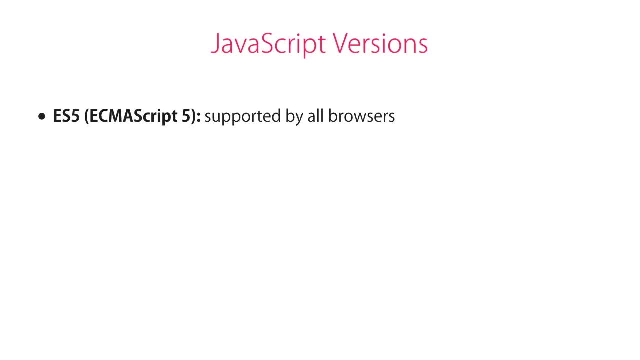 all browsers out there. It's been around for a long time. Now we have ES6,, which is a newer version, and it was introduced in year 2015.. And from that point, the ECMAScript team, which is the team extending javascript, decided to use: 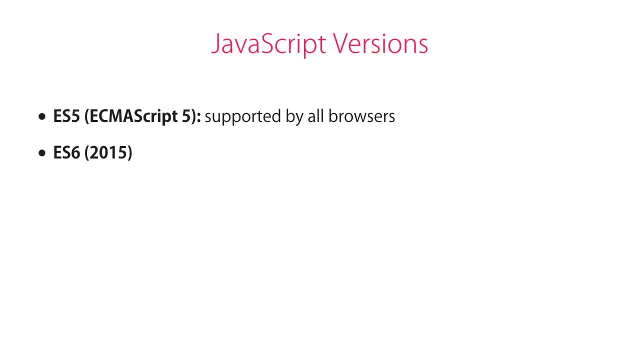 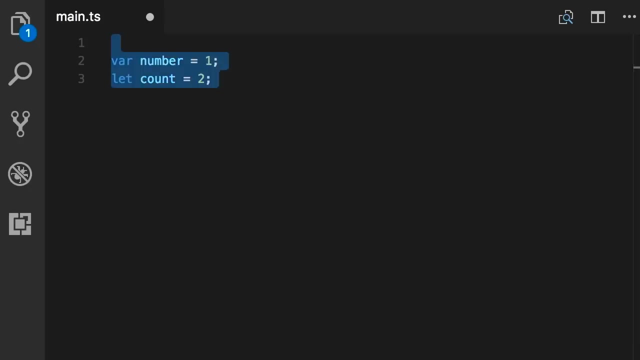 the year number instead of the version number. So we have ECMAScript 2015,, 2016, and 2017.. Now in ECMAScript 2015,- which is basically ES6, we also have this let keyword, But in case you are not familiar with it, let me explain how it works. 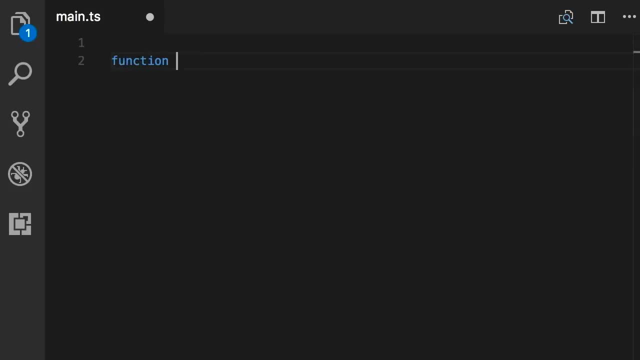 So I'm going to define a function. Let's call it: do something, It doesn't really matter. Now here I'm going to define a for block. So var, we set i to 0.. And as long as i is less than 5,. 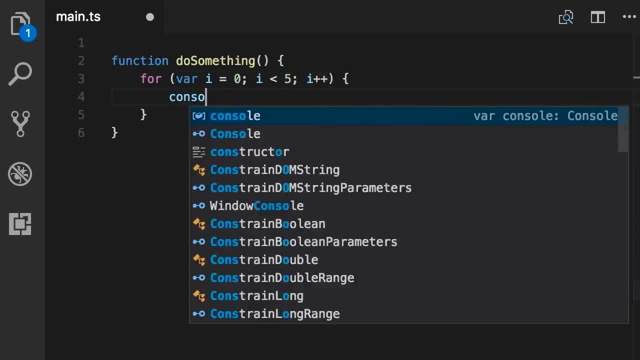 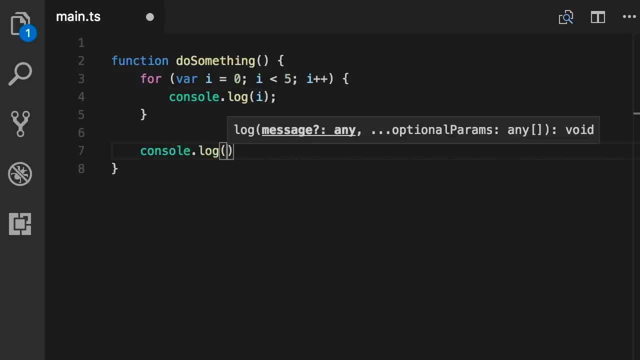 let's increment it. Here we have a block and then log it on the console. Now, finally, at the end of this function, I'm going to log this i one more time, But with the label finally, And then I'm going to call this function. 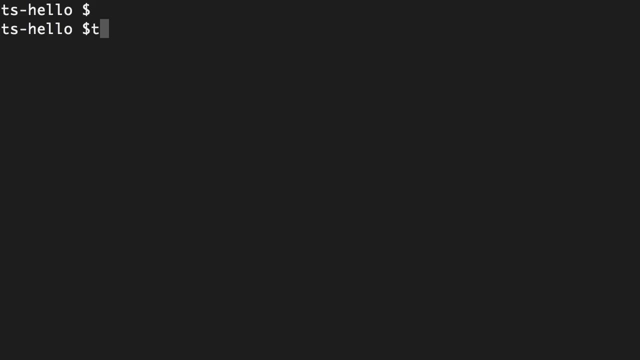 here. So in the terminal I'm going to compile this file maints and also at the same time run it with node mainjs. Note that the value of i at the end of this function is 0. And at the end is 5.. So this is the issue we have. 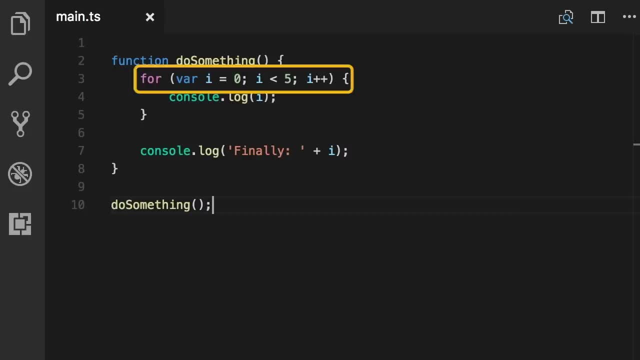 when declaring a variable using the var keyword. So we have declared i here inside this for block, but it's also meaningful and available outside the for block. Now, if you have worked with languages like C, sharp or Java, you know that we don't have this concept. 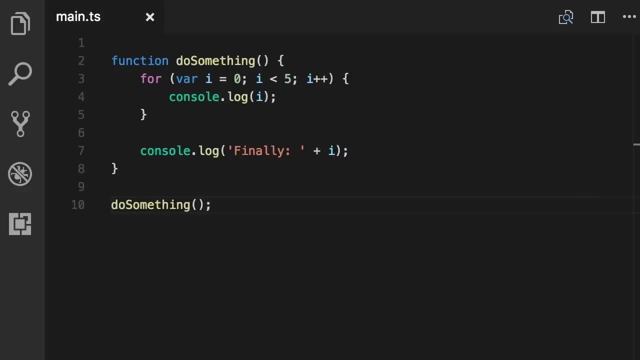 in those languages. In JavaScript, a variable declared with a var keyword is scoped to the nearest function. So in this case, the nearest function is do something. So once we declare i inside this for block, it's available anywhere in this function. Now let's. 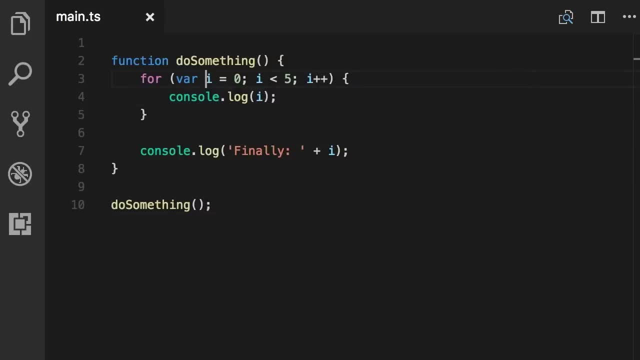 see what happens when we declare this variable using the let keyword. So let Now look. we immediately got a red underline here which indicates a compilation error, And this is one of the beauties of TypeScript, When you're writing TypeScript code. 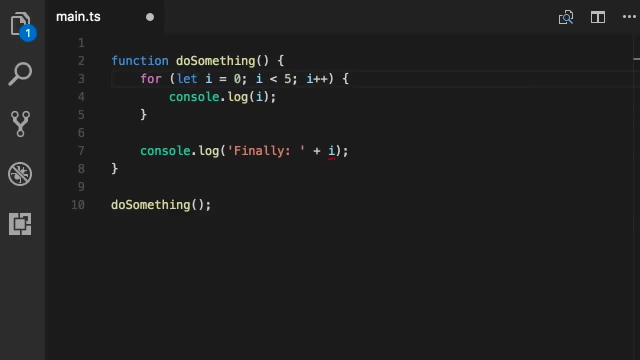 you can catch these errors at compile time, before you run your application, before you deploy it. Let's hover our mouse here. So this is the error: Cannot find name i. So now i is scoped to the nearest block instead of nearest function, And this is the proper way. 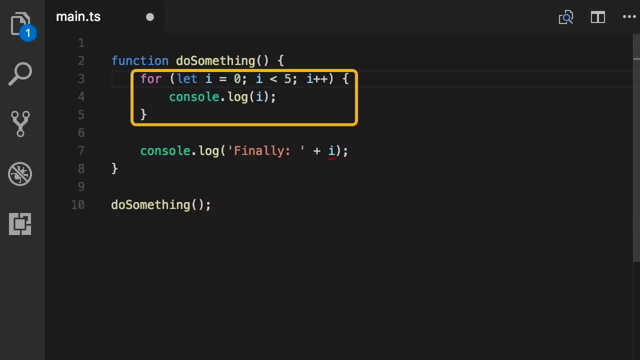 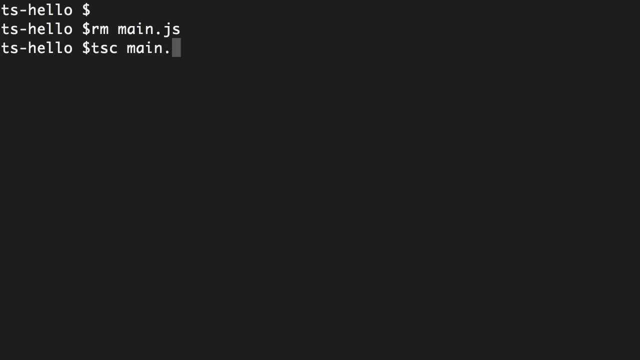 to declare variables, which prevents a lot of issues later down the road. Now I want to clarify something. Let me save this file Back in the terminal. first I'm going to remove mainjs. Now I'm going to recompile our mainjs. 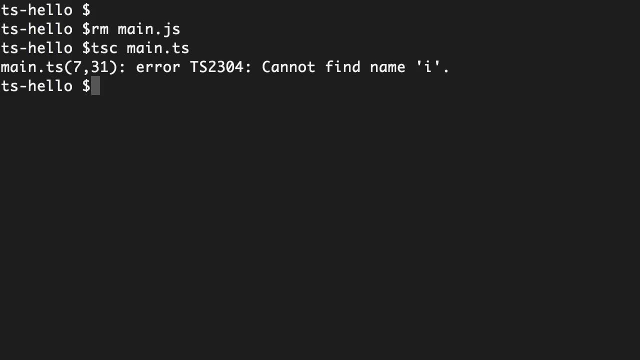 Okay, we got our error here. cannot find name i. However, if you look at the files in this folder, we do have mainjs. So even though we have a compilation error, the TypeScript compiler still generated mainjs. Let's have a look. 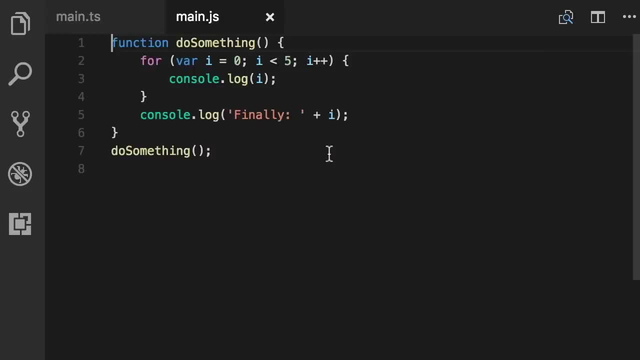 at the content of this file. So this is the code that is generated. So, by default, TypeScript compiler compiles our TypeScript code to ES5 or ECMAScript 5, which is the older version of JS. So this is the code that is generated. 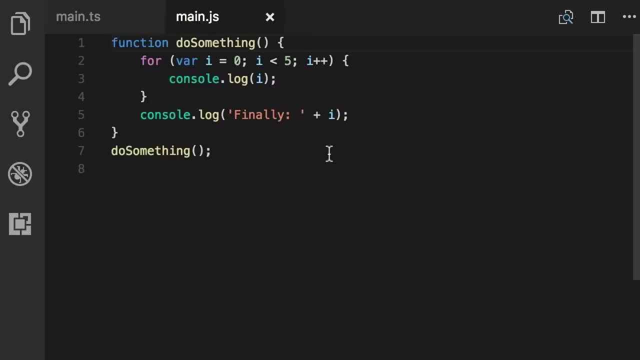 JavaScript that is supported by all browsers out there. Now, there, we don't have the let keyword, So that's why our compiled code now uses the var keyword, And this is perfectly valid JavaScript code. So I can go in the terminal and simply run this code and get the same output. 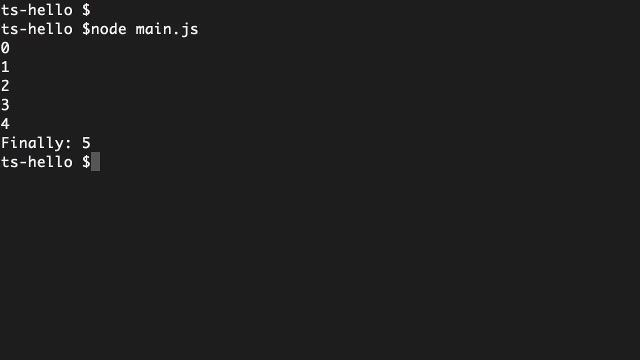 as before. So what I want to clarify here is that TypeScript compiler reports these errors, but still generates valid JavaScript code. So here's the takeaway for this lecture. From now on, anywhere we want to declare a variable, we use the let keyword Once again. 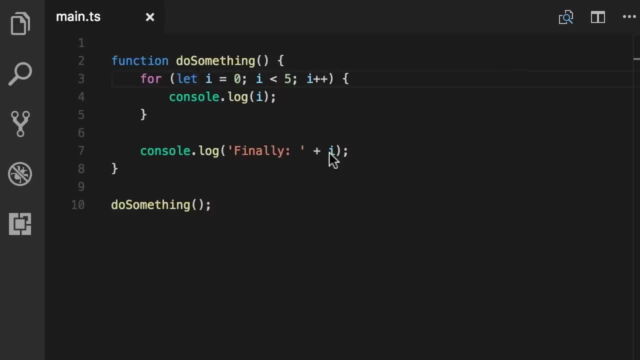 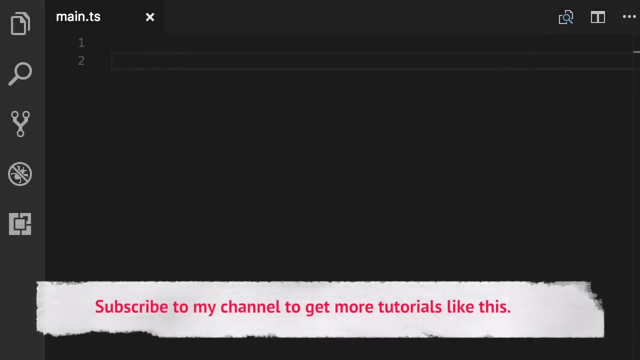 this does not stop the compilation step, but at least we can catch the issues earlier during the compile time. Next, we're going to look at different types we have in TypeScript. In this lecture I'm going to show you different types we have in TypeScript. So let me start by declaring a. 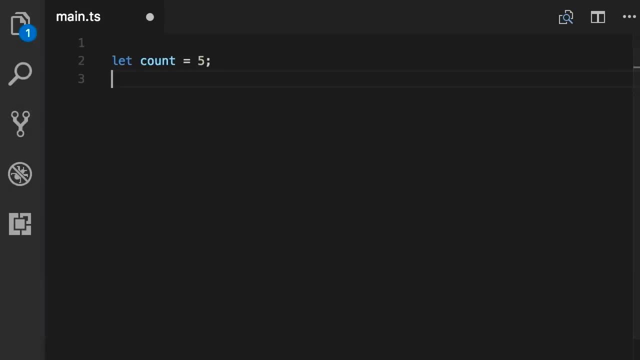 variable called code. Let's say that I'm going to set the variable to code. So let's say I'm going to set the variable to code and I'm going to set it to 5.. Now if I set this to, let's say, a character or a string like a: 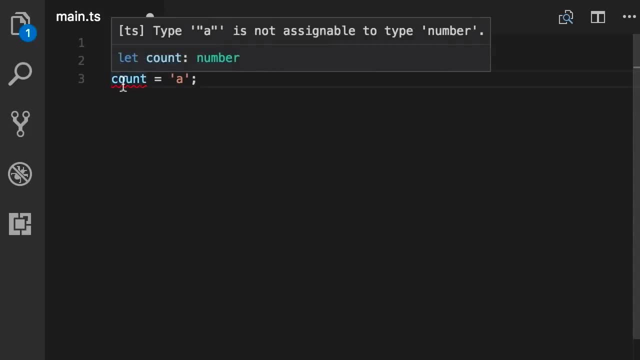 know that I immediately get a compilation error here telling me that this, a string or a character, is not assignable to type number. Now, we can perfectly do this in JavaScript, because in JavaScript we can change the type of variables on the fly, But in TypeScript we get a compilation error. Now, once again, I want to clarify. 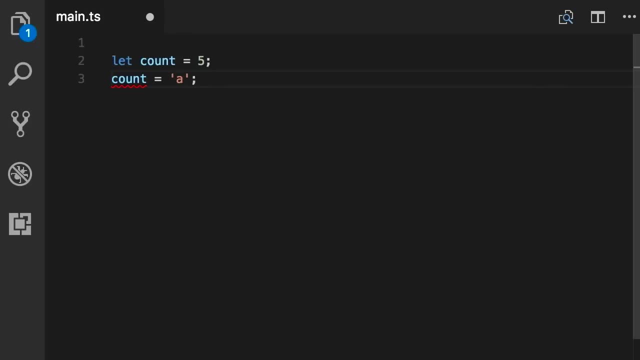 compile this using a TypeScript compiler and we will get valid JavaScript code. So if I go to terminal and type TypeScript compiler maints now, look, this is our mainjs. So we have this count variable and we have changed its value. We can perfectly execute this, no problem. 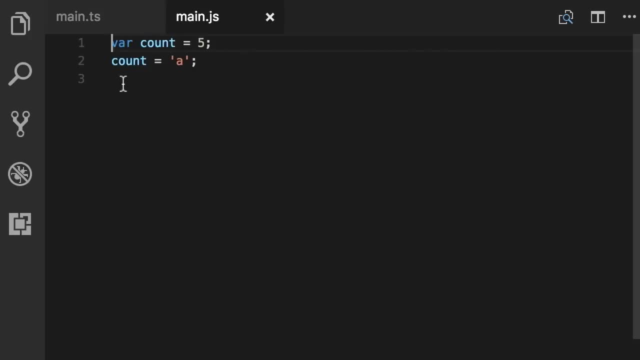 However, code like this is very likely that it's going to break at some point in the future, Because chances are we're going to use this count variable inside a for block, So our program is going to break at runtime. We don't want this to happen, right? That's one of the reasons. 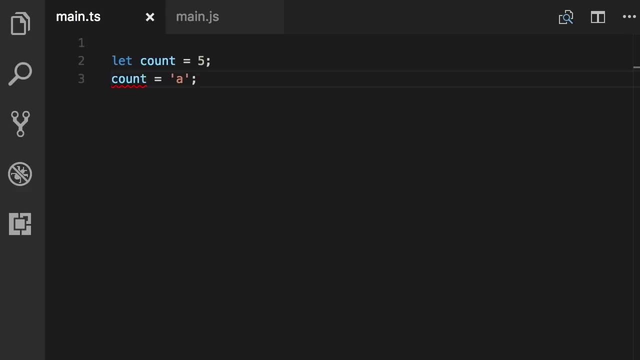 it's better to write the same code in TypeScript, so at least we can get a warning during the compilation step. Now, if you hover your mouse over this count variable, look at the tool tip. You can see a colon and number after this count. So this indicates the type of count variable in our 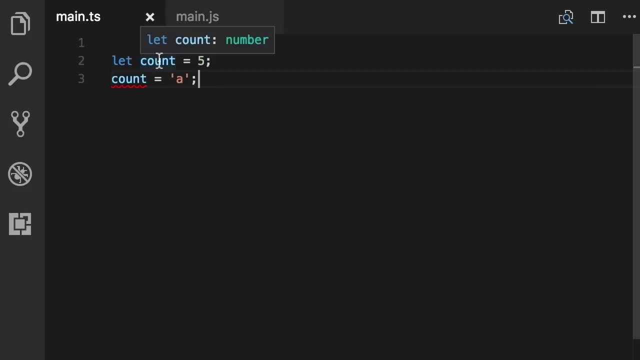 program. So here, TypeScript compiler inferred that the type of this variable should be a number, because we set it to number 5.. Now what if I declare a variable without initializing it? Let's look at its type. Its type is now any, And that's exactly. 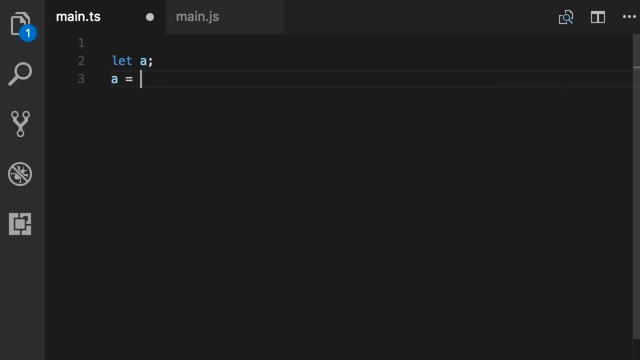 like the variables we declare in JavaScript. So I can set a to 1, then I can change the value to true and then set it to a string. Even TypeScript doesn't complain about this. So what's the solution If we don't know the value of a? 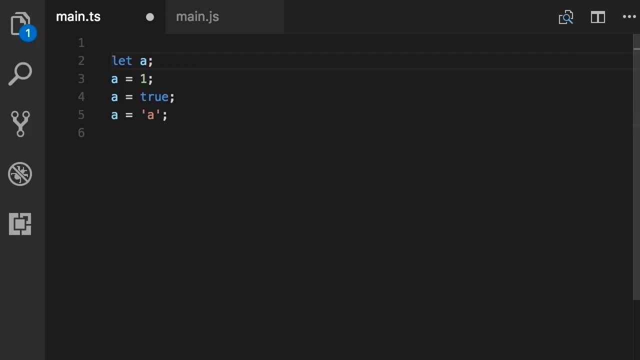 variable ahead of time. that's when we use type annotations. So here we add colon and after that we set the type of this variable like number, And then look on the third and fourth lines. we got compilation errors. Now in TypeScript we have a few different types, So we have number. 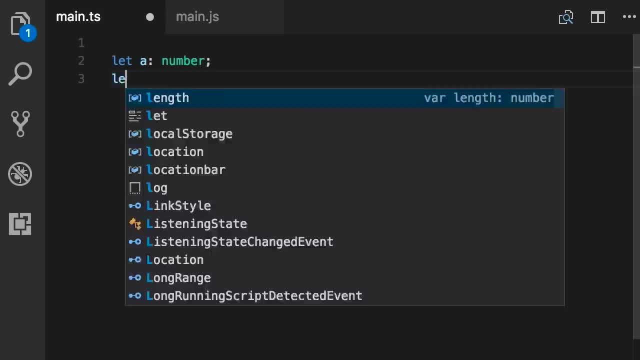 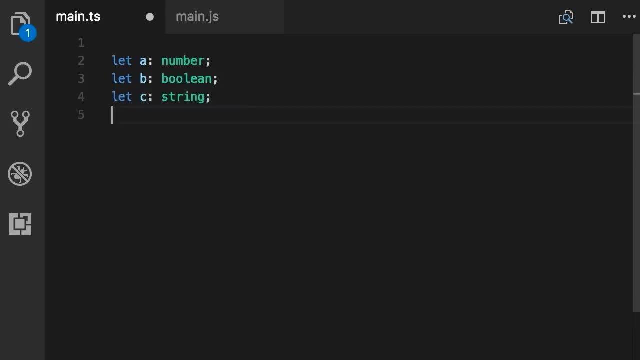 which can include any integer or floating point numbers. We have booleans, which can be true or false. We have strings. We have any that you saw earlier. We have arrays. So let's say we want to declare an array of numbers. We would use number with square brackets. 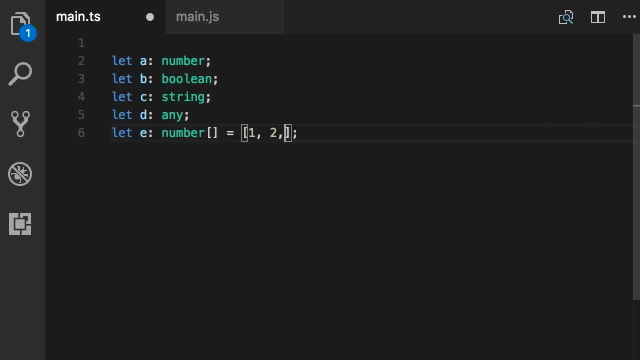 Now we can optionally initialize this to an array like this, Or we can declare an any array and with this, we can set this to an array with these values: 1, true, a and false. Of course, it's not a good practice. we want to avoid this, but I'm telling you what is possible. 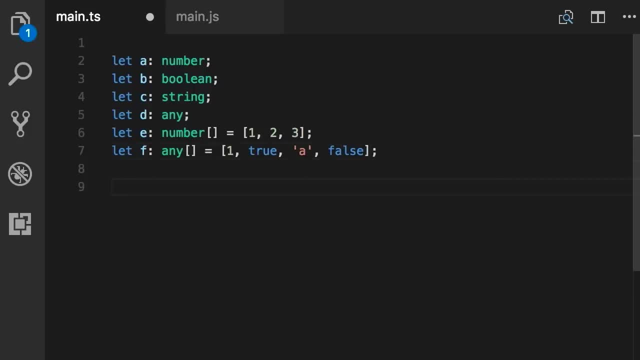 with TypeScript. Now we also have another type that I absolutely love, and that's enum. So let's say we are working with a group of related constants like colors. So in plain old or vanilla JavaScript we would define constant colors like this: So color red. we can set this to 0. 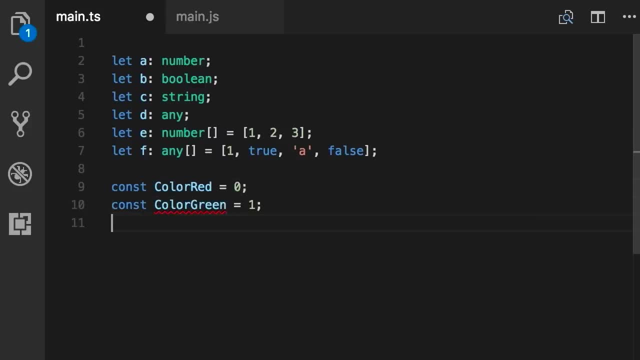 Constant color green, we set this to 1.. And constant color green, we set this to 1.. And this is a little bit verbose. In a lot of object-oriented languages we have this concept called enum, So we can put: 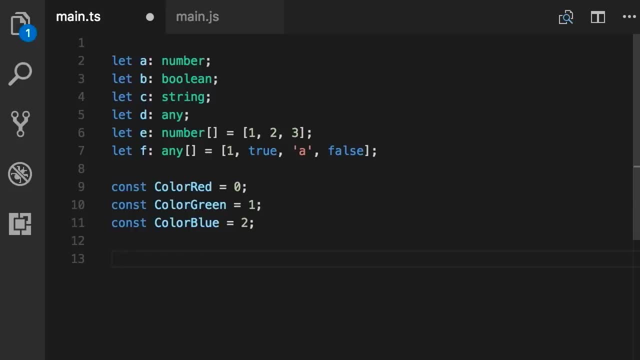 all these related constants in a container. So in TypeScript we can declare an enum like this Enum or lowercase. we give it a name like color- curly braces, and here we set the values, So red, green and blue. 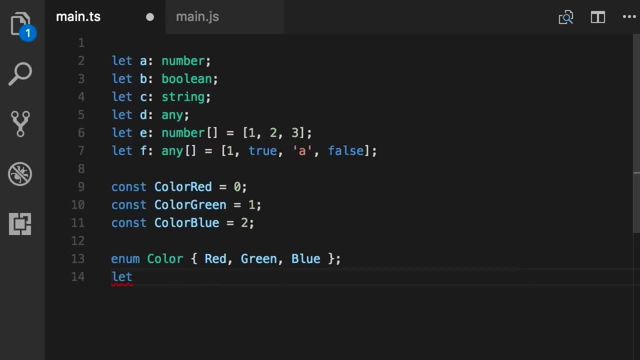 Then we can declare a variable like background color and set it to color dot. now look, we have IntelliSense here. So this tooltip you see here allows us to complete this code without remembering all the details, And this is one of the things I love about TypeScript. 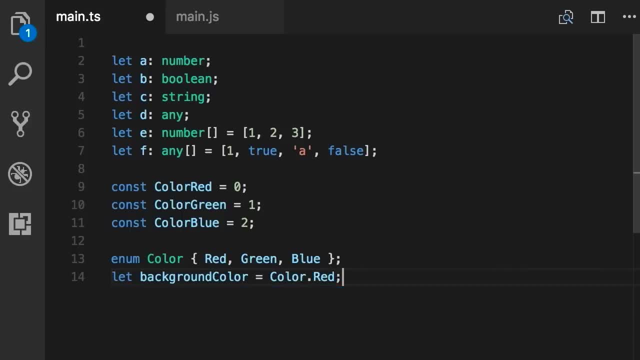 So let's set the background color to color dot red. Now, in terms of the values, the first element here automatically gets the value of 0. And each subsequent element gets an incremented value. So we don't have to explicitly set this, But as a best practice it's better to do so, because chances are. 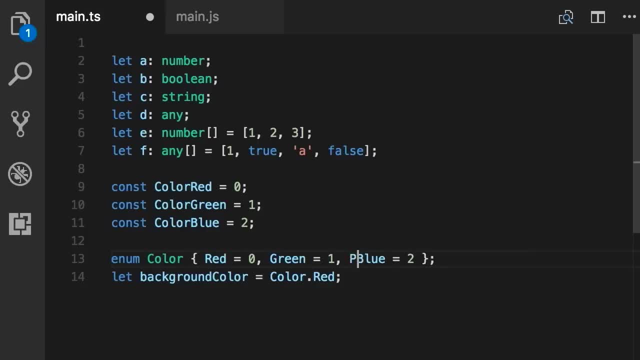 sometime in the future someone may come here and add a new color here, like purple, and then purple would automatically become 2, and the value of blue would change to 3.. So this may break parts of our application. So let me revert this by explicitly. 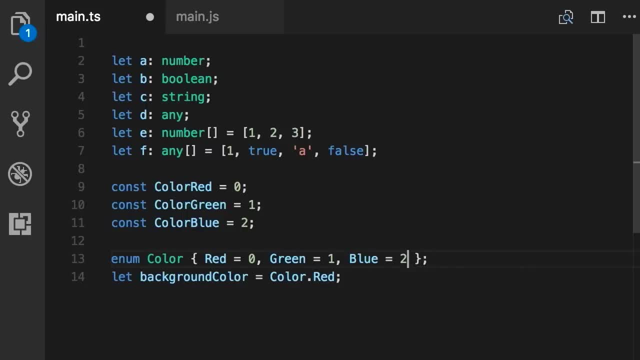 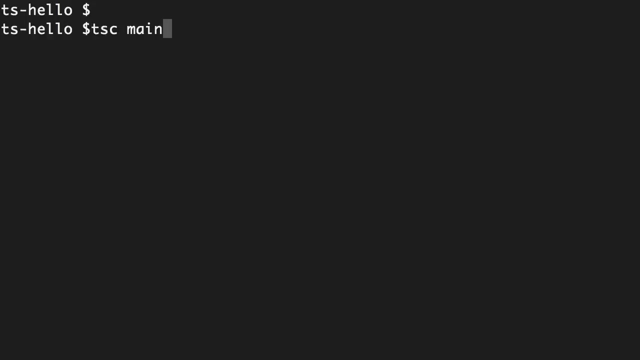 setting the values. So if somebody adds a new color here, like purple, then it will not change the value of blue. Now let me show you something. Let's compile this code and see how we get enum in JavaScript. So TypeScript compiler: main dot ts. 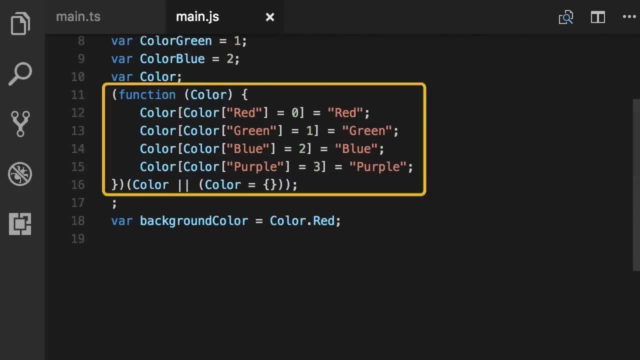 Look at this piece of code here. This is how we can implement the concept of enums in JavaScript. You can see it's very complicated. Now compare this with the other one. So this is the concept of enums in JavaScript. You can see it's very complicated. Now compare this with the other one. 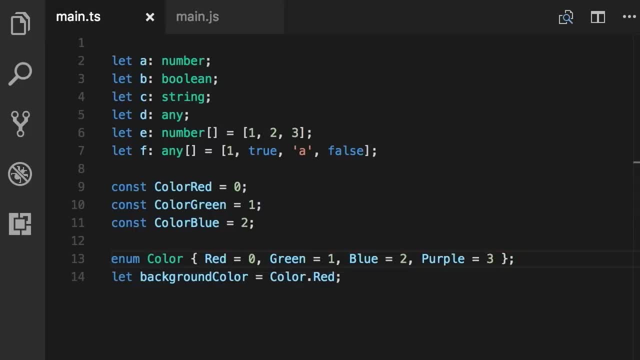 You can see it's very complicated. Now compare this with the other one. So the more you work with TypeScript, the more you're going to love this language. In this lecture, I'm going to show you the concept of type assertions in TypeScript. So I'm going to start by 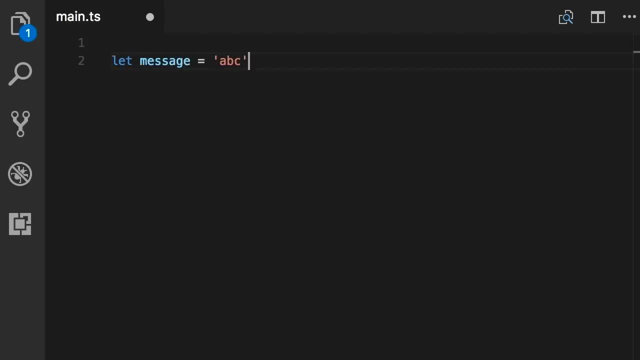 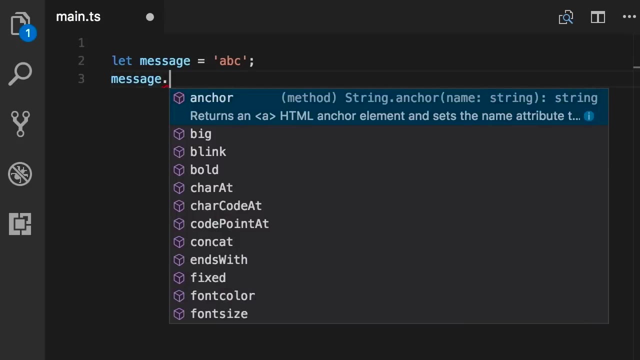 declaring a variable, like message, and setting it to a string. Now here we can type message, dot. and look, we get this beautiful intelligence and in this tool tip we can see all the things we can do with a string. So all these. 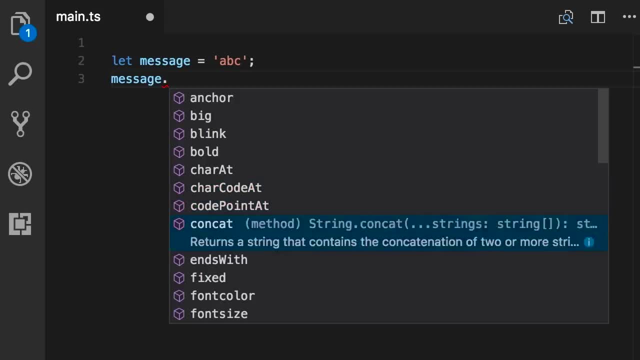 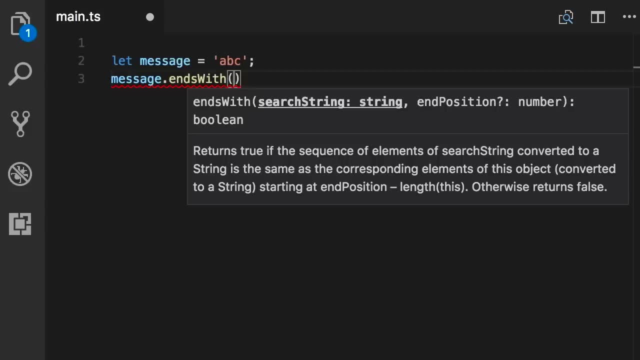 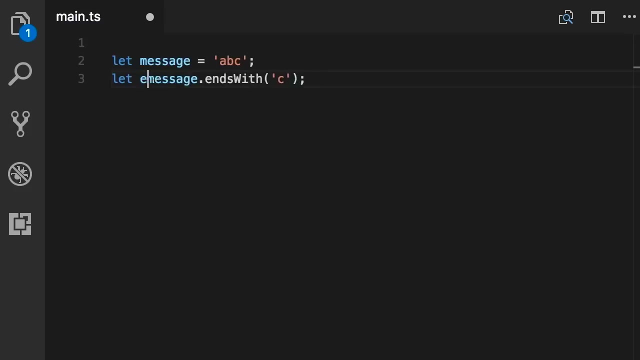 items with these purple icons are functions. for example, we have this function called ends with. we can call this and see if this message ends, let's say, with c, And this returns a boolean, So we can store the result in another variable like ends with c. 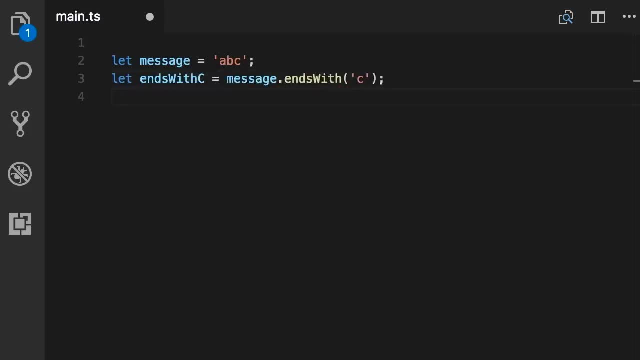 However, sometimes TypeScript may be a little bit confused about the type of a variable, For example, I'm going to remove this initialization here and initialize this variable on the second line, abc. Now look at the type of this message variable It's any, because by default, when we don't set a value, the type is: 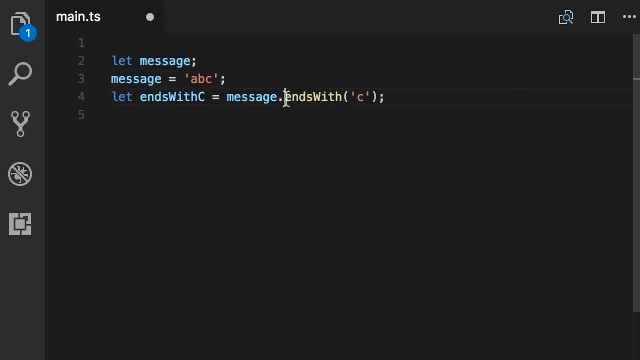 any. Now the problem here is that if I delete this and type period, look we don't get that intelligence anymore, Because ends with is something that we can do with a string, not with an object of type any. So what should we do In this case? we need to explicitly: 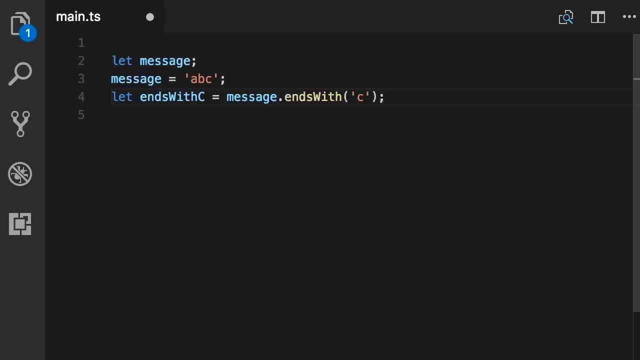 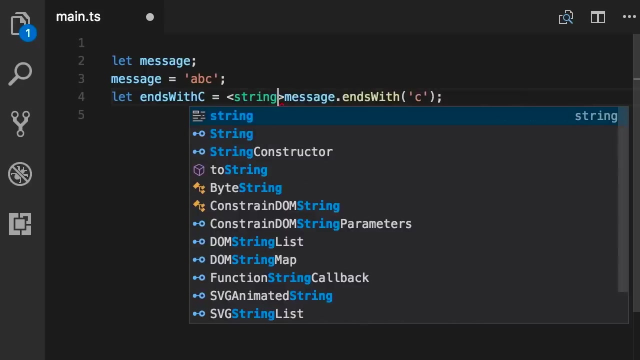 tell TypeScript compiler that this message variable is actually a string, And this is what we call type assertions. Now how do we do type assertions? There are two ways. One way is to prefix this variable with angle brackets, and here we put the type like string. Now we need to enclose. 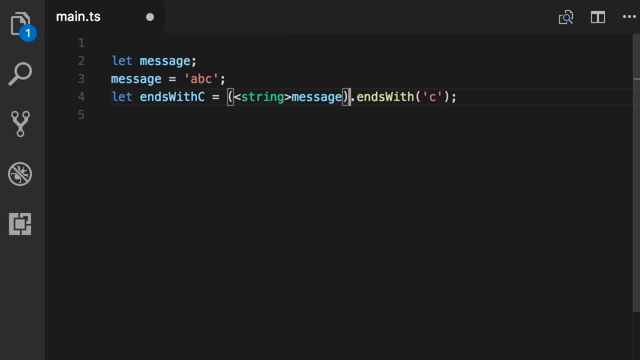 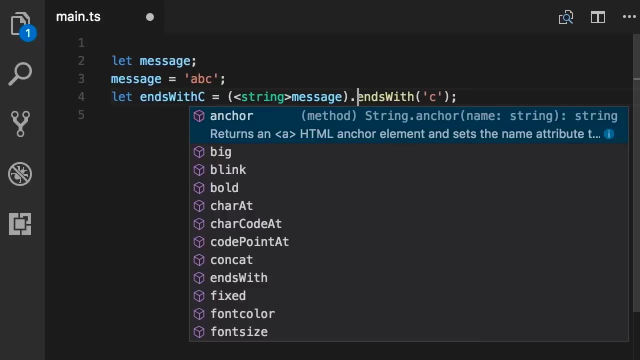 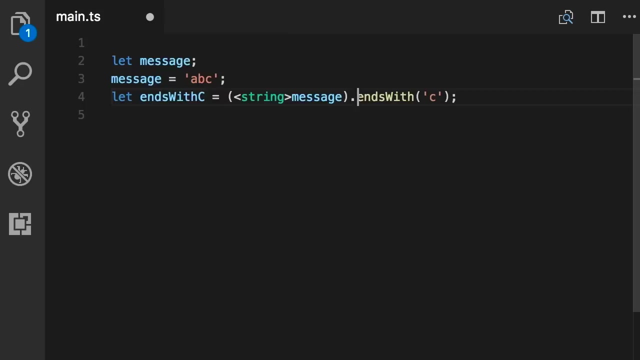 both these parts in parenthesis, like this: Then if we press period, we get our beautiful intellisense with all the functions or methods available on string objects. Now there is also another way to do: type assertion. So let's change the name. 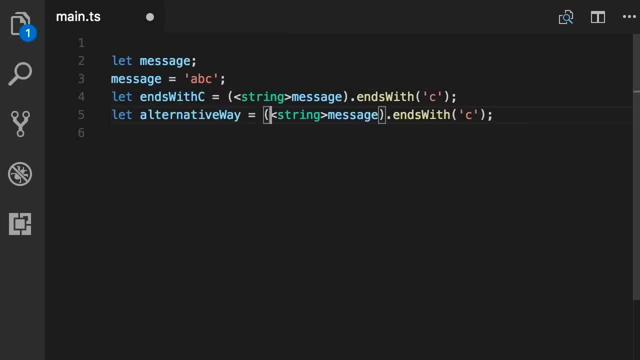 of this variable to alternative way, and here instead of angle brackets we use message as string. They are exactly the same. The approach you choose is purely your personal preference, But the first approach is what you see more in a lot of tutorials and code bases out there. 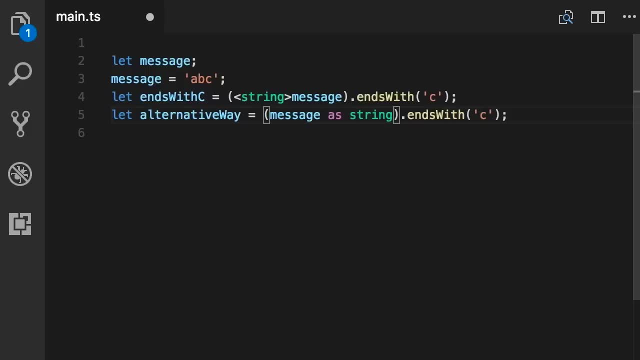 Now I just want to clarify something here. This type assertion does not change the type of this variable at run time. In fact, it's not going to restructure that object in memory. It's purely a way to tell TypeScript compiler about the type of a variable. so 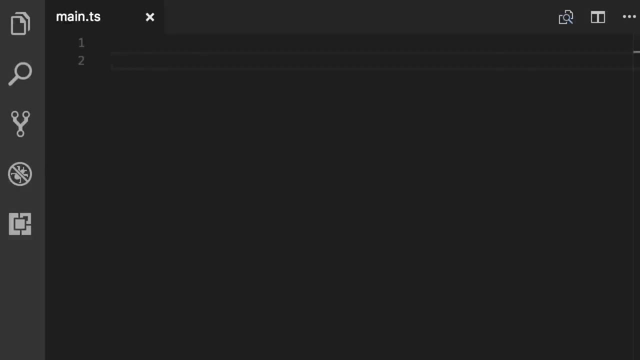 we can access the intellisense. Another concept you need to know when using TypeScript to build Angular applications is the concept of arrow functions. So in JavaScript we can declare a function like this: Let log. we set this to a function. this function takes. 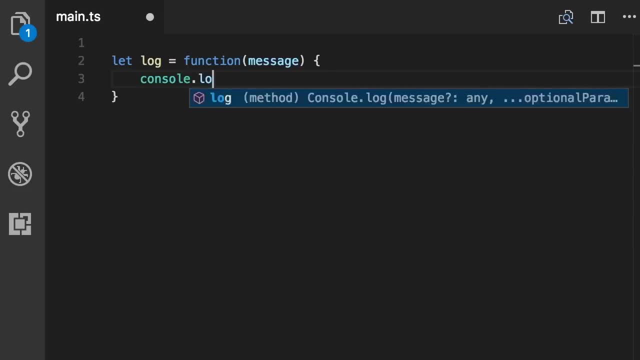 a message object and simply logs it on the console Like this. Now, in TypeScript there is a shorter way to define this function, So let's call the other one: do log. Now we don't need the function keyword anymore, We can simply add the parameters. in this case, 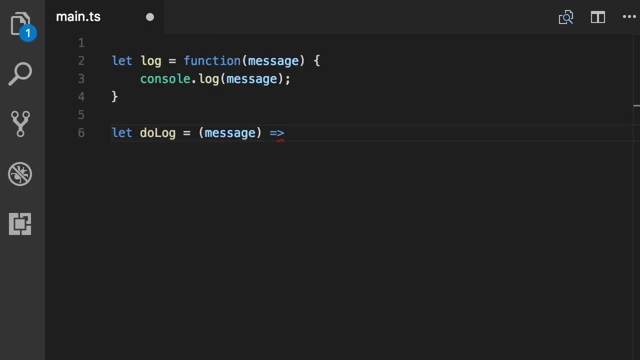 message. Then we add this arrow- and that's why we call this an arrow function- And finally the code block, So consolelog message. Now, if our function has only one line, we can even exclude these curly braces, So we can make this code. 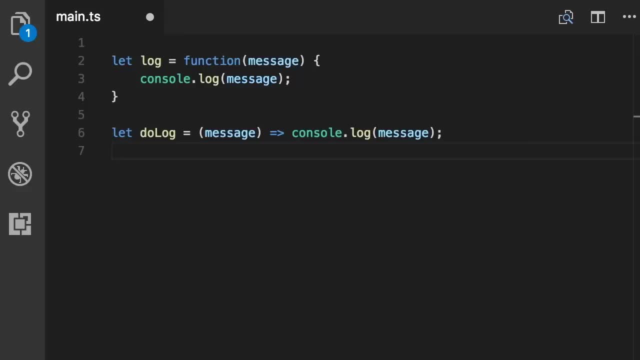 a little bit shorter and cleaner, like this. If you are working with C sharp, you have seen this before. in C sharp we call this a lambda expression. In TypeScript we call it an arrow function. It's exactly the same thing. 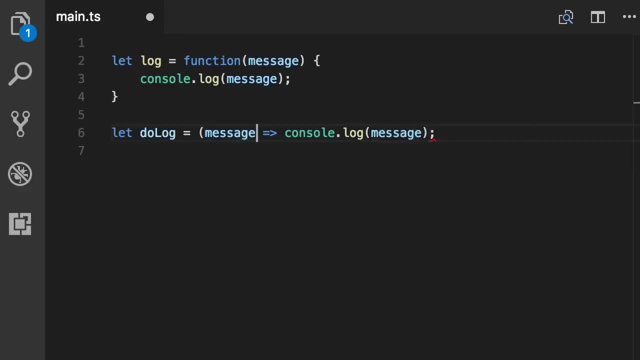 Now, if you have one parameter here, you can even exclude the parenthesis, But I personally don't like this because I think it makes the code a little bit less readable. So I always like to put my parenthesis here to indicate to the reader of this code that these are. 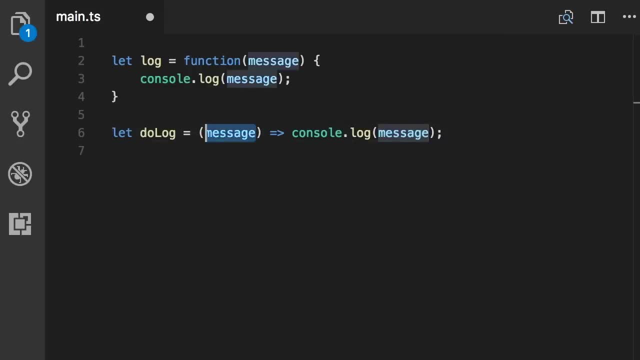 the parameters. Now what if we don't have any parameters? We just add empty parenthesis and, of course, here we don't have the message. So if you have not seen this before, get used to it. it's a really nice and clean way to define functions. 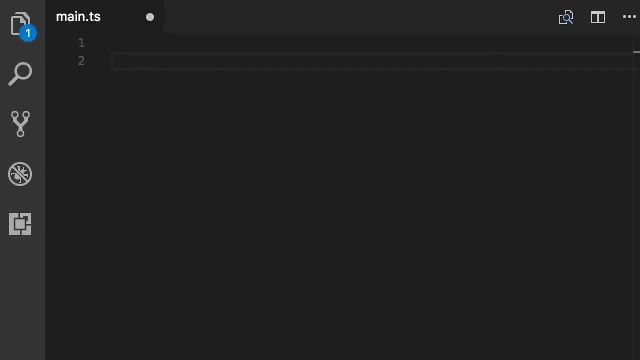 Alright, now let's see how we can use custom types in TypeScript. So I'm going to start by declaring a function like draw point. So this function takes an x and a y and simply draws it on the screen. Now we don't want to worry about the actual drawing algorithm. 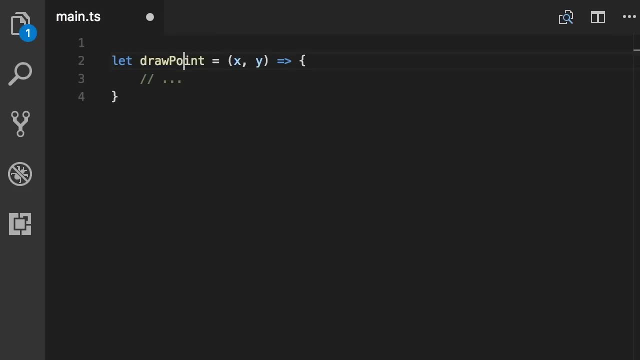 we just want to focus on the signature of this function. Now, this function is not too bad. here we have only two parameters, but sometimes, when working with more complex concepts, you may end up with a function that has so many parameters, like this. 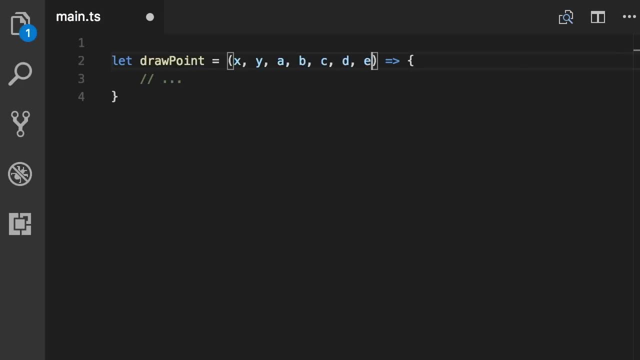 This is really, really bad, and it's something you should avoid at all times. In those situations, it's very likely that a group of these parameters- maybe all of them- belong to a single concept. As an example, think of a car. A car has so many different properties. 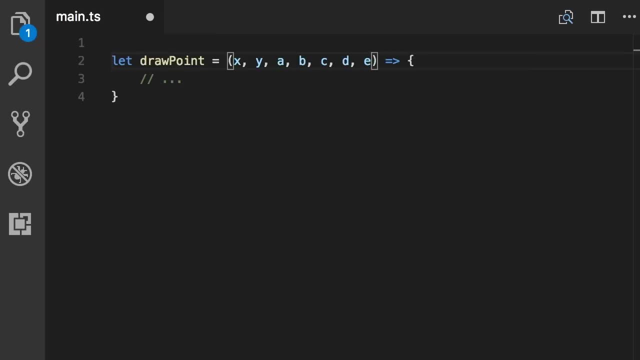 We don't want to pass all those properties to a function like drive car. Instead we want to encapsulate them inside an object and only pass that one object here. So in this example, instead of passing x and y here, it's better to pass 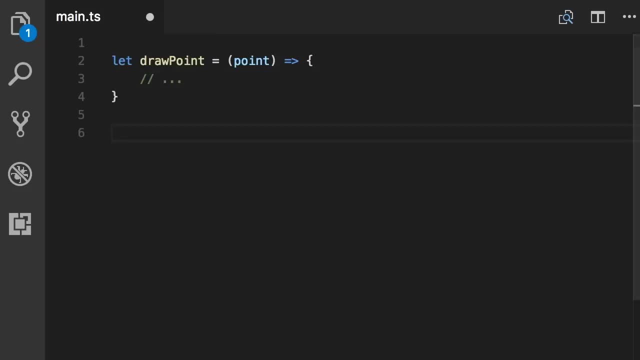 a point object And then we can call this function like this: draw point. we give it an object with two properties, x and y. So now our function has a cleaner syntax. However, there is a problem with this implementation. Instead of a point object, 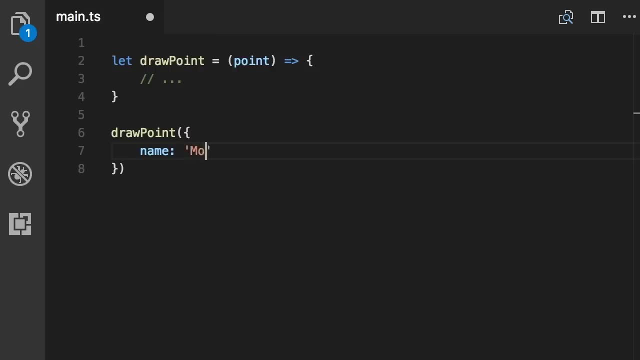 I can pass a person object that has a name property And nowhere. here we are getting a compile time error. But we know that this code is going to break at runtime Because the algorithm in our draw point function is expecting x and y properties. 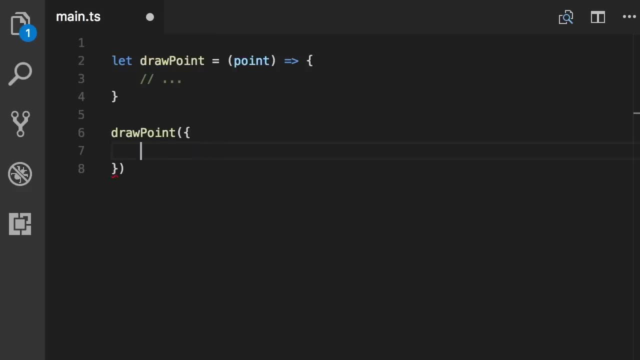 So what's the solution? Well, let me revert this back. Okay, we've got x and y, So there are two solutions to solve this problem. One way is to use what we call inline annotation, So just like we can annotate this parameter with a type like number. 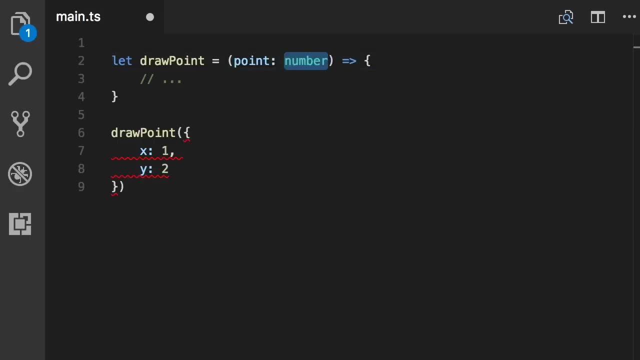 we can annotate it with a custom type or custom object. So here we add curly braces to indicate an object. This object is going to have a property called x, which is a number, And also another property called y, which is again. 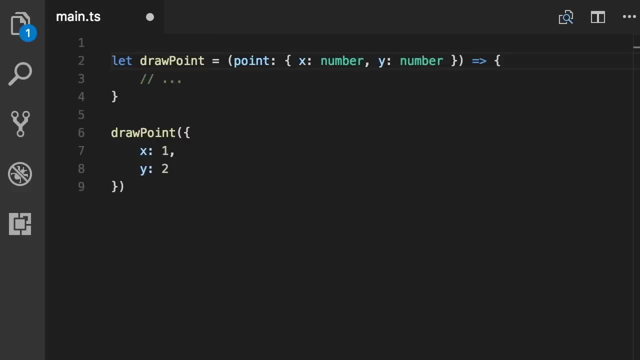 a number. So this is what we call inline annotation. It works fine for simple cases, but the problem with this, as you can see, is that this is a little bit verbose. Also, chances are somewhere else we might have another function. 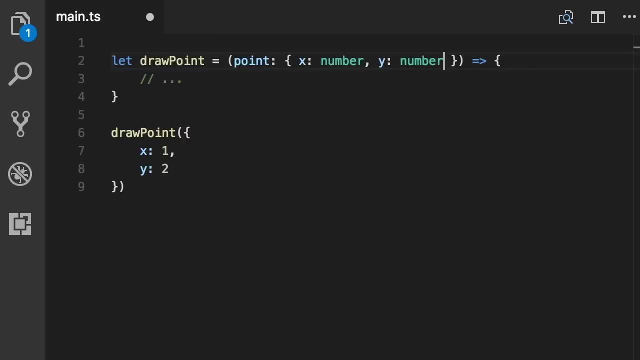 that expects a point object. We don't want to repeat this object literal in multiple places. So in those cases a better approach is to use an interface. If you have worked with object oriented program languages like C, sharp and Java, you know the concept of interfaces. 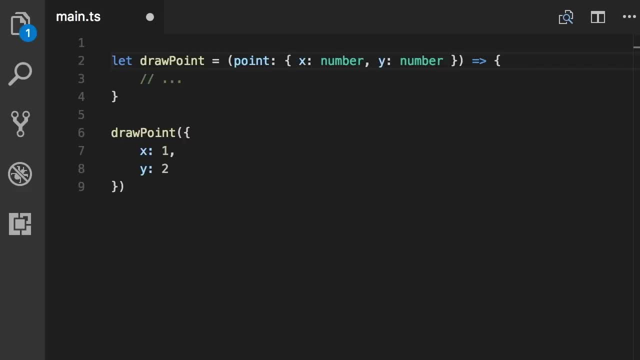 You have the same concept in typescript. Now, if you have never worked with interfaces, let me show you how they work. So, on the top, I define an interface and I'm going to call this point Curly braces. then I 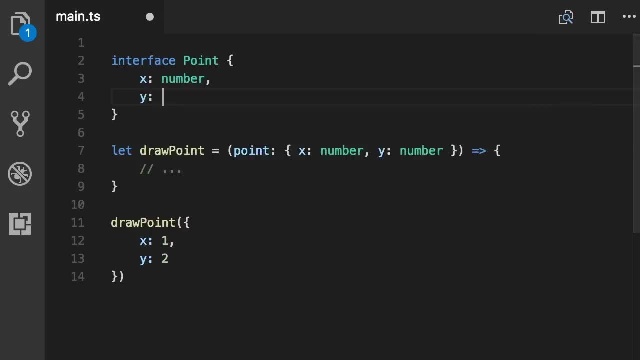 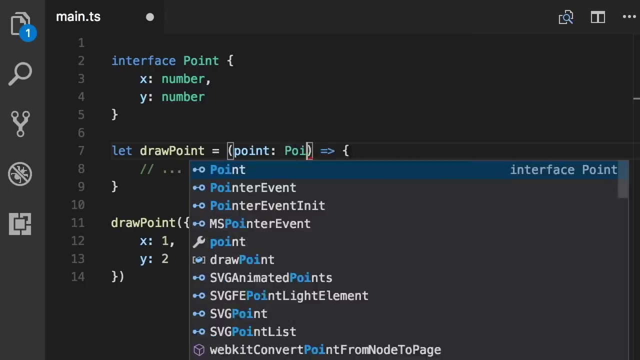 add x as a number and y as a number. So with this interface I'm defining the shape of an object And then I can simplify this declaration and set the type of this parameter to point. This is much cleaner and 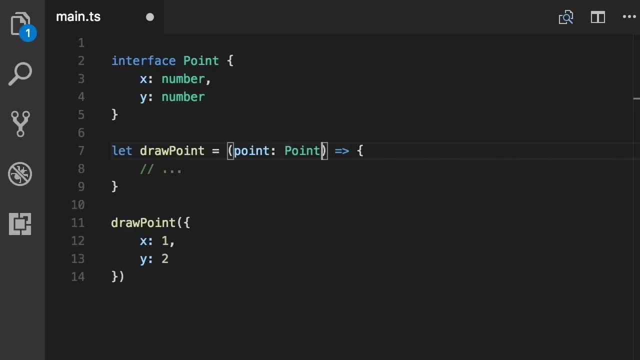 we can also reuse this in multiple places. Just one thing: note the naming convention I have used here. So because I'm introducing a custom type, I've used pascal naming convention, So the first letter of every word in the name. 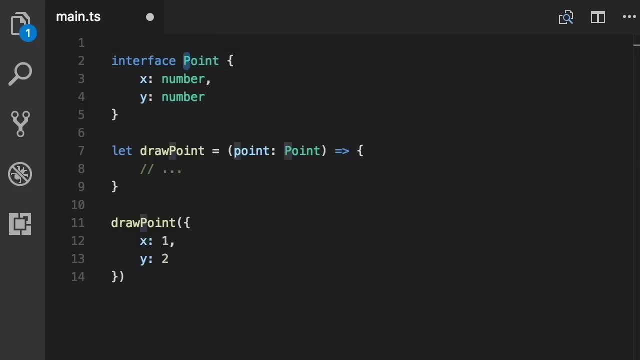 of the interface should be capitalized. So here we have uppercase P, not a lowercase p. okay, So when using interfaces, always use pascal naming convention. So in the last lecture we used an interface to define the shape of a point object. But there is 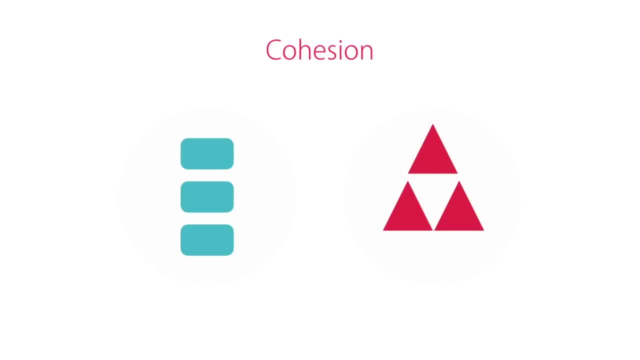 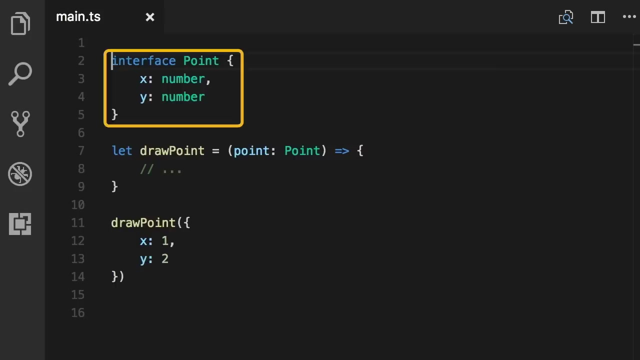 a problem with this implementation. In object oriented programming languages we have this concept called cohesion, which basically means things that are related should be part of one unit. They should go together. This is what we call cohesion. Now back to this example. on the top, we have used an interface to define. 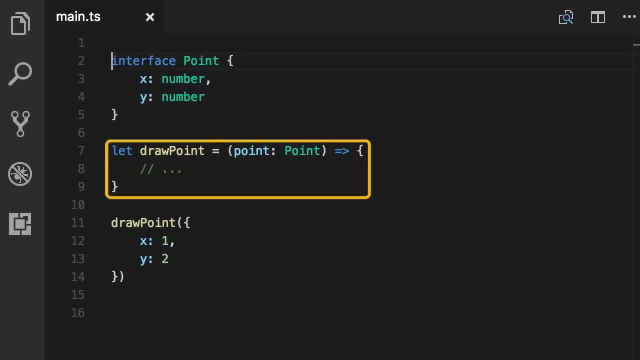 the shape of a point object, And below that we have a stand alone function, And this is where we have violated the cohesion principle. So the concept of drawing a point is highly related to the structure of a point. It should not be a separate function. 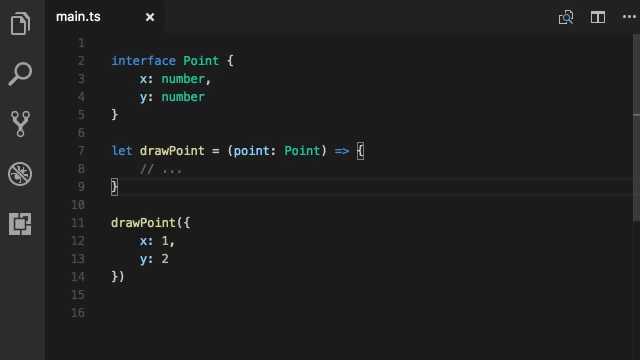 Now, if you're going to build a utility library for working with points, chances are you're going to create another function, like get distance, that calculates the distance between two points, So point A of type point and point B of type point, And this goes to this code block. 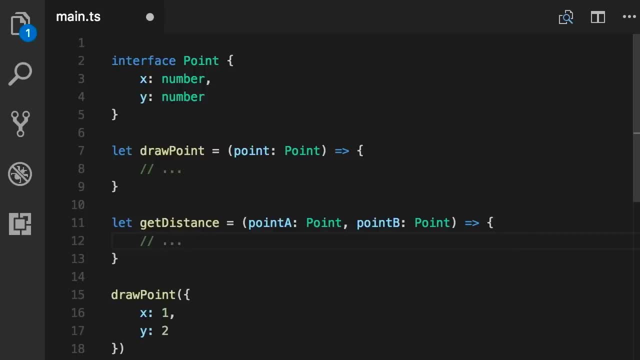 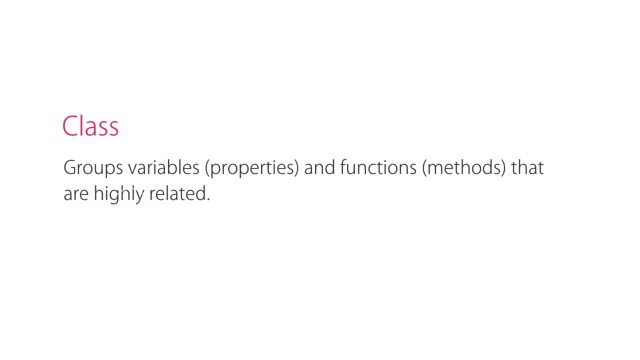 Again we have violated the cohesion principle. We have two functions hanging in the air, separate from the point object. Since these concepts are highly related, they should be part of one unit. In object oriented languages we call that unit a class, So a class. 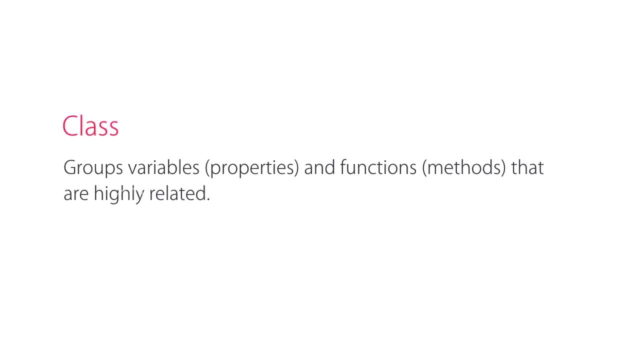 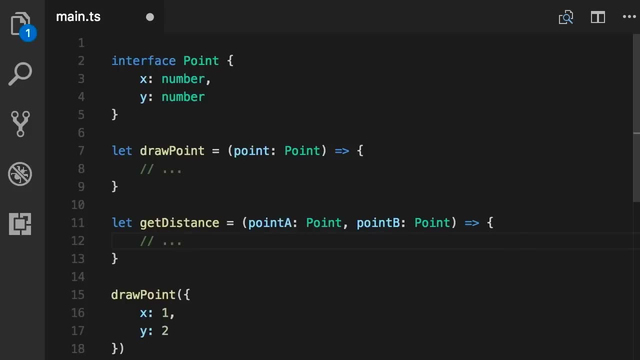 groups, properties and functions that are highly related. Now, in this implementation, unfortunately, we cannot move these two functions inside our interface, Because interfaces are purely for declarations. They cannot include any implementation. In other words, we cannot have the algorithm for calculating the distance between two points. 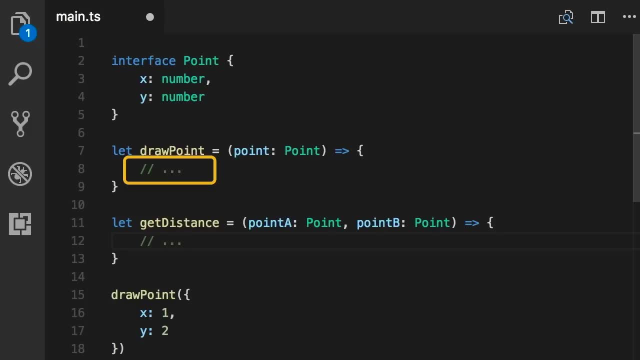 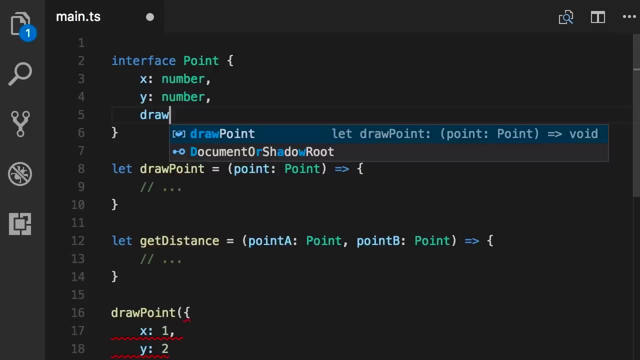 or drawing a point inside this interface. What we can do instead is to add a function here, a function declaration. so we're going to have a draw function that takes no parameters and returns void, Which means it doesn't return anything. Now you might be asking: why don't we have this point? 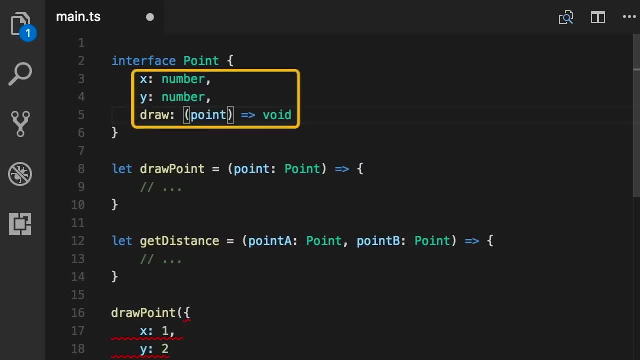 parameter here, Because if all these members- x, y and draw- are part of one unit, we don't need to pass x and y as parameters to the draw function. This function can directly access these properties- x and y- in the same unit. 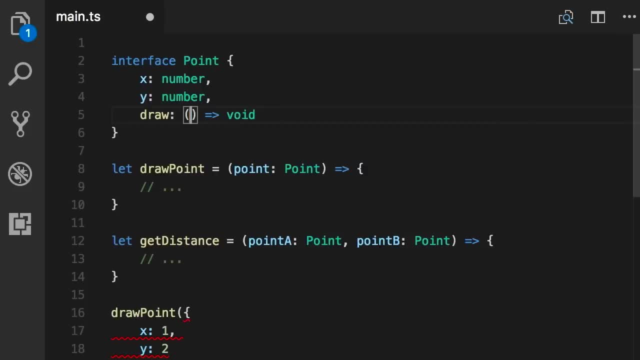 So we don't need this parameter here Now. in interfaces, as I said, we cannot have implementation, We can only have the signature of a function. So with this interface we're telling typescript compiler that our point objects should have two properties: x and y. 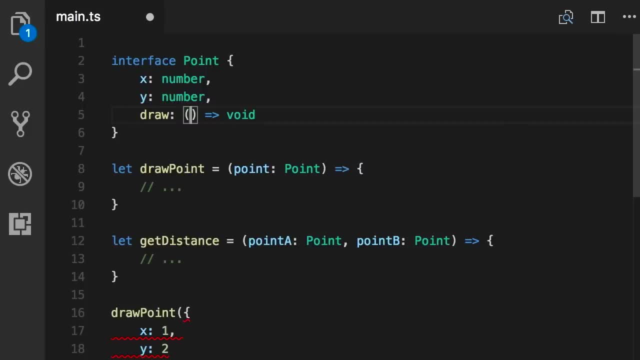 and a function called draw. The implementation of that is somewhere else. So what should we do now? to apply the cohesion principle here, We need to use a class instead of an interface. So on the top I'm going to change the type to class, and here: 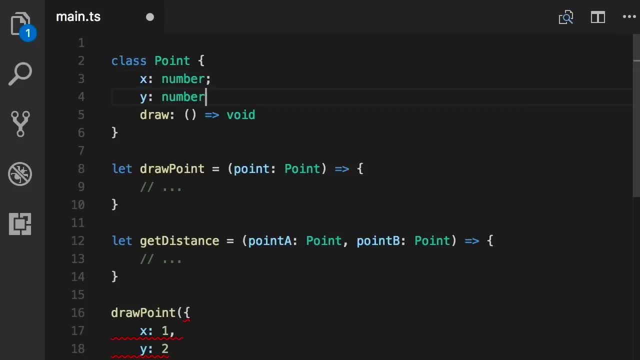 I'm going to replace this comma with semicolon, so our point class has three members. the first two members are what we call fields that we use for storing data, And the third member is a function. Now, here in this class, we can have: 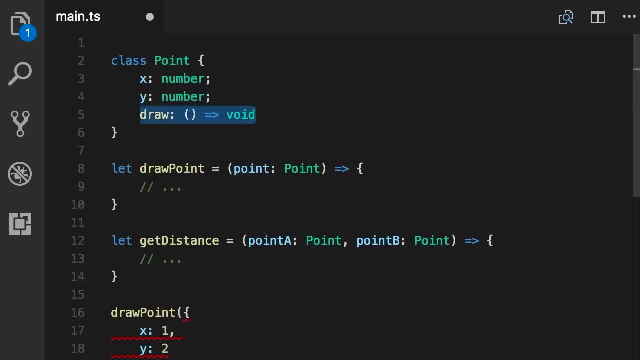 the actual implementation of this draw function. So we can simply define it like this draw, and then add all that logic for drawing a point. Now, similarly, we can have another function, getDistance, that returns the distance between this point and. 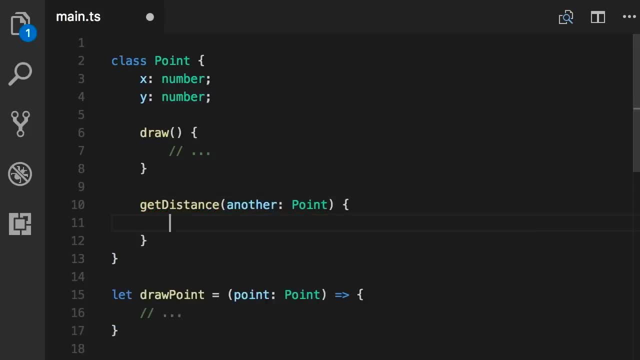 another point like this: Again, all that logic will end up here. Now, with this restructuring, you can see that everything about a point is in one unit, in one class. So we have the coordinate, which includes x and y. 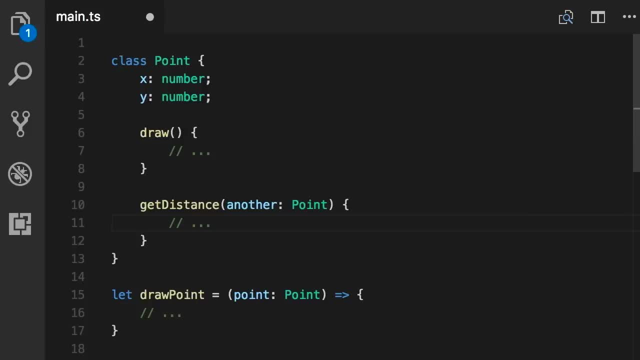 and two functions: draw and getDistance. Now, in object oriented programming terms, we refer to these members as fields and to these functions as methods. So when a function is part of a class, we call it a method. Alright, now, with this new implementation, 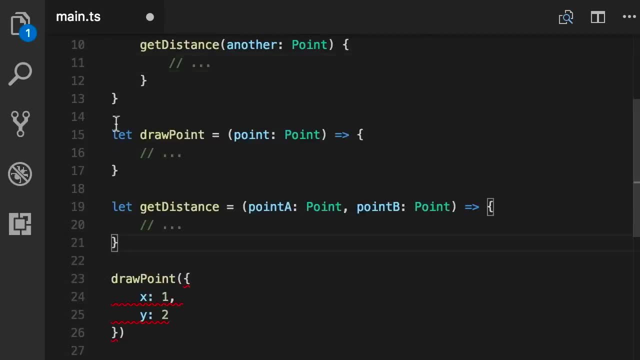 we don't want these two functions hanging in the air, So delete. This is a much better structure. Also, you're not going to call drawPoint like this anymore, So here's our point class. In the next lecture I'm going to show you how to create an object of this type and call the. 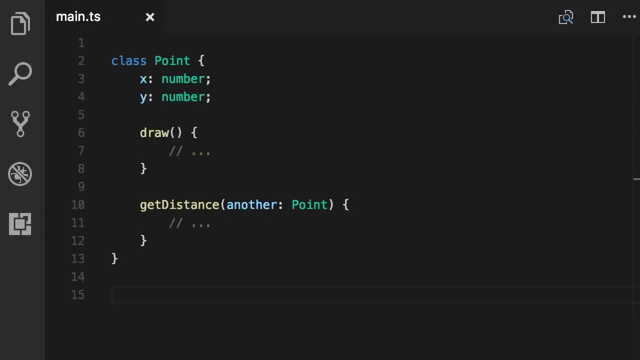 draw method. Alright, so here's our class. Now let's declare a variable of this type. So let point be of type point, And then we can type point dot. look, we have this beautiful intelligence. we have two methods. 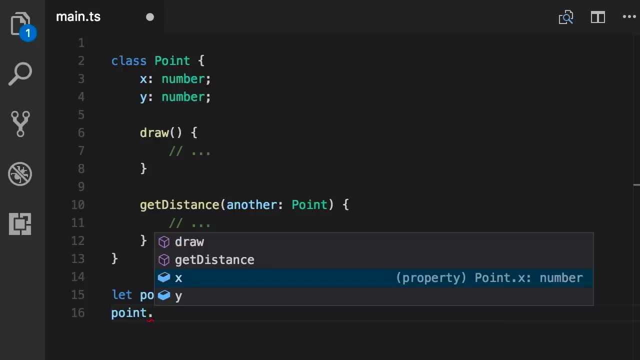 draw and getDistance and two fields, x and y. Now in TypeScript we also have a concept called property, which is different from a field, but a lot of people use these terms interchangeably. Later in this section you're going to learn the difference between: 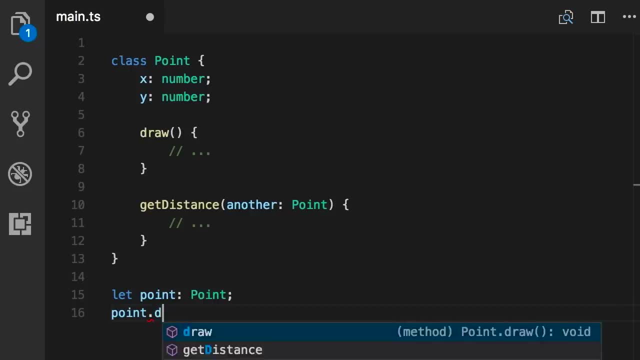 fields and properties. Now, if you want to call the draw method, simply call it like this. So this draw method is now part of the concept, of a point. It's not a function hanging in the air polluting the global namespace. Now for this demo. I'm going to add: 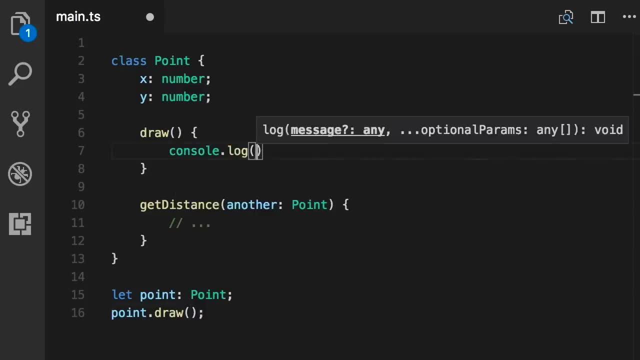 a simple console dot, log here and display the coordinate of this point, So x. now here I want to add the x field, but we cannot use it like this. We need to prefix it with this dot, So that refers to this field in this class, And then 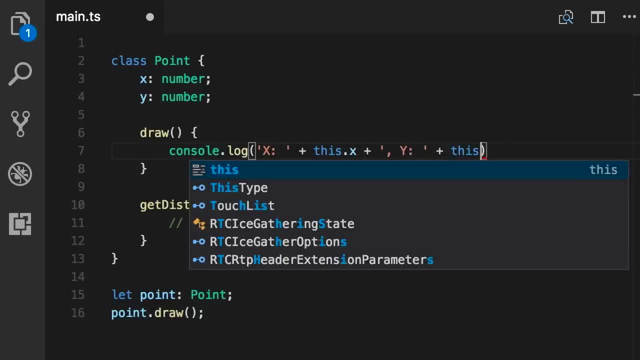 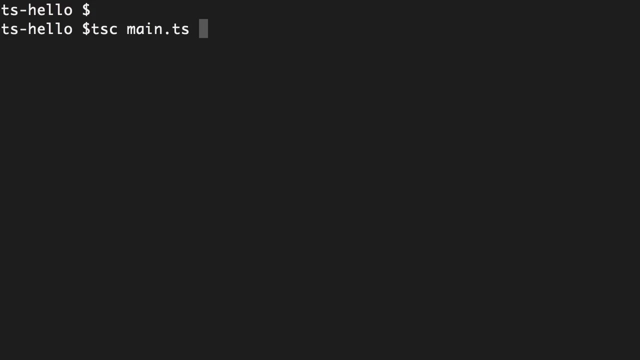 I'm going to add y is once again this dot y. Now let's compile and run this program and see what happens. So, tsc, what should we type here? Maints, and we can shortcut by adding this pipe here: 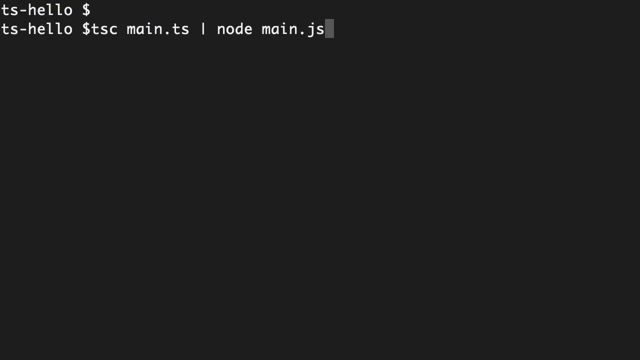 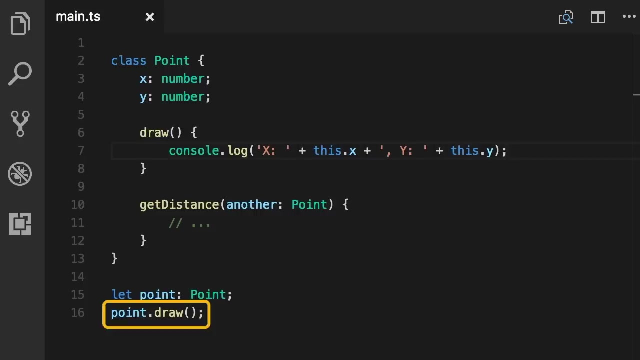 type node and then mainjs. okay, We got a runtime error: Cannot read property: draw of undefined. So this is the problem When we call this draw method. this point object was undefined Because here, unlike the basic types we have in TypeScript, like numbers, strings, booleans, 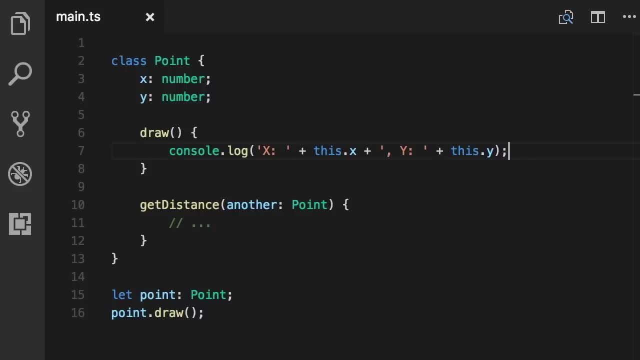 we're dealing with a custom type. When defining an object of a custom type, we need to explicitly allocate memory to it. How do we do that? Well, here, where we declare the point object or the point variable, we initialize it using the new operator. So this object. 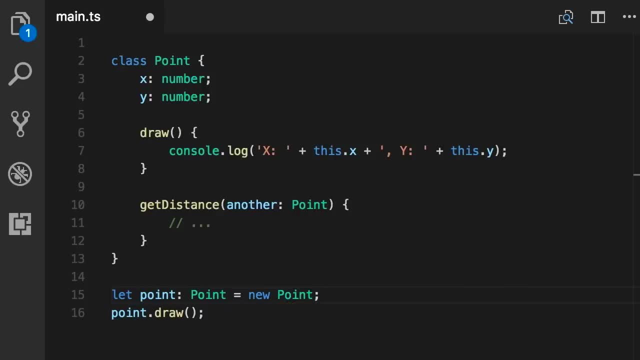 is a new point, And here we add parenthesis. This is the syntax. Now you can see that we have repeated this point here twice, so we can make this code a little bit cleaner by removing this type annotation, Because TypeScript compiler can infer: 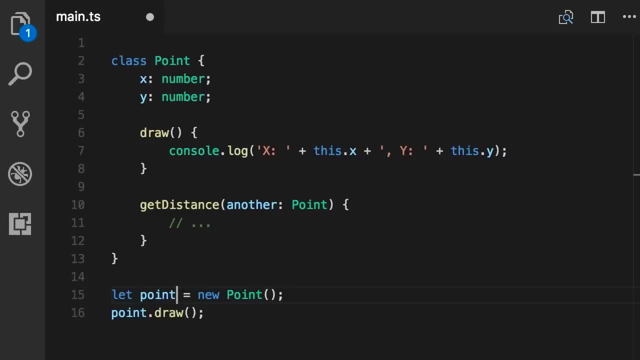 from this assignment here that the type of this object is a point object, And let's verify that. So look, you're working with a point object. Now one more time: save. so back in the terminal TypeScript compiler maints and then node. 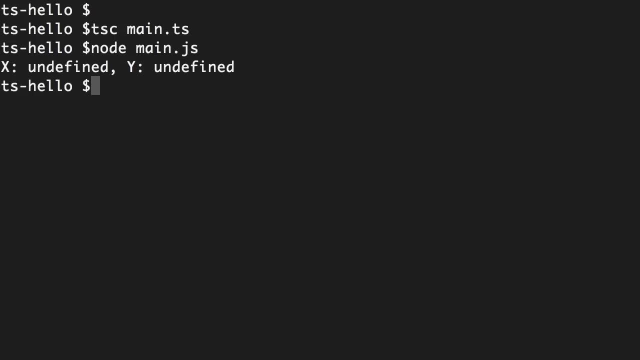 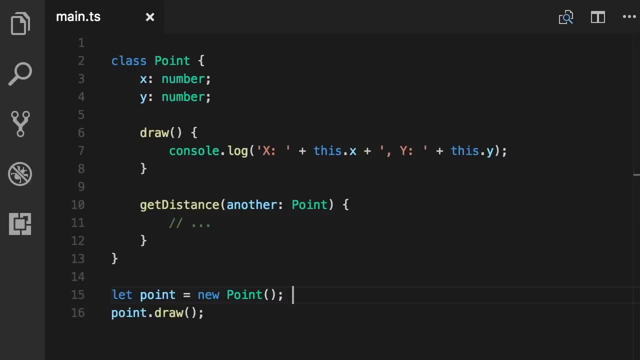 mainjs. Okay, we didn't get an error, but you can see that these x and y fields don't have a value because by default, they are undefined. So we can get back here and set pointx to, let's say, 1, and 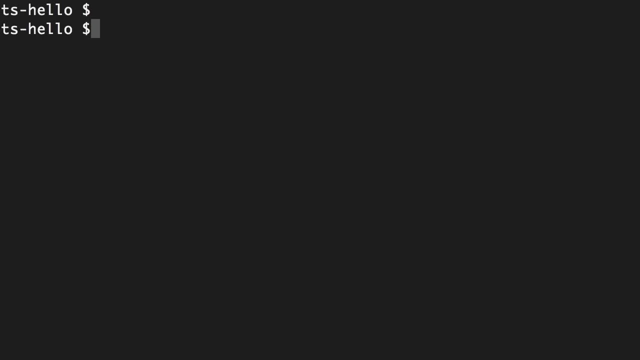 pointy to 2.. Now back in the terminal TypeScript compiler maints. I actually made a mistake earlier, so instead of this pipe operator we need to use double ampersand. on Mac I don't know the windows equivalent, so with this we can combine. 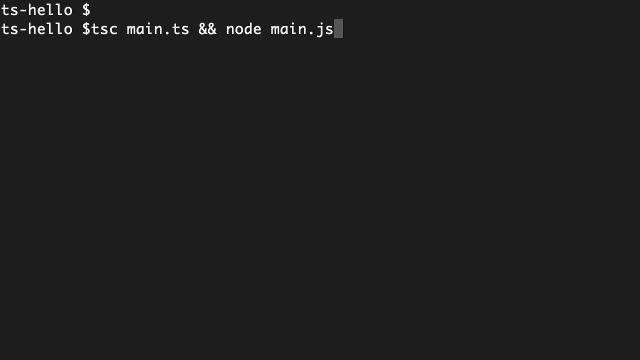 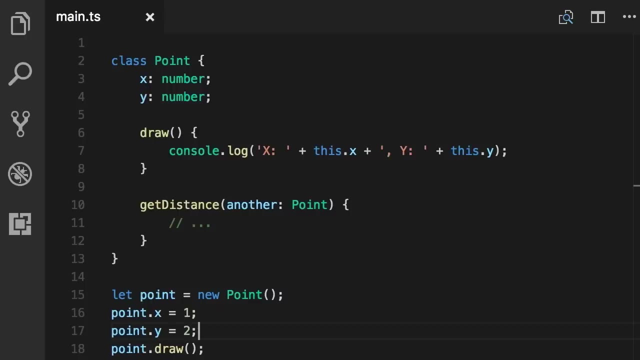 multiple commands, So node mainjs. Alright, beautiful. x is 1 and y is 2.. So this is how we use the classes that we define in our programs. Now I want to highlight something here: This point here is a class, but this point here is an object. 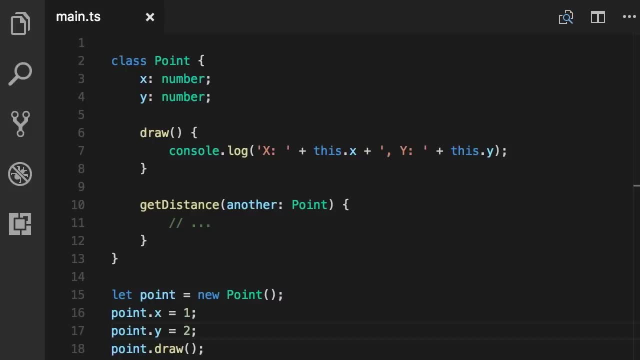 An object is an instance of a class. As a metaphor, think of the concept of a human. Human could be a class, but when we create instances of this class like John, Bob, Mary, these are all objects. So that's the difference between. 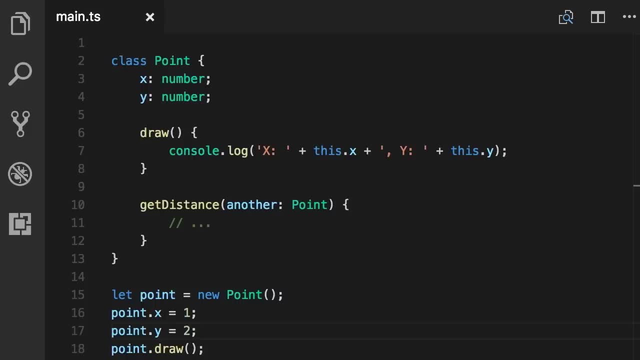 a class and an object. Next we're going to look at constructors. Alright, so I've simplified the code from the last lecture. I simply removed the method get distance because we're not going to use it later in this section. So here on the top we define a point class. 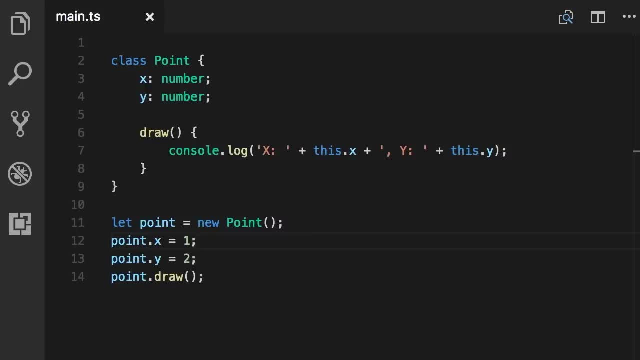 and then, below that, we initialize a point object. Now this code is a little bit verbose, because we have three lines to create a point object and put it in a valid state. What if this point object had a few other properties that we had to initialize like this: 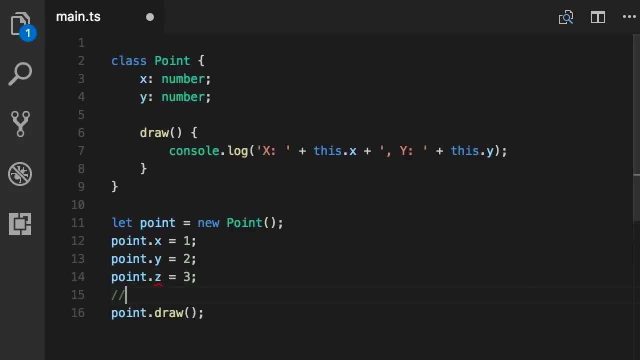 And maybe a few more here. Is there a cleaner way? Absolutely, So let me delete this first. Alright, in object oriented programming languages we have this concept called constructor. So every class can have a constructor, which is basically a method that is called when we create an instance of that class. 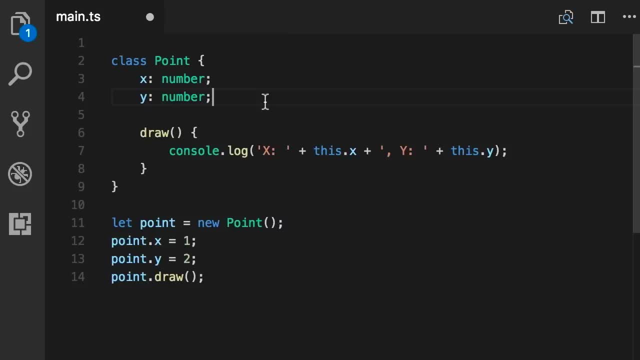 So let me show you how it works. In the class I'm going to add a method. the name of this method is constructor. This is a reserved keyword in typescript. Now this method can have parameters, so x, which is a number, and y, which is also a number. 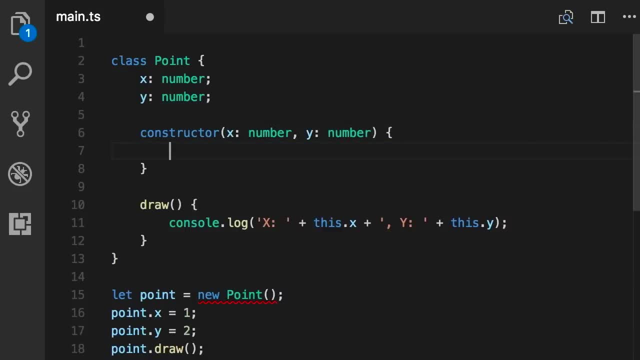 And then here, in this method, we can initialize these fields. So what should we write here? This dot x, we set it to this x argument that we get here, And similarly this dot y, we set it to y. Now, look, we got a compilation error here, Because when creating a, 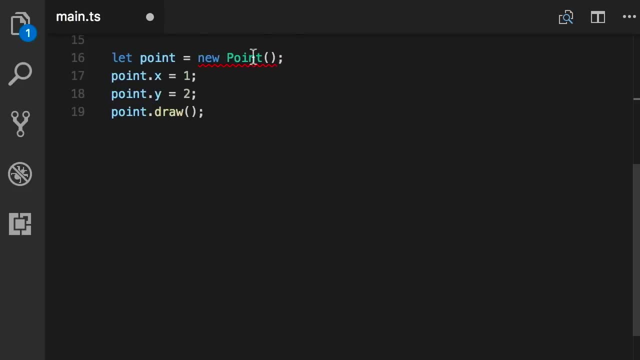 new point. object: we need to supply these values. Look at the error. supplied parameters do not match any signature of call target. So here we need to supply the values for x and y, 1 and 2. And with this we can simplify. 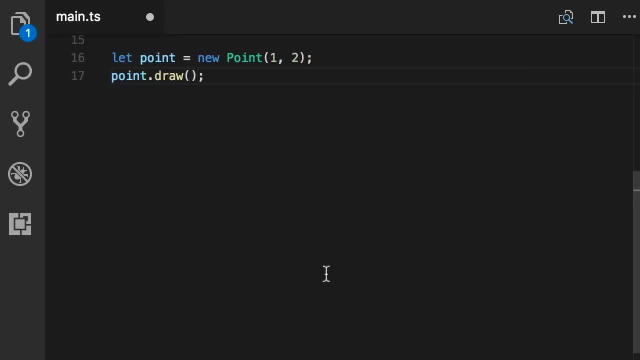 this code and get rid of these two extra lines, And here is the end result. Now what if somewhere else in our program we don't know the initial coordinate of a point? In other words, what if I want to create a point object: 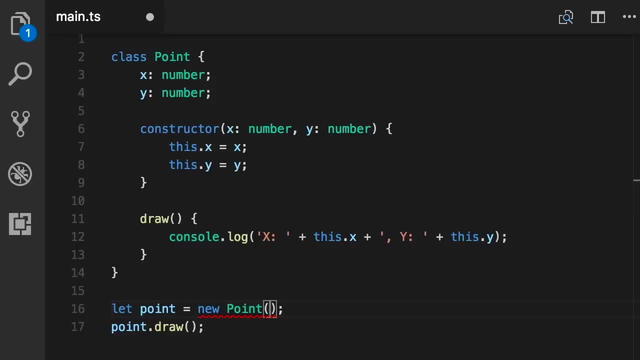 without setting these values? Is that possible? Yes, absolutely, But it's a little bit different from how you have seen that in other languages like C sharp and Java. In C sharp we can have multiple constructors. in typescript we can't. So the solution for 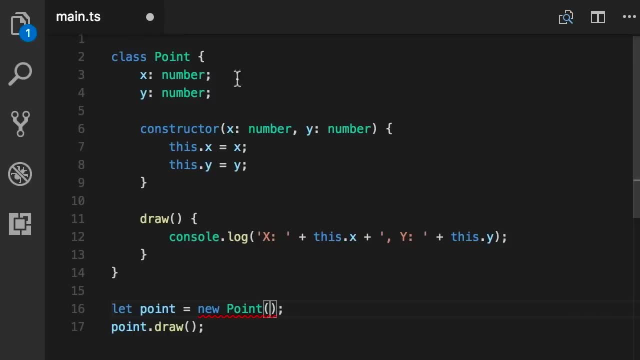 this is to make these parameters optional. So here after x I add a question mark and that makes x optional And similarly y should be optional as well, Because once you make a parameter optional, all the other parameters on the right side of that parameter should also be optional. 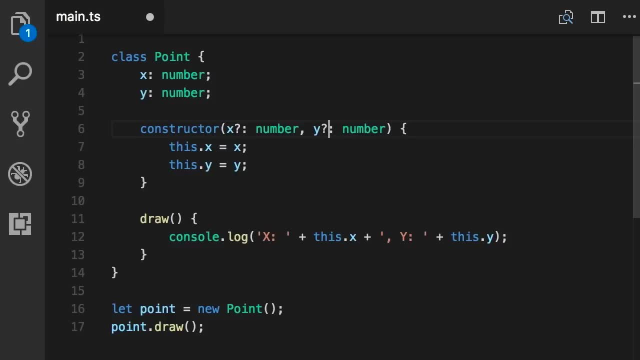 This is a rule by typescript and a lot of other program languages. So now, look, we don't have a compilation error when creating a point object without initial values. Alright, so here I've created a point object with an initial coordinate. Now what if, in our program, you want to have this rule such that 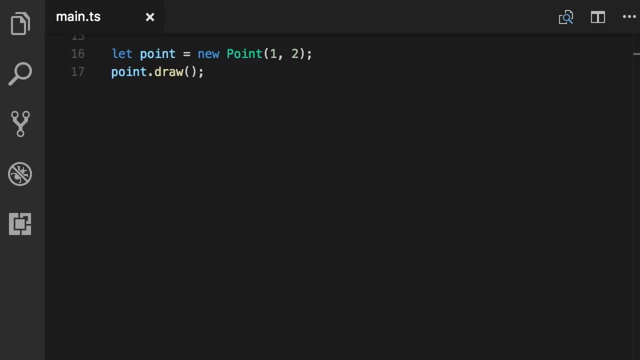 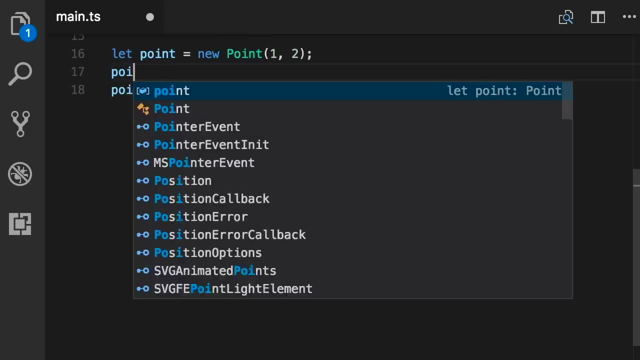 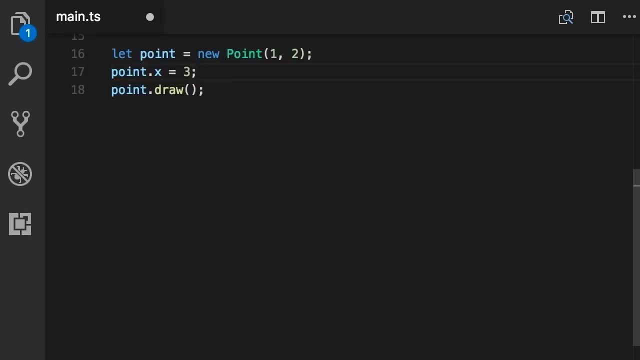 when we initialize a point object, we should not be able to change the x or y values. With this implementation, I can always come here and set pointx to a different value. How can we avoid this? Sometimes we need this feature in our programs because it will make them more predictable. It. 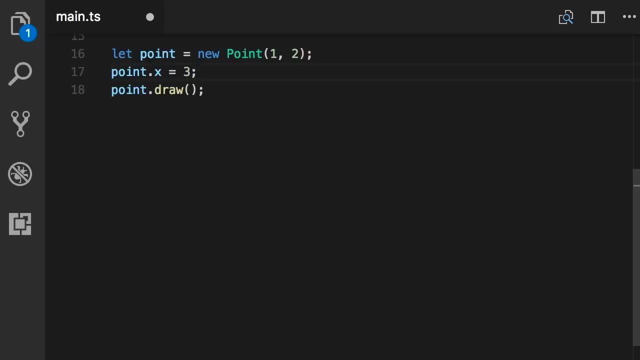 reduces the chance for bugs. So how should we prevent the coordinate of this point object to change after it's initialized? Well, in object oriented languages we have this concept called access modifiers. An access modifier is basically a keyword that we can apply to a member of a class to control. 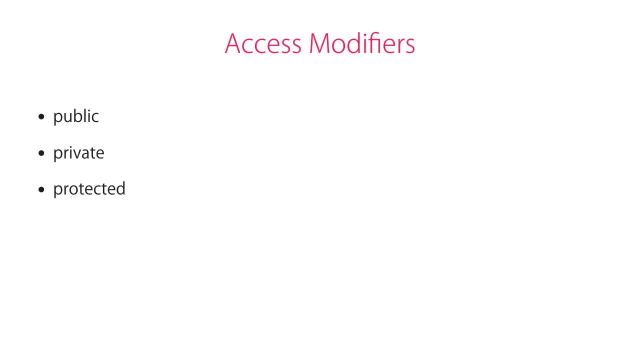 its access from the outside. So in typescript we have three access modifiers: public, private and protected. Public and private are the most common And by default all members are public. Let me show you what I mean, So here. 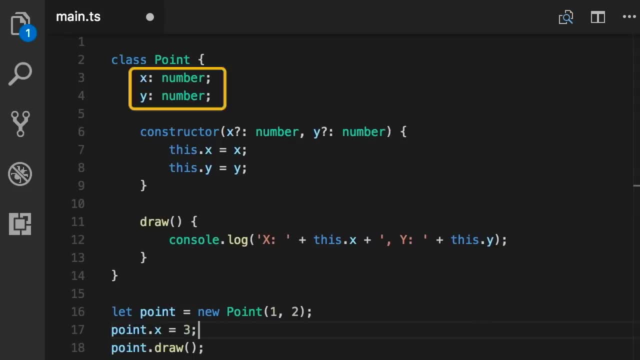 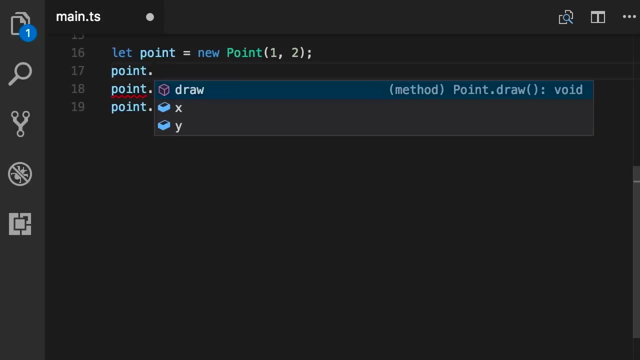 in our point class we have three members right, We have two fields and one method. So when we create a point, object and type pointlook, these are the members of the class and because they are all public, we can access them here And that's why we can see them in the IntelliSense. 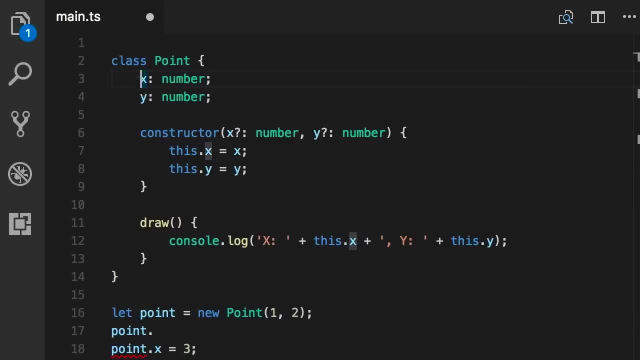 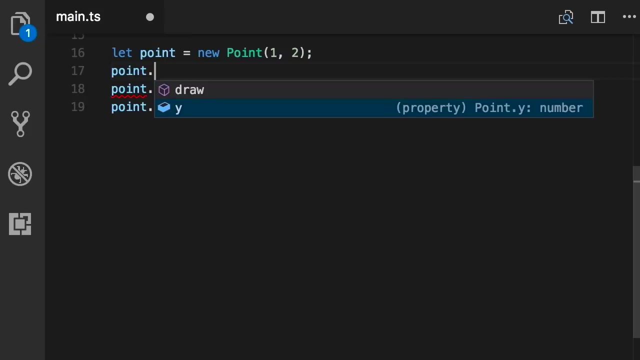 However, I can go here and prefix this field with the private keyword. Now, once we create this point object, if I type pointlook, x is not in the list, It's not accessible, It's private. So if we try to set, 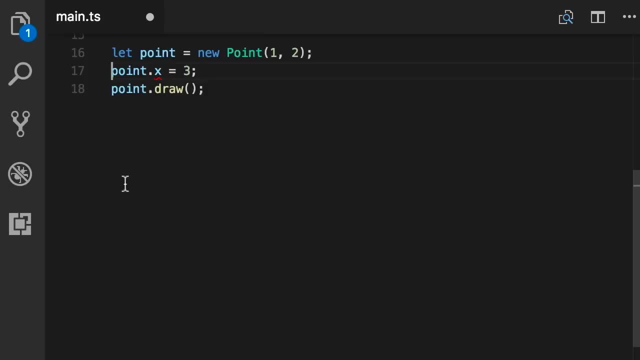 pointx to 3,. look, we have a compilation error in typescript. It says property x is private and only accessible within class point. Now, with this technique, I can go here and I apply the private keyword on the y field as well. And now, 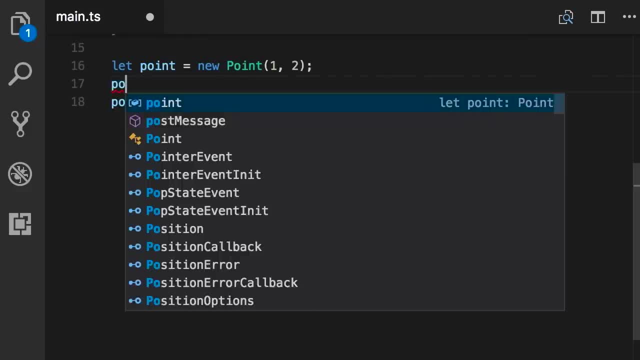 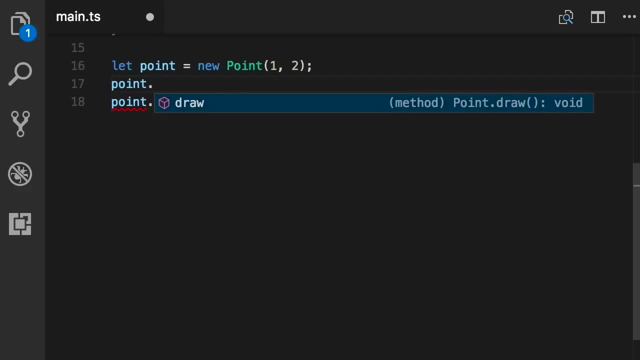 once I initialize a point object, I can no longer change its coordinates. I can only call the draw method: Okay. So this is why we use access modifiers To control access to certain members of a class from the outside. You can apply these access modifiers on fields, properties and methods. 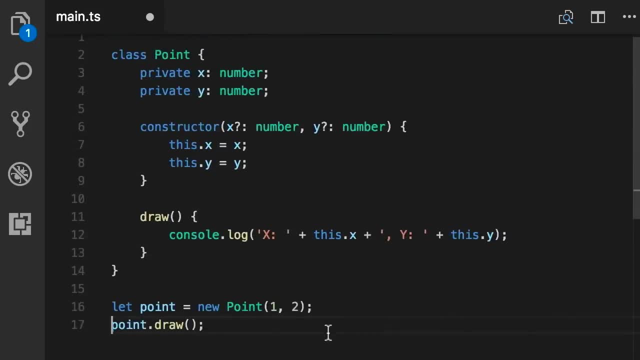 Now by default, if you don't set an access modifier, it's assumed to be public. So here the draw method, as you know, is public. I can also add the public keyword here, but this is redundant. It's just making my code noisy. 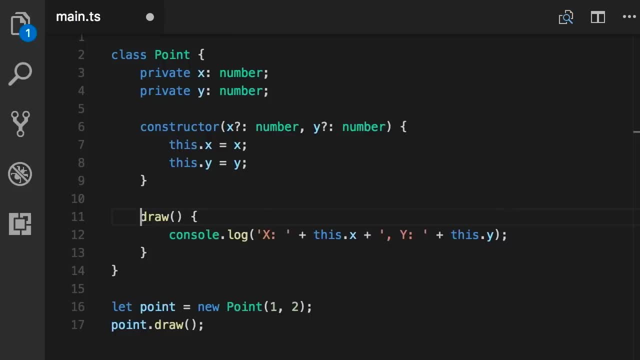 So you don't really need to add this. It's better to keep your code short and clean and use the private access modifier only when you need to. Next, I'm going to show you one of my favorite features of typescript around access modifiers. 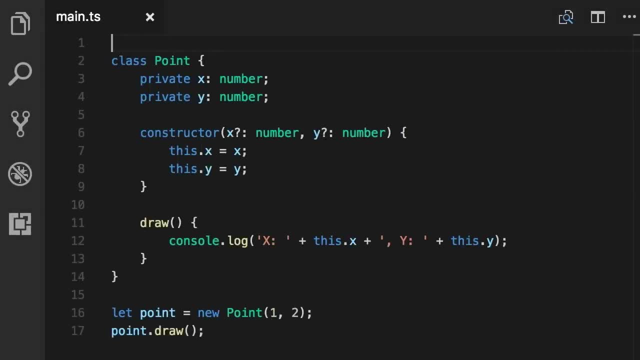 As you write code with typescript, you see constructors that follow a pattern like what you see here. So here we have two parameters in our constructor and we use these two parameters to initialize the fields in this class. The code looks a little bit redundant. This dot x. 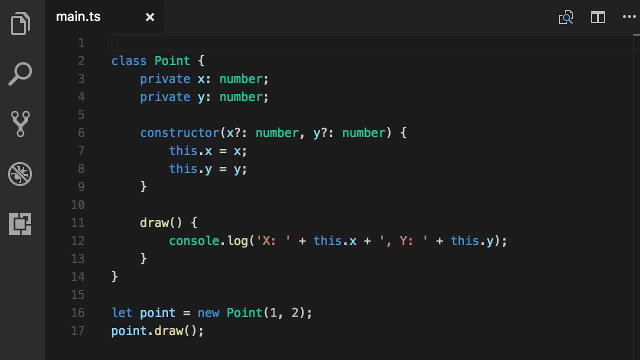 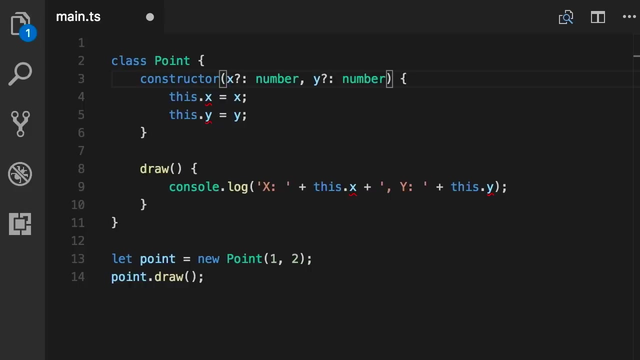 equals x and this dot y equals y. Typescript has a fantastic feature that helps you achieve the same thing with less code. So here we can delete these two fields here, and in our constructor we can prefix our parameters with an access modifier. So here I want to. 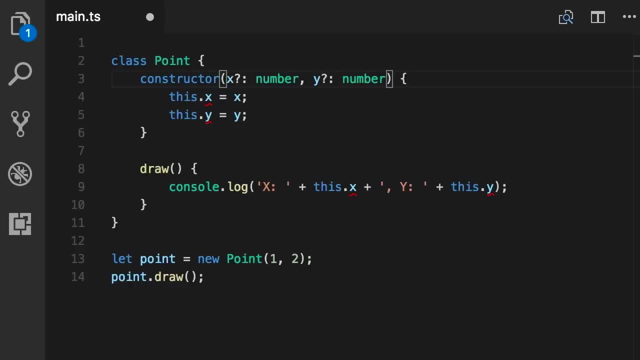 have two private fields, x and y. I can simply prefix these with the private keyword like this. So typescript compiler will generate these fields for us, And also you don't need these ugly repetitive assignments either. So if we prefix a constructor parameter with an, 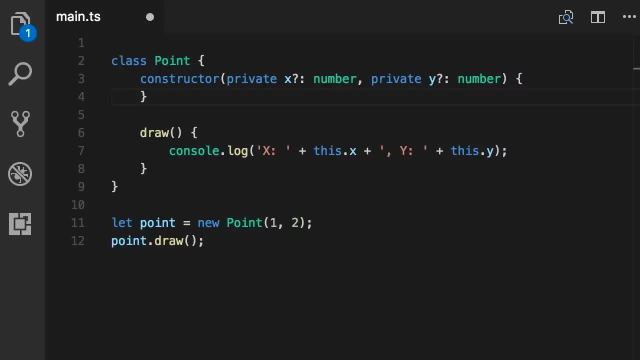 access modifier, whether private or public, typescript compiler will generate a field with the exact same name and it will also initialize that field with the value of this argument. It's one of my favorite features and you're going to see that a lot in this course. 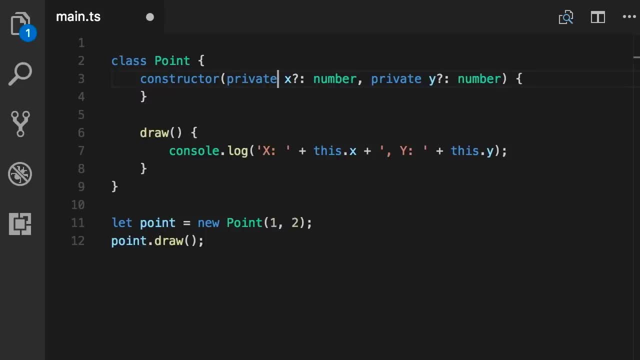 Now I'll clarify something before I finish this lecture. In this case our fields were private, but if they were public we would use the public keyword here. So this means when we create a point object, we can access the x field. 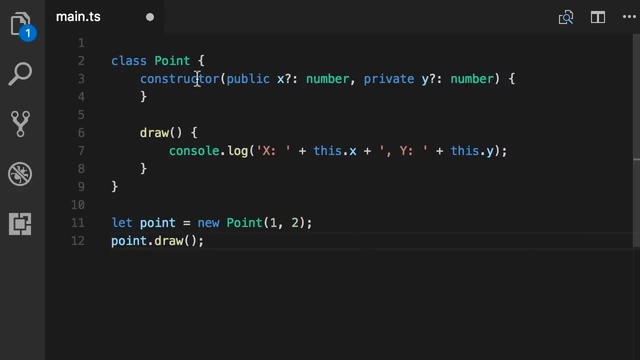 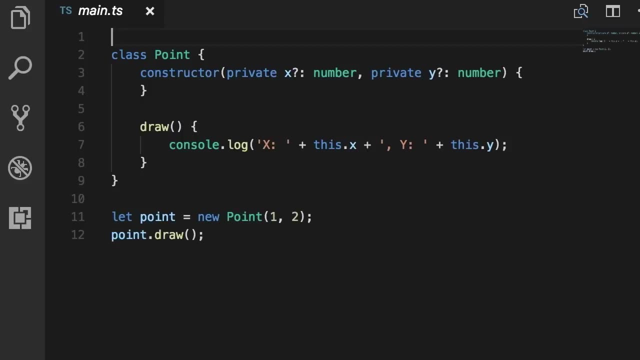 Okay, So I'm going to revert this back to the private. Alright, now. this implementation has a tiny problem. We can set the initial coordinate of this point and we can also draw it, but there is no way for us to read. 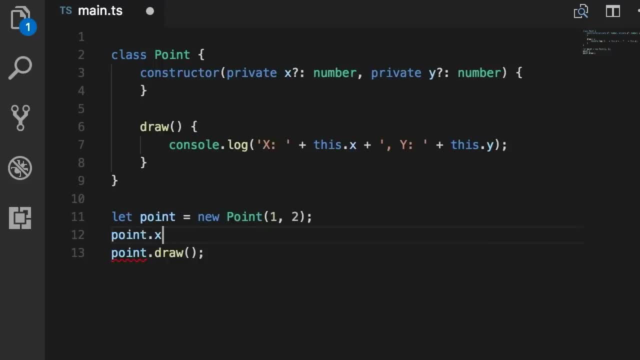 the coordinate. So I cannot access pointx here to display to the user What's the workaround. Well, one simple solution is to define a method like this: Get x, and here we simply return thisx, Because in this class we do have access to all the private members of this class. 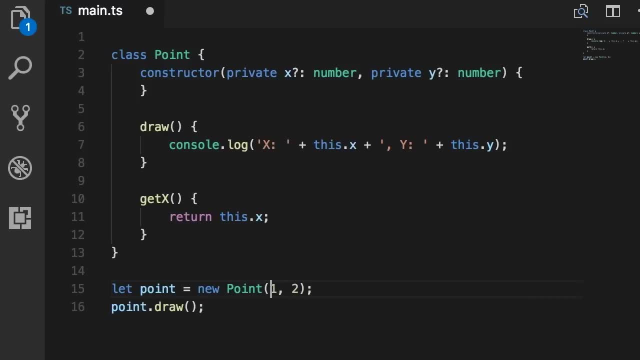 but we cannot access them from the outside. Okay, Now here I can always call pointgetx to get the x value and display it to the user. Now let's talk about another use case. Maybe we want to give the user the ability to set the initial coordinate here, but we also 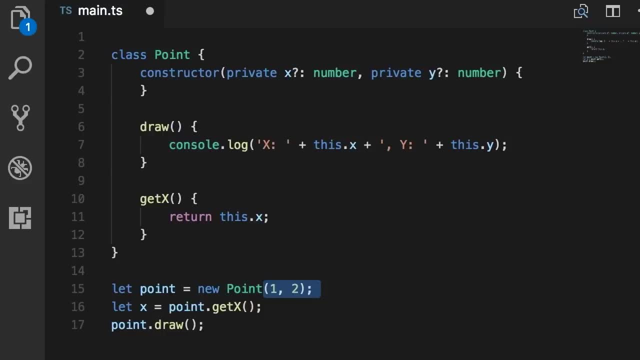 want them to be able to change this coordinate later, only if they provide a value within a given range. What do I mean by that? Let me show you. I'm going to define another method here. set x. now this method is going to get a value. 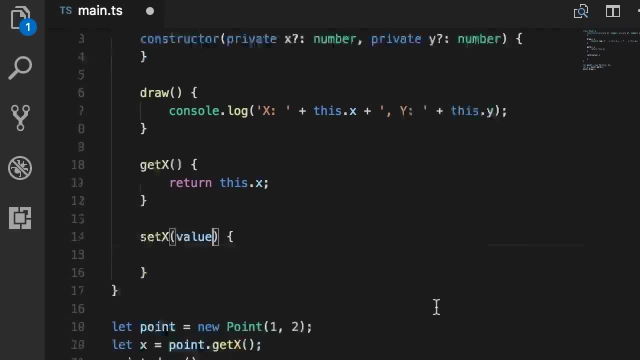 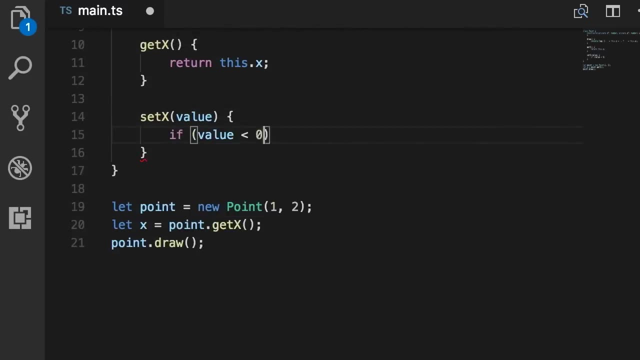 That's the new value for the x field. Let me scroll down Now. here first we can do some basic validation. So if value is less than 0, we want to throw an error, Throw new error. Value cannot be less than 0.. 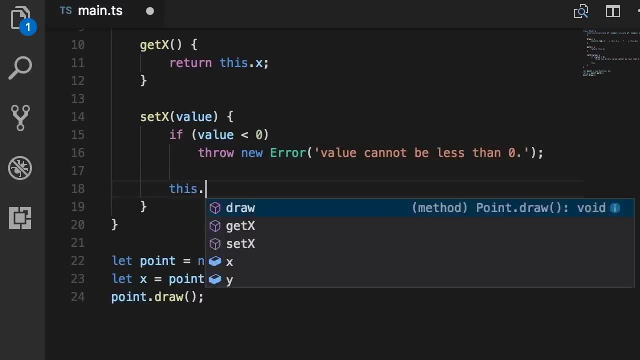 Otherwise, we want to set this, the x, to this new value. Okay, Now, with this implementation, we can always change the value of the x field, like this pointsetx. we set it to a new value. Now, if you have a use case, 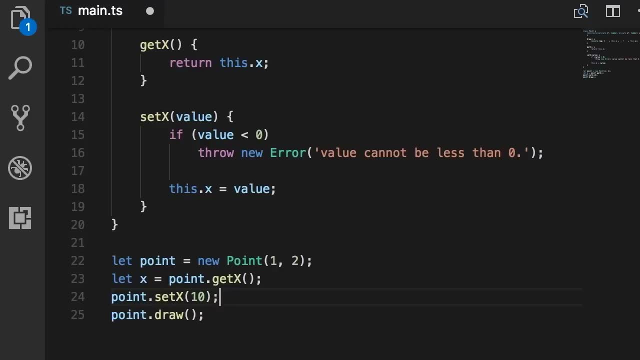 like that. in your applications you can use what we call a property. So in typescript and in a lot of object oriented programming languages we have a concept called property, which is exactly for this very use case. So look at how I can define. 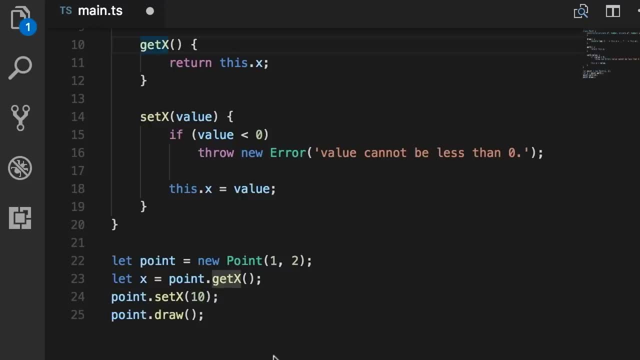 a property. here We start with a keyword, which is get or set, and then the name of the property, which is, in this case, x, and after that we're going to have parenthesis, just like a method. Okay, Now, similarly, I'm going to change this to: 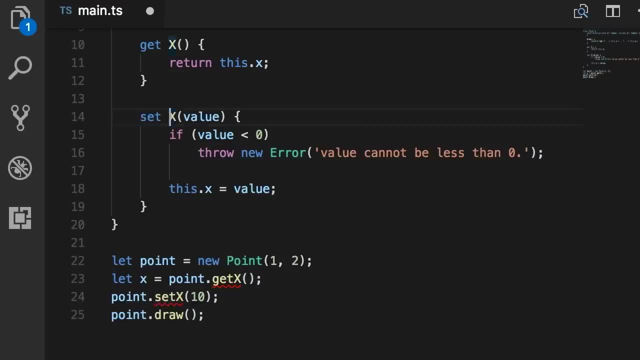 set with a space. so we have the set keyword and here it's like we have a function, a method. Now what is the difference? The difference is that we can use these properties like fields. So here I can read x like this: 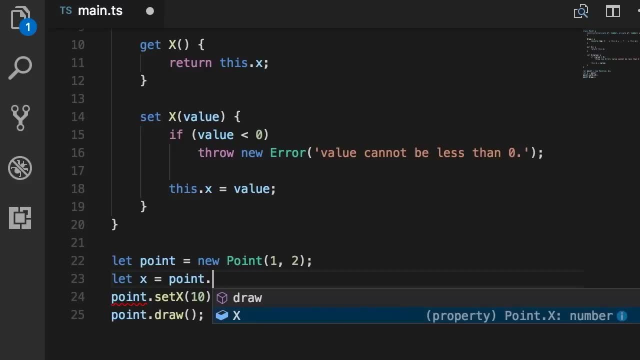 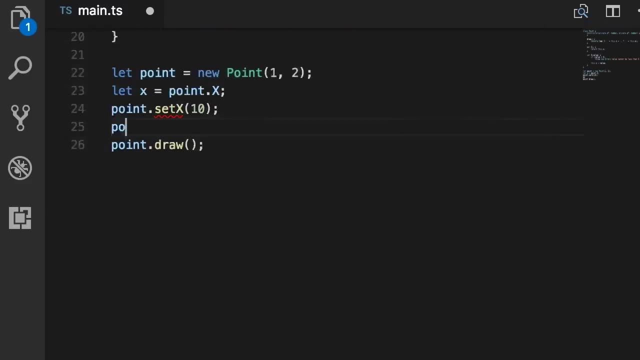 dot. note the icon of x. it's the same icon we have for fields. it's not a method anymore, So we can read x and we can also set it like this: pointx. we set it to 10.. We don't have to call. 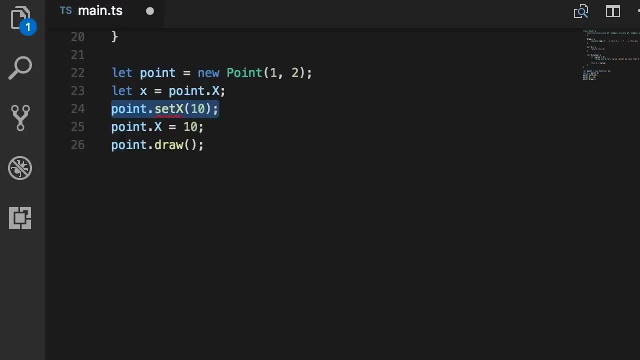 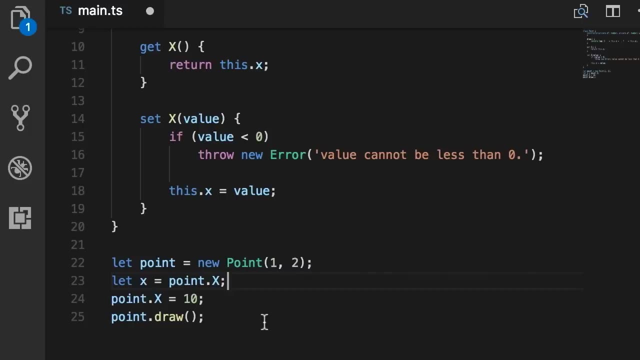 a method like this. it's a cleaner syntax. Okay, So this is what properties are for. If you have private fields, then you want to give- maybe a read only- access to the outside, or if you want to give the consumer of your classes the ability. 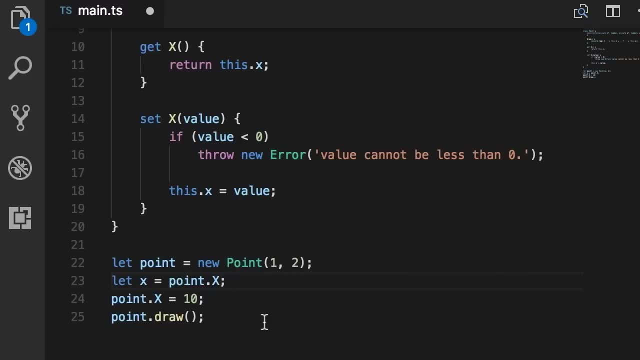 to set the values, but you want to have some basic validation. that's when you use a property. Now, in this case, if I want to give only the read, only access to this underlying field, I can simply comment out the setter. So we call this method a. 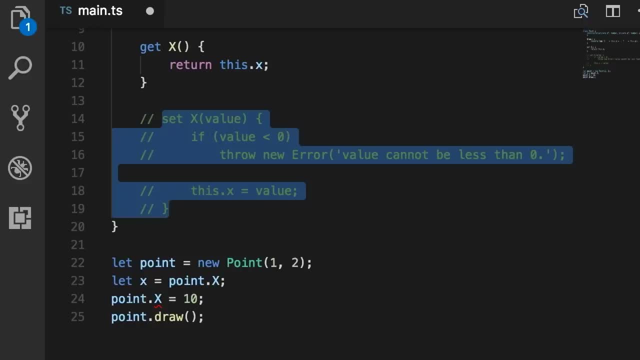 setter and the other method a getter. Okay, And now look at this compilation error. we cannot change the value of x. Now let's bring this back. one last thing before we finish this lecture. So here I have used a capital x. 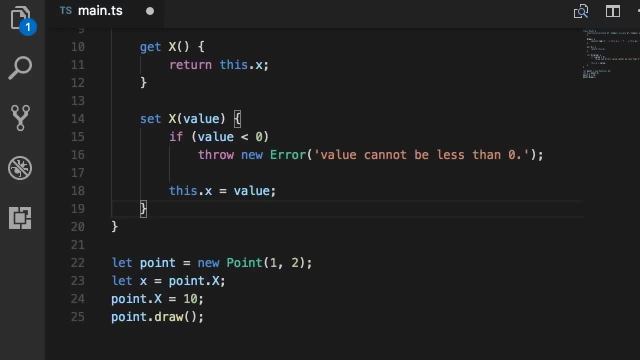 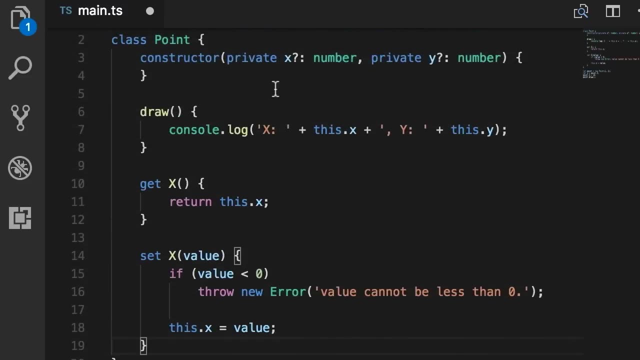 for the name of my x property. In javascript and in typescript we use camel notation to name our field. So that's why earlier we defined this private field here using camel casing notation. Camel casing means the first letter of the first word is lower case. 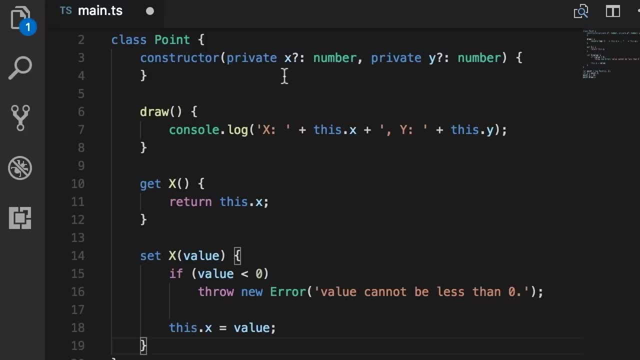 And the first letter of every word after is upper case. Now what should we do to use camel casing notation for our properties? If I name this, the lower case x, it clashes with the existing field. So let me revert this back a convention we use to solve this problem. 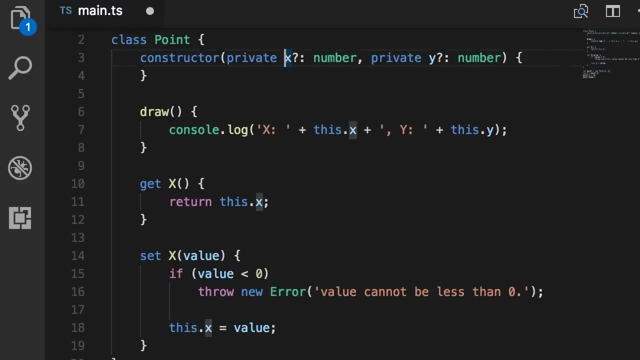 is to prefix the name of the underlying field with an underline. So let's rename this using f2, and prefix it with an underline. Okay, Similarly, for the y parameter or the y field, I'm also going to use underline y. Then we can rename this. 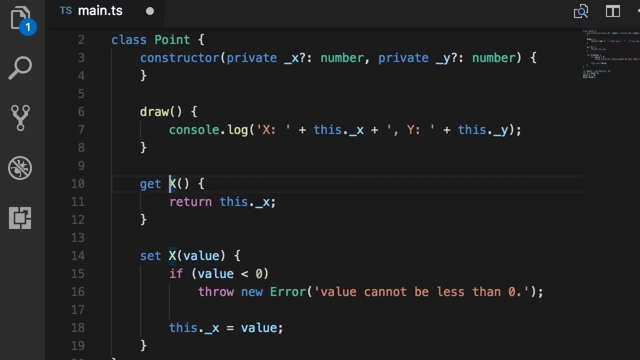 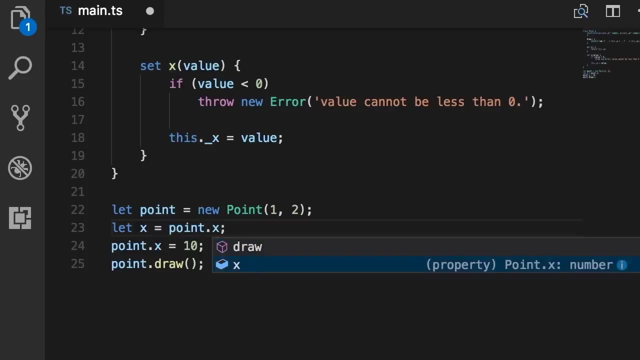 property from capital x to lower case x. Once again, we press f2, lower case x and note that both instances, both the getter and the setter, are updated. Now we can work with this x property exactly the same way. we used the x field. 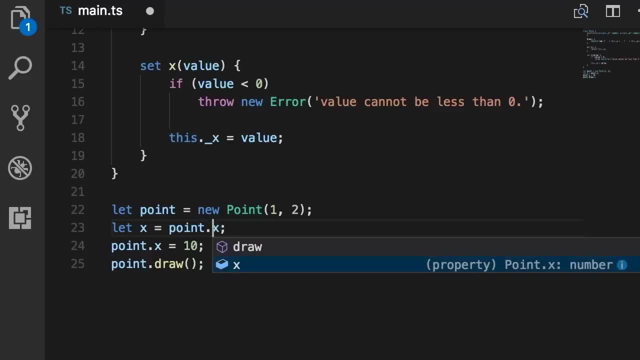 So here's the lesson: A property looks like a field from the outside, but internally it's really a method in the class. Well, more accurately, it's either one method, which is a getter or a setter, or a combination of a getter and a setter. 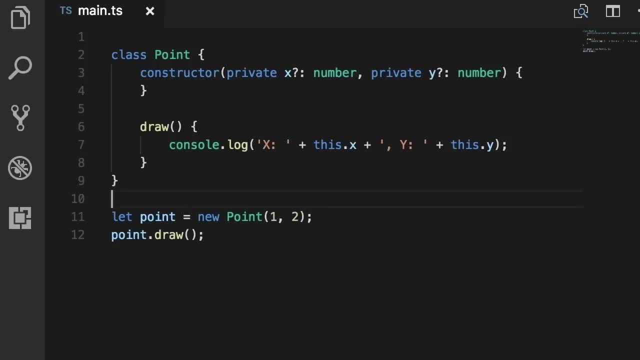 Alright, I've simplified the definition of the point class. I removed the properties, so we have a simple constructor and the draw method And we're using this point class below its definition. Now this is a very simple program with only one file, but the real world application consists of. 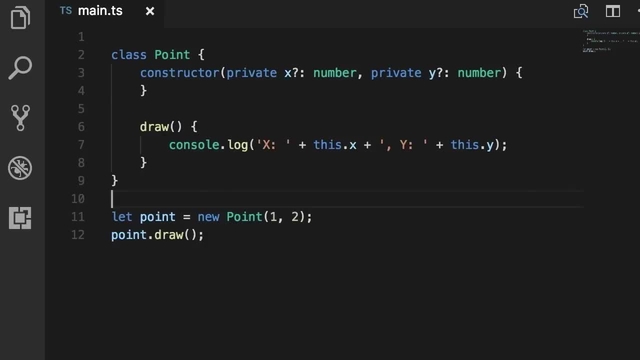 tens or hundreds of files. We don't want to write all the code in one file like maints. So ideally I want to move the definition of this point class somewhere else in a file like pointts. So here in this project I'm going to add a new. 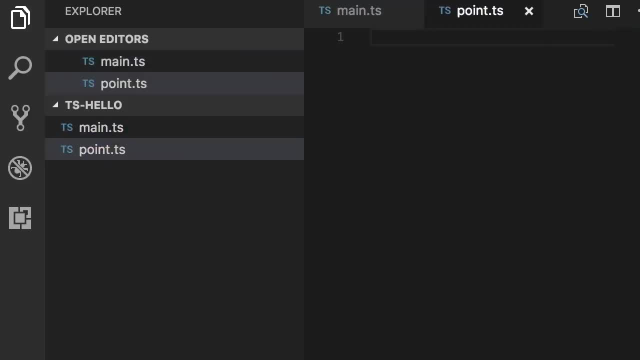 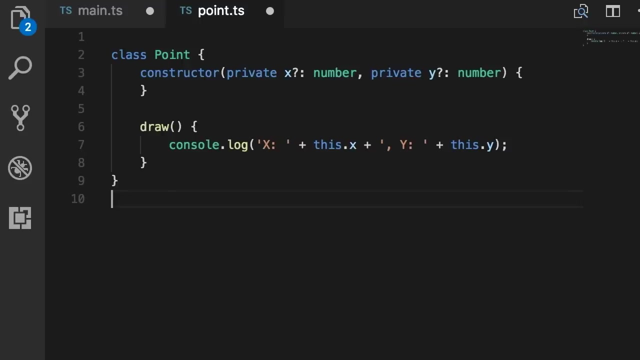 file pointts. now back in maints. I'm going to select all this code, cut it and move it to pointts. Now in typescript we have this concept called modules. Now, what a module is requires a little bit. 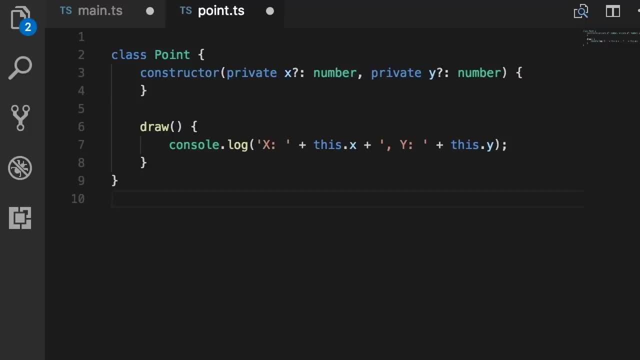 more explanation, but for now let me give you a simple pragmatic definition. In typescript you can think of each file as a module. So in this program we can say we have two modules. But this is not quite accurate because these files are not. 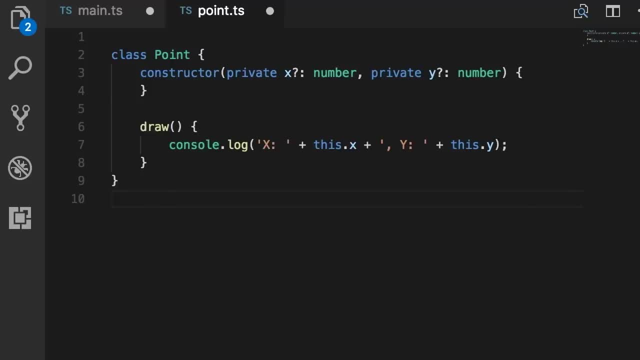 modules yet. So in pointts we have defined this class called point, but this is not accessible anywhere outside this file, So this file defines its own scope. In order for us to use this class somewhere else in our program, we need to export this to the. 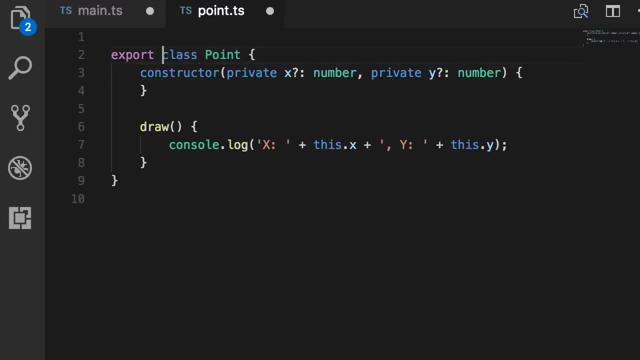 outside. So we add the export keyword here and now this is visible outside this file. Now that we are exporting something on top of this file, from typescripts point of view, this file is a module. Now we need to go back to our maints. 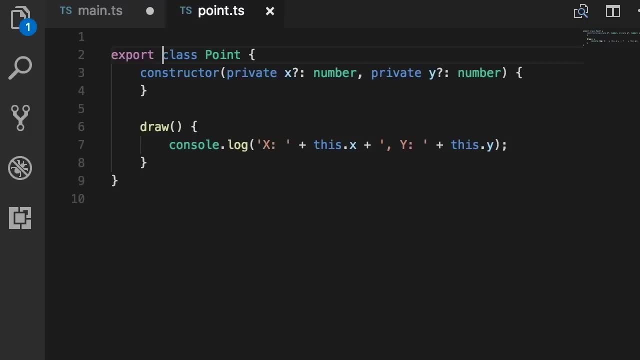 and import this class so we can use it. So back in maints, look, we have a compilation error: cannot find name point because we have not imported this into maints. So on the top we write import. in curly braces we add the name of the types we want to import, in this case 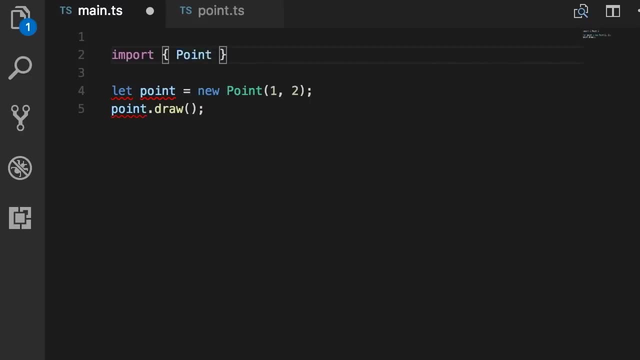 point Now. if there are multiple types we want to import, we separate them using comma. So we import, point from now. here we put the name of the module in quotes. What is the name of the module? It's the relative path to that module. 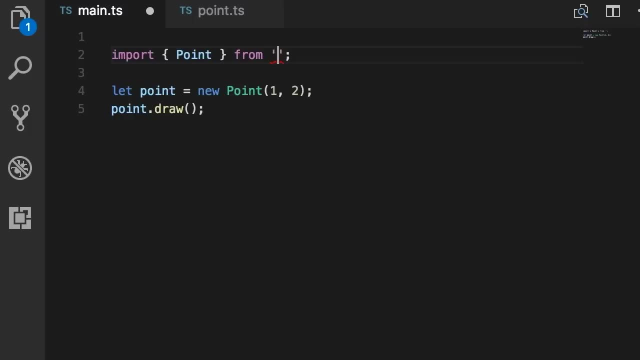 from this file. So both these files are in the same folder. we can use period slash, which refers to the current folder, and then point is the name of our module. So it's not pointts. Look, we get a compilation error. 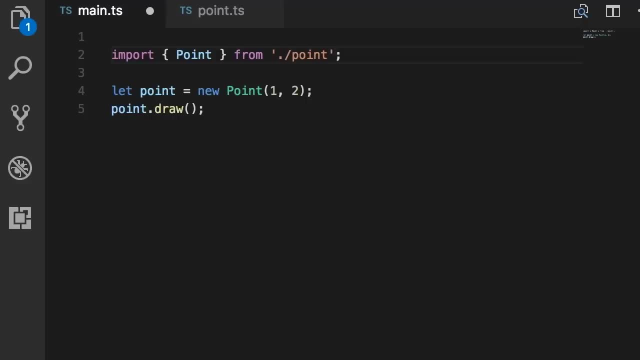 So the name of our module is point. Now we no longer have a compilation error here and we can create an instance of this point class and use it Now. there is a lot more to talk about when it comes to modularity in typescript, but that's all you need to know. 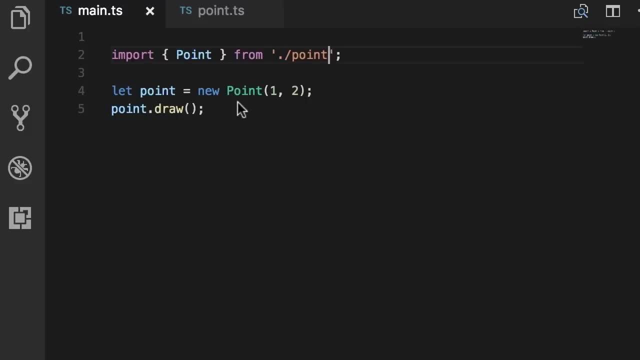 for now, in order to start building applications with angular, Because in angular framework we have a lot of types that are exported, so we need to import these into our typescript files and use them. You're going to see that a lot in this course. The only difference. 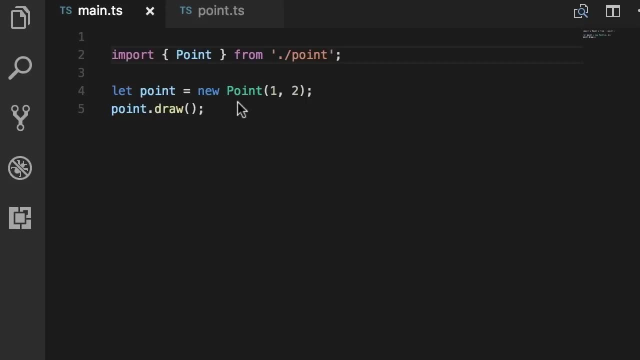 is that angular modules are defined in a different way. so we don't add the relative path to these module files, because these files are not really part of our application. They're somewhere inside node underline modules folder. So when it comes to importing types defined in angular, we use the library name as the. 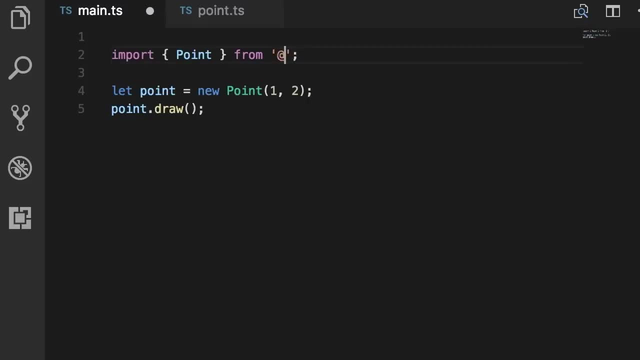 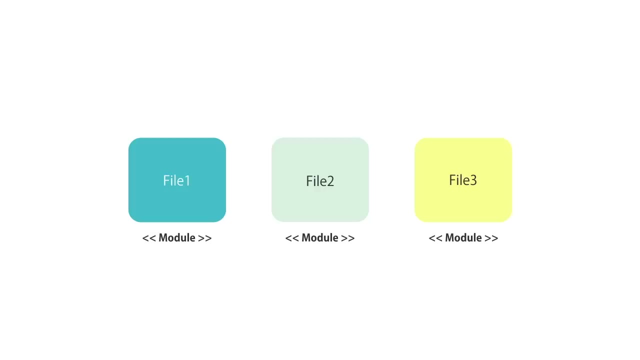 module name. For example, one of the libraries is at angular slash core. Okay, So here's the lesson In typescript. we divide our program into multiple files. In each file, we export one or more types. These types can be classes, functions. 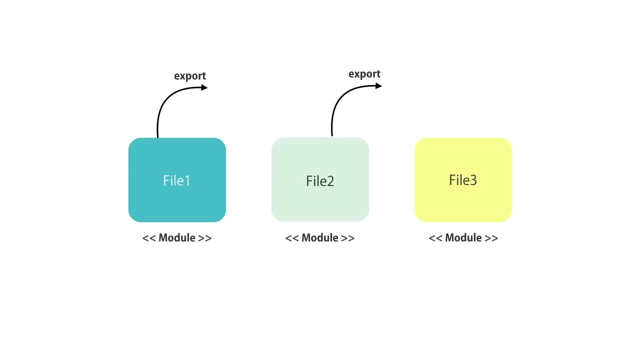 simple variables or objects, And wherever we need to use these types, we need to import them first. When we have an import or export statement on top of a file, that file is a module from typescript's point of view. In angular we also have the concept. 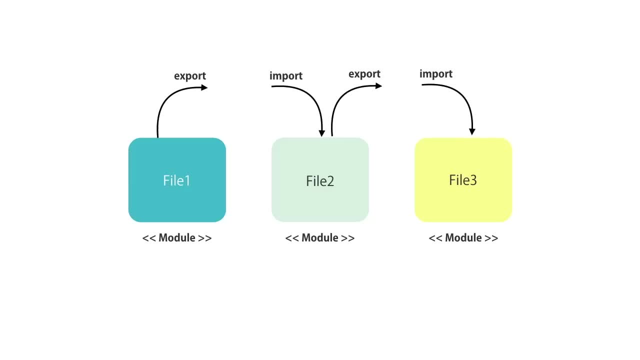 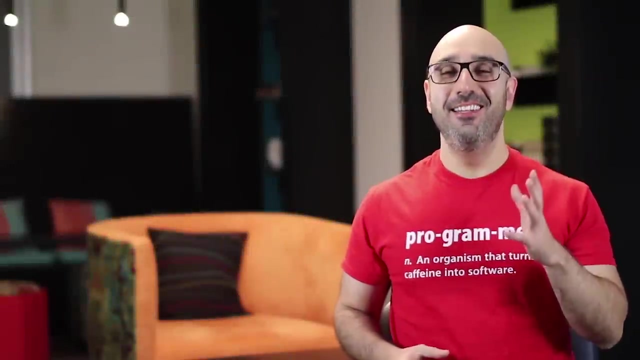 of modules, but angular modules are a little bit different. They're not about organization of code in different files. they are about organization of your application into smaller functional areas. You're going to learn about angular modules in the next section. I love your enthusiasm for learning angular. 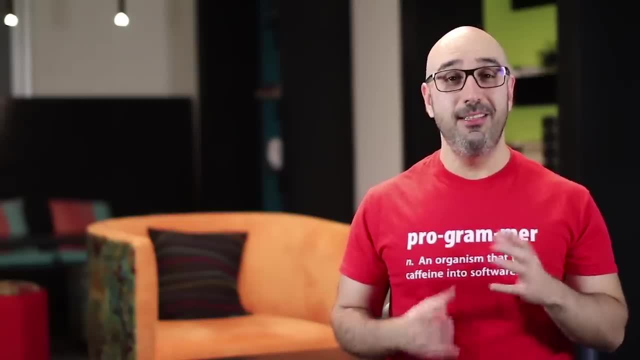 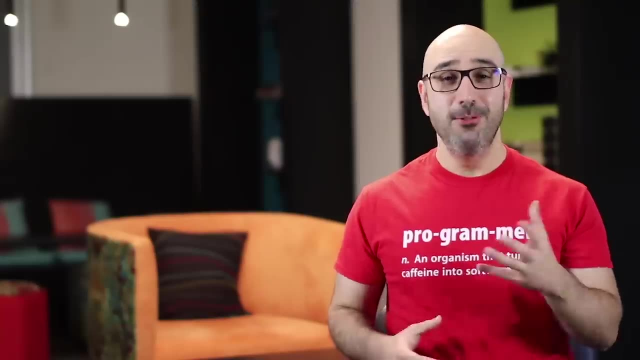 As I told you before, this tutorial is part of my complete angular course, where you will learn everything about angular, from the basic to the advanced topics, all in one course. You seem to be determined enough to learn angular and I'm so excited to see you made it this far, So I highly 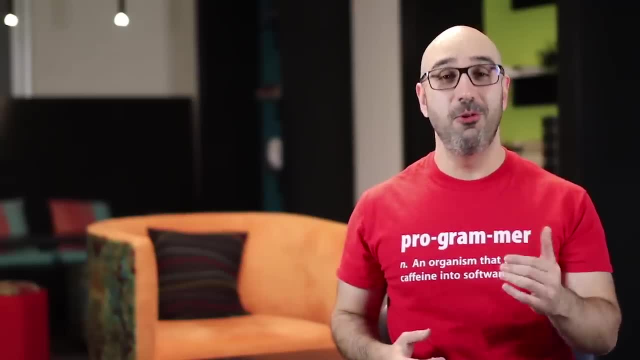 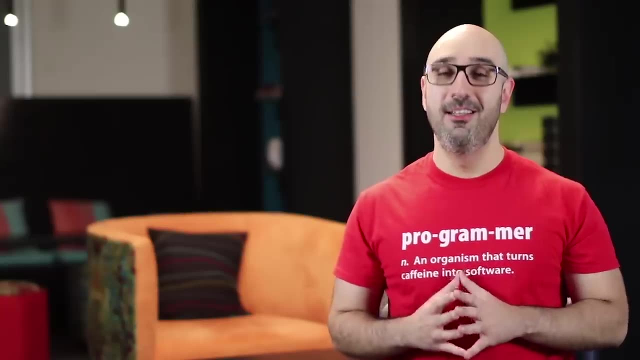 recommend you to click on the link in the video description and enroll in my complete angular course. So thank you for watching. If you enjoyed this video, please like it and share it with others And, finally, subscribe to my channel for free new videos every week. Have a great day. 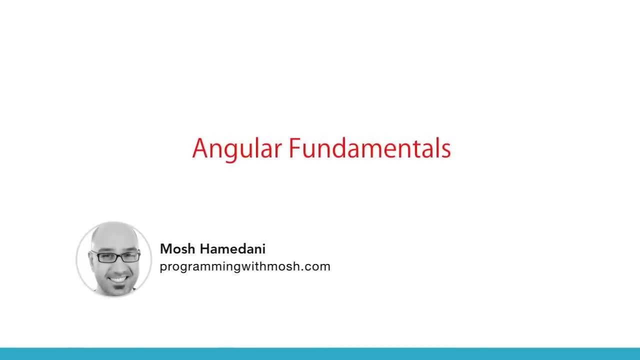 In this section, we're going to look at the fundamentals of building applications with angular. By the end of this section, you will have a basic understanding of angular building blocks, such as components, templates, direct objectives and services. So now let's get started. 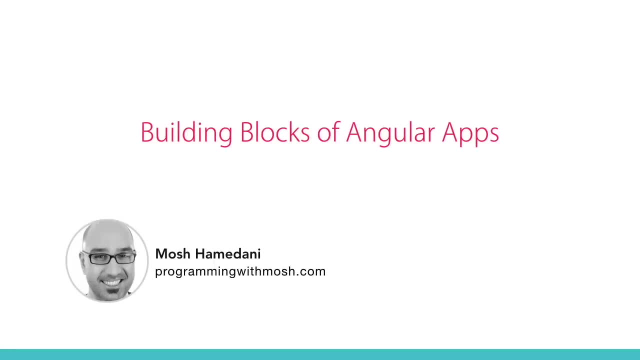 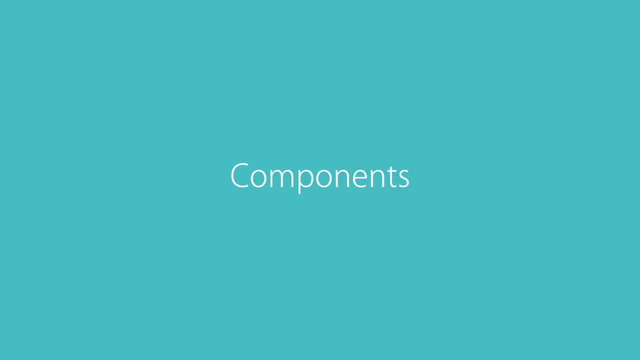 So now that you have some basic familiarity with angular, let's look at the building blocks of angular apps. At the heart of every angular app, we have one or more components. In fact, in a real world app, we have tens or hundreds of components, But what is a component? 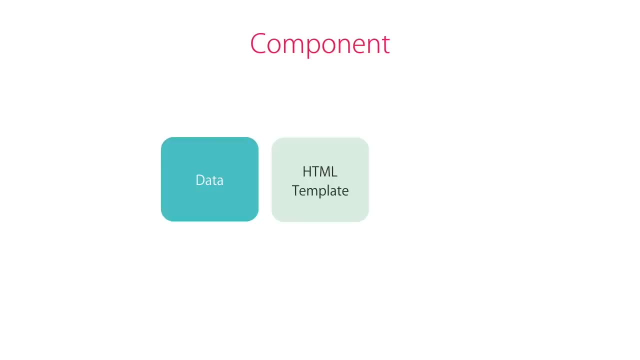 A component encapsulates the data, the HTML markup and the logic for a view, which is the area of the screen that the user sees. Let's look at a real world example. Imagine we're going to build a website like udemy, So on this page we 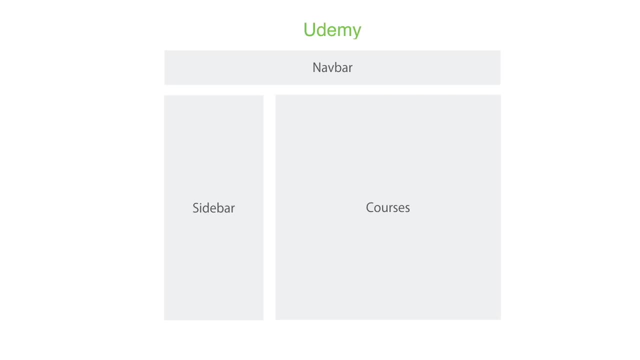 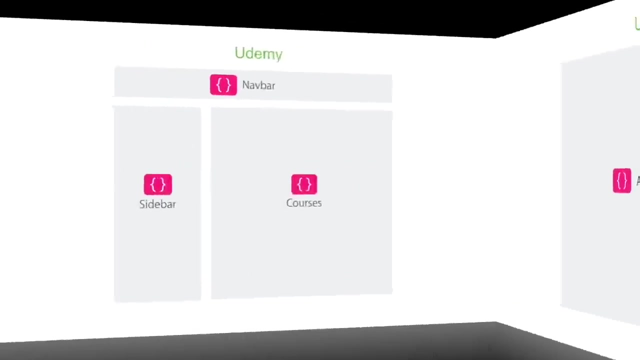 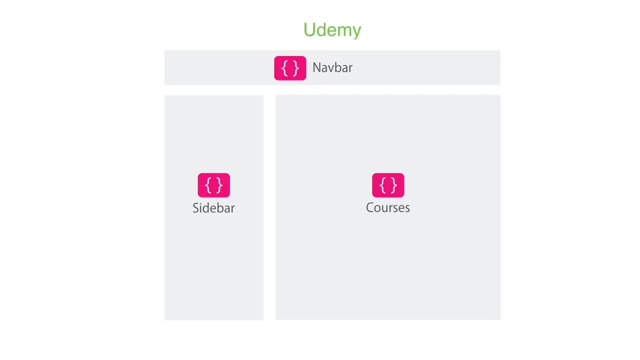 have a navigation bar, a sidebar and an area to display the list of courses. Now we can think of all this as one view or one component, or we can break this view into smaller, more maintainable and potentially reusable components. 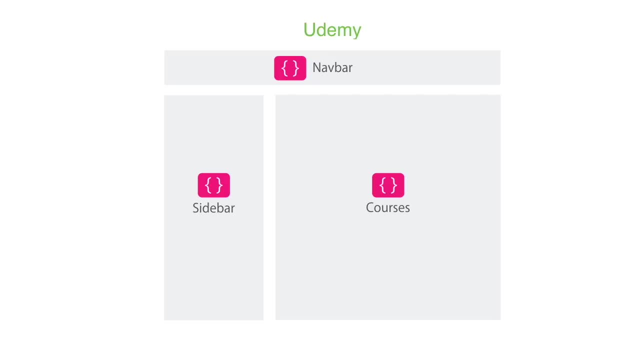 Like navbar component, sidebar component and courses component. Similarly, in courses component we want to display one or more courses. Potentially, we can break up this component into smaller components And also to take this to the next level, each course component can include a rating component. 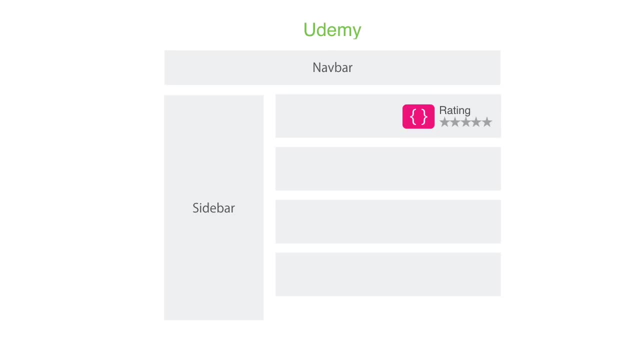 Now we can reuse this rating component in multiple places in the same app or in an entirely different app. As you see, Angular embraces component based architecture, which allows us to work on smaller and more maintainable pieces that can also be reused in different places. So, once again, 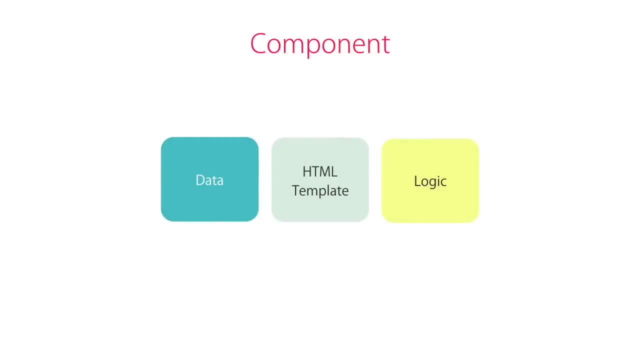 a component encapsulates the data, the HTML, markup and the logic for a view, which is an area of the screen that the user sees. Every application has at least one component, which we call app component or root component. A real world Angular app. 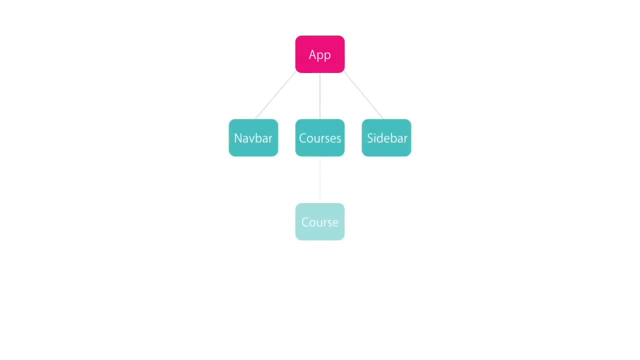 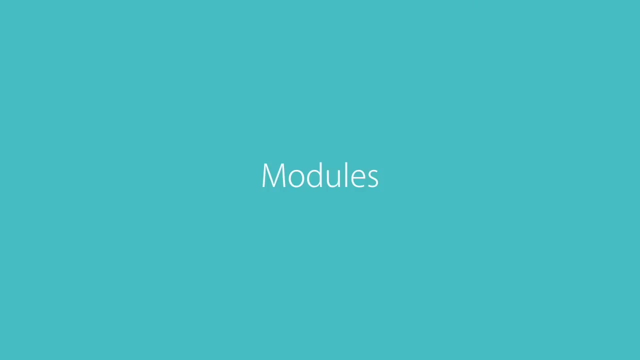 is essentially a tree of components, starting from the app component or the root component. Now in Angular we also have another concept called modules. A module is a container for a group of related components. Every Angular app has at least one module, which we call app module. 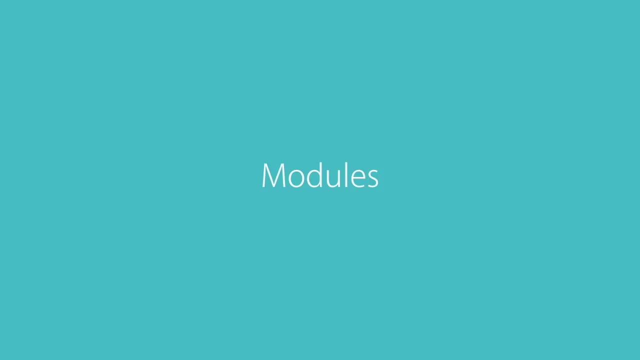 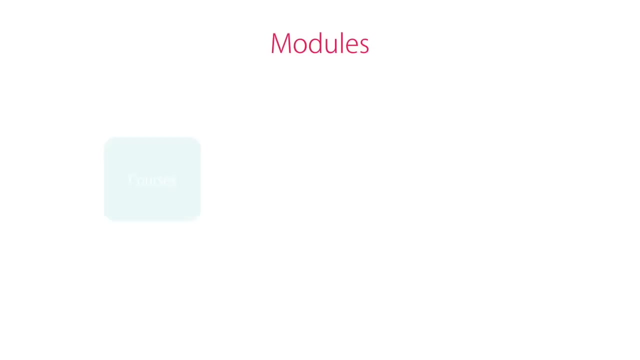 As your application grows, you may want to break that module into smaller, more maintainable modules. So in our Udemy example, we can potentially have modules like course module, which includes all the components for displaying courses. We can potentially have another module like messaging module, which includes a bunch. 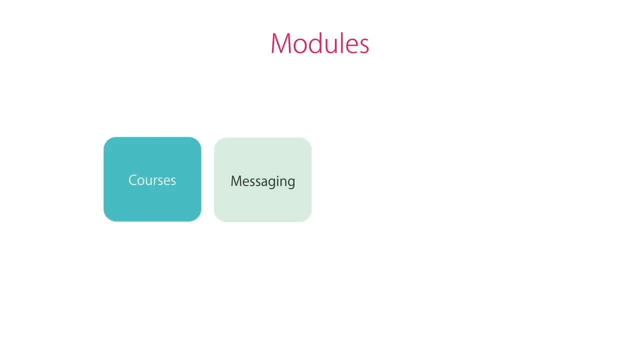 of components for the area of the website where you can send private messages to your instructors. We can have an instructor module, which includes the components for instructor's dashboard that you don't see, and potentially admin module, which is the area of the Udemy website. 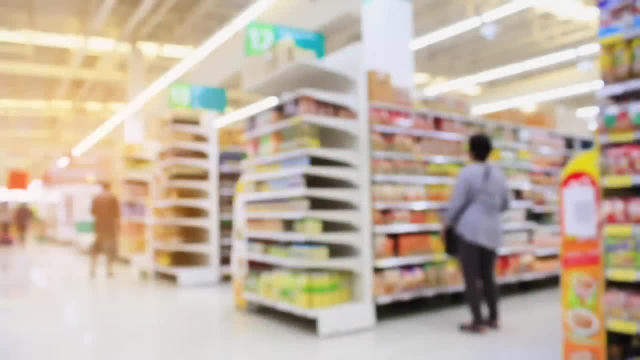 managed by the Udemy staff. As an analogy, think of a supermarket. In a supermarket, we have different aisles for different products. We have a section for fruits and vegetables, we have another section for snacks, another for hardware and so on. 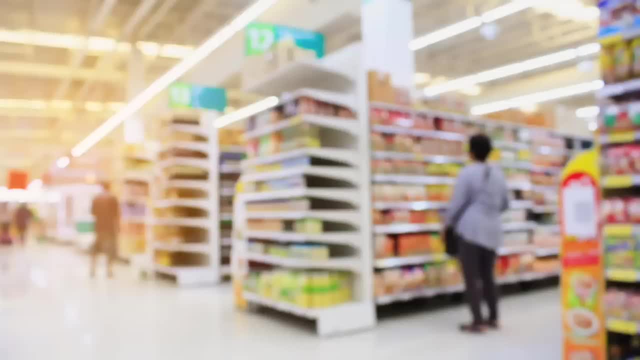 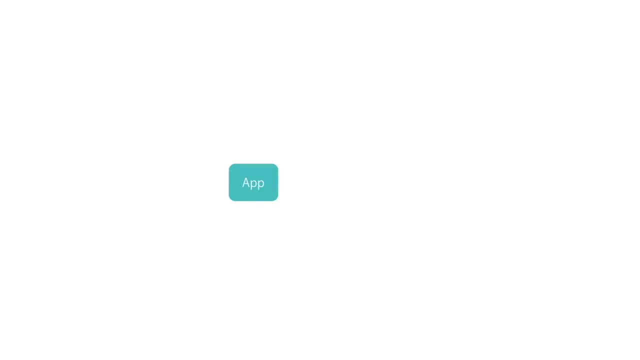 The bigger the supermarket, the more aisles we have. In a tiny grocery store, we have probably one or two aisles at the most. The same applies to our Angular apps. So if you're building a simple application, we have only one module which we call. 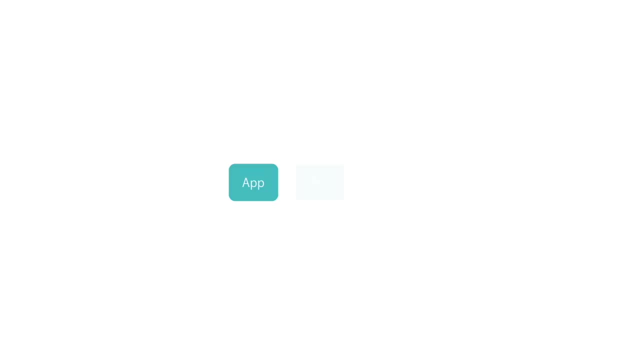 the app module. But as our application grows in functionality, we may need to break that module into smaller modules, with each module responsible for a specific area of our application. In that module we have a bunch of related components. okay, So this is the big picture. As we go through this course, you will learn. 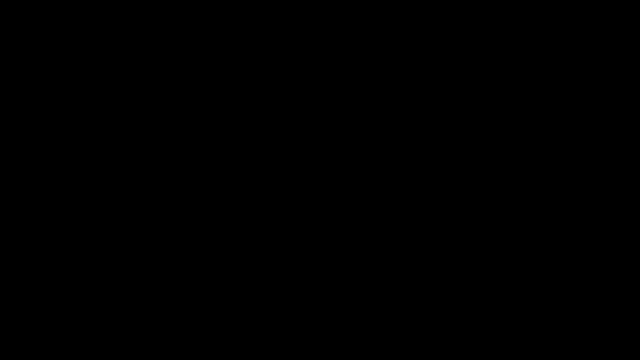 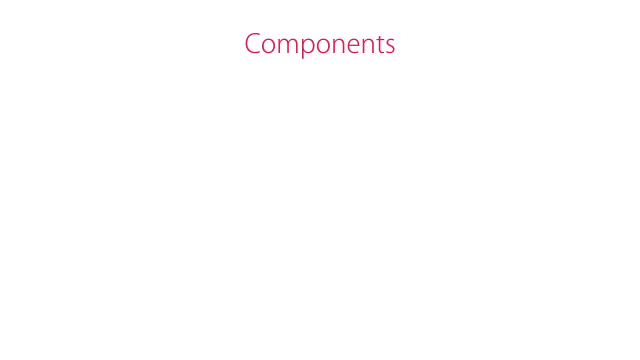 about these building blocks in more detail. Alright, now let's see this course: Components in action. There are basically three steps you need to follow in order to use a component. First, you need to create a component. second, you need to register that component in a module. and third, 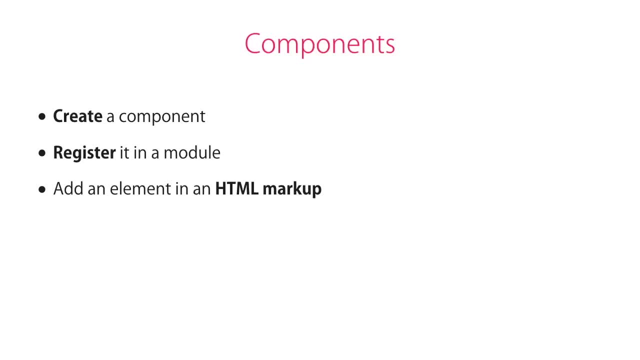 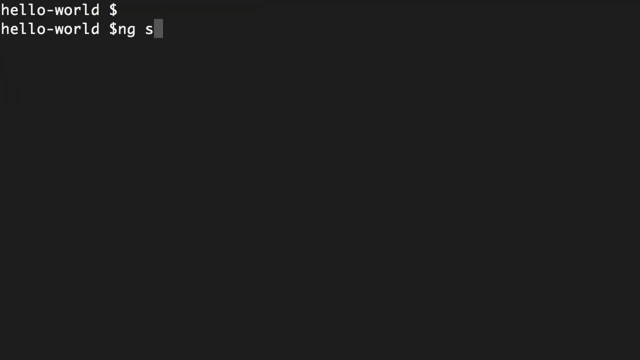 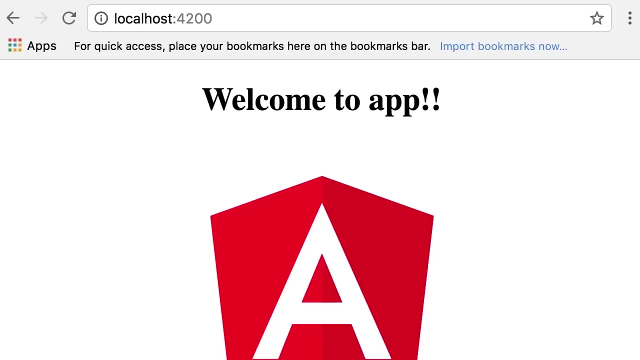 you need to add an element in your HTML markup. Let me show you what I mean by this. So back in our first Angular project. first of all, make sure to run ng serve to serve this application. So now, if you head over to localhost, 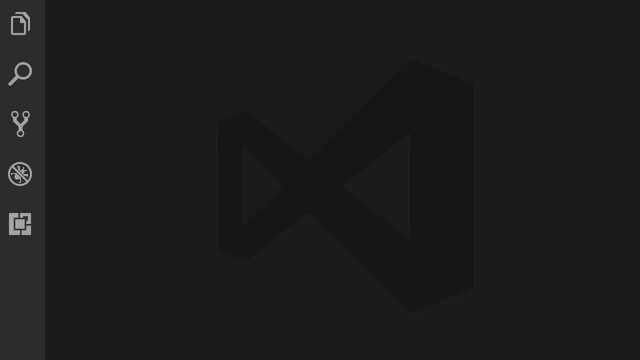 port 4200,. this is what you see, Beautiful. Now, back in VS code, I'm going to create a new component, So let's open up the file panel Here in the source folder under app. here I'm going to add a new file. 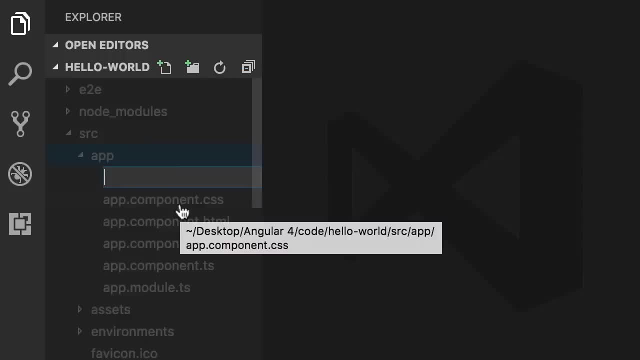 Now let's imagine I want to create a component to display the list of courses. So look how I named this file: Coursescomponentts. This is the convention that we use when building Angular applications. Now, if the name of the component has multiple words, we separate. 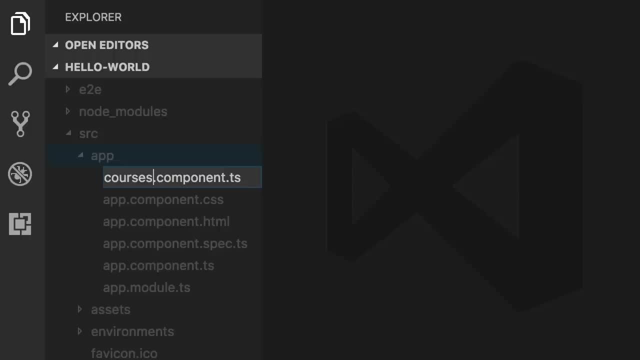 them using a hyphen. For example, if you're building a component called course form, you would call this course-form And then componentts. Okay, So coursescomponentts. Now here we start by creating a plain TypeScript class. 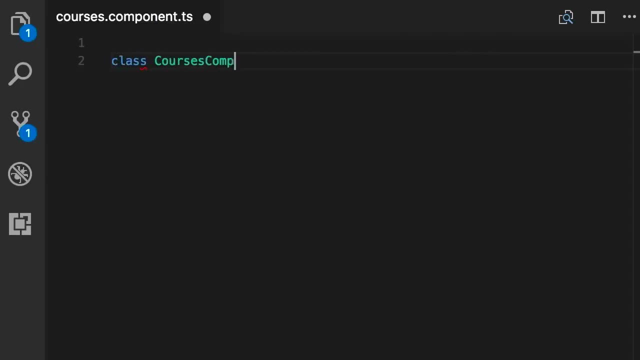 So classcoursescomponent. Once again, look at the naming convention. Here I'm using the Pascal naming convention, So the first letter of every word should be capital, And also by convention we use the suffix component in the name of the class. 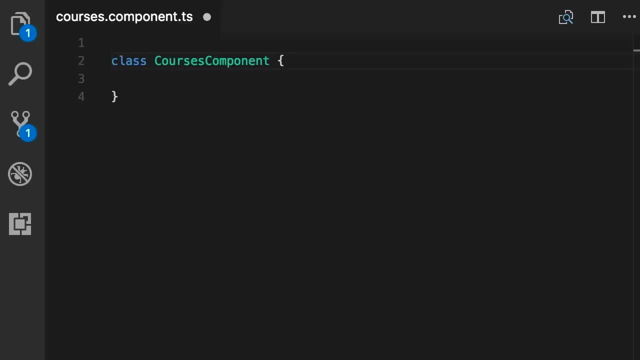 So here's our class. In order for Angular to see this class, first we need to export it. Now, so far, we have only a plain TypeScript class. This is not a component. In order to convert this to a component, we need to add some metadata. 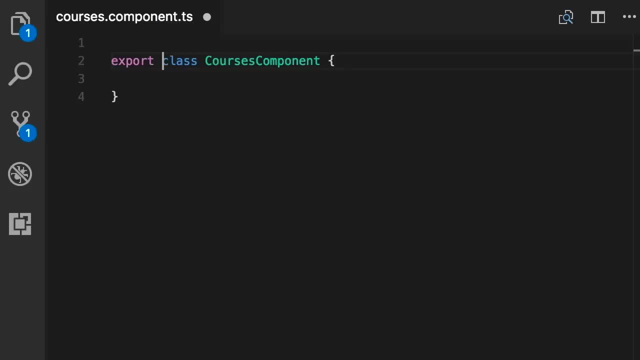 to it that Angular understands We use a decorator to achieve this. In Angular we have a decorator called component that we can attach to a class to make that class a component. So first we need to import this decorator on the top. So import curly braces. 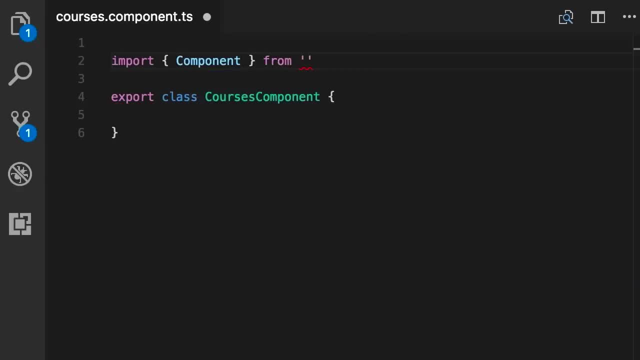 component, from now the name of the library. So at Angular slash core, This is the core library of Angular that you're going to see a lot in this course. So here we import the component decorator and then we need to apply it. 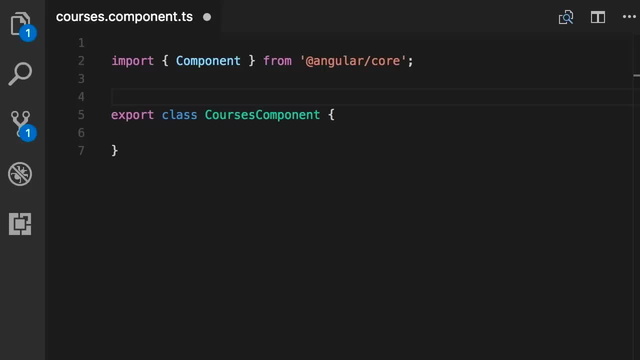 to this TypeScript class. Now look at the syntax We use at sign component and then call this like a function. So this is what we call a decorator function. Now this function, as you see here, takes an argument. So here we pass an object and in this object we add one or more properties. 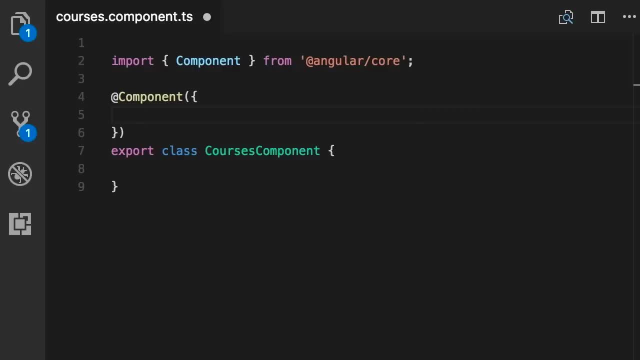 to tell Angular how this component works. For example, one property that we use quite often is selector, So selector, and we set this to a CSS selector. So in CSS, if I want to reference an element like this, I use a selector. 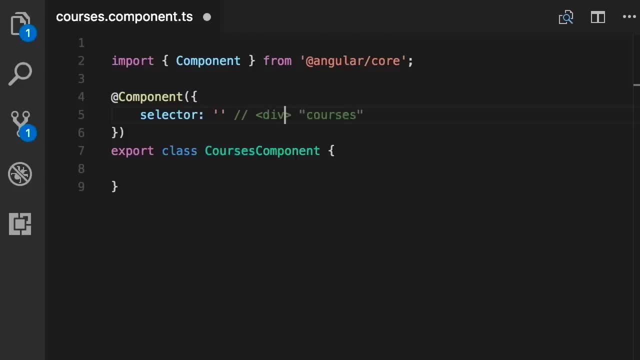 like this: If I want to reference an element like a div that has a class called courses, my selector would be dot courses, And if I want to reference an element with the id courses, this is my selector. Just basic CSS. So here we want to reference an element called courses. 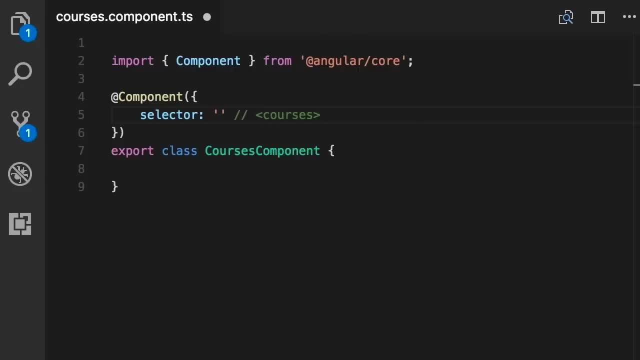 Why? Because with components we can extend HTML vocabulary So we can define new elements like courses, and inside that we will have the list of courses. Or in the future we can define a custom element, a custom HTML element called rating, and wherever we use that, Angular will render. 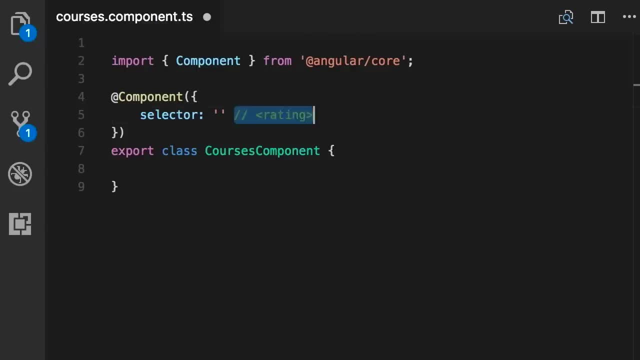 a rating component. Okay, So let's delete this. My selector for this component is courses. Now, the second property we add here is template, And that's the HTML markup we want to be rendered for this component. Now, here I want to render something very simple, so let's just add: 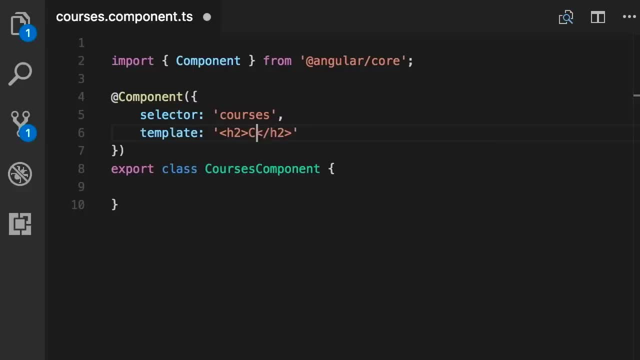 an h2 element and call this courses In a real world application. our templates can be several lines of code. In that case, we can put them in a separate file, and I'm going to show you how that works later in the course. So this is. 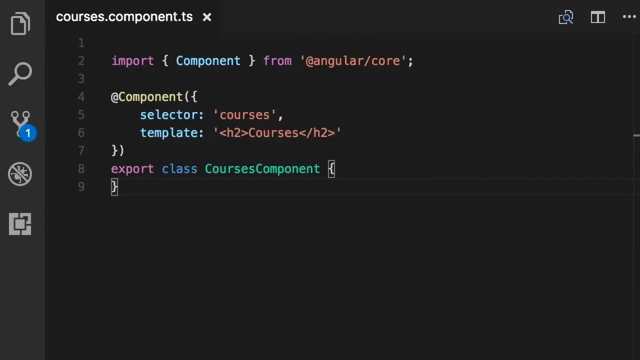 a basic component in Angular. That was the first step. The second step is to register this component in a module. Now, currently our application has only one module, which we call app module. Let me show you where that is. So back here. 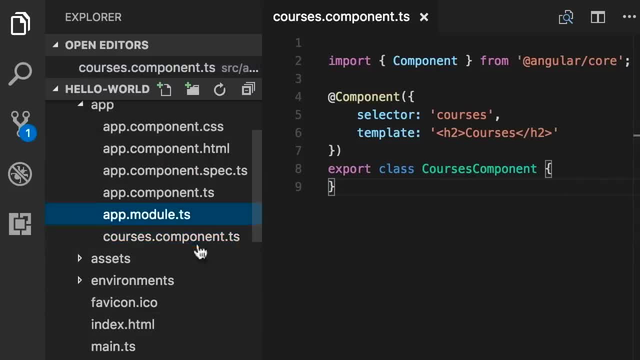 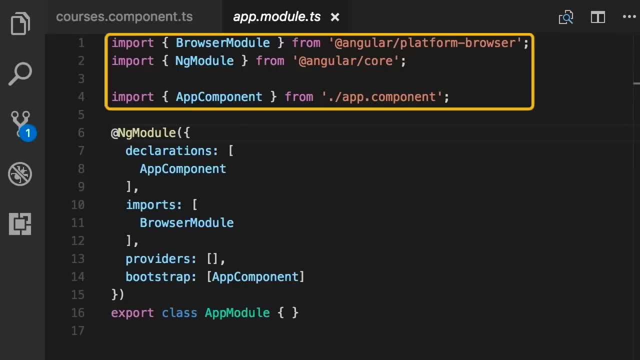 in the app folder. look, we have appmodule. Now, once again here, we have three import statements on the top, so nothing special here. On the bottom, we have a TypeScript class called appmodule, And note that this class is decorated with another decorator. 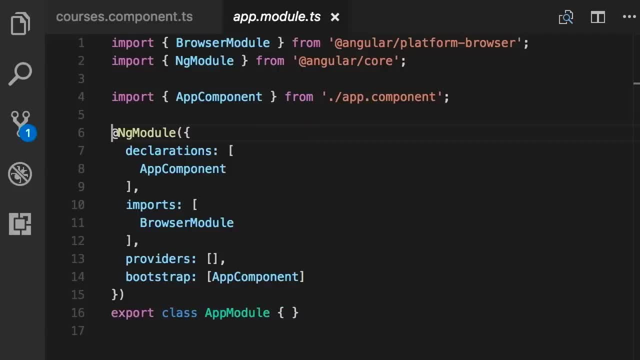 function called ngmodule. So with this we convert a plain TypeScript class to a module from Angular's point of view. Now don't worry about all these properties here, like declarations, import providers and bootstrap. You're going to learn about them later in the course. What I want you to focus on now: 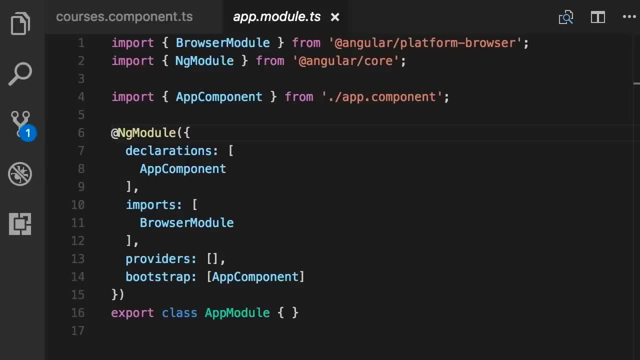 is this: property declarations And this is where we add all the components that are part of this module. So by default, when we generate an application we have one component called appcomponent and you can see that component is part of this module. Now I'm going to add our new component here. 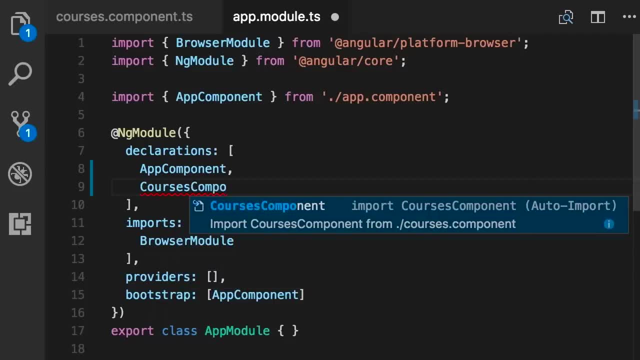 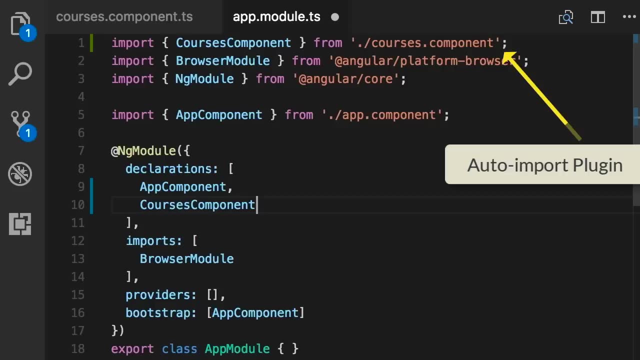 So courses component. So whenever I type the name of a class here and press enter, it automatically imports it on top of my file. So import courses component from: and here's the name of our TypeScript module. So period slash which refers to the current. 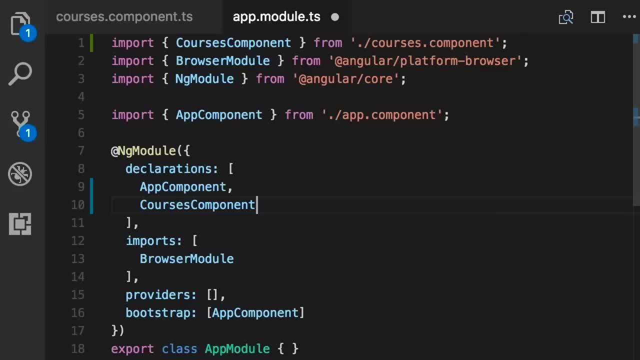 folder. and here's the name of the file: coursescomponent. Now, note that here we don't have ts. In fact, if you add that TypeScript component doesn't like that. So the name of the module is just the name of the file, without the extension. 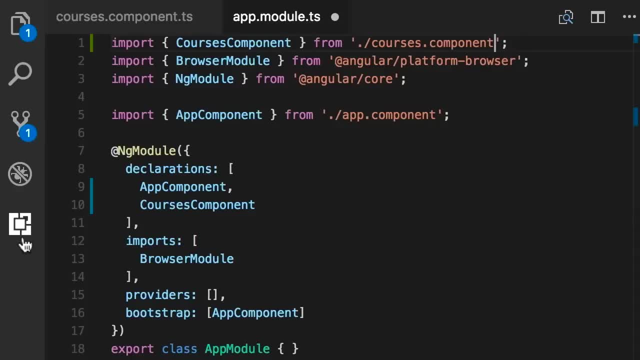 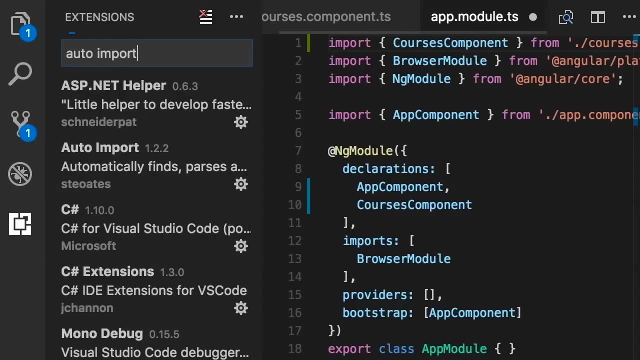 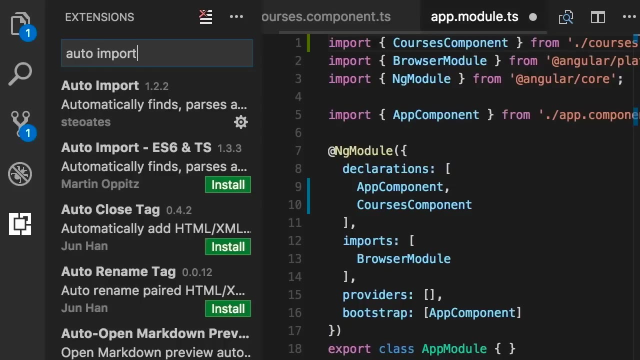 So if you want to add this plugin to your VS code, simply go here and in the extension search box, search for auto import. So currently I'm using auto import 1.2.2.. Simply install it and then you'll have to restart VS code. 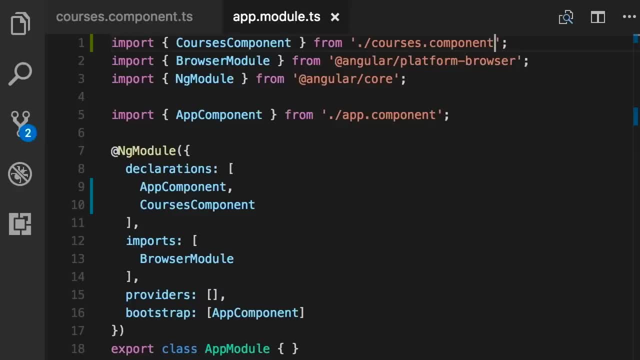 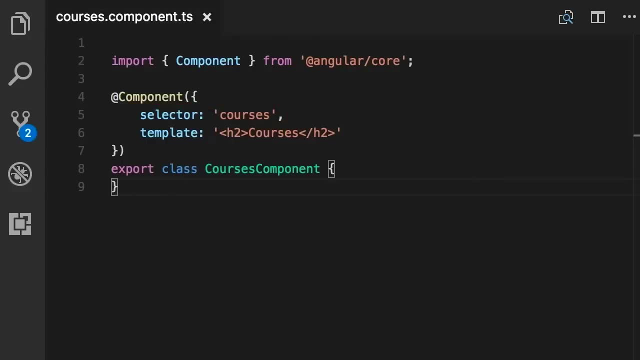 Alright, so here's our second step. Now the third step: Back to our component. so this is the selector for this component, Which means anywhere we have an element like courses, angular is going to render the template for this component inside that element. 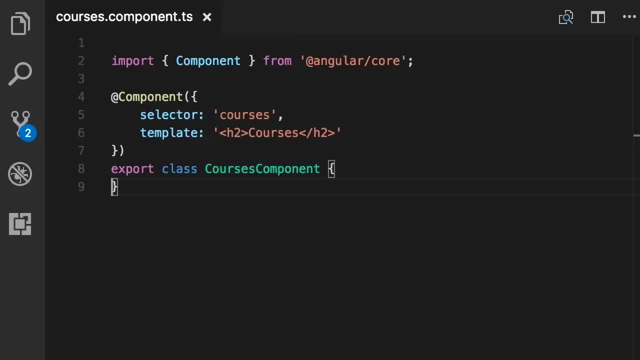 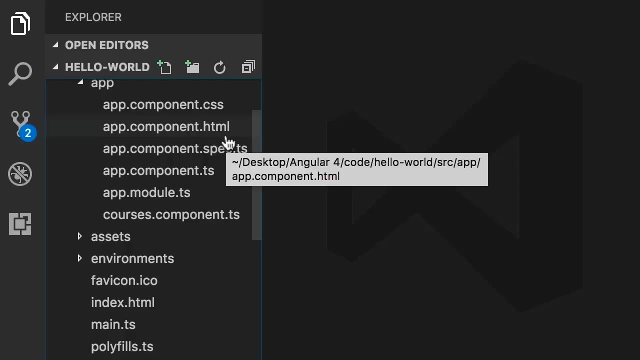 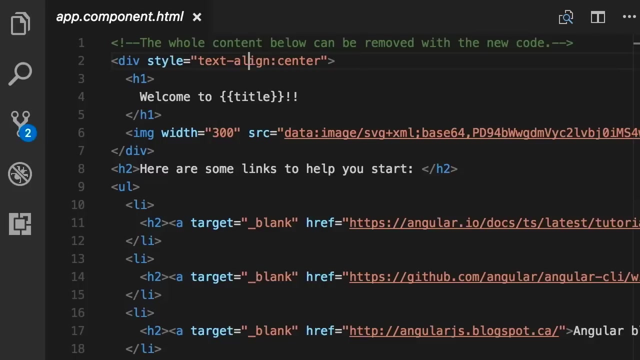 But where are we going to add that element? Let me show you. So back here in the app folder, we have this appcomponenthtml. This is the external template for our app component. Let's have a look. So all this markup you see here is for rendering the homepage. 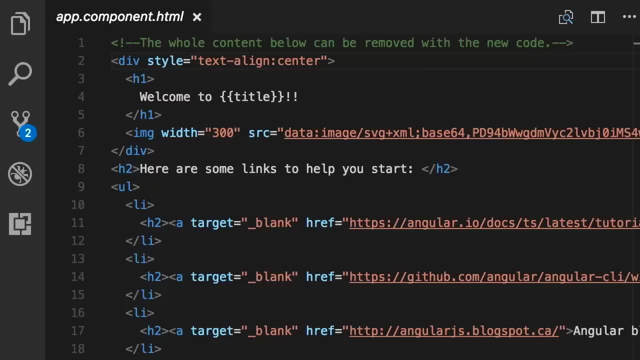 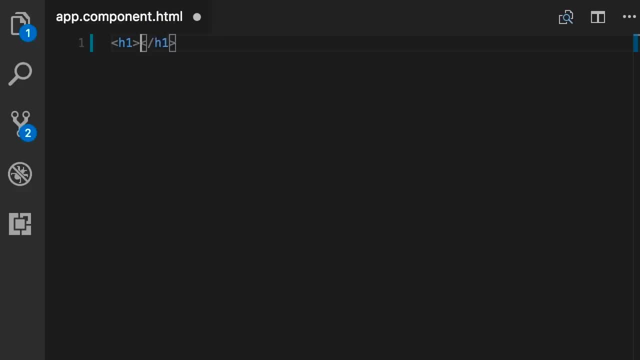 And this is what we get. Now I want to simplify this. I'm going to get rid of all this markup, add a simple h1,, call this angular, and below that I'm going to add our custom element courses. So when angular sees this element, 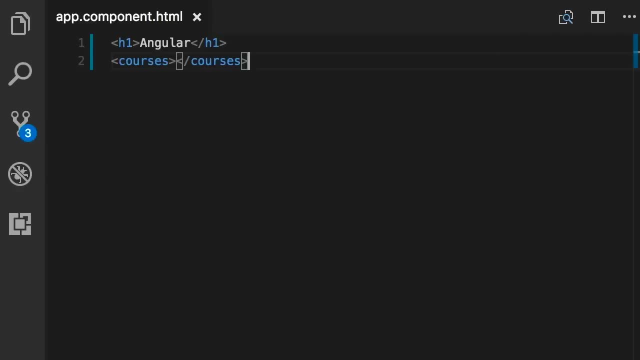 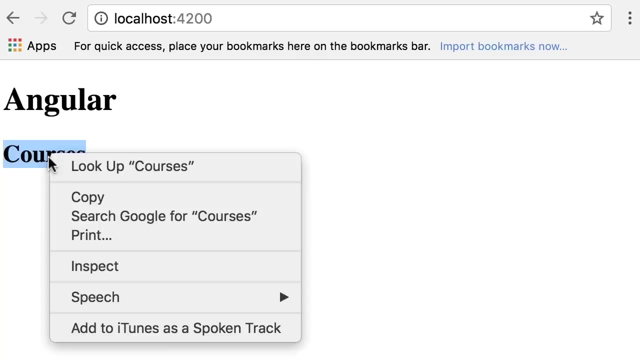 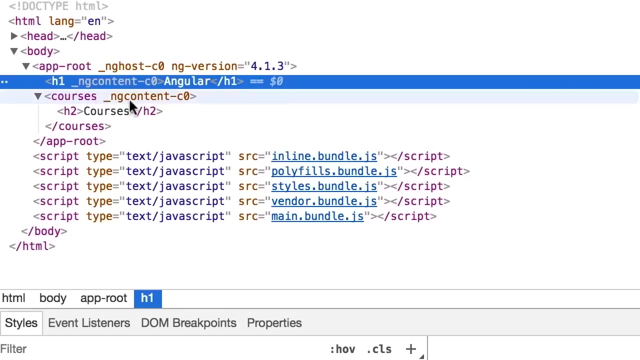 it's going to render the template of our courses component. Alright, now back in the browser. this is our new homepage, So let's right click this courses element and inspect this. So look what we have here. We have this h1, and below that we have our courses element. 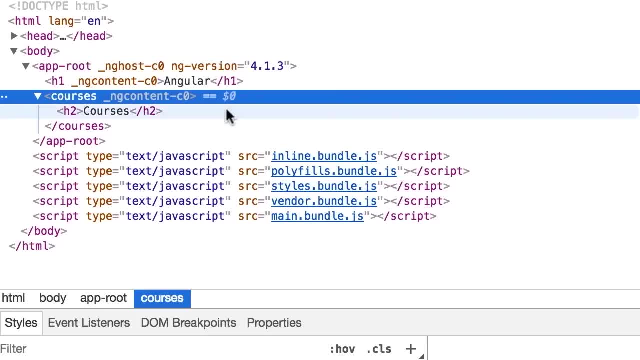 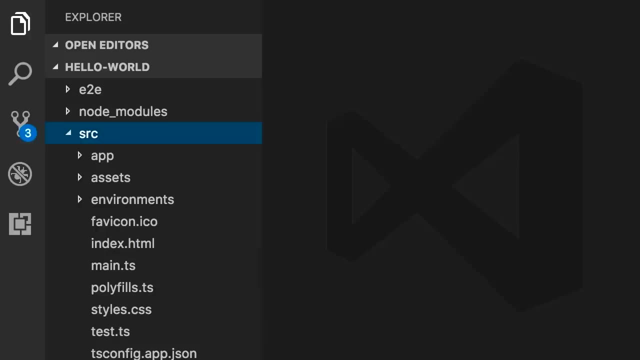 and inside this you can see we have the template for our courses component. So this is how angular applications work. As another example, look at this app root element inside the body element. Where is this app root Back in the source folder? look at indexhtml. 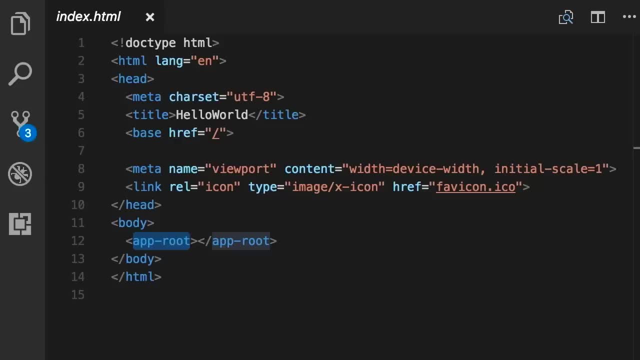 So this is the basic template for our application. right Now, inside the body element, we have an element called app-root. This is a custom element because we don't have an element in html called app-root. So from angular's point of view, we should have a component. 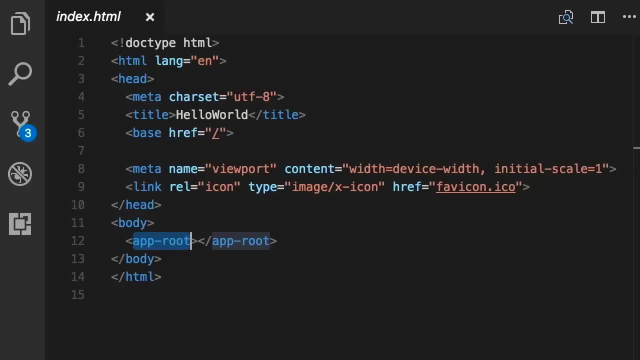 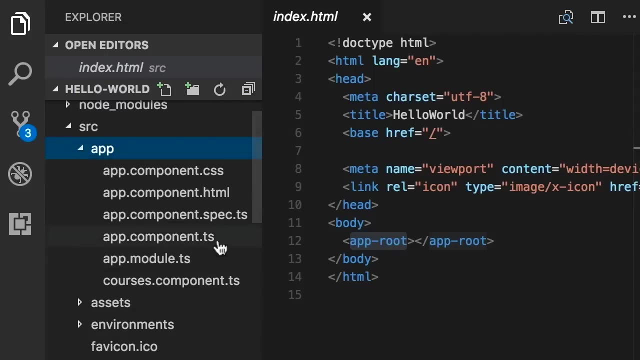 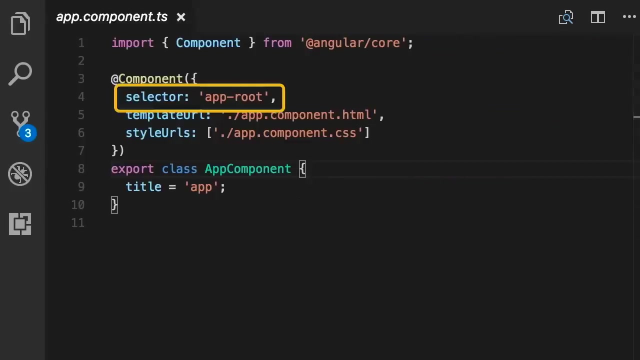 with a selector for this element, And that's our app component. Let's have a look at that. So back in the app folder, let's look at appcomponentts. So here's our root component, our app component. Look at the selector: app-root. 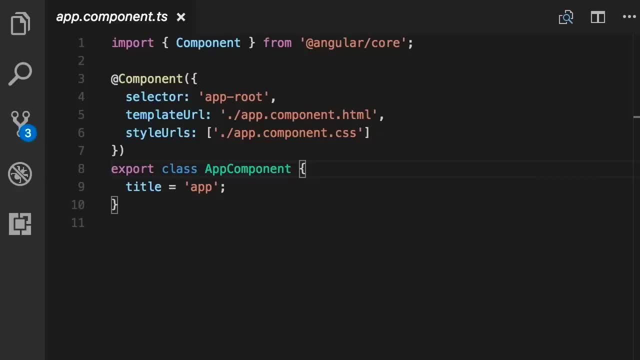 So whenever angular sees an element like that, it's going to render the template for this component inside that element. In this case, our template is external, so we have template url and you can see the name of our template file: appcomponenthtml. 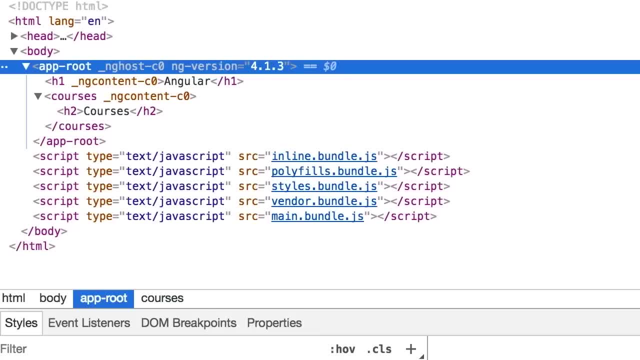 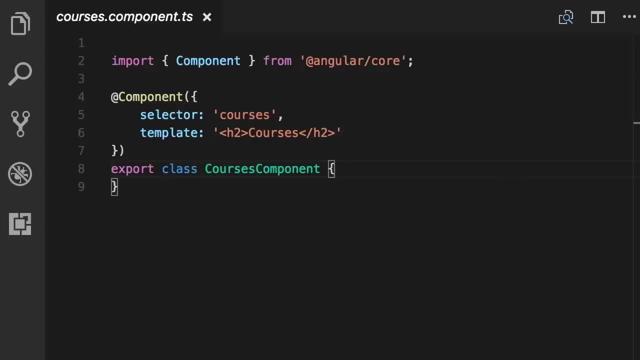 So that's why inside app-root here we have the template for app component, which includes an h1 and the courses element. Alright, let's quickly review what we have done so far. So we created this courses component here, then we register this in app-module. 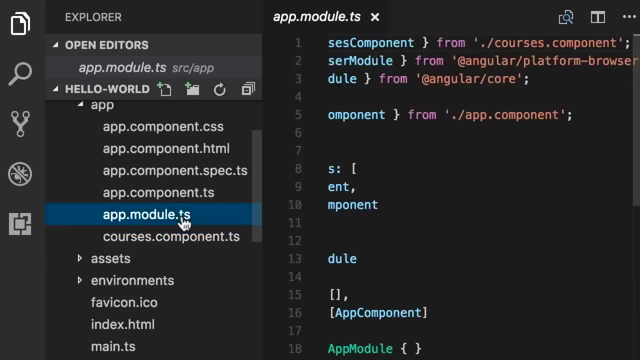 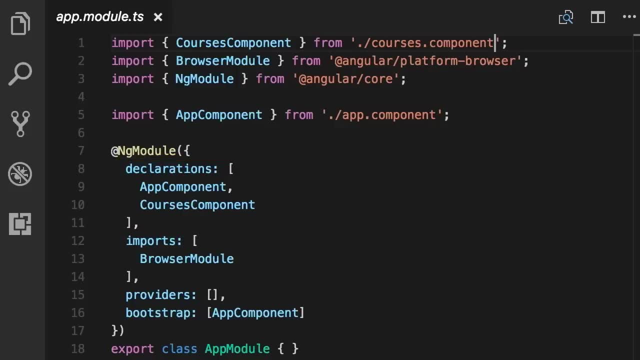 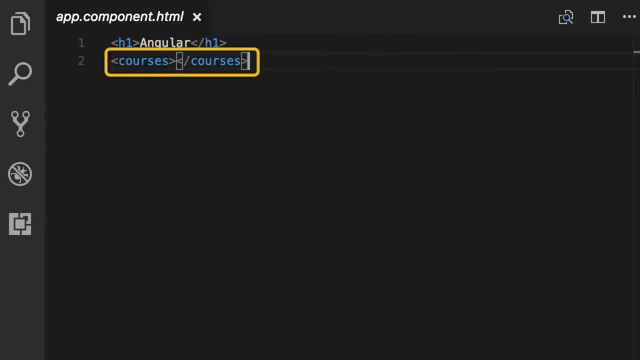 so here in appmodule we added our component inside the declarations array and then finally used this component in the template for app component. So let's quickly review appcomponenthtml. we added this courses element here. Three steps, okay. 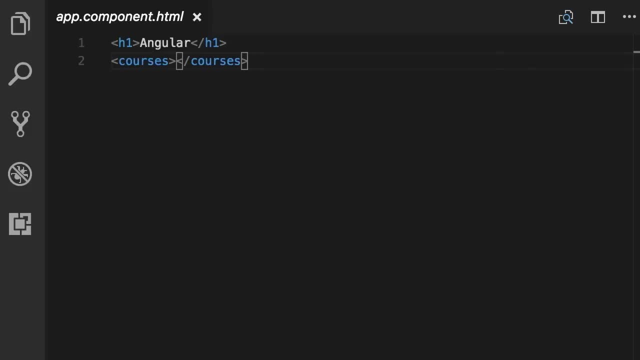 Now there are two problems with this approach. The first problem is that this approach is a little bit tedious. There are so many steps, So first we had to create this typescript class, then we had to import this component decorator on the top, and next we had to. 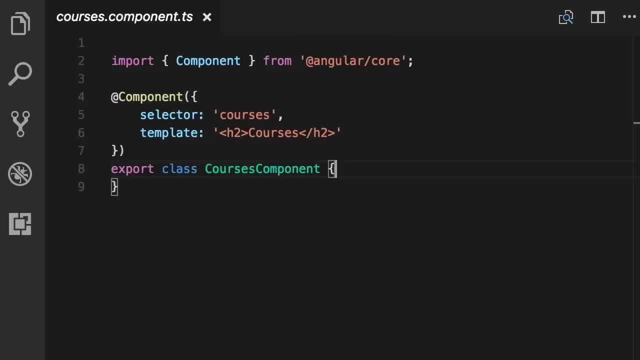 apply it on this typescript class. There is so much boilerplate code here. Now the second issue is that if we forget the second step, our application is going to break. Let me show you what happens. So let's go to appmodule. 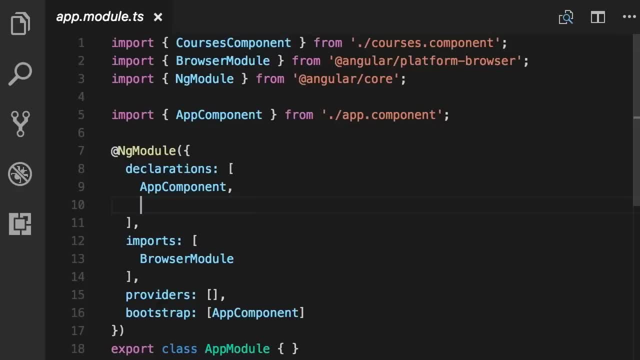 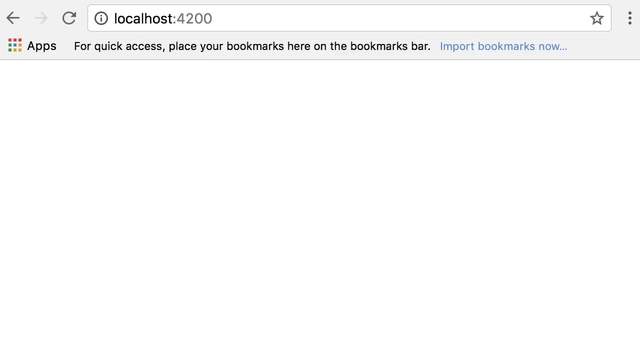 I'm going to delete this line here. Now let's see what happens Back in the browser. we got a blank page, so now we need to look at the console tab of chrome developer tools. So right click anywhere on the page: inspect. 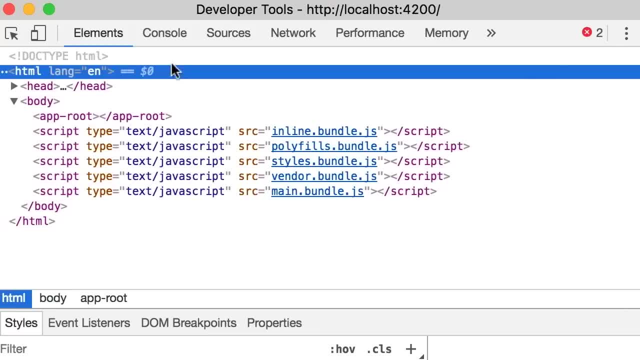 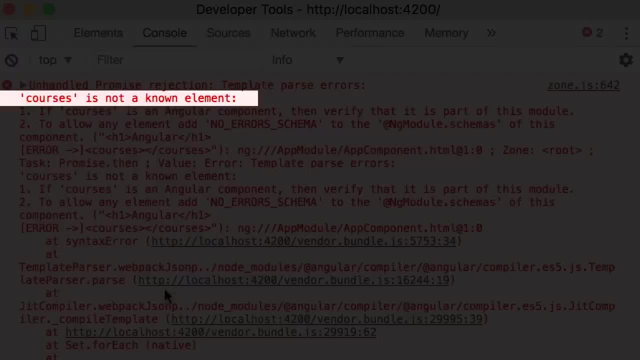 so we can see we have two errors here. we can see the details of these errors in the console tab. So here is the error. courses is not a known element. So if you don't register a component in a module, Angular doesn't know about it and it doesn't know what to do with this courses element. 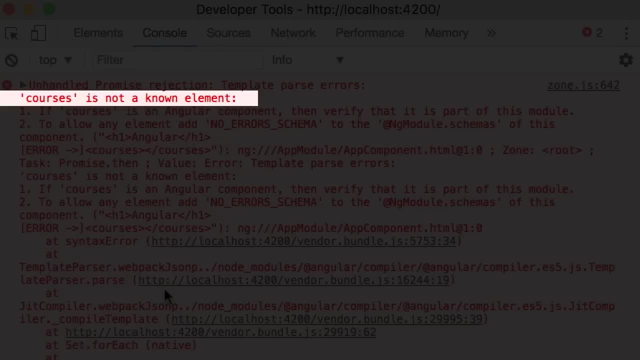 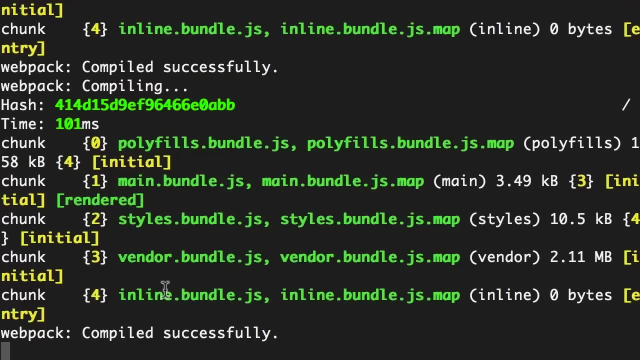 because this is not a native HTML element. So now let me show you a quicker and more reliable way to create an Angular component. We need to go back to the terminal, but look, our terminal is already busy. it's serving the application, so we either have: 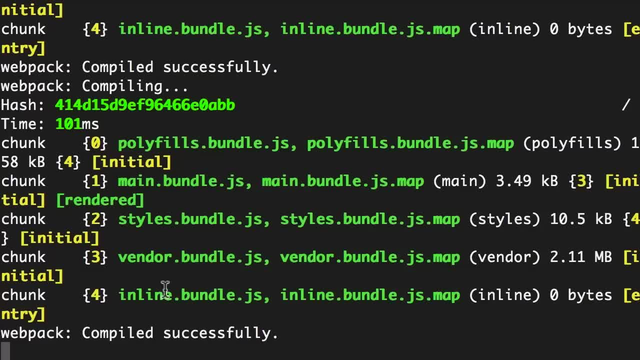 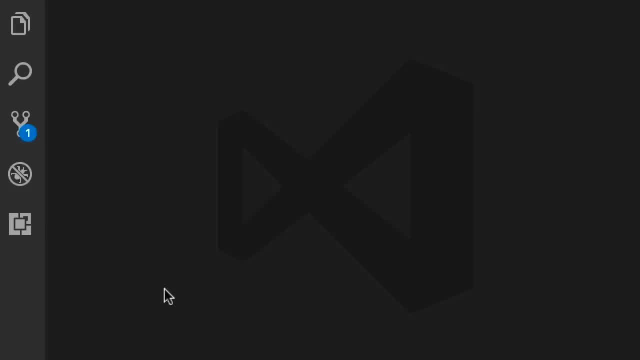 to open a new terminal window, or we can actually open a terminal window inside vs code. So back here. if you press control and back tick, which is the character before the number 1 on your keyboard, look, we have a terminal window here and this is much easier to access. 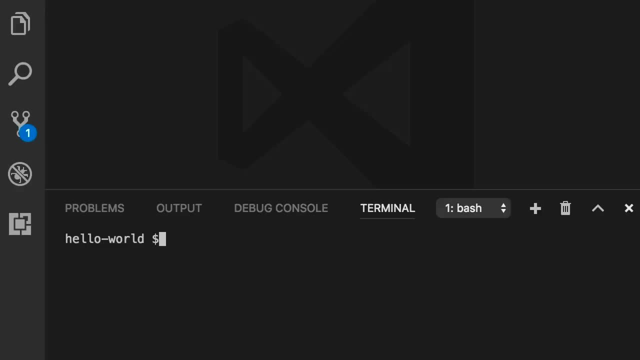 than going back and forth between different windows. So here we can use Angular CLI to generate a component. so just like how we generated an application with ng new, we can also generate a component with this ng. So the syntax is like this: ng- space g. 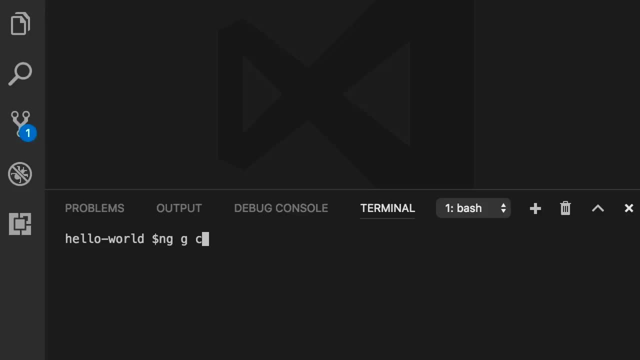 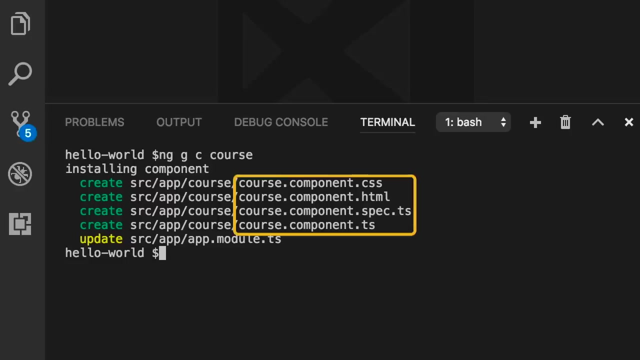 which is short for generate, and c, which is short for component, And then the name of the component. let's say, we want to create a component, called course. So a course. Look at what happened. Angular CLI created a directory, called course, and inside this directory added 4 files. 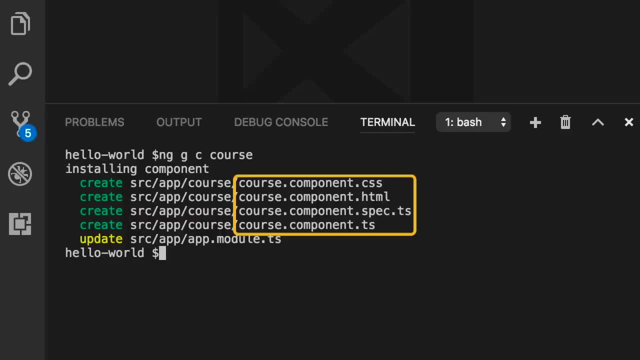 A CSS file for storing the stylesheets for this component, an HTML file for storing the template, a spec file which is for writing unit tests for this component, and, finally, a typescript file, which is the actual component itself. Now, what is interesting here is that it also updated. 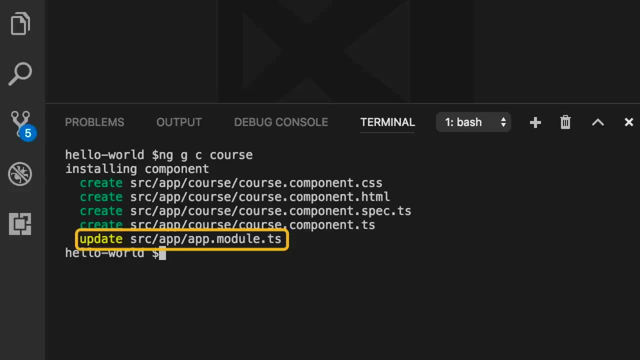 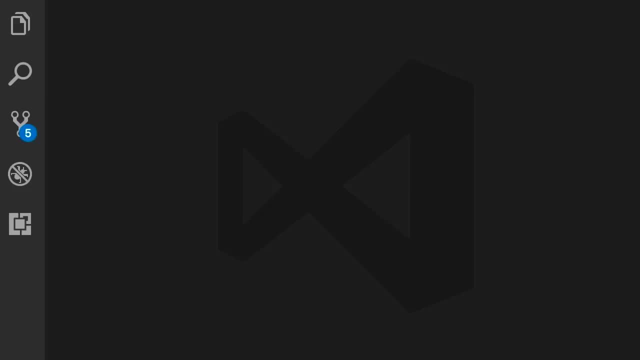 appmodule and registered this new component. Let's have a look. So we can close this terminal window using the same shortcut, which is control and back tick. Now we can open the files panel using command and b on mac or control b on windows. 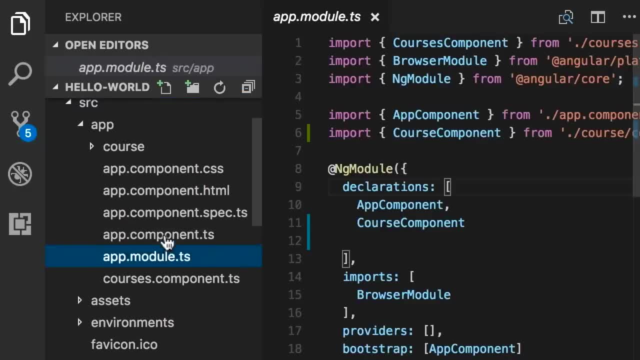 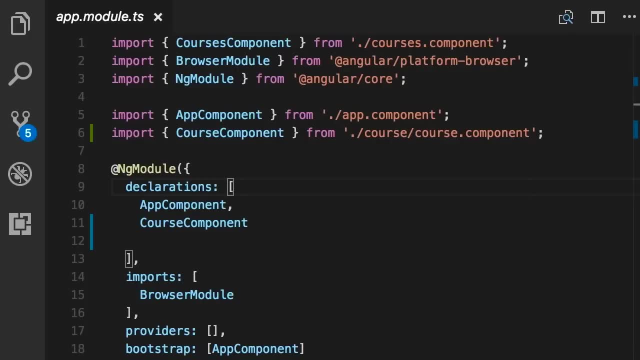 Okay, look at appmodule. So look inside the declarations array. now we have course component, So this way we don't have to remember to come back here and register our new components. Now, before we move on, let me just quickly add our courses component that I removed. 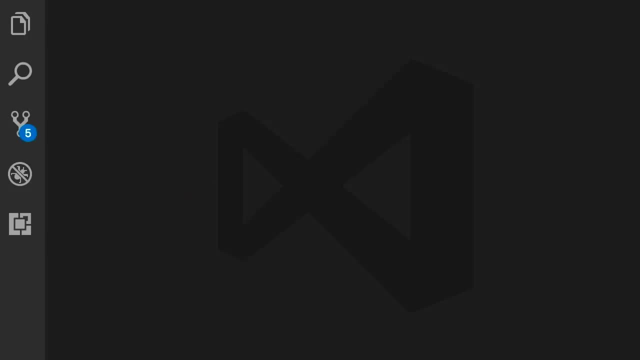 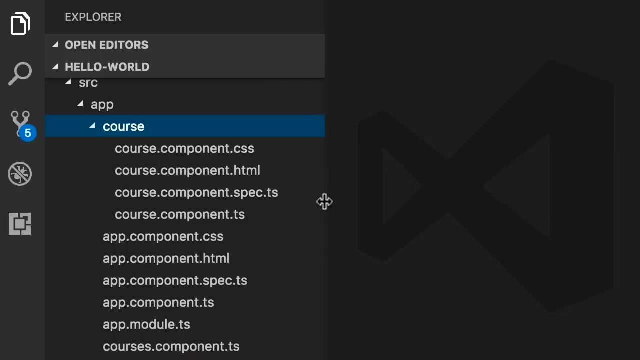 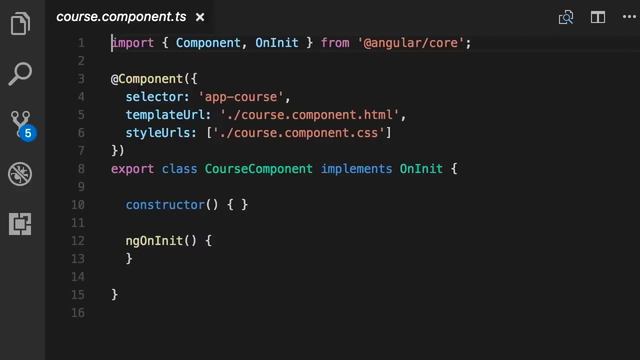 earlier. Okay, Now back in the files panel. this is the folder for our new component. So in this folder we have these 4 files. Now let's take a look at the typescript class. It has all the boilerplate code that we wrote earlier, plus a little bit more. So here we are, importing. 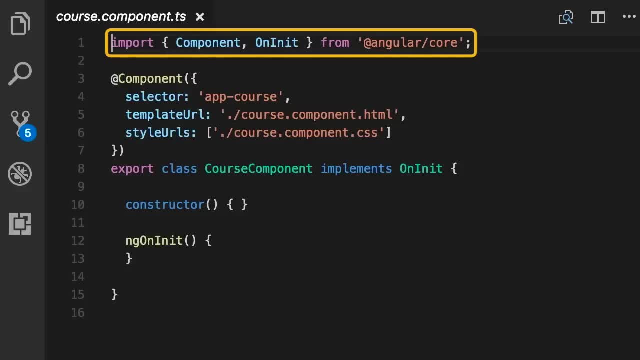 the component decorator and on init, which is an interface- we're going to look at this later in the course- we have this component decorator applied to our typescript class. we have a selector, we have the url of our template file, as well as the url of our 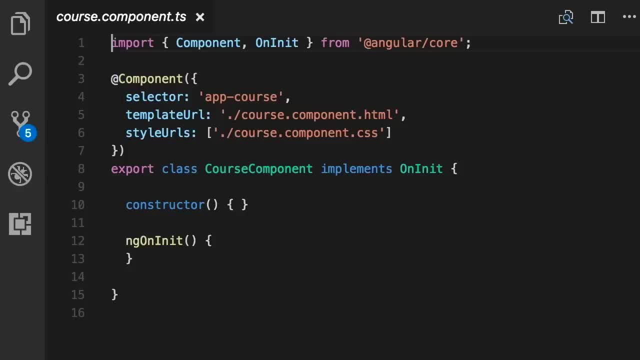 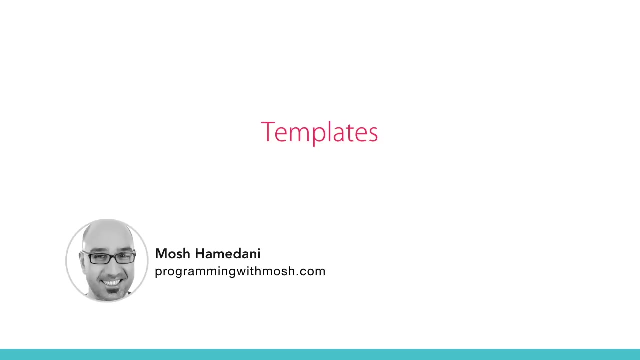 stylesheet file. So angular cli saves us a lot of time. Now, as we go through this course, I will show you how you can use this tool to generate other building blocks for your applications. So earlier I told you that a component encapsulates the data, the logic and the html markup. 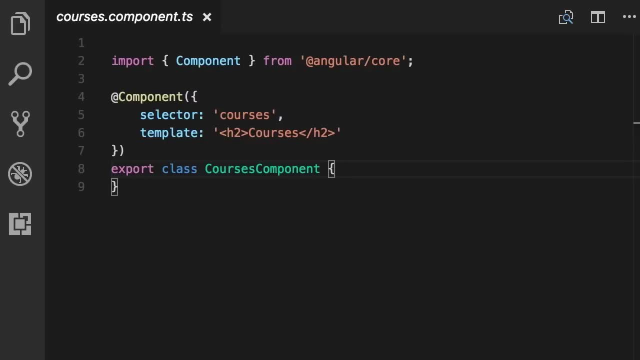 for a view. So in this example, in our courses component, we have the html markup, but we don't have any data or any logic. So let's extend this example and take it to the next level. I want to define a field in this class to hold the 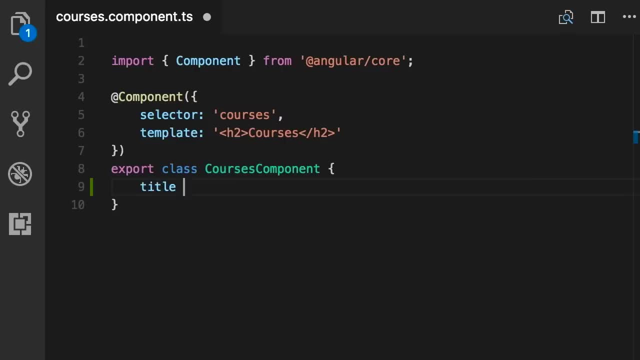 title of this page, So title. I'm going to set this to list of courses. Now I want to display this title in our template dynamically, So I'm going to remove this hardcoded label here. In angular we have this special syntax. 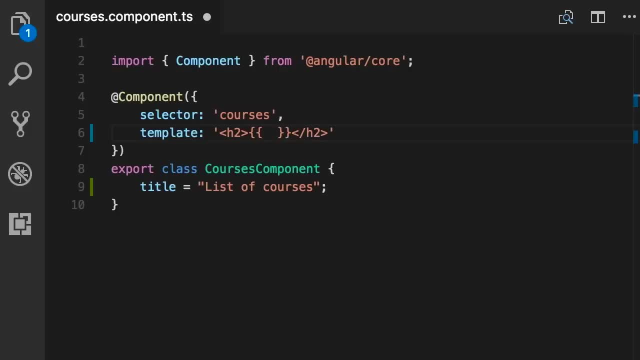 double curly braces and we use this to render something in our template dynamically. So here I can put this title field. this expression will be evaluated at runtime and the value of this title field will be placed in our dom Now, if the value of this title field changes at some point in the future. angular. 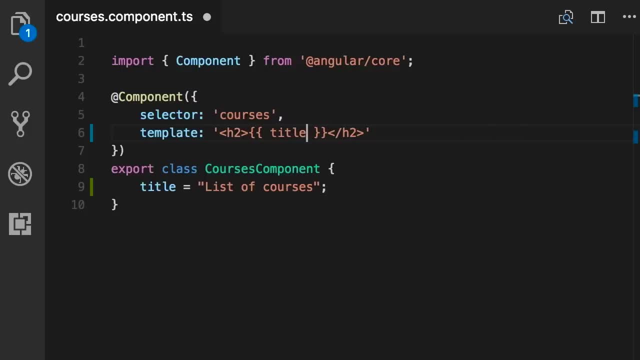 will automatically update the dom. This is one of the beauties of angular framework. So here we have this concept of data binding. So we are binding our view to a field in this component. Whenever the value of that field changes, the view is automatically notified and updated. 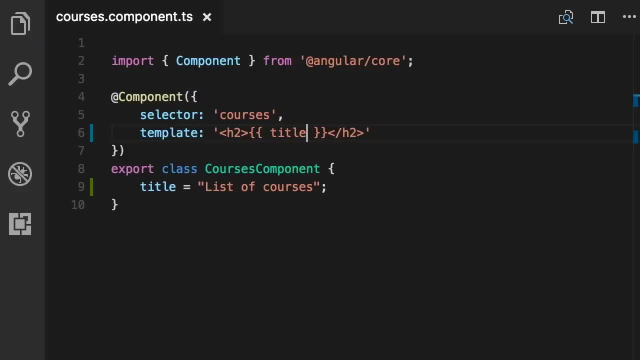 Alright, now let's save the changes back in the browser. Alright, here's our new title: Beautiful. Now back here. we don't always have to put the name of a field here. We can write any simple javascript expressions. For example, I can put a string here: title: 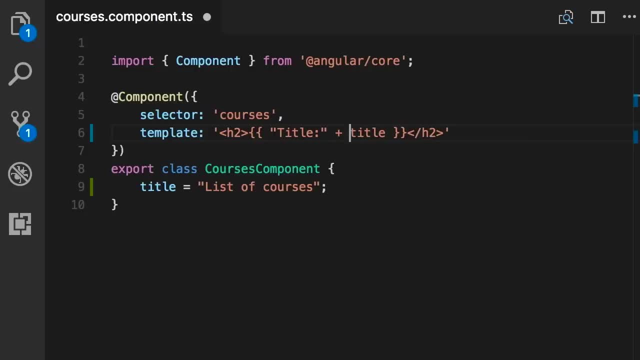 colon and then concatenate this with our title field: Save. Look, this is our new title Here. we can also call a method in this class to get some value. For example, let me define a method, get title, and here I'm going to return. 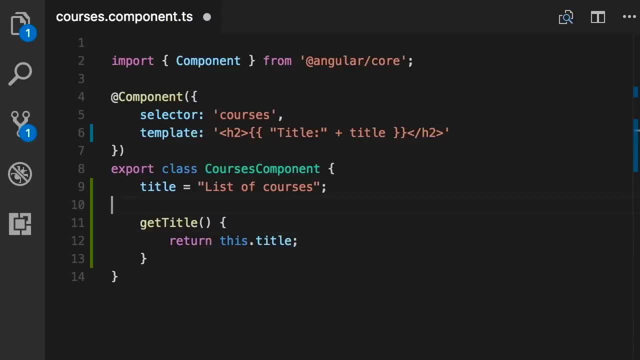 this the title. Now, here we can simply call our new method: get title like this and we'll get the exact same result. There you go, List of courses. So this special syntax here we call it string interpolation. In the next lecture I'm going to 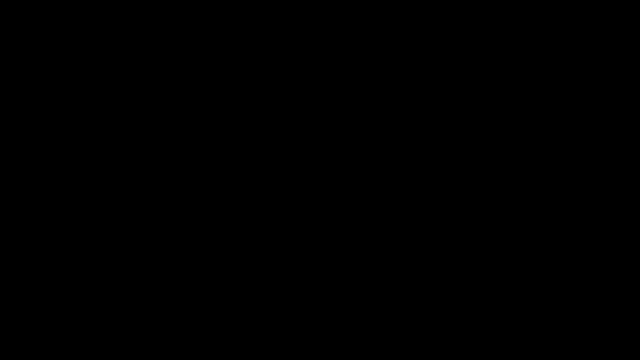 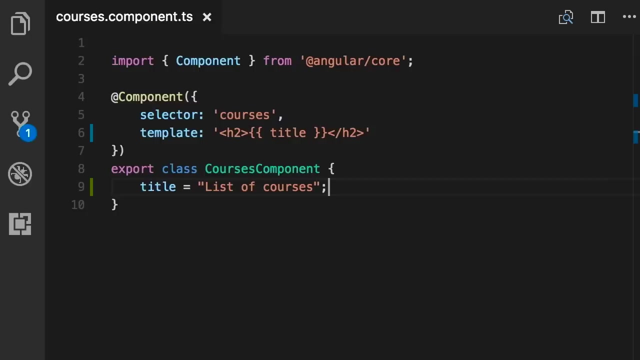 show you how to render a list of courses here. Alright, now let's take this example to the next level. Instead of displaying a simple title field, we want to display the list of courses. So first we need a field to hold the list of. 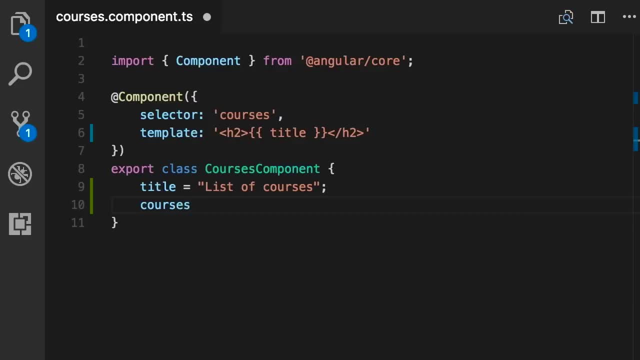 courses, So courses. we set this to an array with three items: Course one, course two and course three. Now this is a simplified example in a real world application. instead of simple strings here we would have objects, But don't worry. 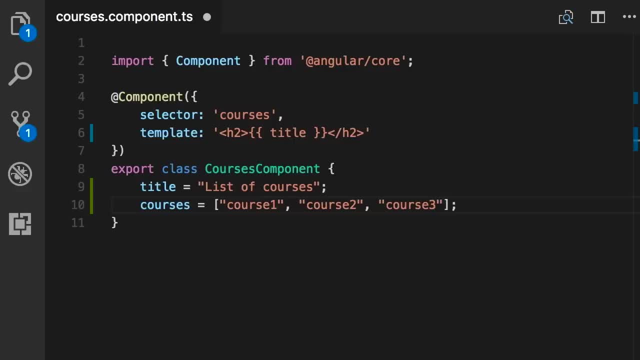 we're going to get there. Now. we want to display these in our template. How should we do that? First, we need to change this single quote to the back tick character. So delete back tick. Back tick is the character before number one on your keyboard. Let me change this as well Now. 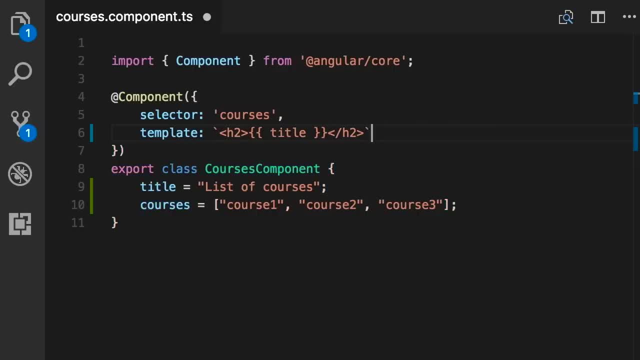 the benefit of using the back tick is that we can break up this template into multiple lines and make it more readable. So I want to put this h2 here, and below that I want to add a ul and a bunch of list item elements like this: 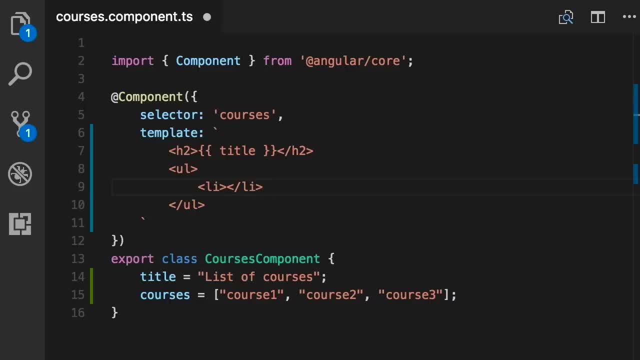 Now we want to repeat this li for each course. Now, for that we need to use one of the angular building blocks called directive. We use directives to manipulate the dom. We can use them to add a dom element or remove an existing dom. 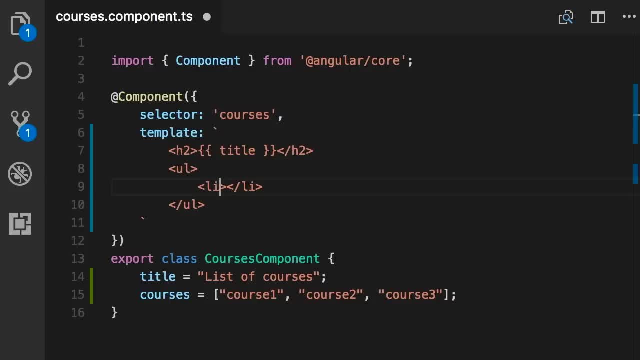 element, or change the class of a dom element or its style and so on. So here we're going to use a special directive called ng4.. We use it like an attribute in HTML, So we set it to a string, and here we're going to. 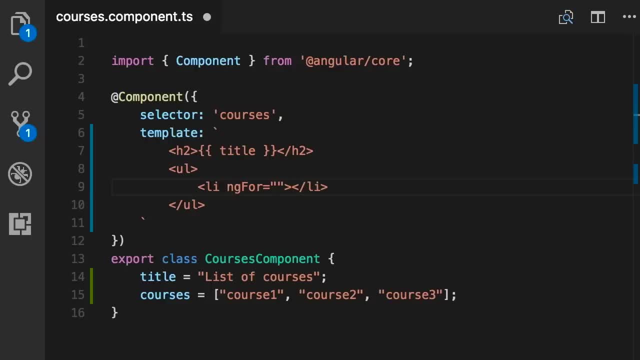 write some expression. Now, before going any further, we should prefix this attribute with an asterisk. This is a special syntax in angular, so whenever you're using a directive that modifies the structure of a dom, you should prefix that directive with an asterisk. In case you're curious about the reason, I have covered it. 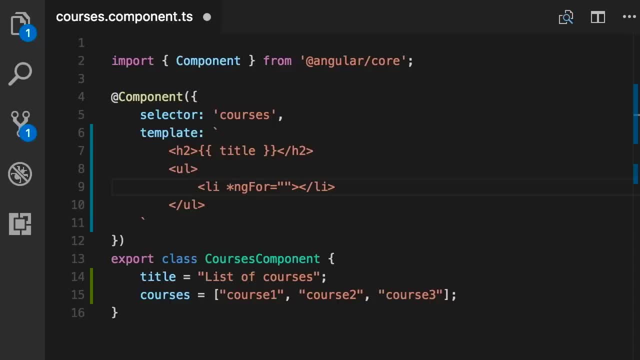 later in the section about directives. So for now, just remember, whenever you're using a directive that modifies the structure of the dom by adding or removing an element, you need to prefix that with an asterisk. Now here we want to write an expression similar to what we: 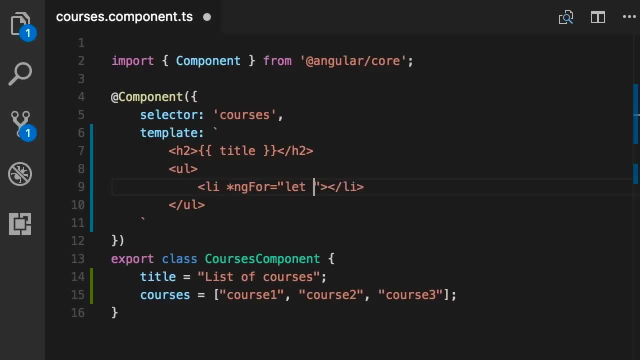 write in foreach blocks. So let course, of course. What does this mean? With the let keyword, we are defining a variable, So the name of our variable is course. This is like a loop variable in javascript. Of is a special keyword. 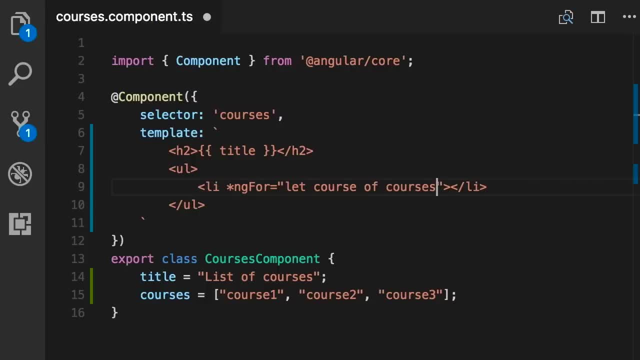 and courses is the field in this class that we are iterating over. So when angular sees this expression, it's going to iterate over the courses field and in each iteration this course variable will hold the value of one course at a time. Now, inside this list item, you want to display this? 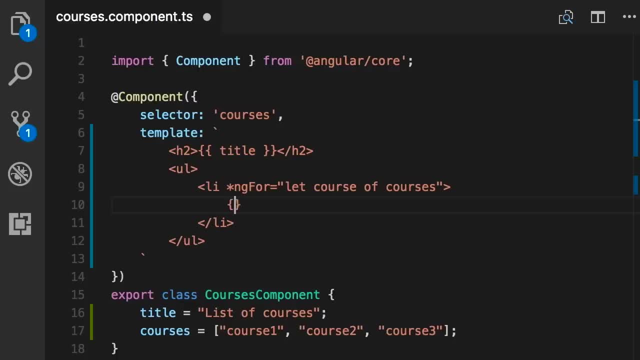 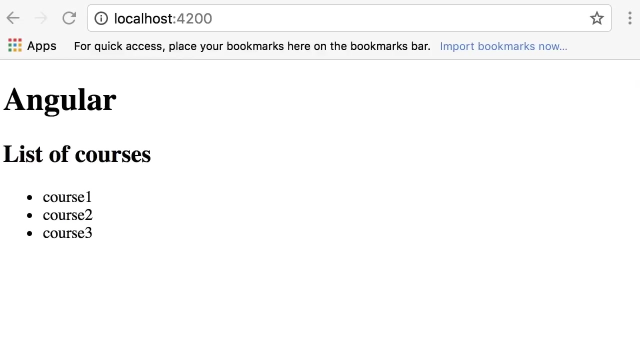 course. So once again we use string interpolation, double curly braces and add this course variable here. Let's look at the result. Save Back in the browser and here we have the list of our courses. Beautiful Now, in most real world applications we get these courses from the server. 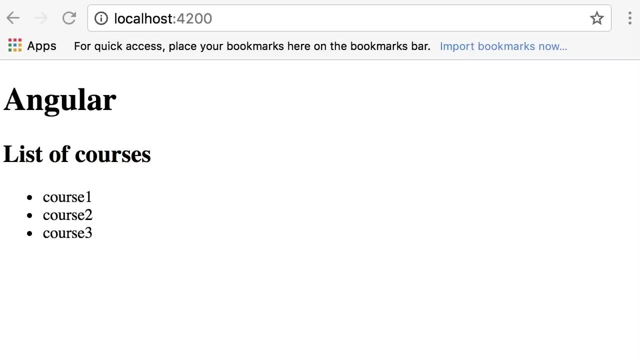 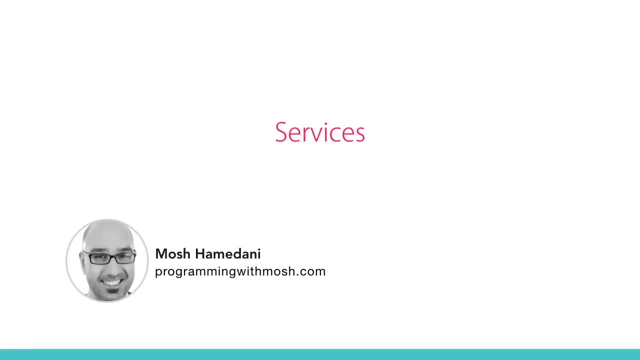 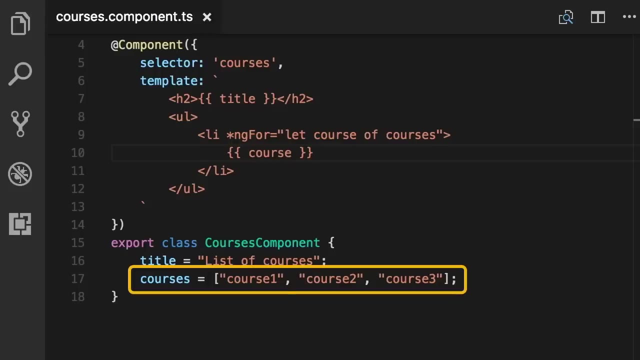 And for that we need to use another building block of angular called a service, And that's the topic for the next lecture. Alright, now we have the list of courses here, But in a real world application, most of the time we get these courses from the server. So instead of hard coding them here, 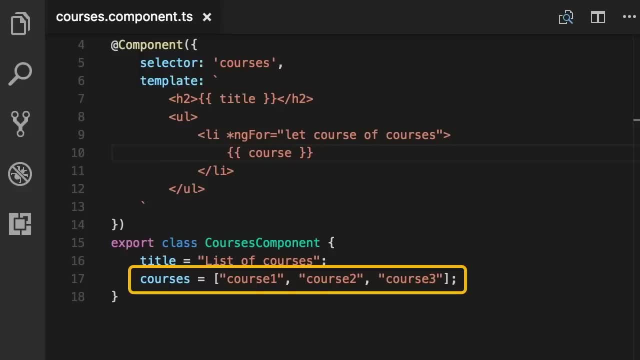 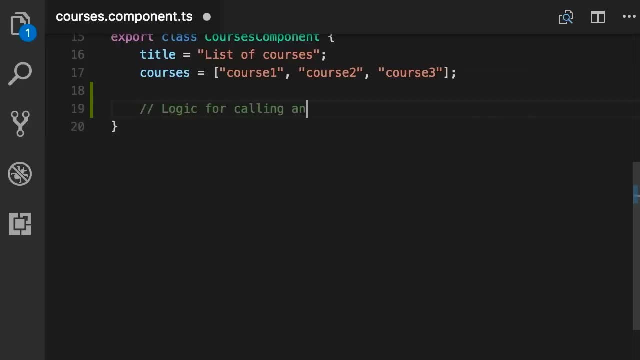 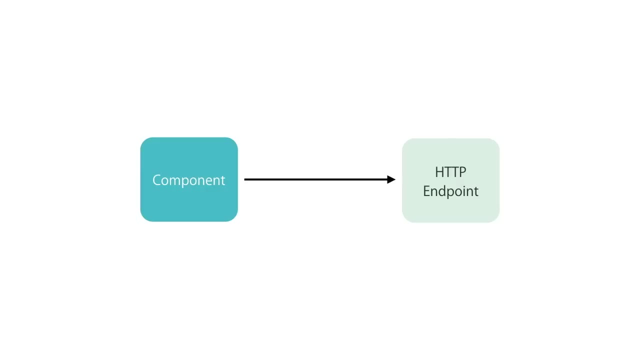 we need to call an HTTP endpoint to get the list of courses. Now here we have two options. One is to add the logic for calling an HTTP service here in this component. But there are a couple of problems with this approach. The first problem is that this logic is going to tightly. 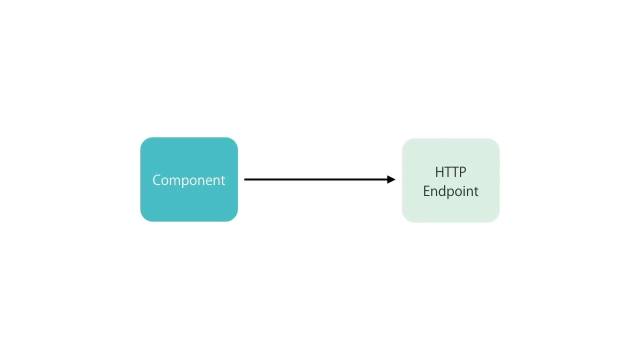 couple this component to that HTTP endpoint Now, in the future, when we want to write unit tests for this class, we don't want to be dependent upon a live HTTP endpoint, Because this is going to make it harder to execute those unit tests. 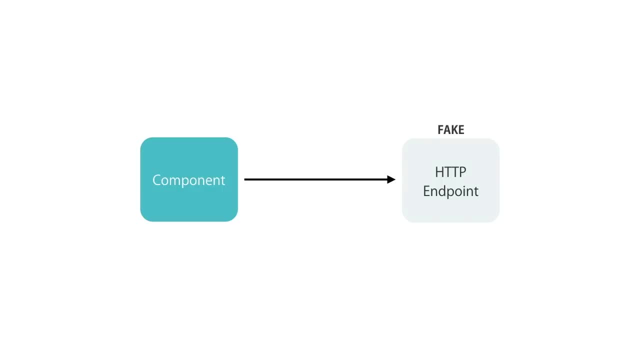 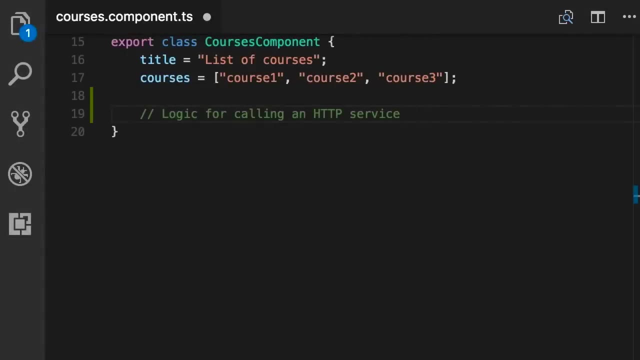 So we want to create a fake implementation of an HTTP service. So this is the first issue with writing this logic inside this class, inside this component. It's going to tightly couple this component to that HTTP endpoint. The second issue is that maybe somewhere else in the application we're going to have another page. 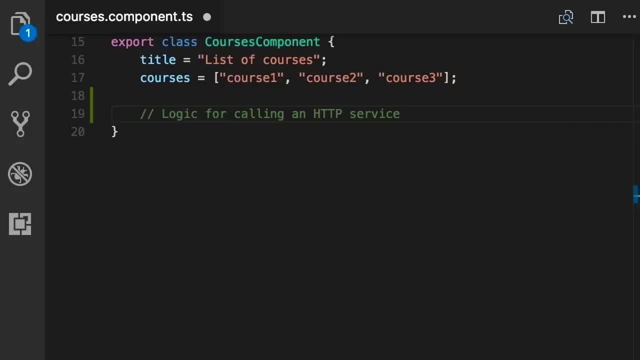 where we display the list of courses. Maybe it's part of a dashboard, Maybe it's somewhere for an admin. With this implementation, we have to repeat this logic, the logic for consuming that HTTP service in multiple places, And that's not good. And finally, the third. 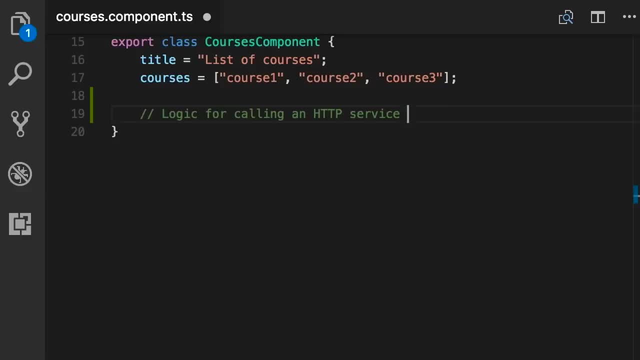 issue with this implementation is that a component should not include any logic other than the presentation logic. That is the logic behind this view. What should happen when we click a button, when we select an item from a drop down list, and so on? Details. 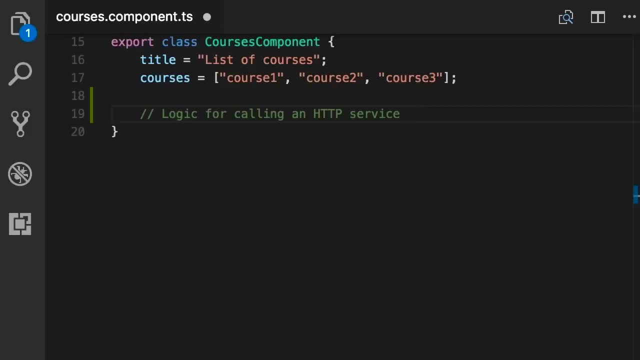 of how courses are retrieved should be delegated somewhere else in your application. So where should we implement that logic? In Angular we use services for that. So we're going to define a separate class, which we call a service, and there we'll add this logic for getting the list of 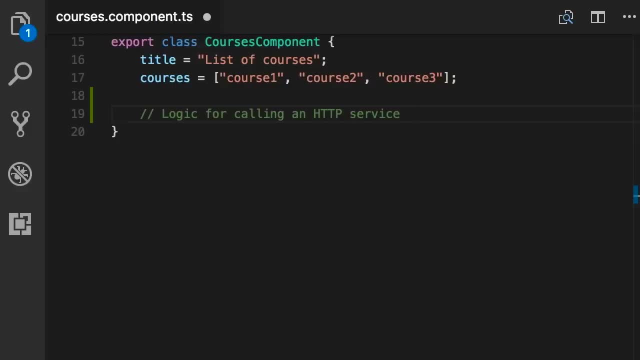 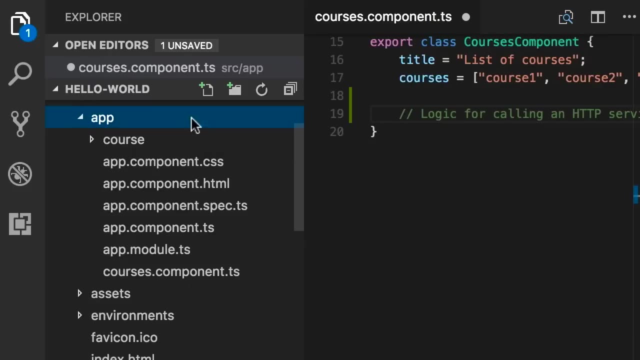 courses from an HTTP service. Then we can reuse this class in multiple places. So let me show you how to do that. Here in the app folder, I'm going to add a new file Now. look at the naming convention: Courses servicets. 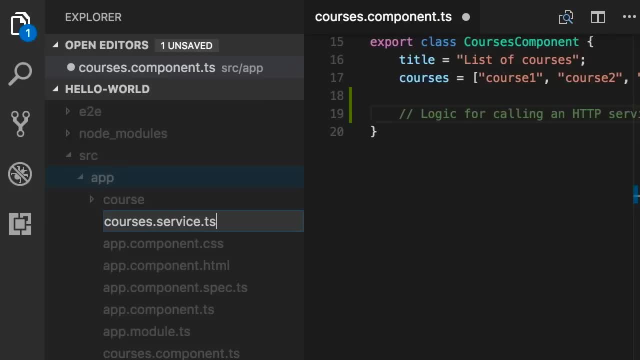 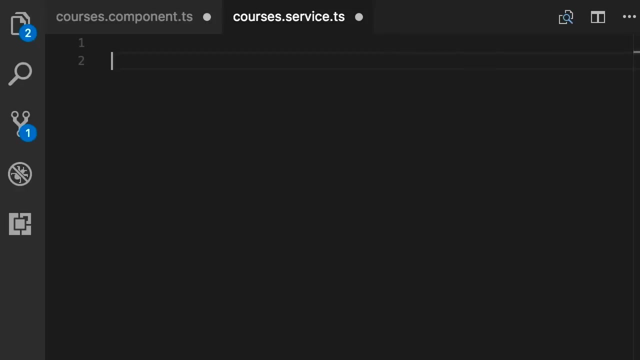 So the name of our service is courses and by convention we have the word service in the file name and finally ts. When creating a component, we use coursescomponentts, So note the difference. Now, here, once again, you want to export a plain TypeScript class, So export. 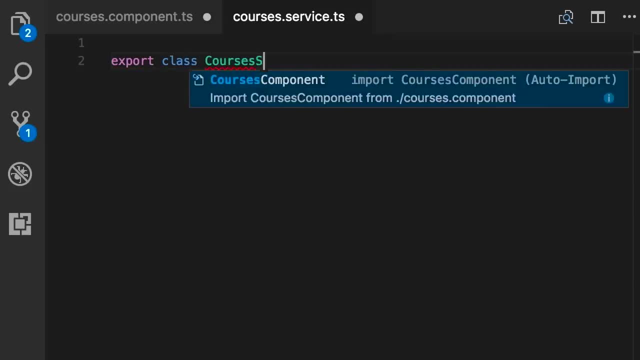 class courses- service. So once again, by convention we add the word service as a suffix in the class name. Now, when creating components, we decorate this class with the component decorator, Remember Component. But in Angular we don't have a decorator for services. 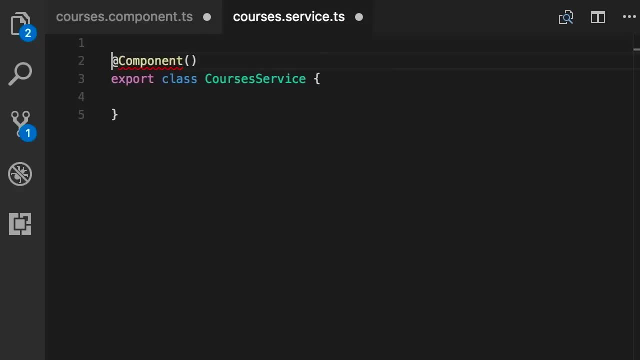 So a service is essentially a plain TypeScript class. So delete. Now. here we want to add a method for getting the list of courses. Get courses For now. we don't want to get distracted with the complexity of consuming an HTTP service, So let's just return the same array that we had in our component. 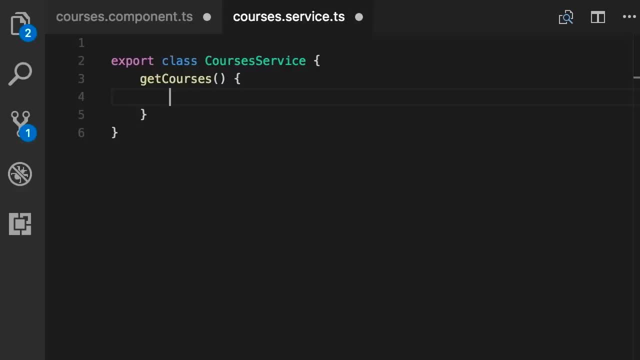 and later I will show you how to consume an HTTP service. So back in our component, I'm going to select this array here, cut back into service and simply return it from this method. Now imagine: here in this method we have that. 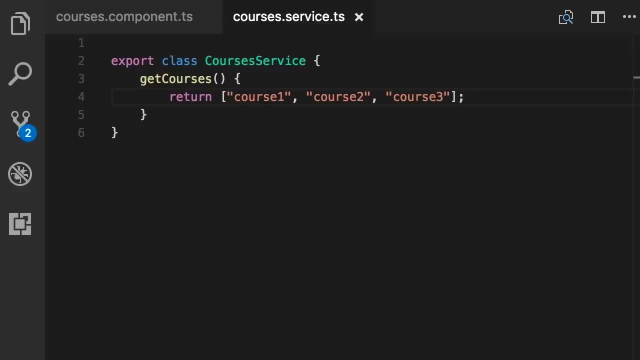 logic for consuming an HTTP service. With this implementation, we can reuse this class, we can reuse this logic in multiple places in our application And also this will separate or decouple our component from this logic. So back in our component. here we are not. 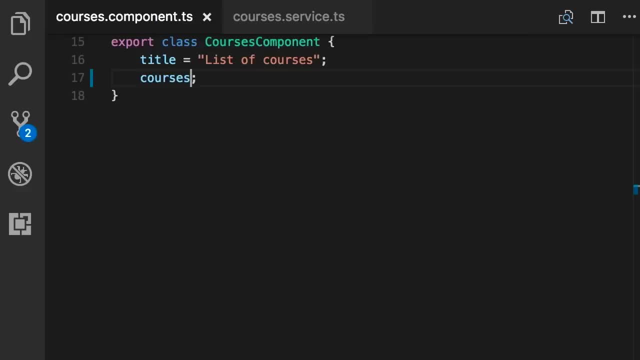 going to have any logic for consuming an HTTP service, And this allows us to unit test this class without dependency upon that HTTP endpoint. So while unit testing this class, we can provide a fake implementation of that service. Now, if that's too complicated, don't worry about it. unit testing is something for the future. 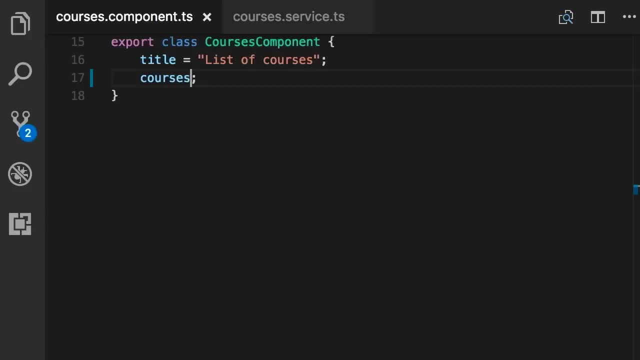 Okay, now we have a service. We need to use this service in our component How. That's the topic for the next lecture. Okay, now we have a service to get the list of courses from the server. We need to use this service. 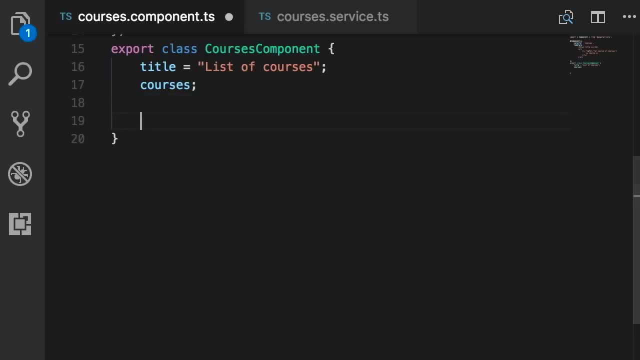 in this courses component. So first we need to add a constructor here. Constructor, Because a constructor is where we initialize an object. So here we need to create an instance of our courses service, Something like this: Let service be new courses service. 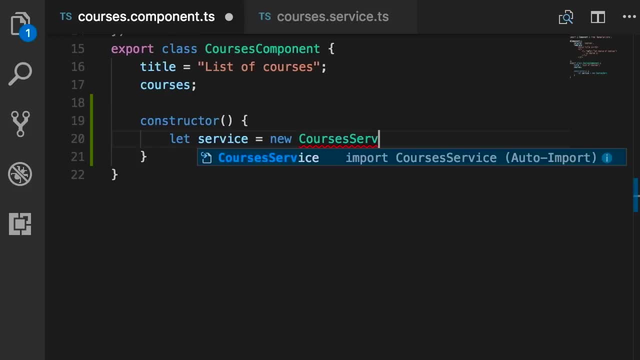 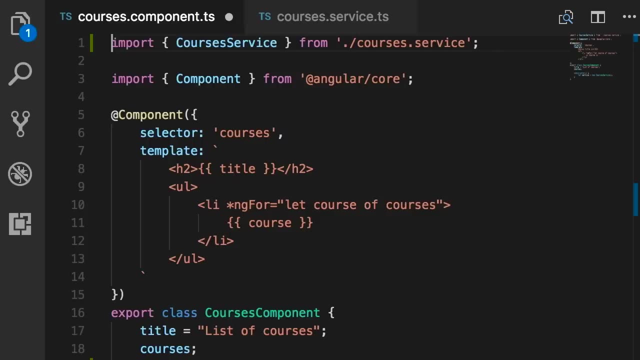 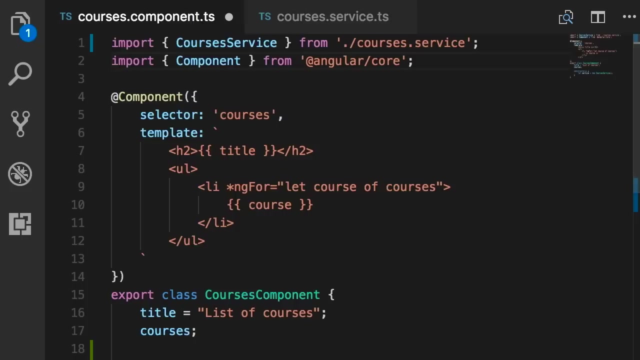 Once again I'm using the auto import plugin, So when I press enter it automatically adds the import statement here on the top. So import courses service from current folder coursesservice. Alright, now back in the constructor. So we have a service and then we can initialize. 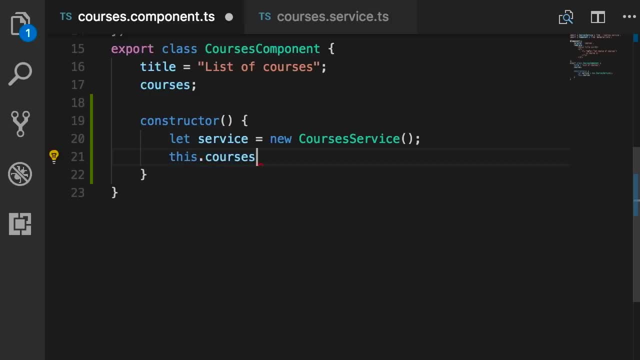 this courses field like this: Thiscourses. we set this to servicegetCourses. Let's test the application and make sure everything works up to this point. Save- Okay, we get the same list, beautiful. However, there is a problem with this implementation. The first problem: 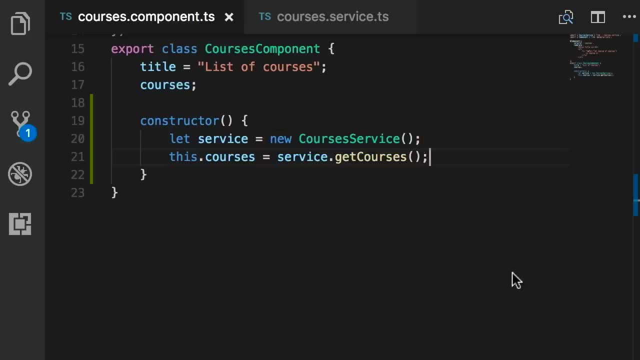 is that by using this new operator here, we have tightly coupled this courses component to the courses service. So this is exactly like the problem we had earlier. If we implemented the logic for consuming an HTTP service inside this component, we wouldn't be able to unit test this class. Now we put 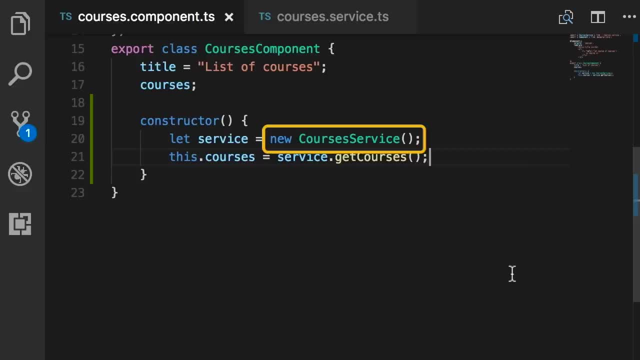 this logic in a different class courses service. but because we're directly creating an instance of this class here, we're still tightly coupled to that implementation. The other issue here is that if in the future we decide to add a parameter to the constructor of courses service, we have to come back here. 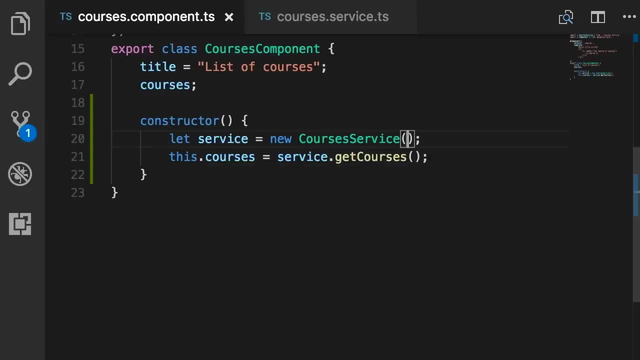 and anywhere else in our application where we have used this courses service and add a new argument like one. So anytime we change the constructor of this service, we end up with multiple changes in our application code. So this is very fragile. So what should we do? Well, instead of recreating an instance of the 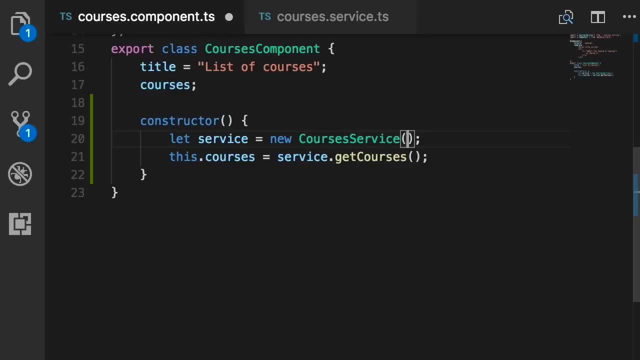 courses service. we can ask angular to do that for us, So we can delete this line here and add a parameter in this constructor. call it service of type courses service. With this, when angular is going to create an instance of our component, it looks: 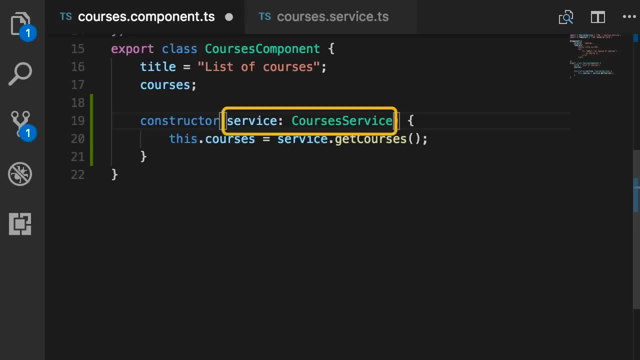 at this constructor, it sees that this constructor has a dependency. This dependency is of type courses service. So first it creates an instance of the courses service and then passes that to this constructor. Now, with this implementation, if we change the constructor of courses service and add 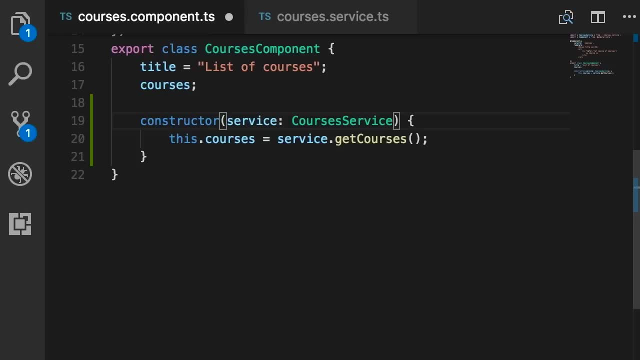 a new parameter. we don't have to modify 100 places in our code to reflect the change. Angular will automatically instantiate a new courses service object. The second benefit of this implementation is that when we are going to unit test this courses component instead of supplying an actual courses service, 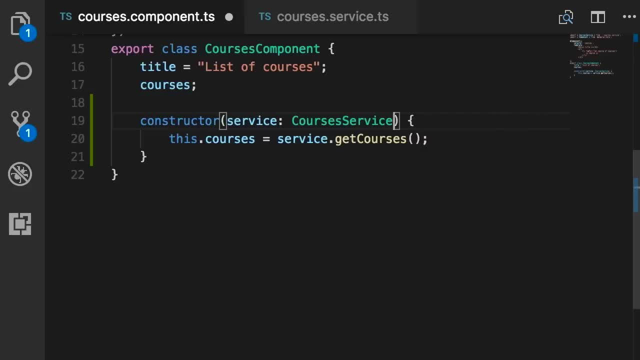 to this constructor, we can create a fake implementation of this service that doesn't use that HTTP service on the backend. In other words, we have decoupled our courses component from courses service. So here's the lesson: When you use the new operator like this inside a class. 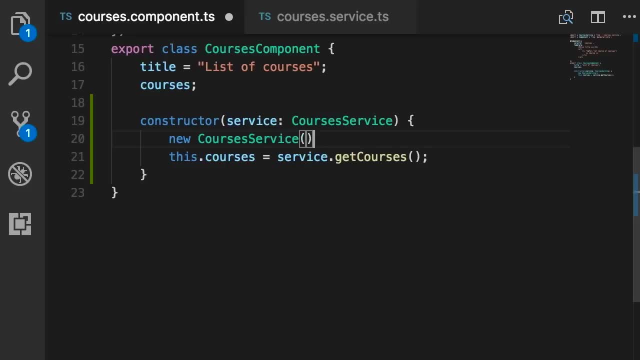 you have tightly coupled your class to that implementation. You cannot change this at runtime. But when you add that dependency as a parameter of a constructor, you have decoupled that class from that dependency. Now we're not done yet. We need to. 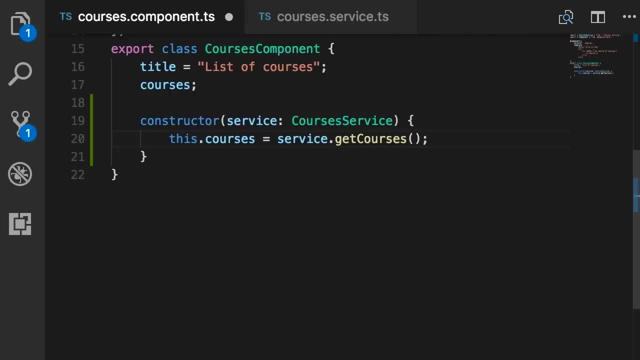 instruct angular to create an instance of courses service and pass it to our courses component. This concept is called dependency injection, So we should instruct angular to inject the dependencies of this component into its constructor. As simple as that. That's dependency injection. A lot of people think dependency injection is so complicated, but it's really. 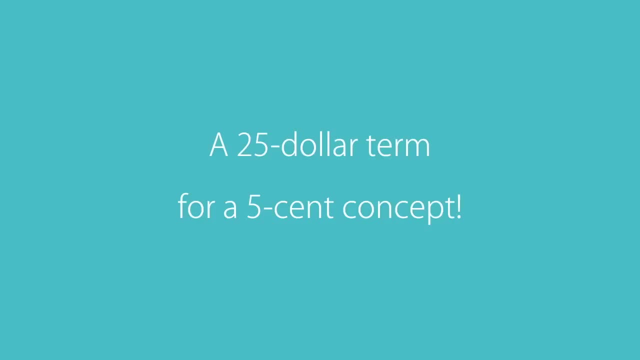 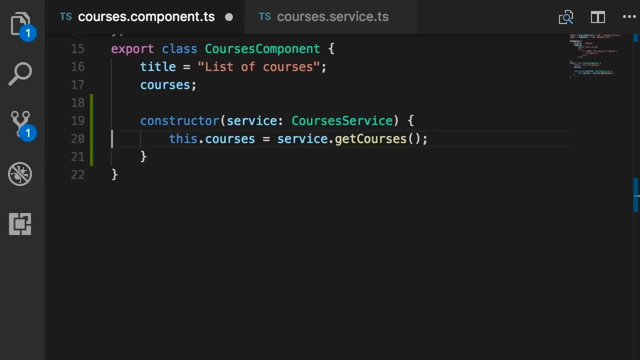 a $25 term for a 5 cent concept. So dependency injection means injecting or providing the dependencies of a class into its constructor. Now angular has a dependency injection framework built into it, So when it's going to create an instance of a component, it 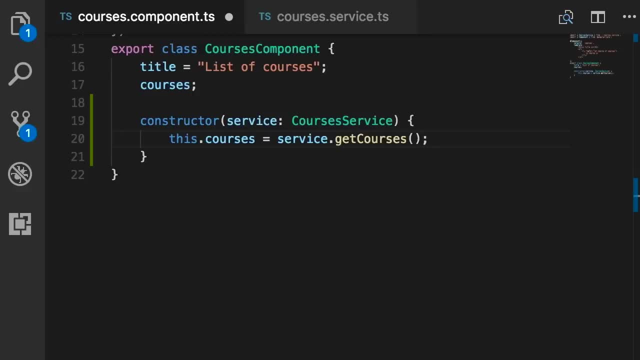 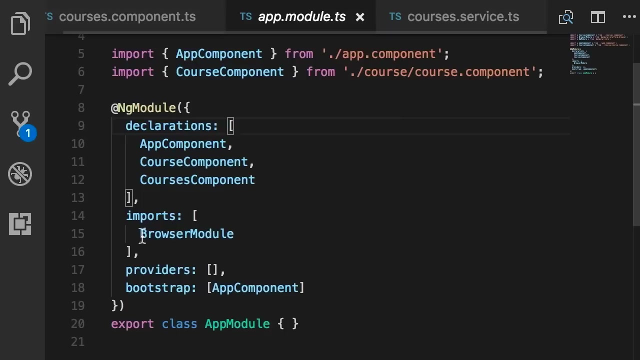 can inject the dependencies, But in order for that to work, we need to register these dependencies somewhere in our module. So let's save the changes. Now we need to go to our appmodule. So here's appmodule. Okay, look at this ngModule. 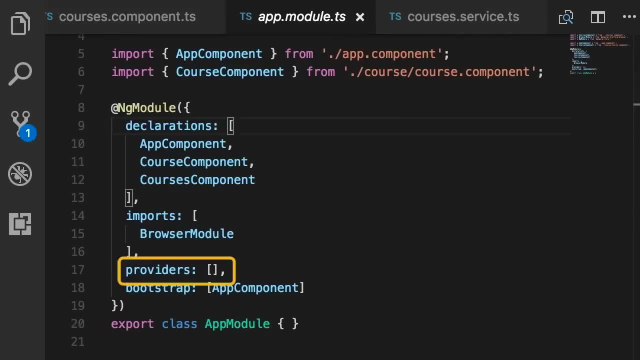 decorator. Here we have a property called providers, Which is set to an empty array. In this array we need to register all the dependencies that components in this module are dependent upon. For example, our courses component is dependent upon courses service, So we need to register. 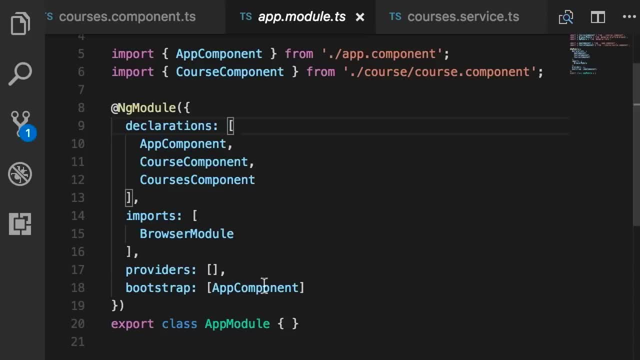 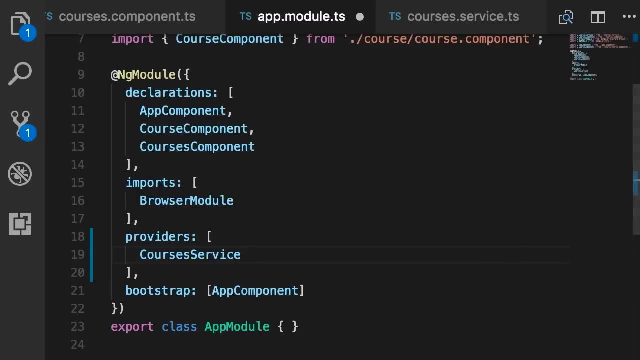 courses service as a provider in this module. So here I'm going to add courses service. Now, if you forget this step, dependency injection is not going to work. Let me show you what happens. So I'm going to comment out this line: save back to the browser. 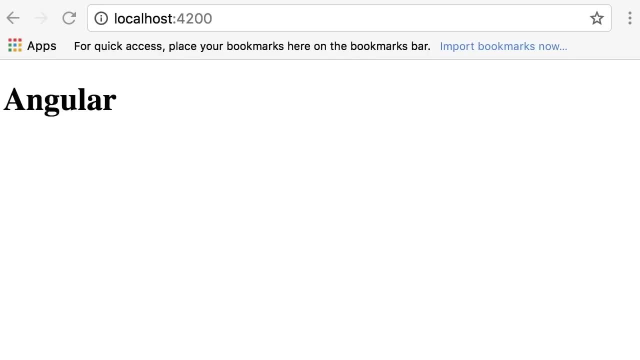 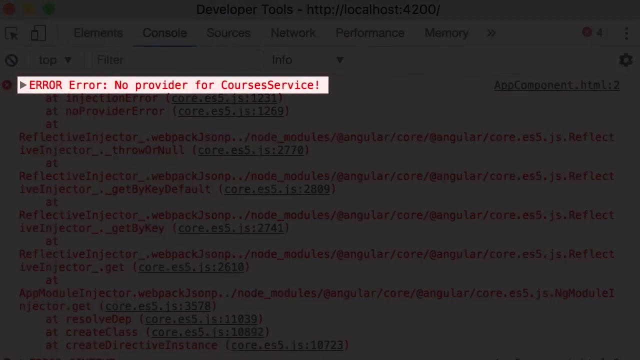 get a blank page, so that means something is wrong. Let's open up chrome developer tools with shift command and i on mac, or shift control i on windows. Look at this error: no provider for courses service. This is an error that you might see quite often when building angular apps. 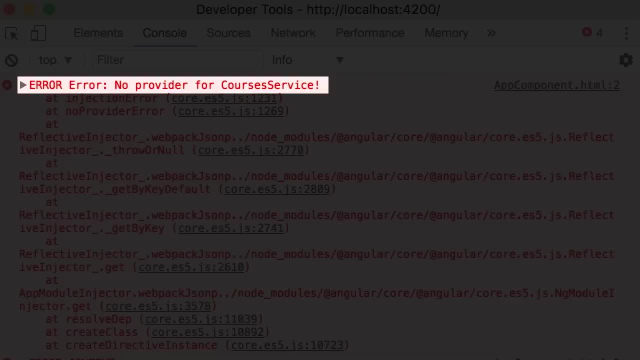 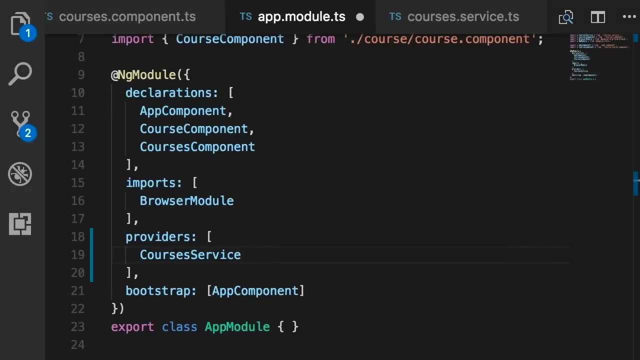 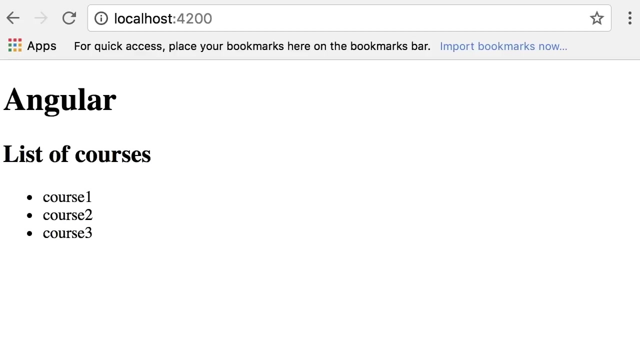 So the error is telling us that we have not registered courses service as a provider in our module. So back in appmodule, I'm going to add this courses service here. save back in the browser and we have the list of courses. Now one more thing before we finish this lecture. When you register a dependency, 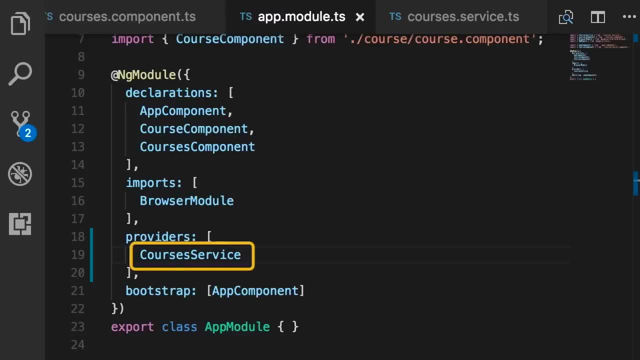 as a provider in a module, angular will create a single instance of that class for that entire module. So imagine: in this module we have 100 components and 50 of these components need the courses service. In the memory we're going to have only a single instance of courses service and 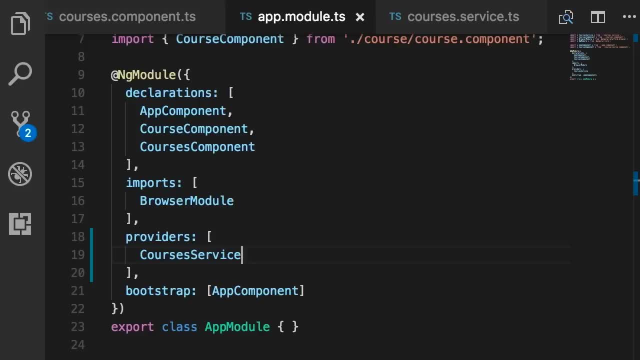 angular will pass the same instance to all these components. This is what we call the singleton pattern, So a single instance of a given object exists in the memory. So a quick round up. back in our component we added courses service as a parameter. 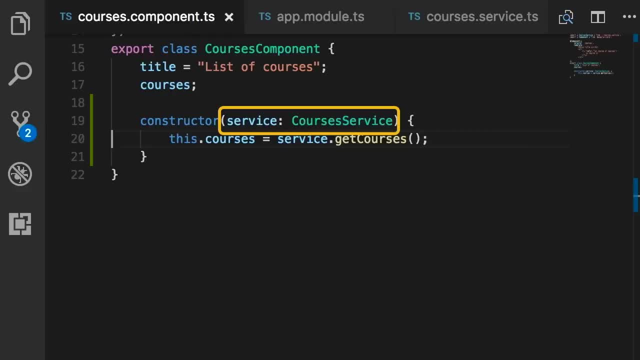 in the constructor, or in other words as a dependency of this class, and then registered this as a provider in our app module. With this implementation, when angular is going to create an instance of this component, first it will instantiate its dependencies and then it will inject those dependencies. 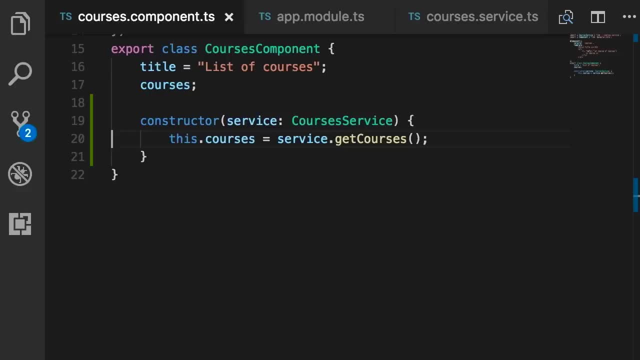 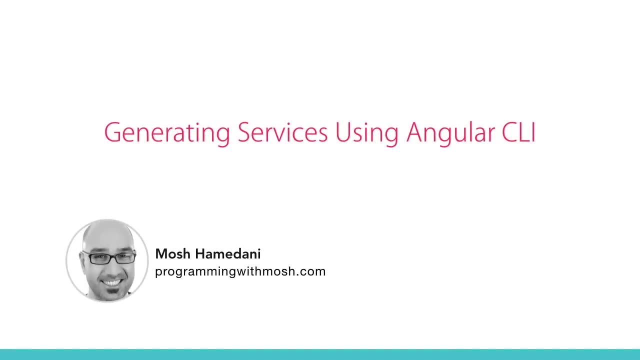 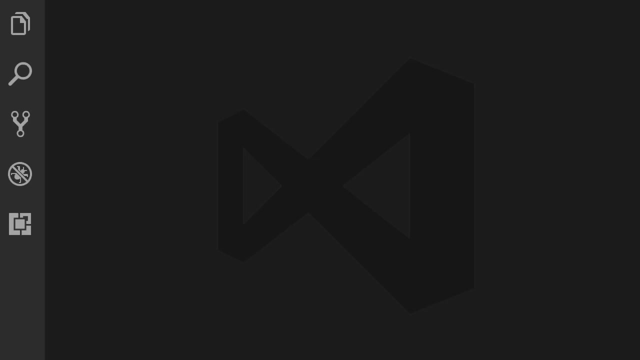 into the constructor of this class, And this is what we call dependency injection. Alright, now let me show you a quick way to create a service in angular. So we go to the terminal once again. you can switch to the terminal window or you can press control. 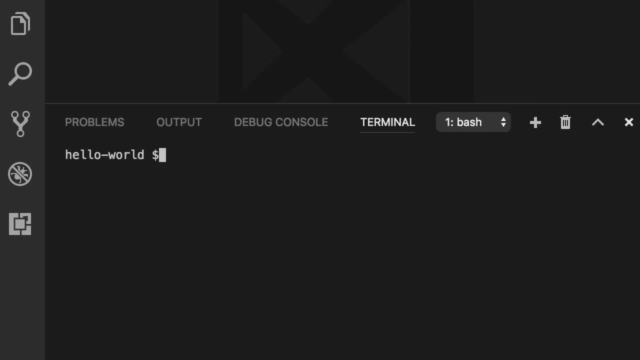 and back, tick in vs code. So here we have a small terminal window. we're going to use angular cli to generate a service, So ng g for generate. previously we used c for components. now we're going to use s for services. Imagine we're going to create a service for sending emails. 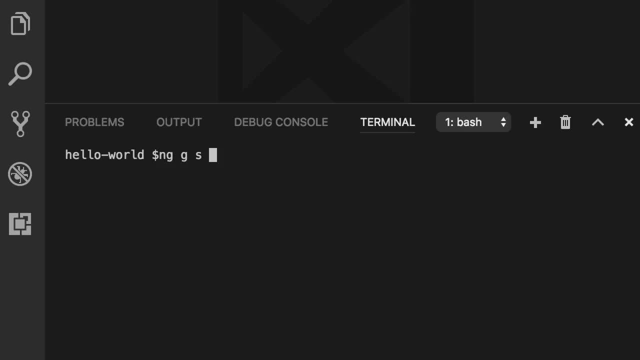 This service is going to call an HTTP endpoint somewhere for sending these emails. So let's call this email And note that here I just add the service name. I don't need to add dot service. Okay, So this generates two files for us. One is the actual service file. 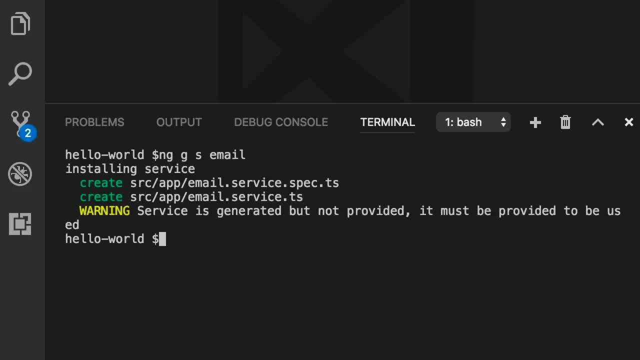 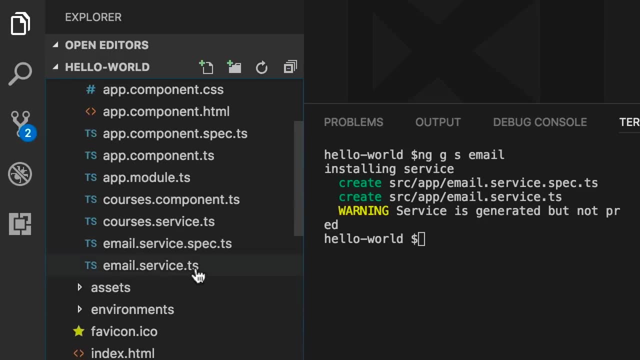 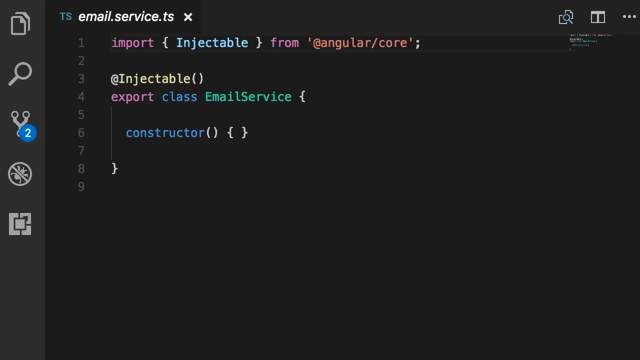 and the other is a spec file which includes some boilerplate code for writing unit tests for that service. So in the app folder, look, here's our new service: email dot service, dot ts. So we have a plain typescript class called email service. but there is something extra here that you didn't see. 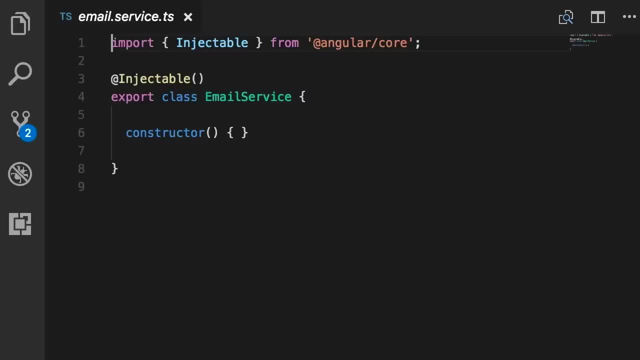 before We have this injectable, which is another decorator function similar to the component decorator function. Why do we need this here? We would need this decorator only if this service had dependencies in its constructor. For example, imagine here we had a dependency like log service of 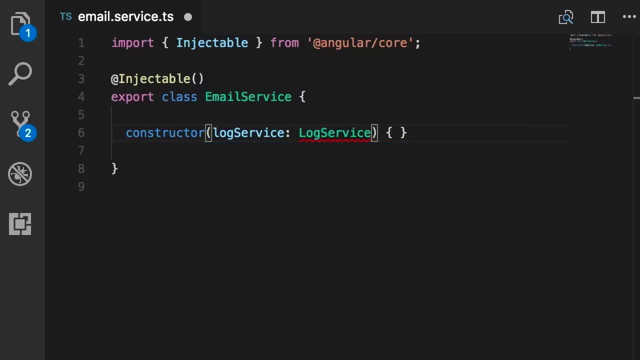 type log service. In this case, we need to apply this injectable decorator function on this class and this tells angular that this class is an injectable class, Which means angular should be able to inject dependencies of this class into its constructor. Now, we didn't use this decorator. 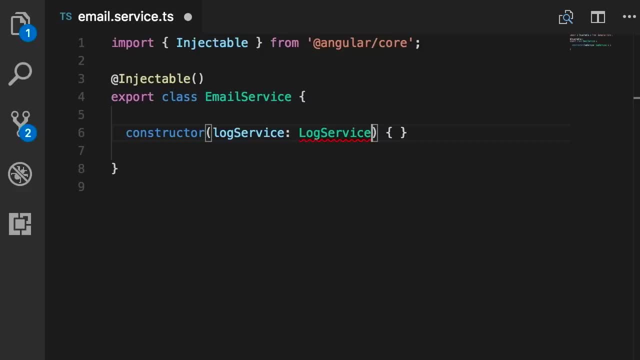 when defining components, because when we use the component decorator, that decorator internally includes this injectable decorator. So that's all about injectable. And, by the way, note that this decorator function is defined in angular slash core library. Alright, now I want you to use what you have learned in this section and build a page like this: 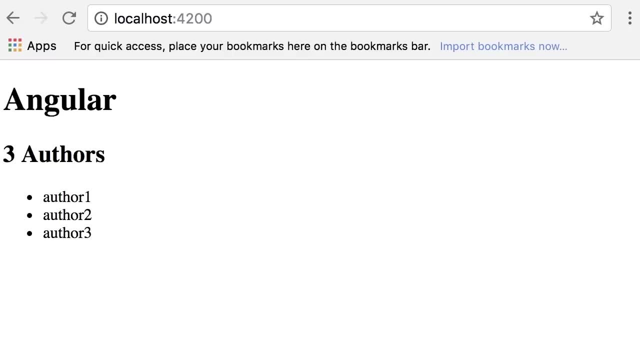 So, apart from the main heading of our application, we have a heading that includes the number of authors. So here we have three authors, and below that we have the name of these authors, rendered using ul and li. So use angular cli to generate a component and a service and write all the necessary code. 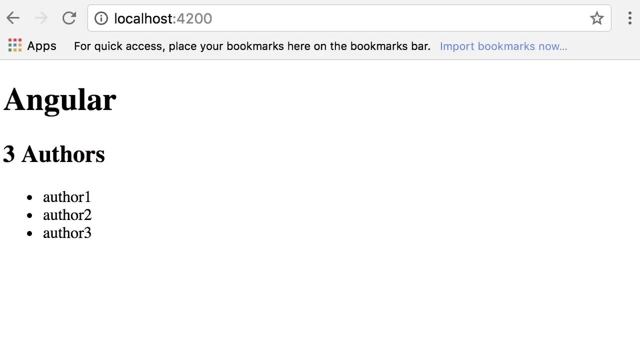 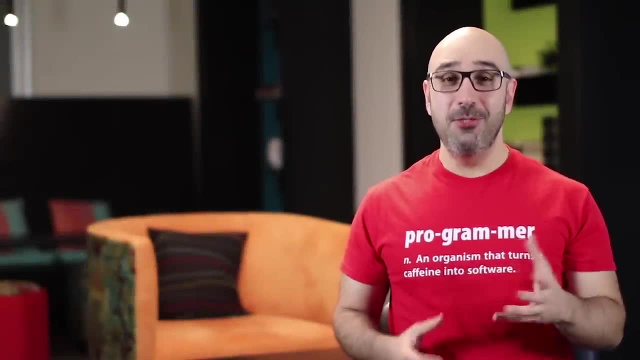 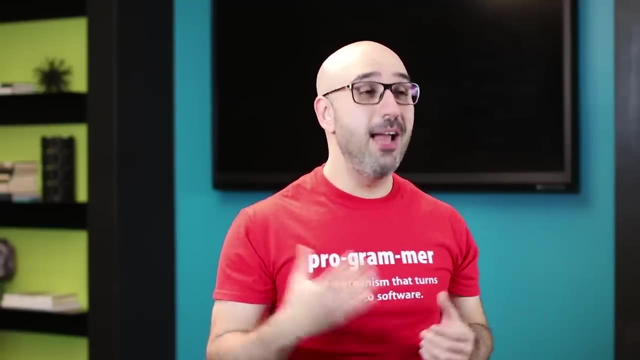 to render a view like this. You can see my solution in the next lecture. I love your enthusiasm for learning angular. As I told you before, this tutorial is part of my complete angular course, where you will learn everything about angular, from the basic to the advanced topics, all in one course. 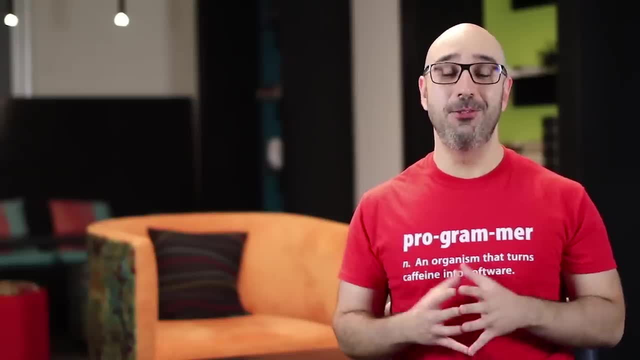 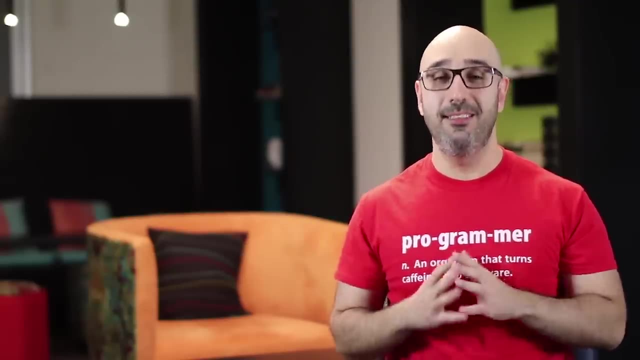 You seem to be determined enough to learn angular, and I'm so excited to see you made it this far. So I highly recommend you to click on the link in the video description and enroll in my complete angular course. So thank you for watching. If you enjoyed this video, please like it and share it with others. 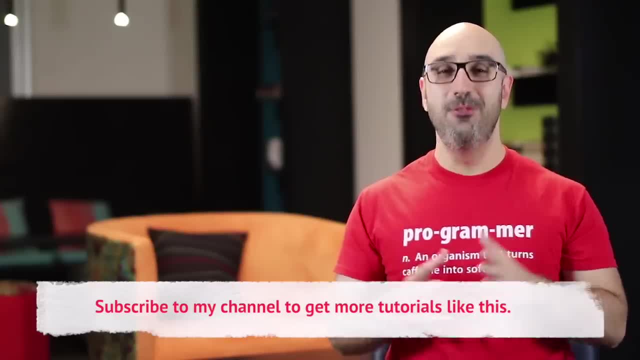 And finally, subscribe to my channel for free new videos every week. Have a great day, Thank you.